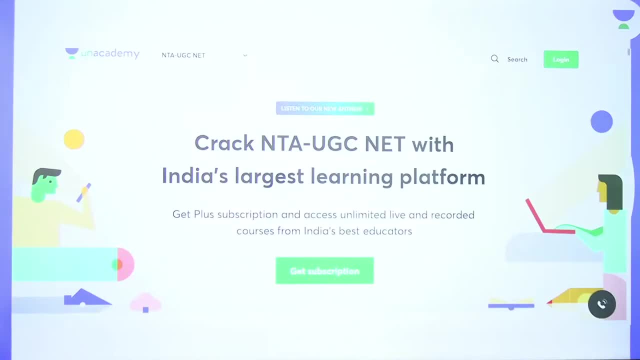 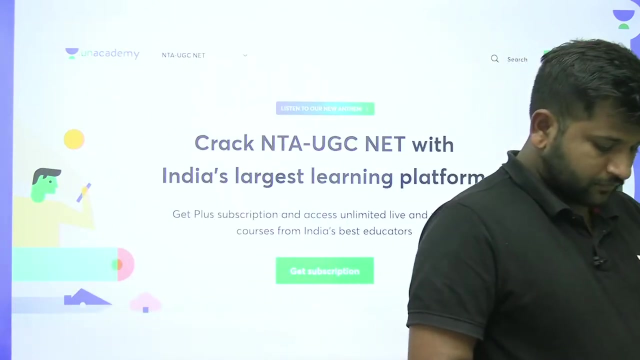 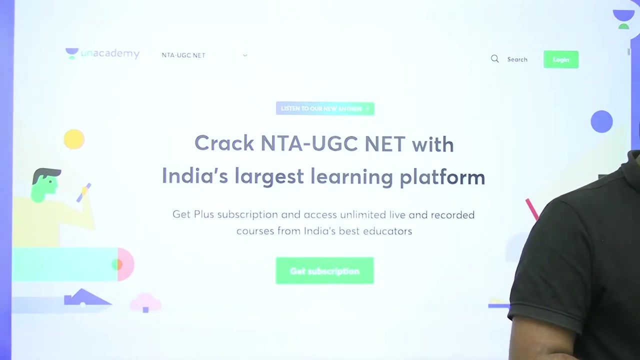 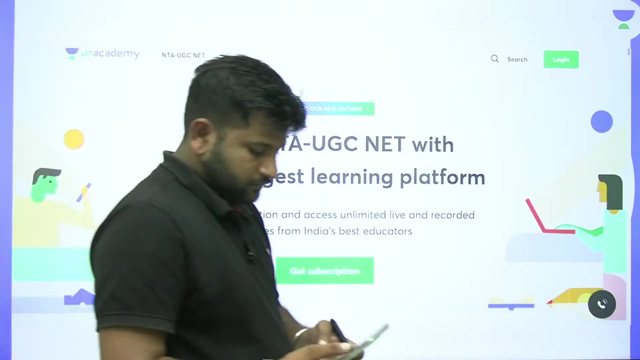 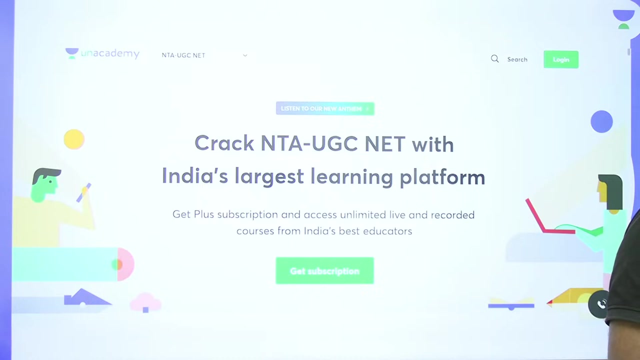 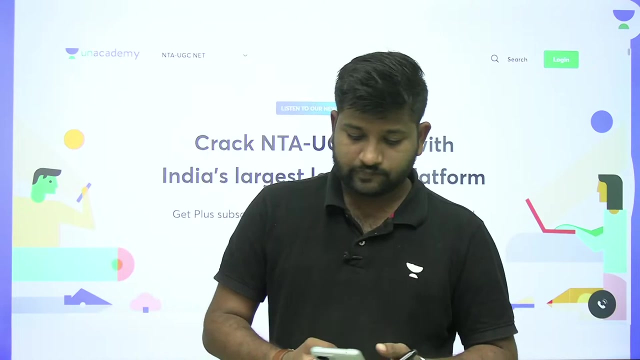 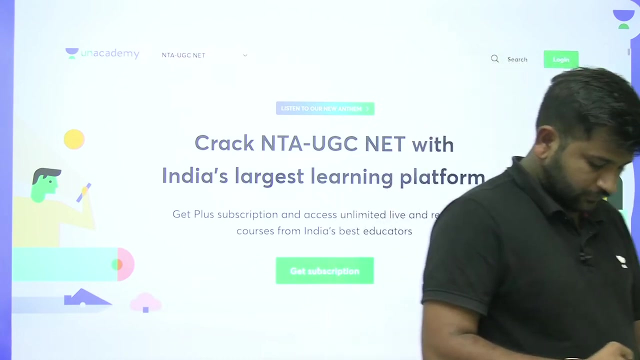 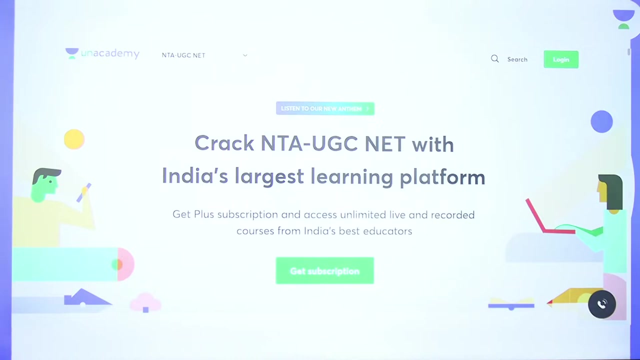 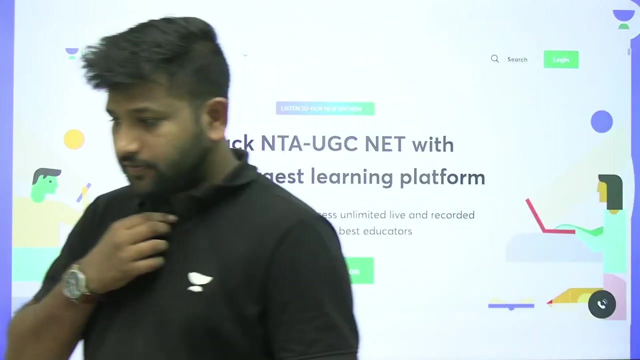 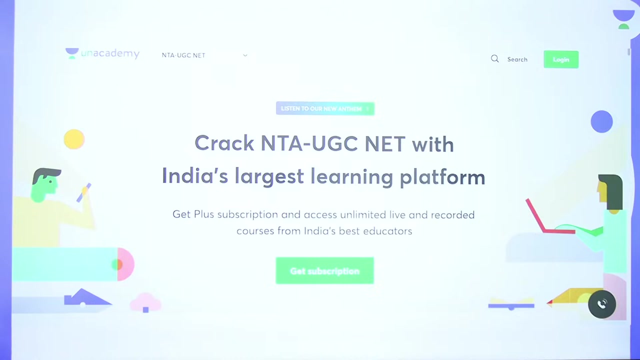 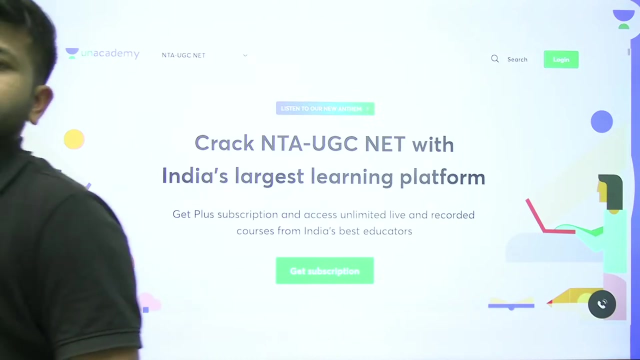 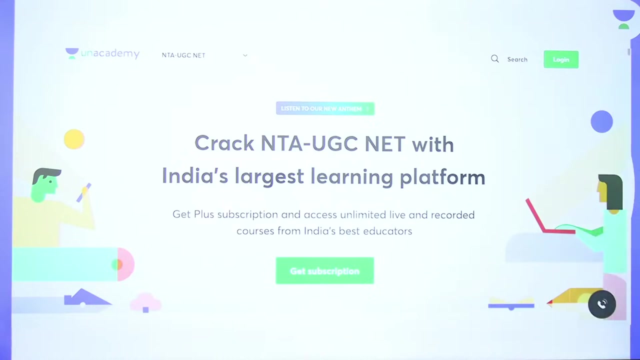 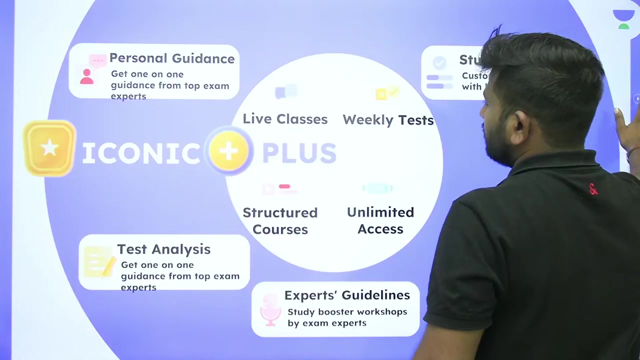 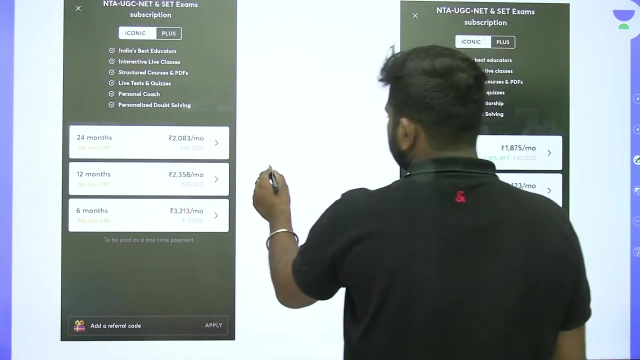 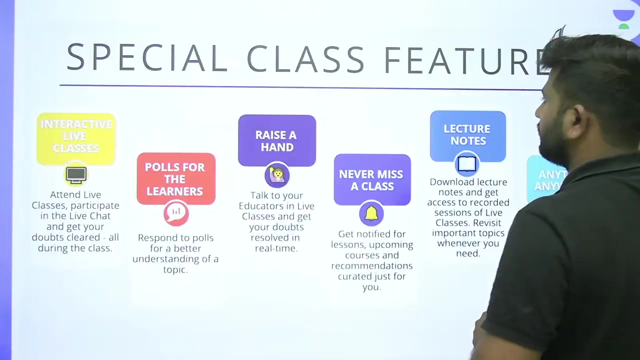 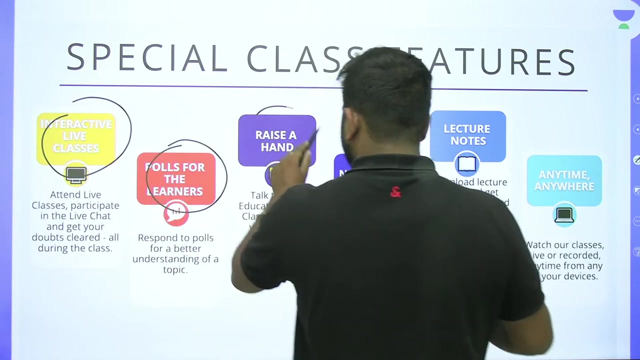 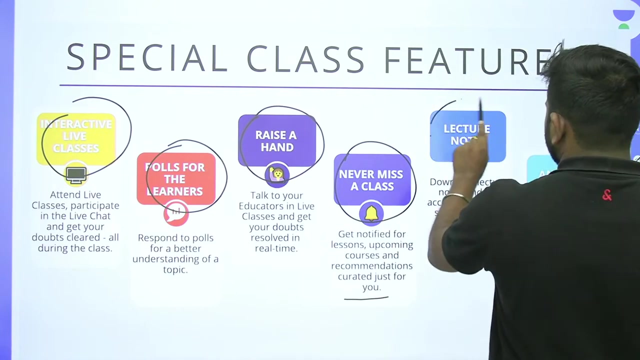 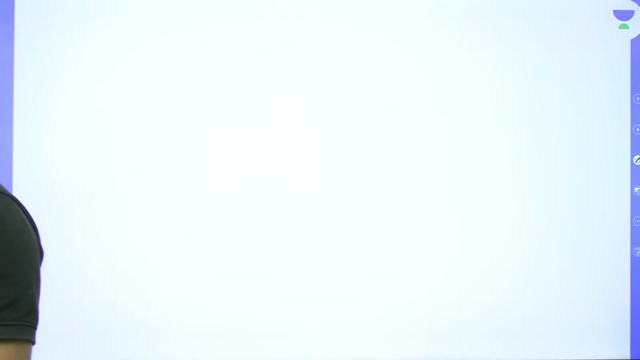 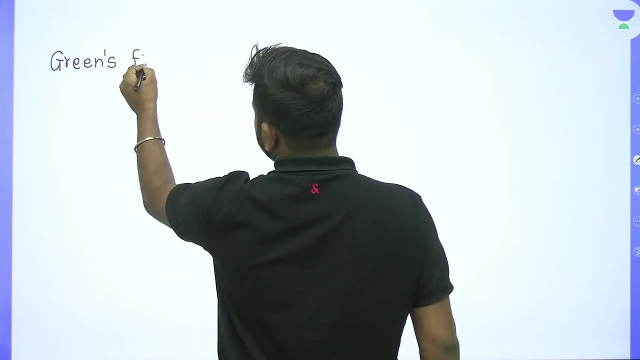 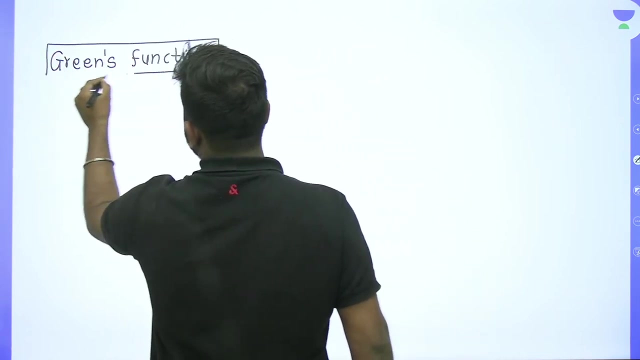 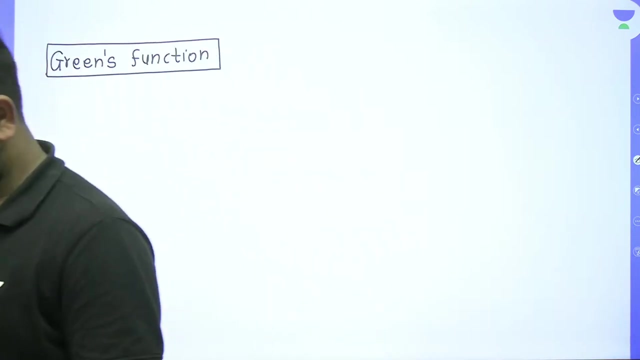 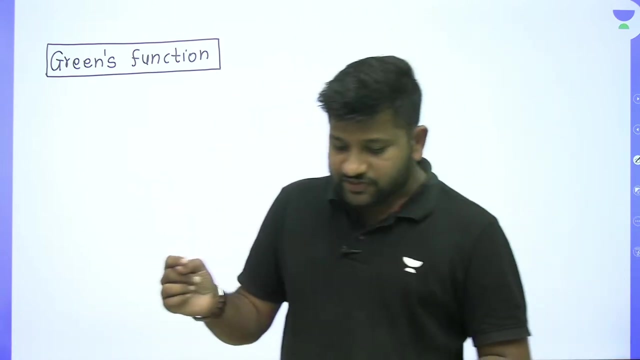 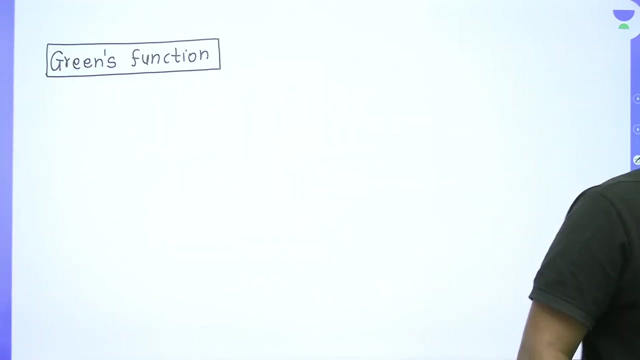 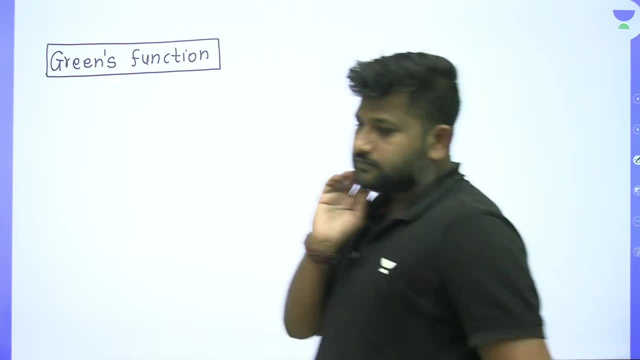 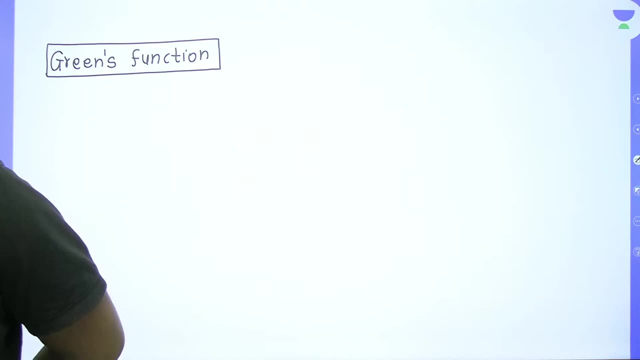 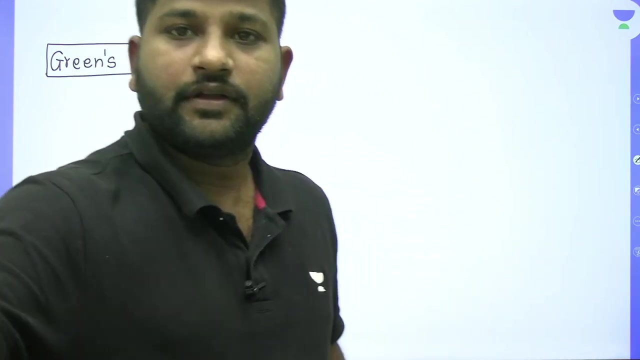 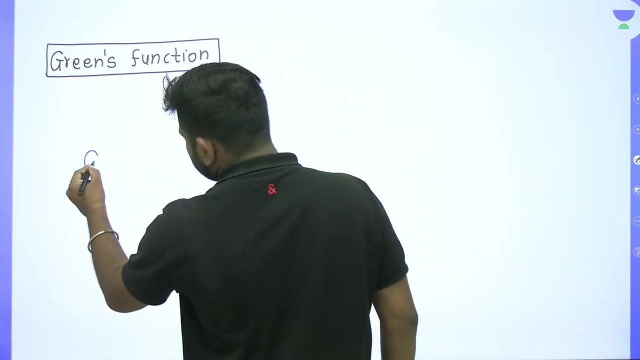 should join quickly. sanjay ji, good evening, good evening. ok. so in the last session we have discussed how to find out the greens function, how to find out about it. g of x- y is equal to. g of x- y is equal to. g of x- y is equal to. 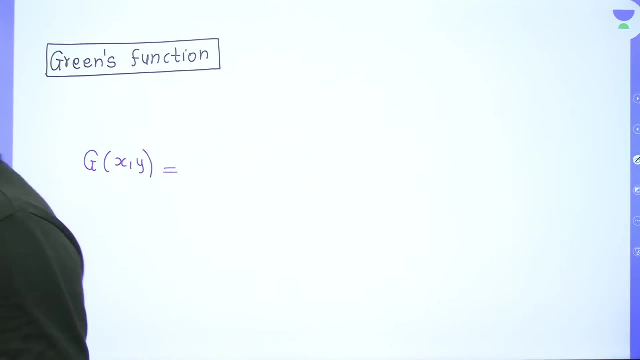 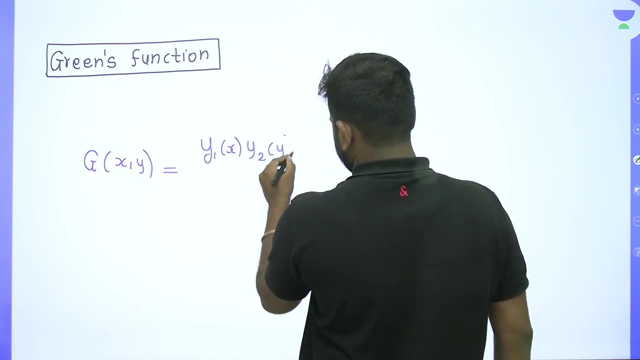 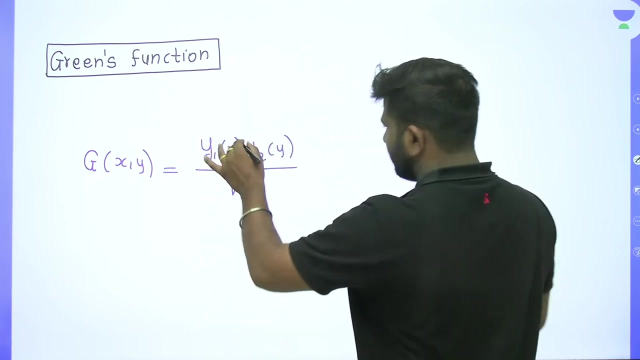 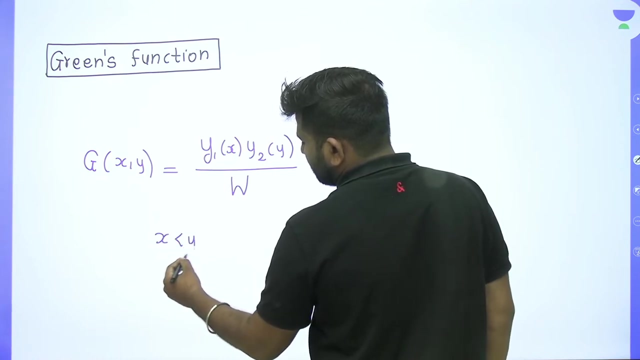 y is equal to y1 of x, y2 of y, divided by your wrong skin. and what was this? earlier I told you that what is inside will be small. that means this is for x less than y. so this is your greens function, and for the second region, your greens function. that is the job. x, y. 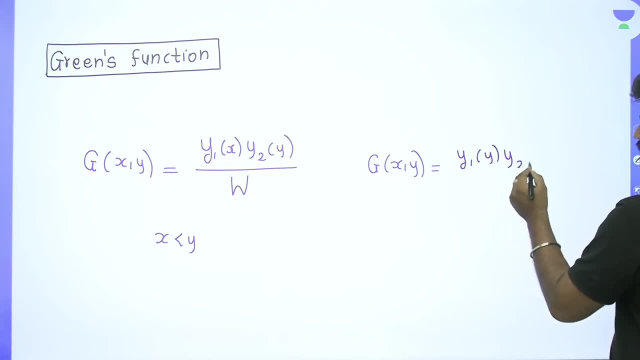 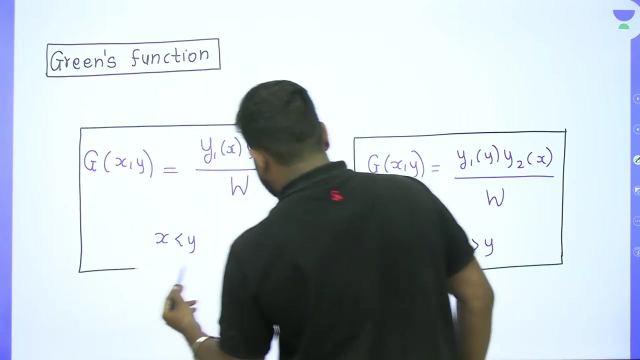 is equal to y1, y, y2, x, divided by wrong skin, w, and this is for whom you are, a y, whatever will happen here will be less. that means x greater than y for you. this will be left. we had a discussion in the last session. now we will solve some numericals on it and we 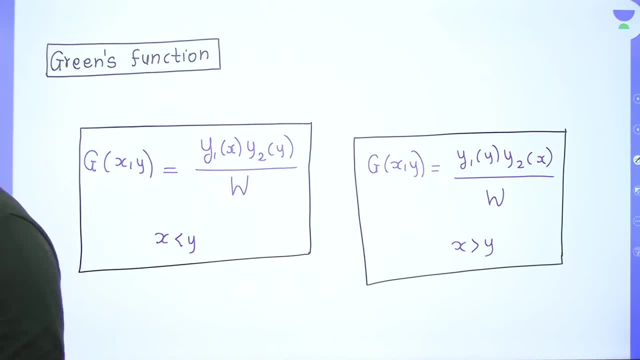 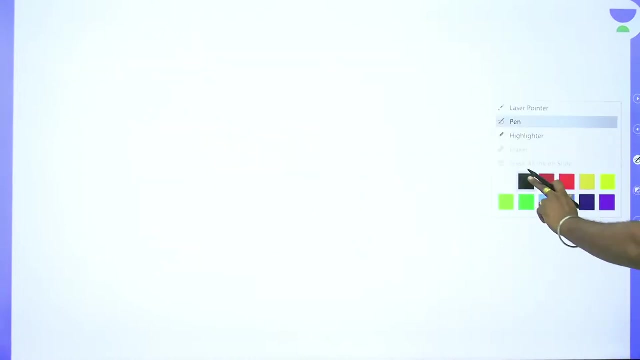 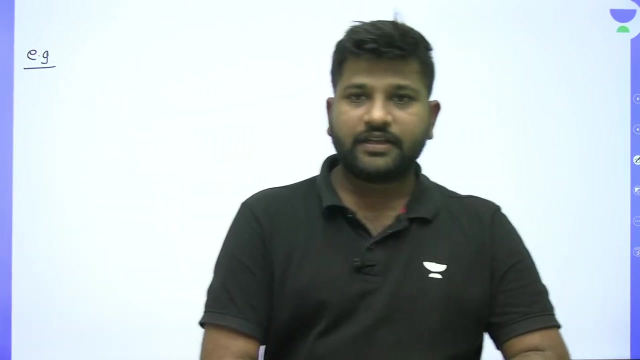 will get the idea. what types of questions can you ask? Okay, let's move ahead. let's discuss one example, example. just take the example. we are taking the example here. Okay, Okay, find the Green's function of the boundary value problem. 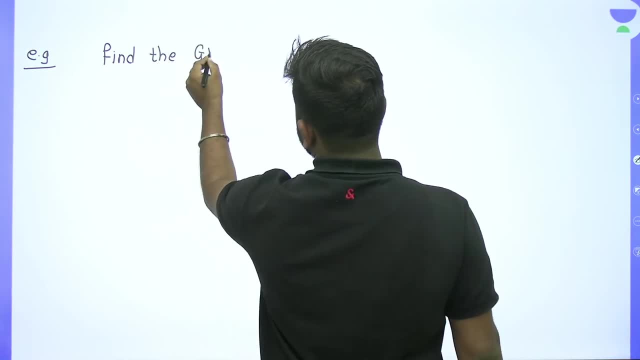 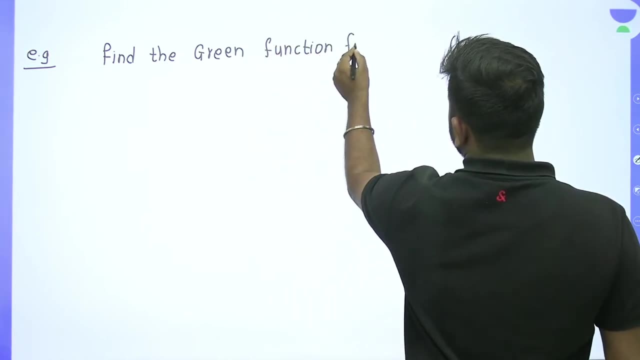 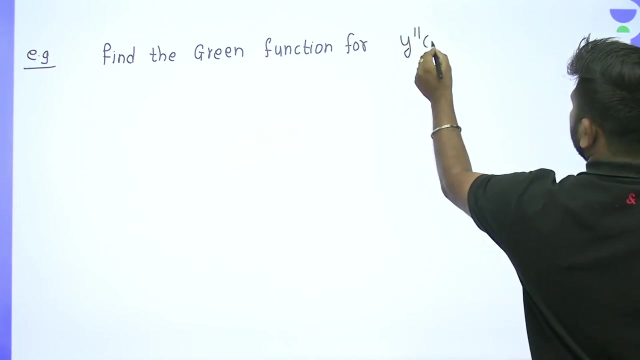 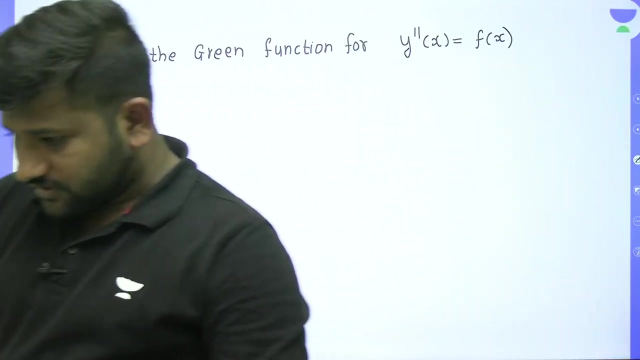 find the Green's function, find the Green's function, for what we have to find out here is: you have to find out this Green's function, for which y double prime of x is equal to f of x. and they have asked to find out the Green's function. 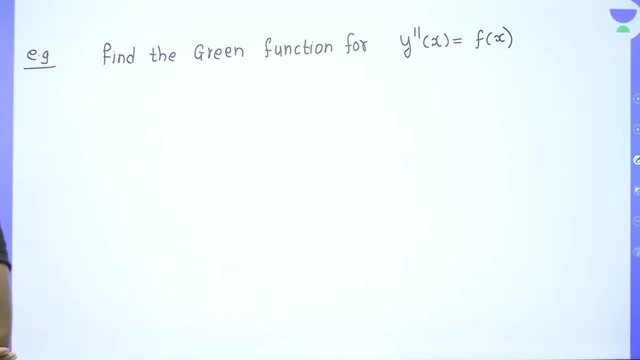 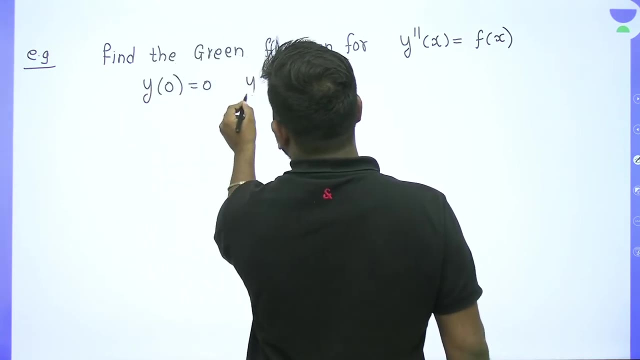 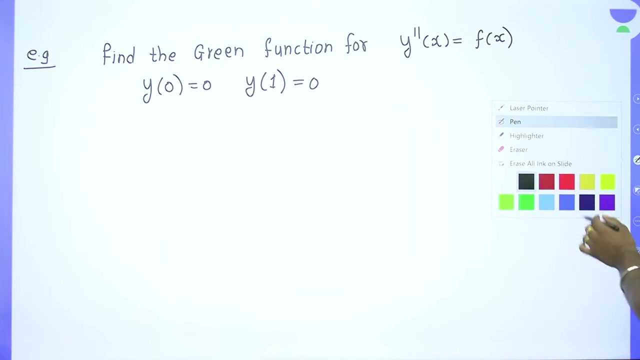 so for that we have to find out the Green's function you have given the boundary y of 0 is equal to 0 and y of 1 is equal to 0, so this is the boundary they have given. so this type of questions in exam. 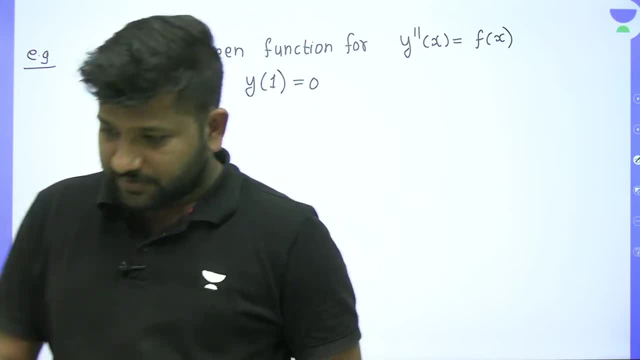 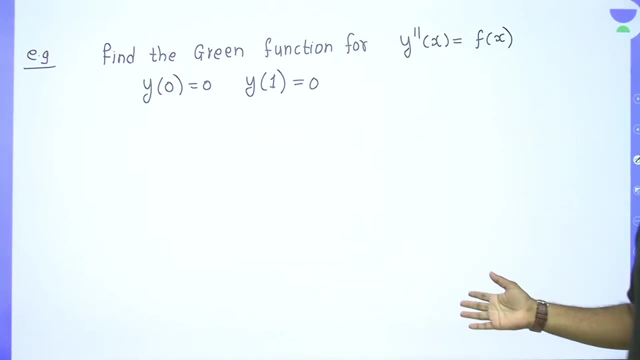 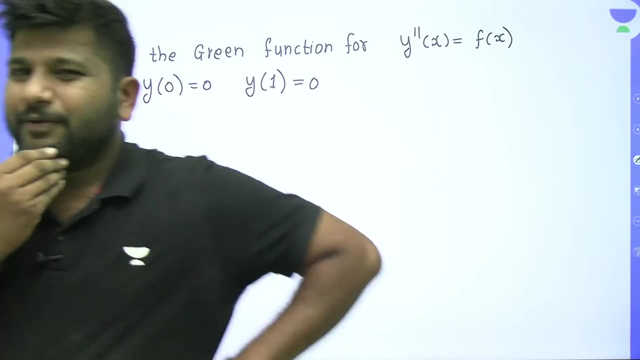 is asked. so for that, we have to find out the Green's function. so how you will find out the green's function? mark of question, you get from here, So don't neglect this. This is very important. Let's go ahead Now. you will think here that, Sir, we have to find out the green function. 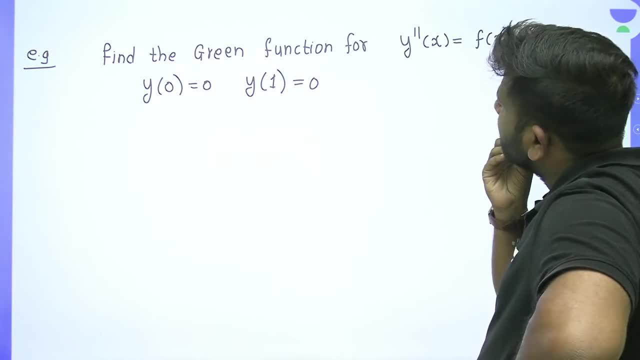 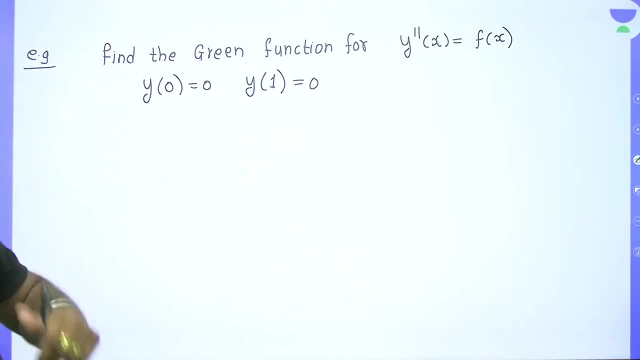 We have given y double prime of x. This is a box. How will we find out its green function? Here we have a solution and nothing else. Only this differential equation is given. Nothing else is given. So how to solve it? It is very simple. Just keep watching. 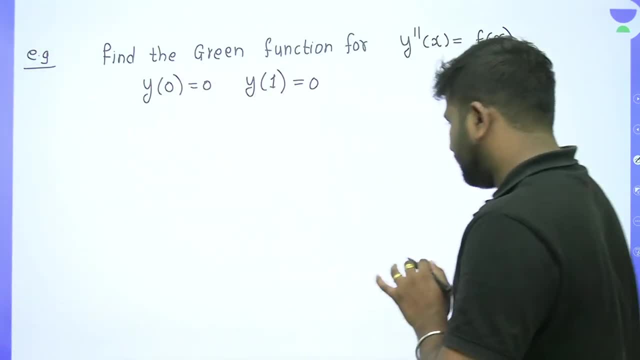 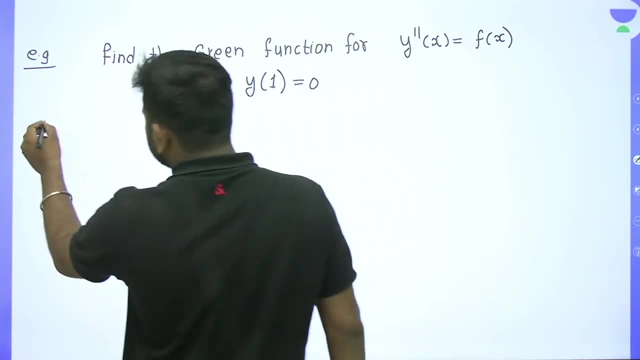 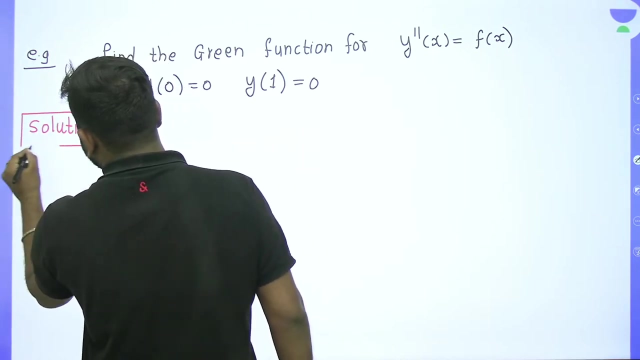 Now, if you understand this problem, then all the rest will be clear to you. There is no problem. So if we see its solution, then see what will be its solution Now in the solution here. see the solution of this problem carefully. 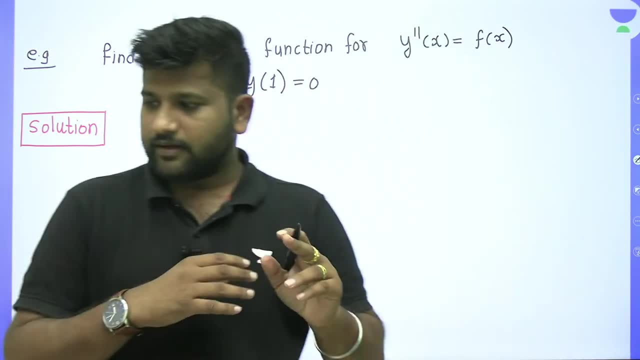 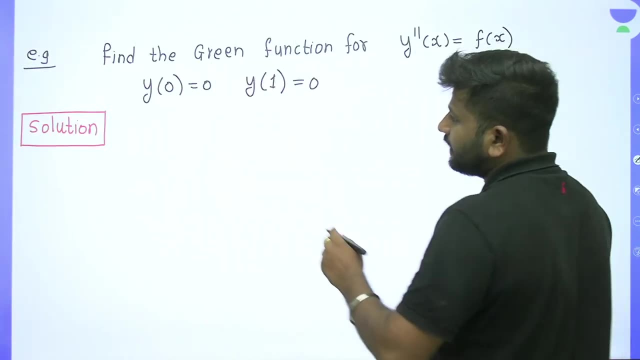 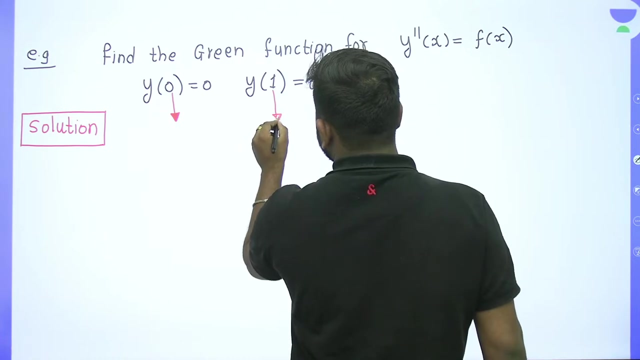 I will explain you a little slowly. You can solve the next problem easily. Now there are two types of boundaries here. If you see here, then what is zero here, What is your zero here And what is your one here? So first look at them in the boundary. 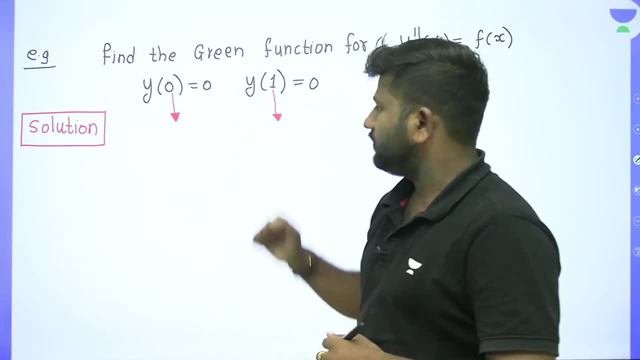 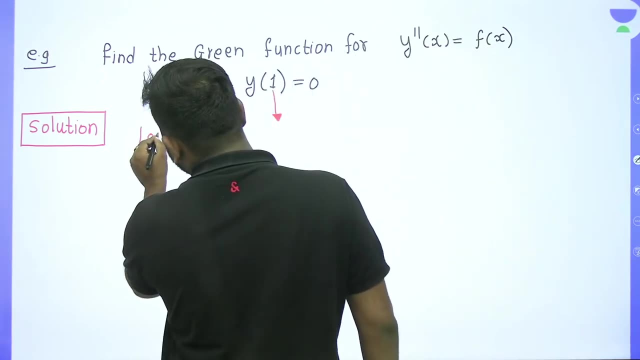 So this boundary condition is given to you. So here y is zero and y is one. So who is the lower zero and who is the higher one? So this is called the lower boundary. It is not called this. We will say that this is the lower boundary. 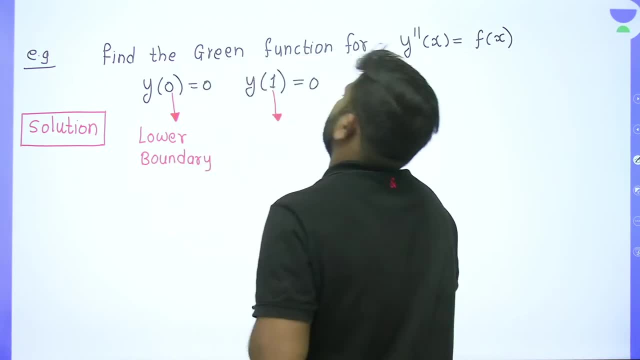 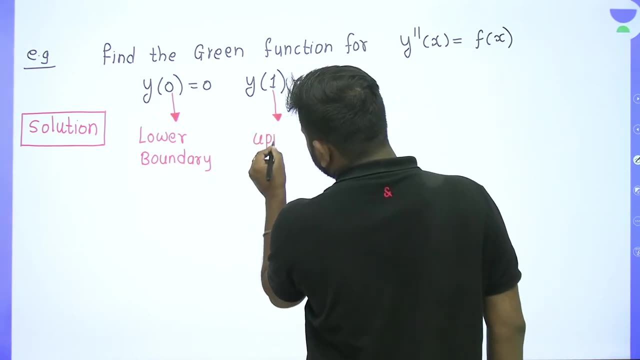 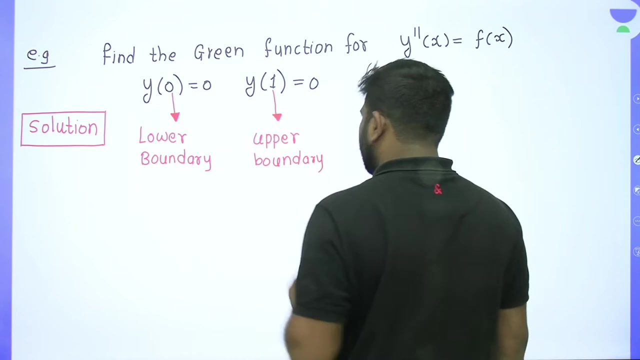 What is this Lower boundary And what is this here? This is one, So we will call this the upper boundary. So this is the lower boundary of zero. What is the corresponding of one? This is the upper boundary. So this is the lower boundary and upper boundary. 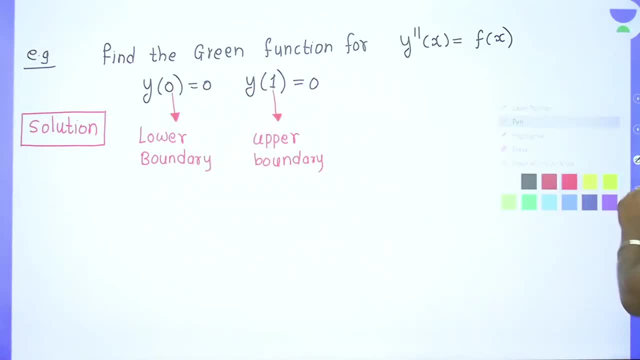 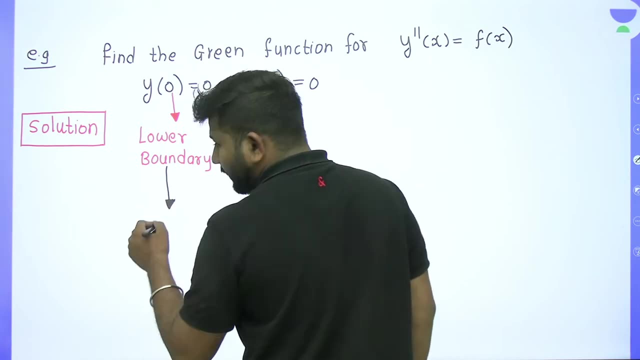 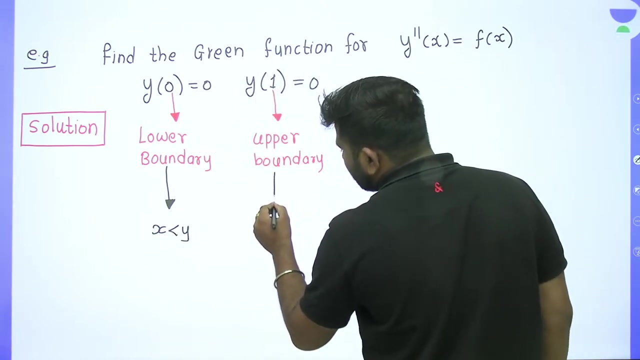 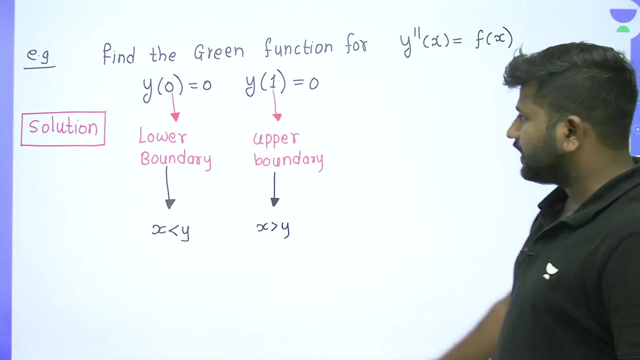 If there is a lower boundary, Okay. If there is a lower boundary, then the corresponding solution of the lower boundary will be x less than y, Okay, And the corresponding solution of the upper boundary will be x greater than y. So you should know this boundary from this boundary condition. 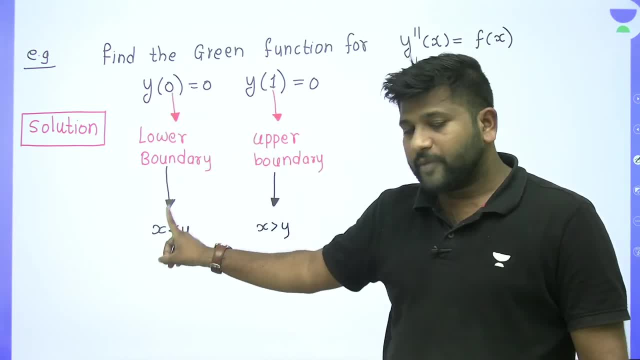 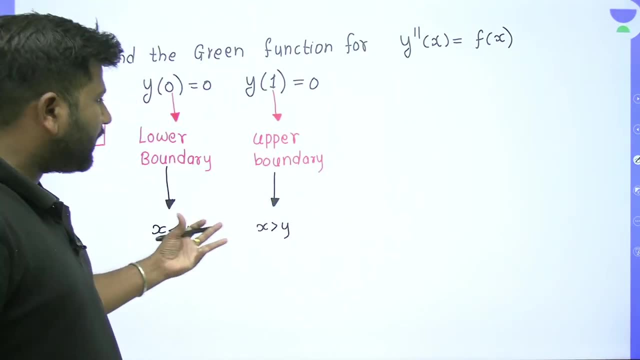 You have to remember this thing: If you have a lower boundary, then the lower boundary means x less than y. Upper boundary means x greater than y. If you understand these things, then you will have some problem. But when you go ahead, then all the things will be clear to you. 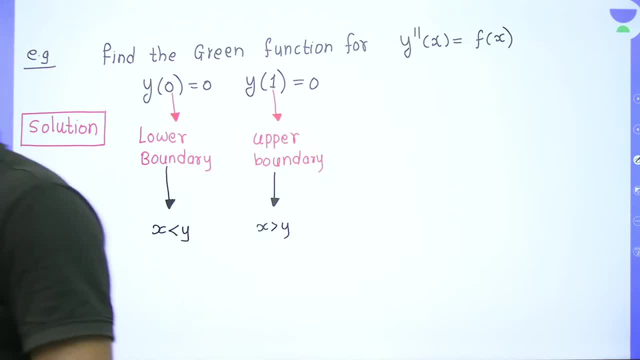 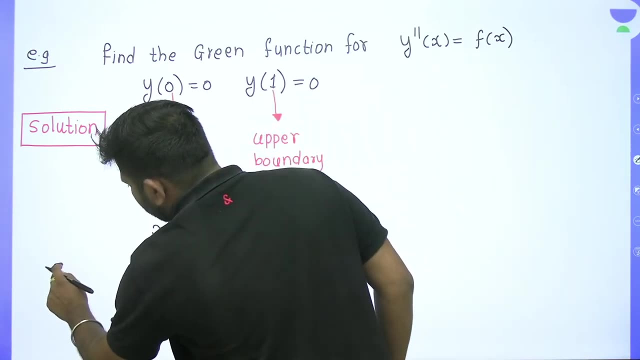 Don't worry about it. Good evening Ajit ji. Good evening. So let's simplify this. So here we have the differential equation. This differential equation is given to us here. What is that? y double prime of x is equal to f of x. 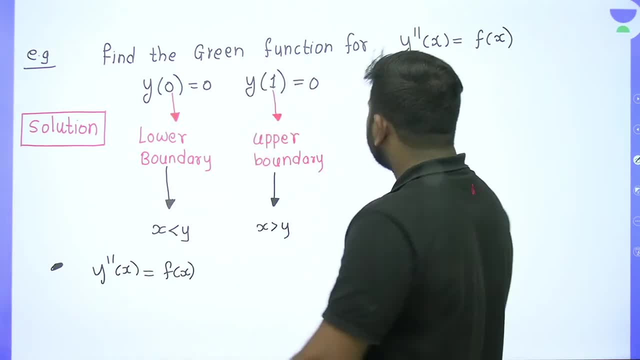 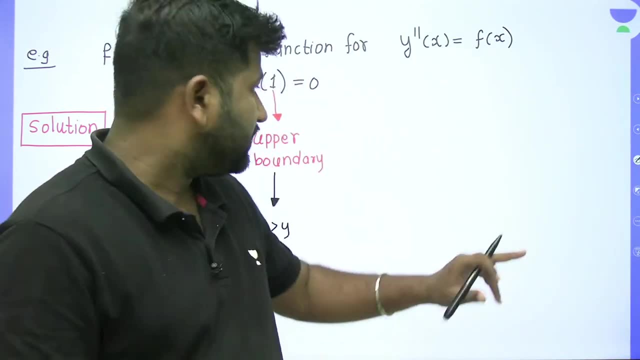 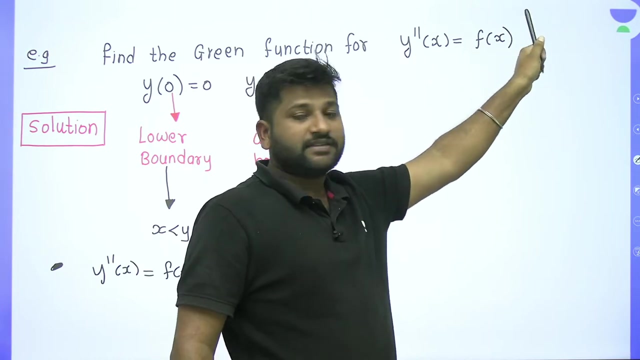 And keep one thing in mind: Whatever be the value of f of x, your Green's function is not dependent on f of x. Understand This f of x. if someone took sine x, someone took cos x, someone took tan x, 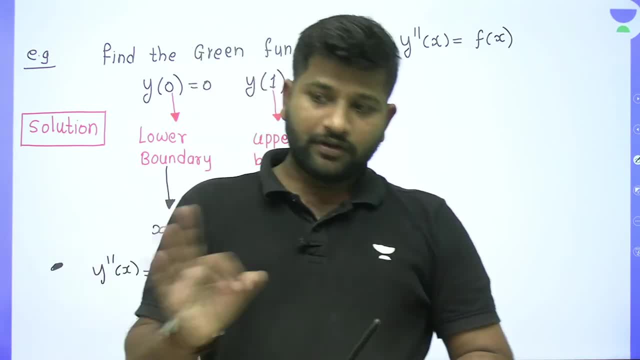 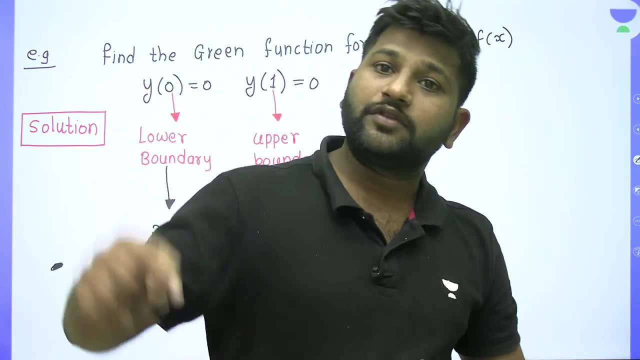 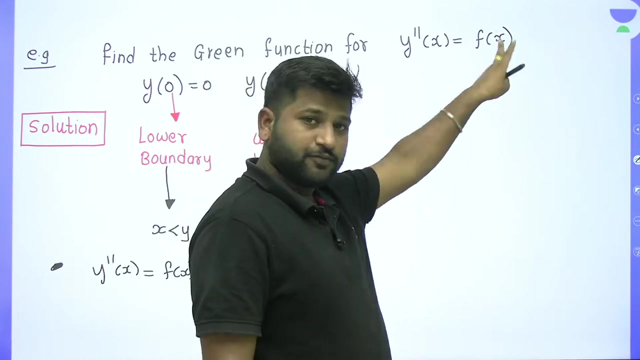 So for the given differential equation, the Green's function is independent. The Green's function is not dependent on this side. So where is the use of this side To find out the solution of the Green's function. Okay Differential equation To find out the solution of this differential equation. this is useful. 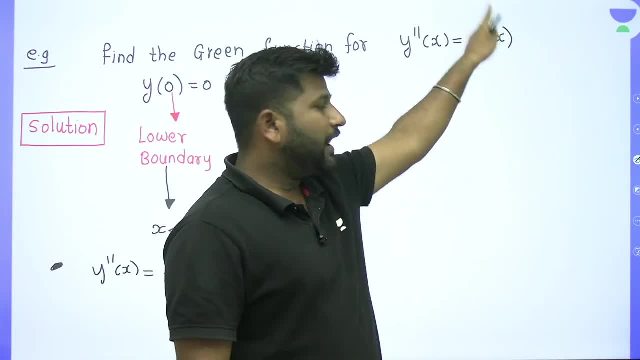 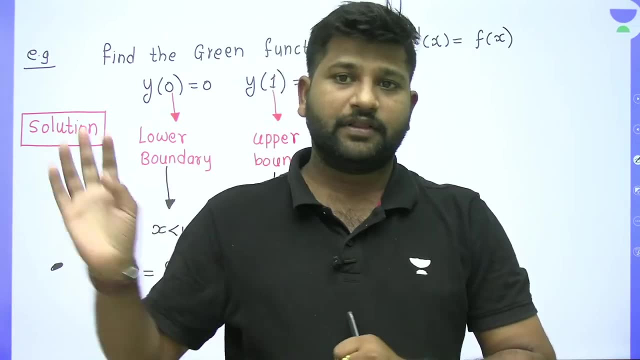 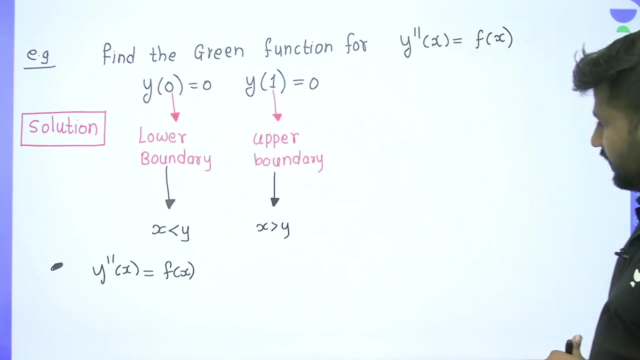 But to find out the Green's function, whatever be the f of x, there is no effect on the Green's function. Green's function is independent of f of x. Okay, Now let's simplify this. What will be y double prime? 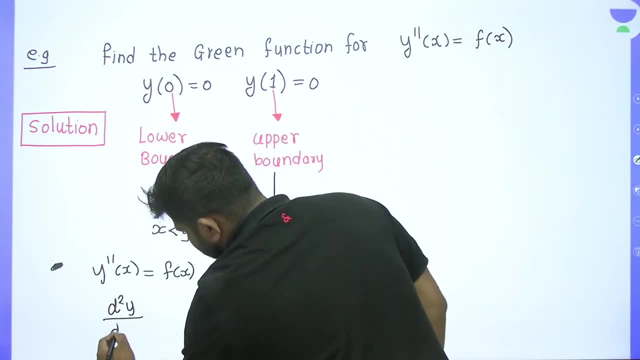 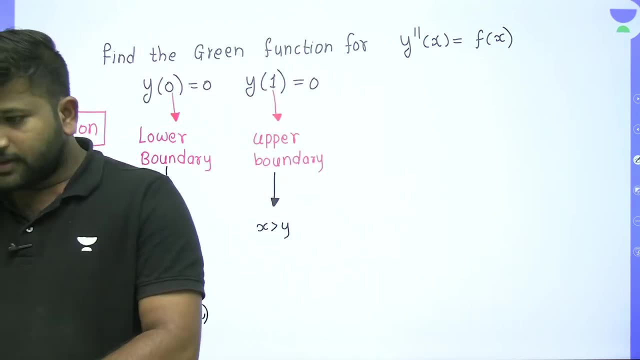 That means this will be d square y by dx squared. Okay, Which is equal to This is f of x. So this differential equation is given to you. Your Green's function is not dependent on f of x. So if you have notes, then see: 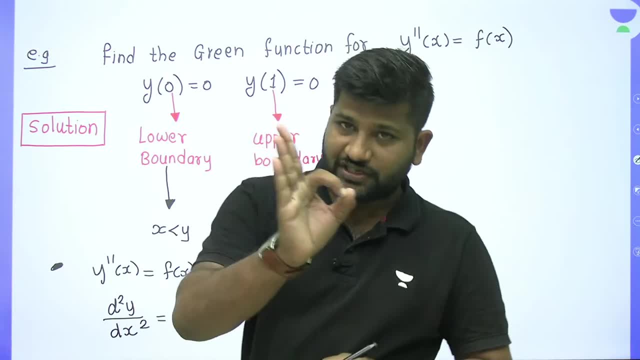 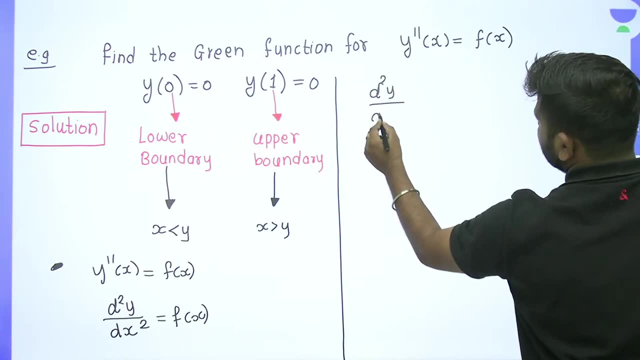 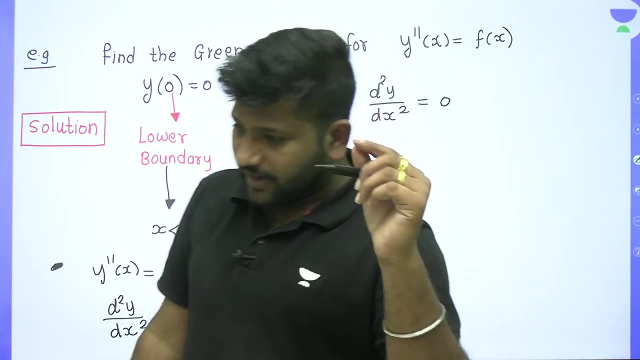 I have taken it. Consider the homogeneous equation. You take the homogeneous equation. That means you have to take d square y by dx. squared is equal to 0.. To find out the solution, you have to take this. I gave you this step in yesterday's session. 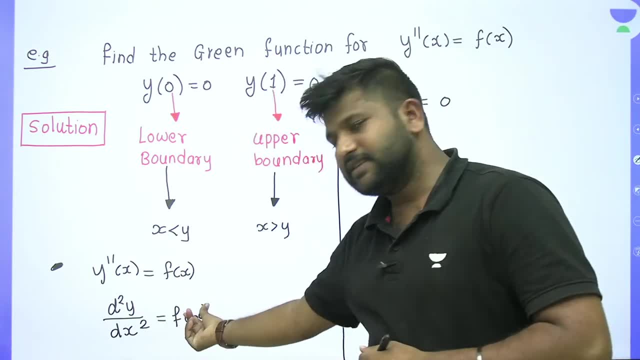 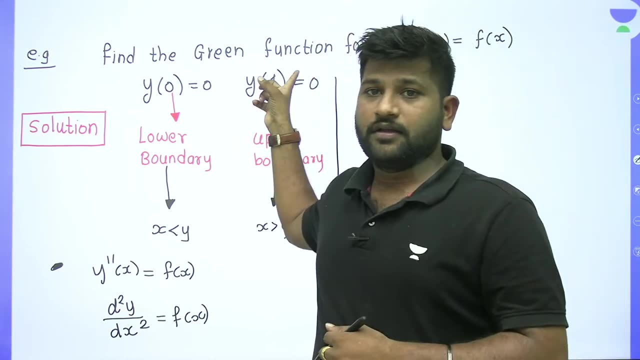 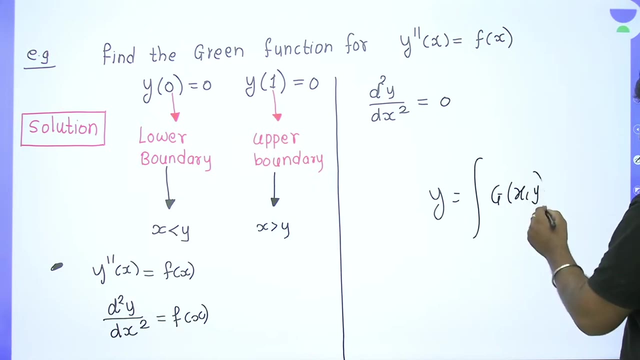 We are finding out the Green's function. That's why you have to take this f of x as 0.. Now where will this f of x be used? It will be in the solution of this differential equation. Keep this in mind. The solution of this is: y is equal to integration, g of x, y, f of x, dx. 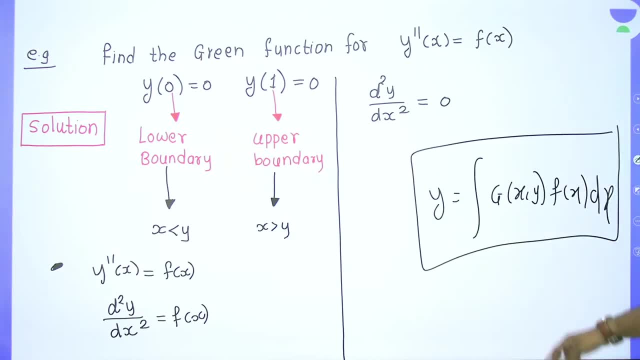 This is its solution. We will discuss that later on. So this f of x will only be used in the solution. This f of x has no use in g of x. So let's move ahead Now. what will happen if we find out the solution of this? 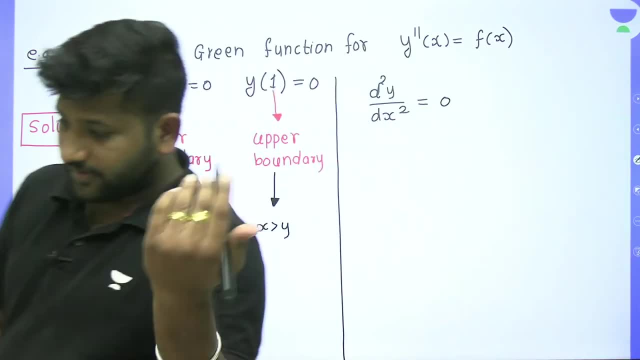 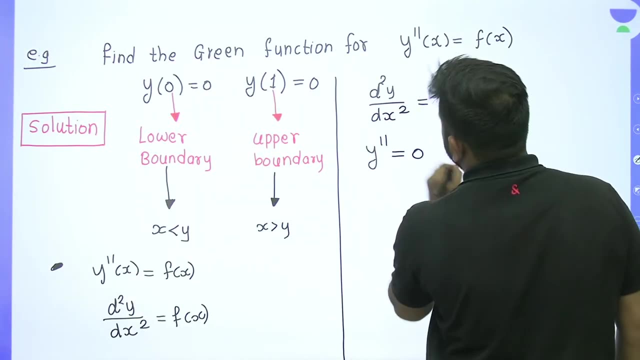 See. Now we have to find out the solution of this. How will we do it Now? there are a lot of doubts here. So can I say this: as y double prime is equal to 0? Right, Can I say y double prime is equal to 0?. 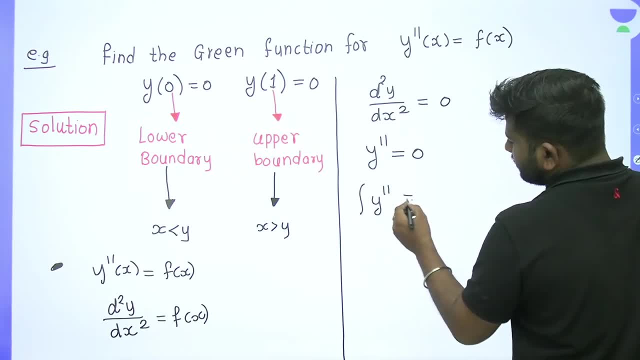 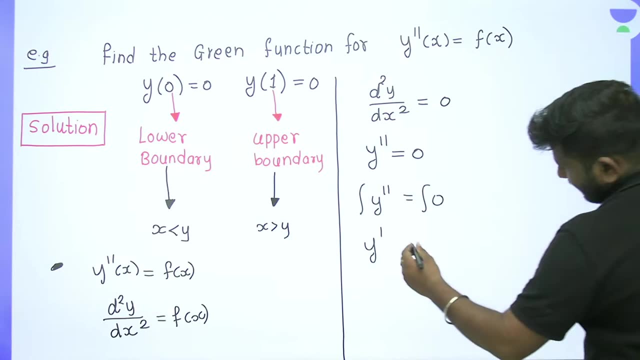 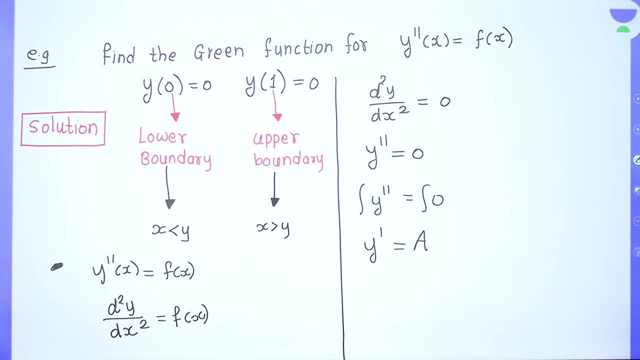 Yes, y double prime is equal to integration of 0. Right Now, if we take integration, then what will happen? 1 prime will be less And how much will be its integration? here It will remain 0. But a constant will come with it. 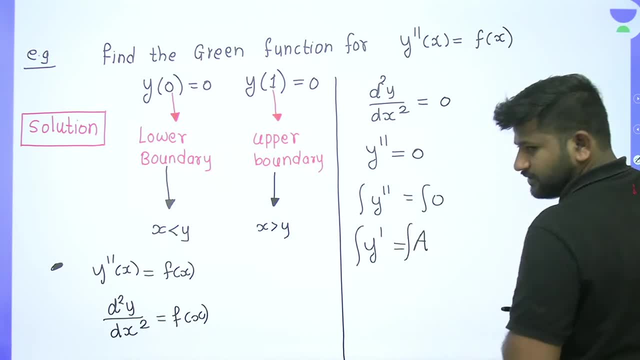 That constant is this. I can do it like this: Then take its integration again. Right, Take its integration again. If we take their integration, then what will happen? y is equal to ax And one integration constant will come again. So y is equal to ax plus b. 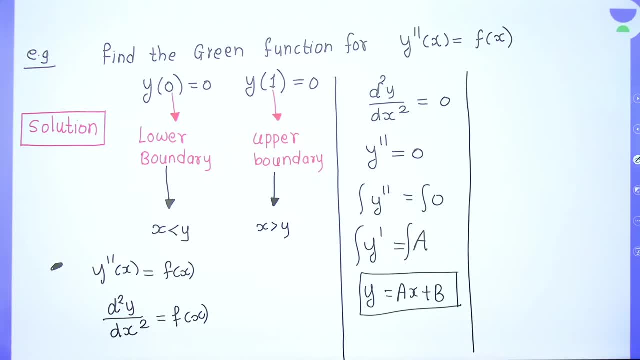 So this is the solution here Understood. So y is equal to ax plus b. This is your solution here. Is this clear to everyone? Right Now? you have to find out two things here. We have two reasons here. So the first reason we will see. 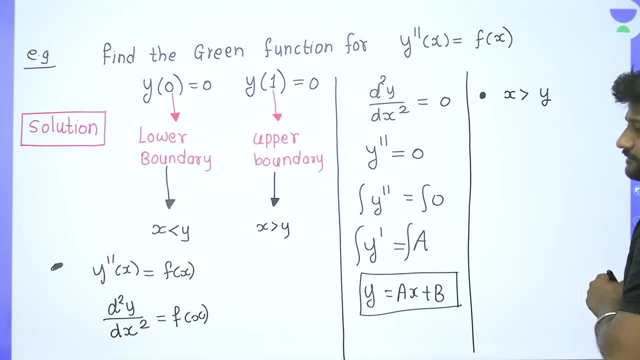 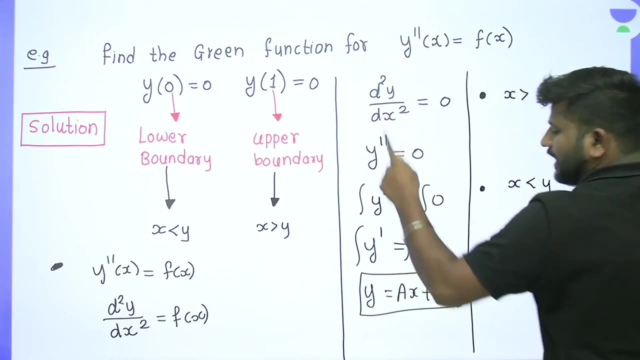 what will happen for x greater than y, Right. And the second reason is x less than y. So we need these two solutions. See what I told you yesterday. We are following the same step. First here, lower boundary, upper boundary. So here we have found the solution: y. 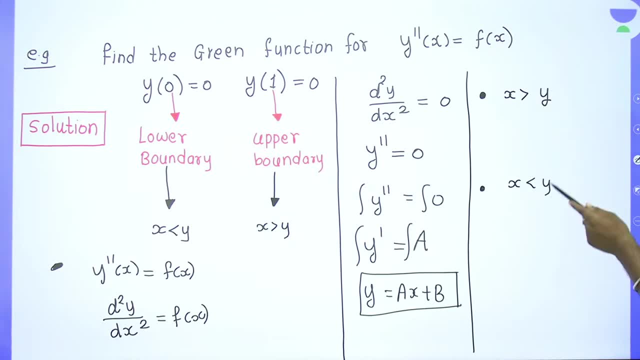 Now this y is for x greater than y And for x less than y. we will write here. So for this, let's say I am writing here that this is your y1.. So we will write y1 in its form, But here we will take a different constant. 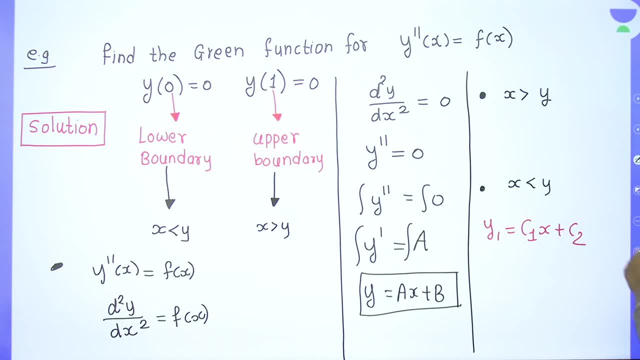 That is c1x plus c2x. We will write this, And what will happen for this? Let's say this is y2.. Same, There will be no changes in the solution, Only the constant you have changed. So this will be d1x plus d2.. 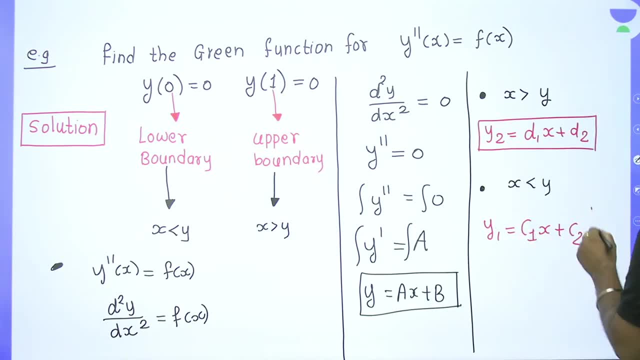 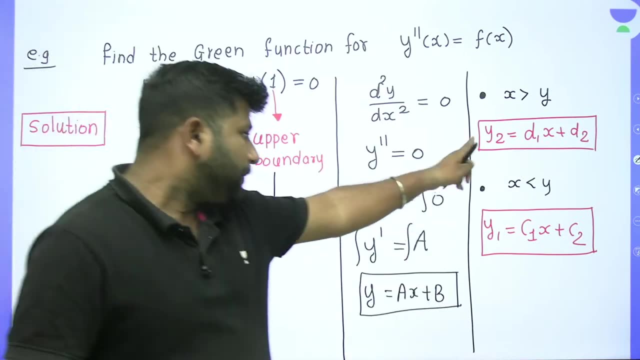 So this will be your y1 and y2 for the different regions. There will be no change in the solution. When you will do it for the region, just change the constant. So here you see: 1,, 2,, 3, 4- unknowns. you got. 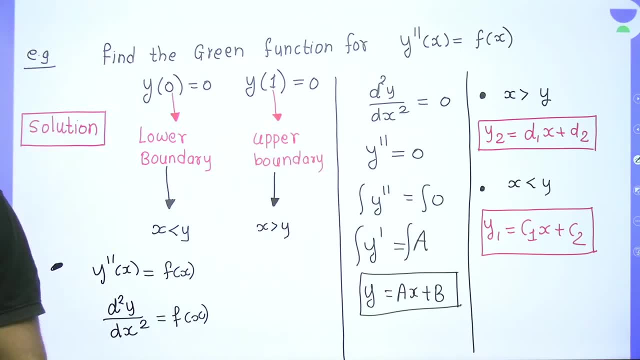 What I told you in the step, What steps you have to follow. So here what we got here, that is y1 and y2.. Are you able to understand what is happening here? Ok, It is simple. Now these four unknowns, that is, d1, d2, c1, c2. 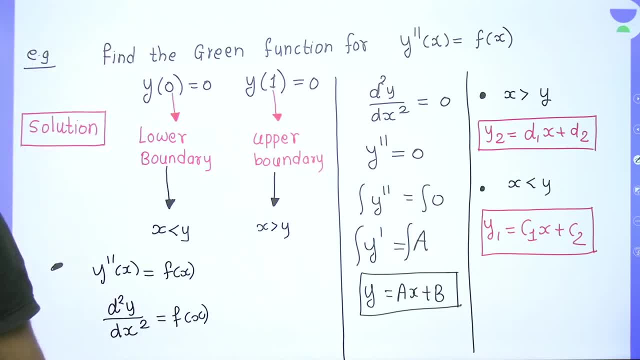 these are the two unknowns. So we have these unknowns Now. these unknowns we have to find out by using boundary conditions. We have to find out these by using boundary conditions. So apply the boundary condition. So I am moving ahead. 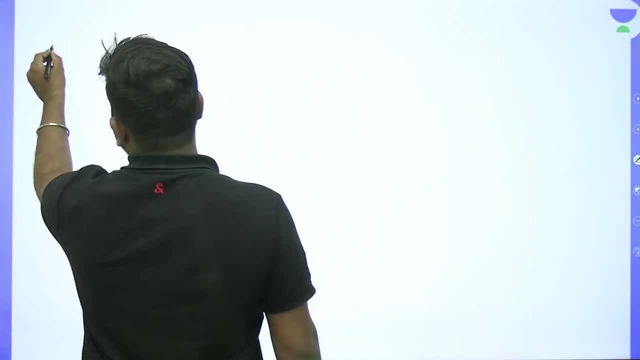 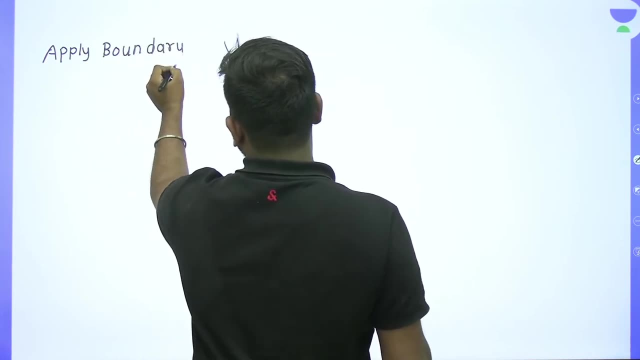 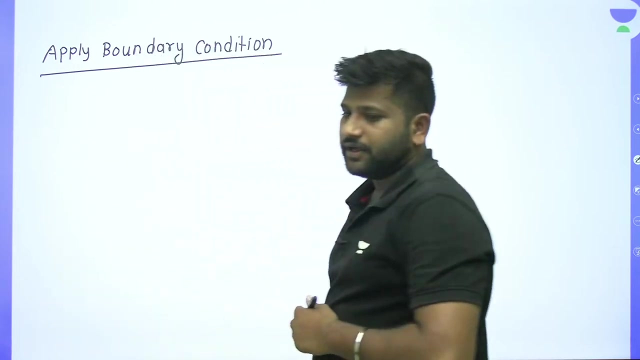 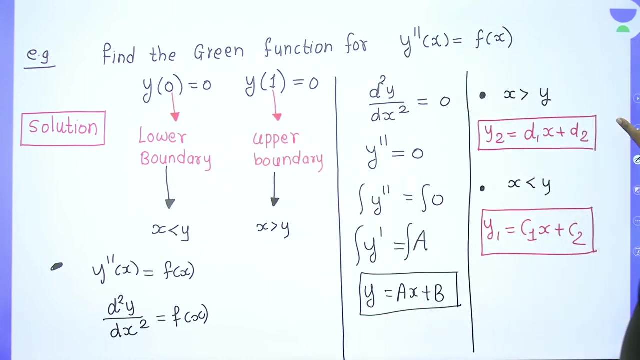 Apply boundary condition. What we have to apply: Apply boundary condition. Apply boundary condition. So you have to apply boundary condition. Ok, Now, if you want to apply boundary condition, then see what boundary condition you got First, boundary condition is: y of 0 is equal to 0.. 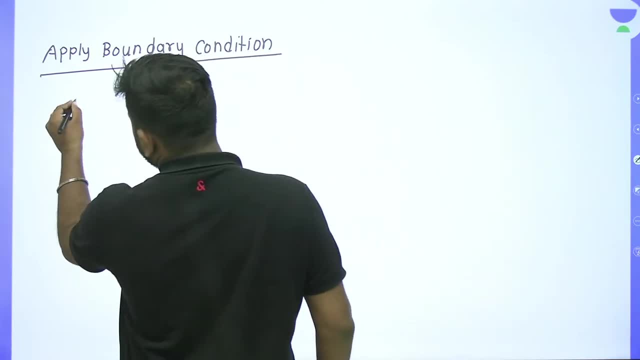 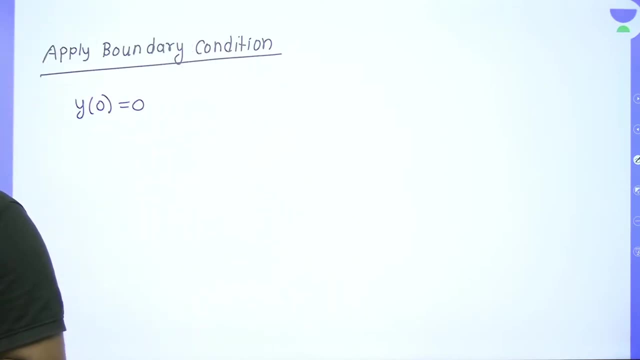 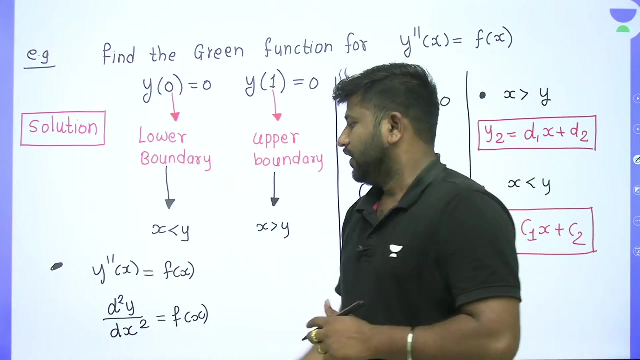 First condition is: first condition is: y of 0 is equal to 0.. first condition is: y of 0 is equal to 0.. This is your first boundary condition. Ok, Now, this first boundary condition that I have taken, that first boundary condition. 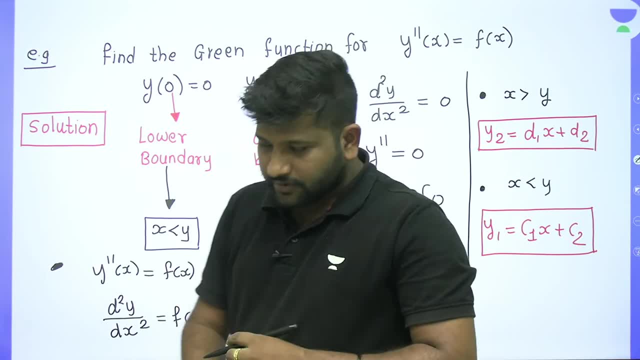 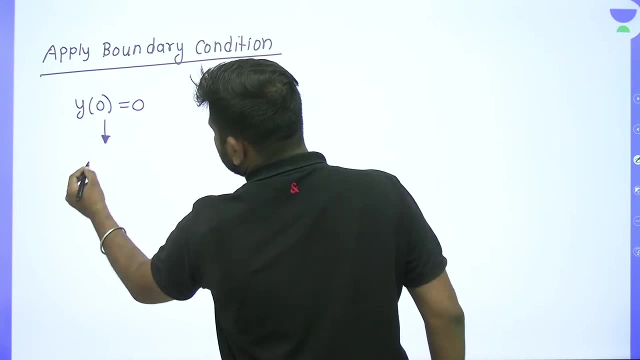 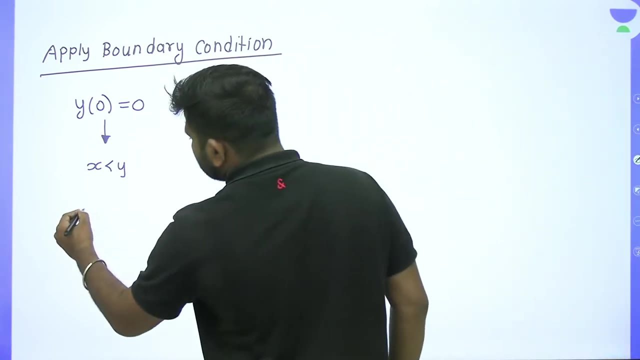 means lower boundary. Lower boundary means x less than y. That means what we are writing. this is for the x less than y. This is for the x less than y. Now, for x less than y, what is your solution? x less than y. 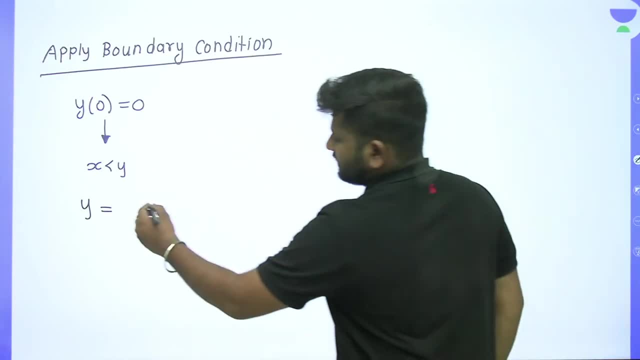 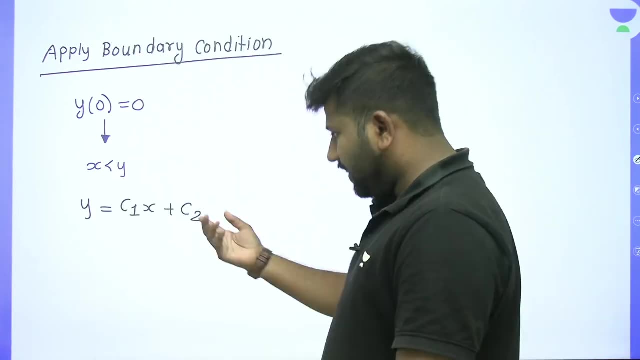 So, for x less than y, solution is c1x plus c2.. What is c1x plus c2.. This is your solution. This is your solution. Now apply boundary condition in this. Now apply boundary condition in this. So here, if y is 0, 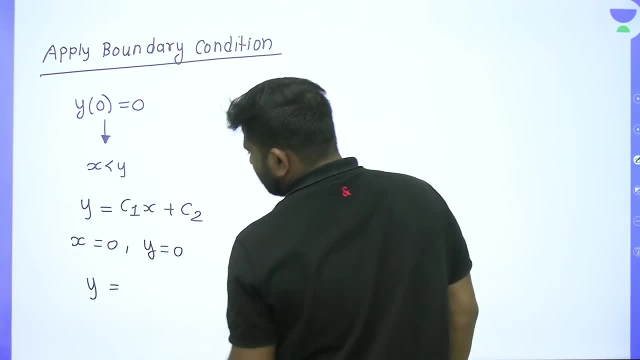 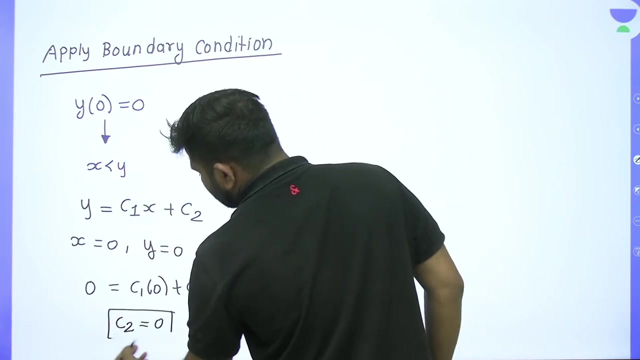 then what will be the value of y? It will be 0. That means what is the value of y? Sorry, If you have substituted in this, then what will you get? If you have substituted in this, then what will you get? Put y as 0 is equal to. 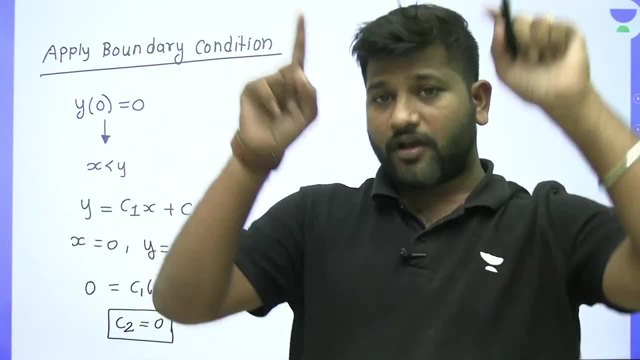 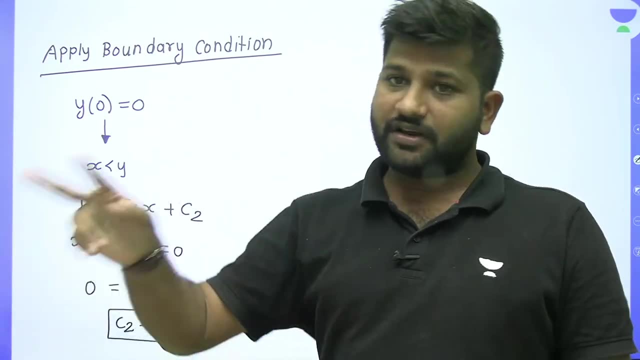 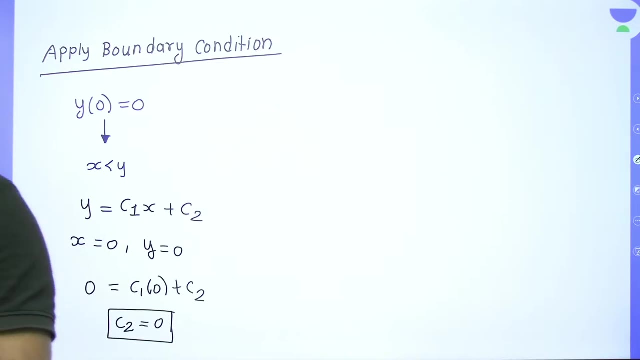 c1x, 0 plus c2.. That means you will get: c2 is equal to 0.. So for the use of boundary condition- that's why we have to use boundary condition here- see here, one constant is gone from the first boundary condition. ok, shivini ji, good evening, good evening. 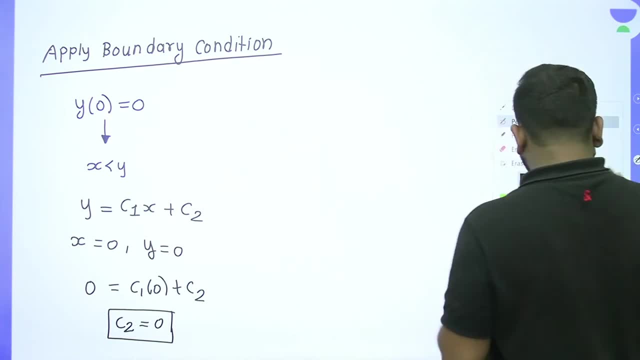 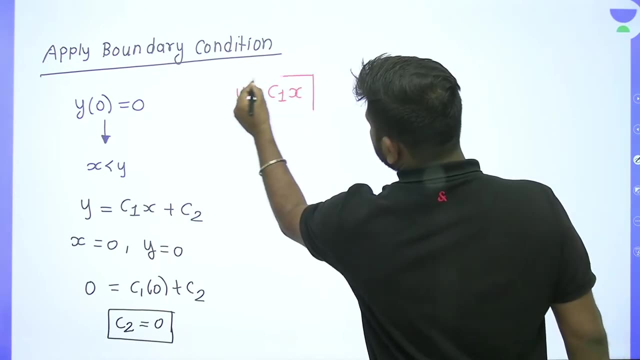 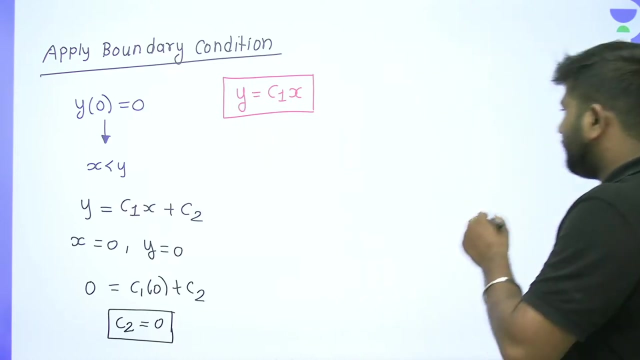 so i hope you understood this. that means your solution will be: if you put c2 in this, then y is equal to c1x. i hope you understood this. how it came? we have found out this boundary condition from this boundary condition. now we will use another boundary condition. 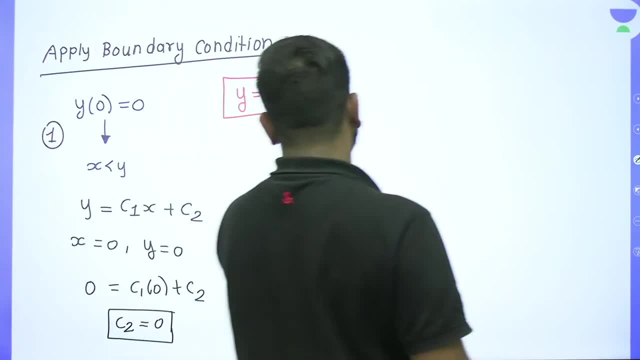 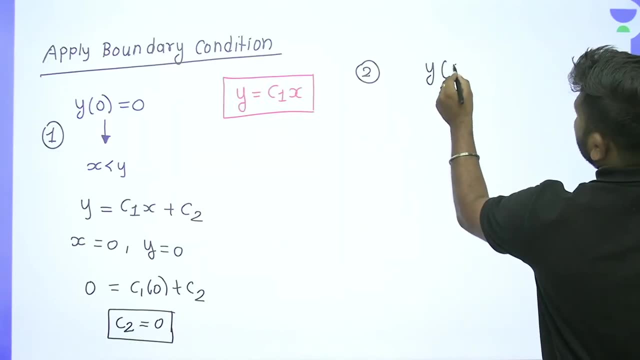 so this was your first boundary condition. now what is the second boundary condition? second boundary condition is: y is equal to 0. now which boundary is this, lower boundary or upper boundary? upper boundary means x greater than y. so for x greater than y, your solution is: y is equal to d1x. 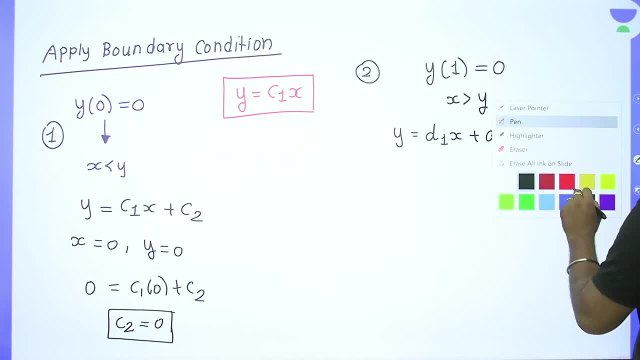 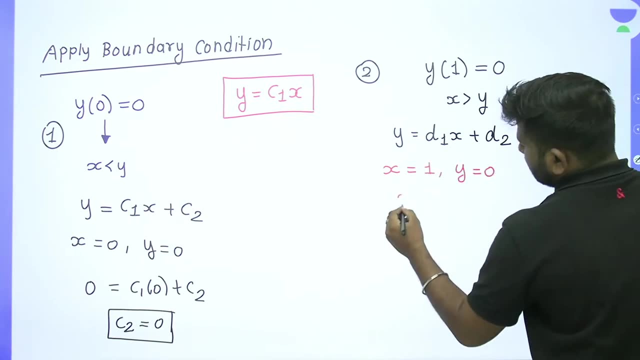 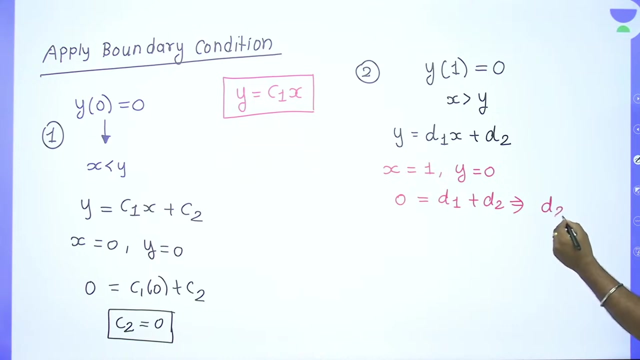 plus D1 plus D2, and in this you put the boundary condition that when X is equal to 1, the value of Y will be 0, that means 0 is equal to D1 plus D2, this implies that the value of D2 will be minus D1, so see this. there are two unknowns here too. now one unknown has disappeared in this by using boundary condition. 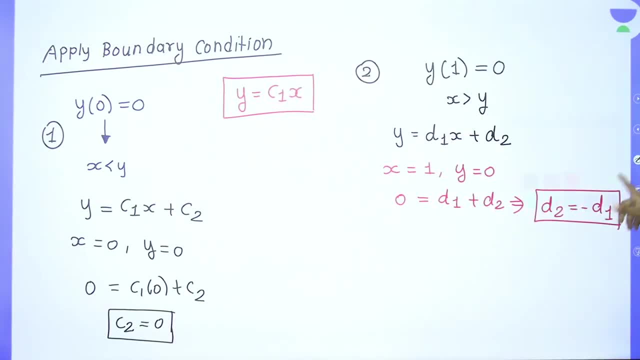 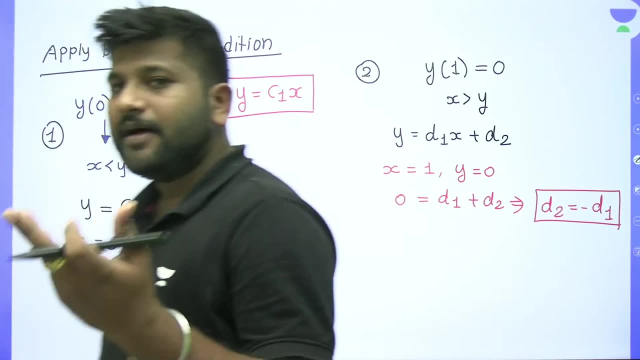 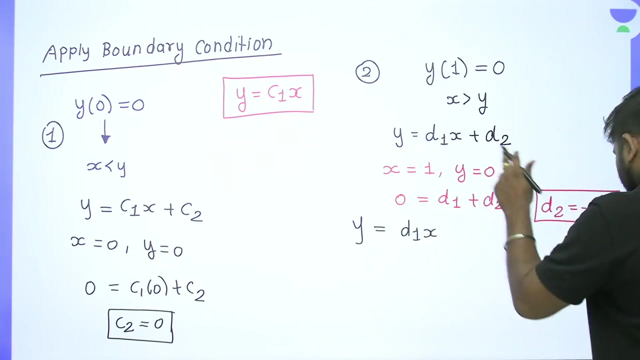 we have disappeared one unknown by using boundary condition. see, here it will not happen, right? that means now our work is easy. so if you put it in this, then the value of Y will be your D1X. substitute the value of D2, so it will be D1, now take common from here, so here your D1 will be D1 into X minus 1,. 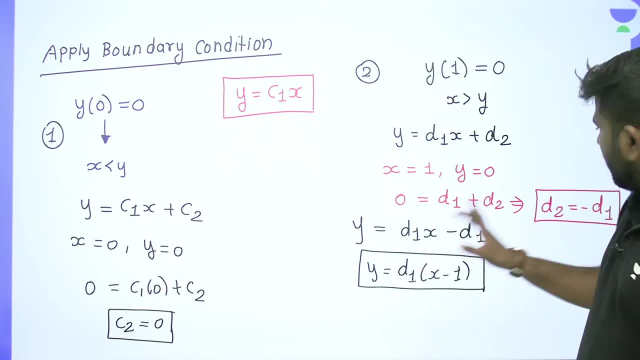 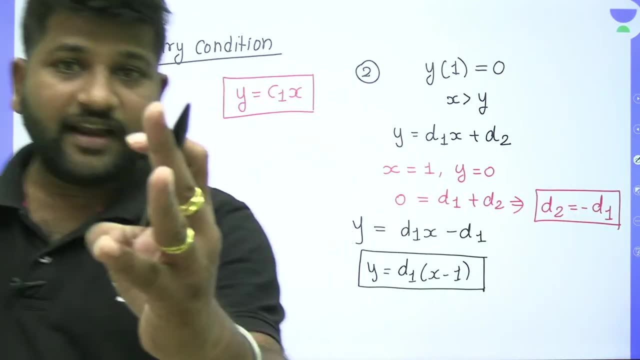 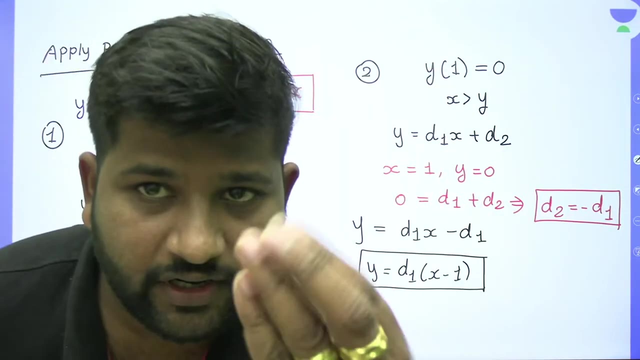 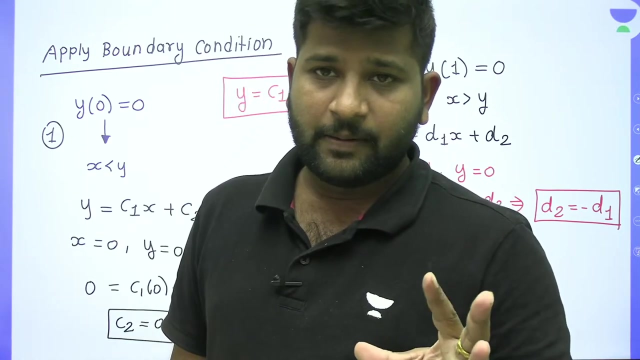 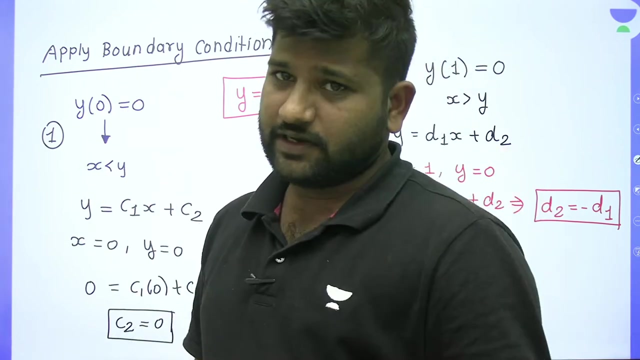 so see this, we have this. ah, two solutions. there were four unknowns in this. now, from these four unknowns, with the help of boundary condition, we have converted these four unknowns into two unknowns. with the help of boundary condition, we have done all these things. see, here, the question will come. it is very simple. there are two techniques here. I am telling you a technique that some questions are solved like this, some questions you can solve directly with options, by using the properties of the boundary condition. 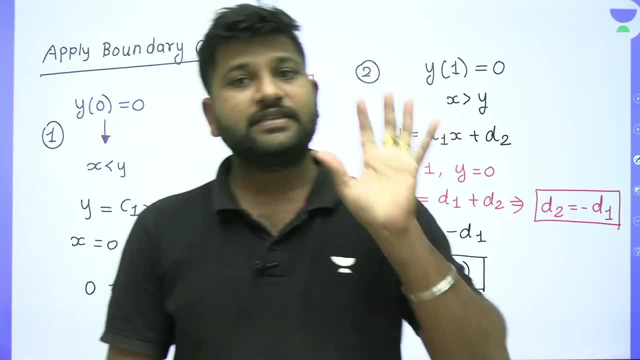 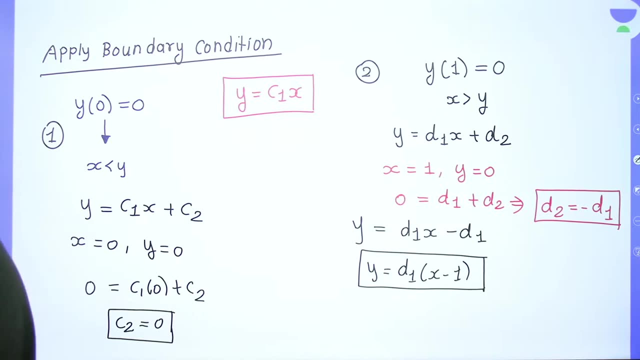 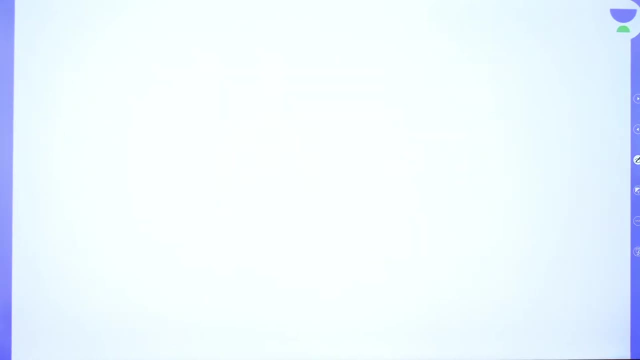 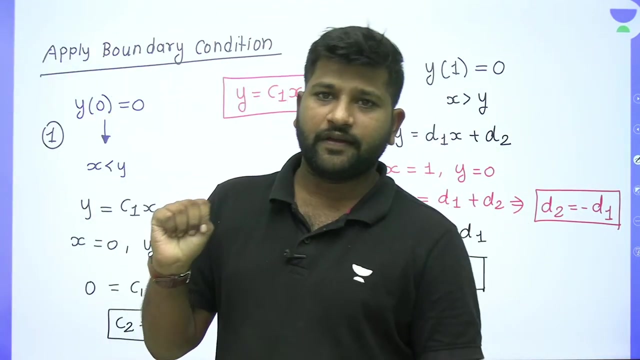 by using the properties of the boundary condition. by using the properties of the boundary condition, you will solve it, but first understand this procedure. okay, come on now. your work is done. now what you have to do, if you have this was your one step. this is a, I think, step number something third or fourth step. I think it was the fourth step. so you got this. what you have to find now? you have to find out the wrong skin. 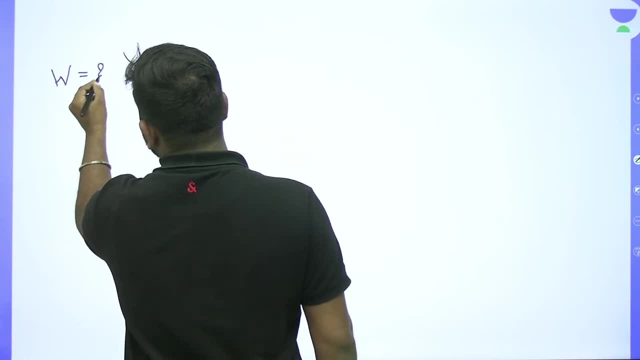 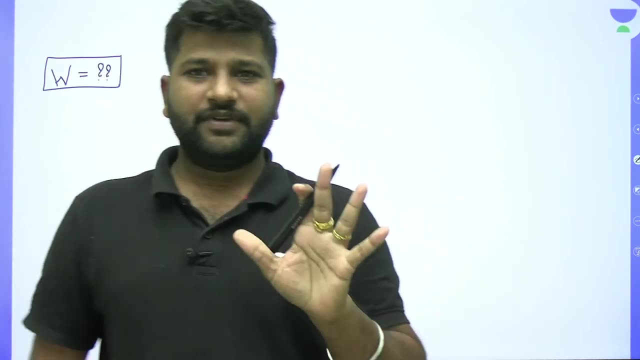 what you have to find out. what you have to find out. what you have to find out wrong skin. how to find out wrong skin. this is not a difficult task. finding out wrong skin is easy when your vector is linear, independent, dependent. there is also the role of wrong skin. 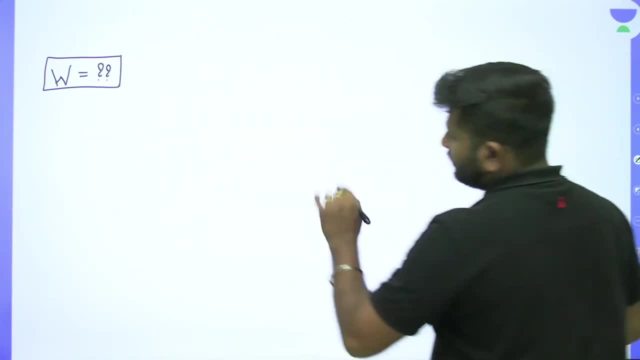 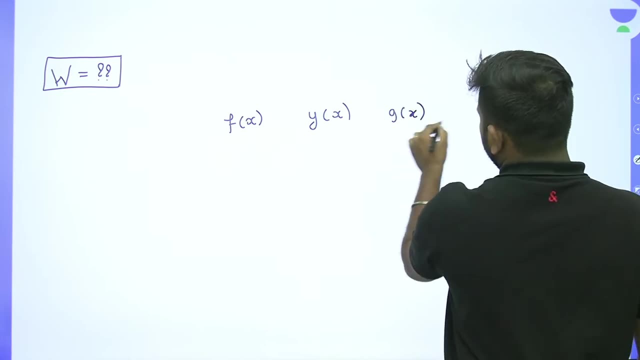 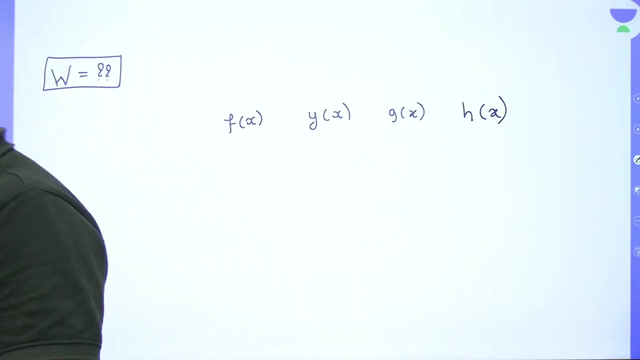 now, what does wrong skin mean? see, if you have, I give you two. one function, let us say we have this function f y g, h. Let's say you have 4 functions. if you want to find out the wrong skin of this function, 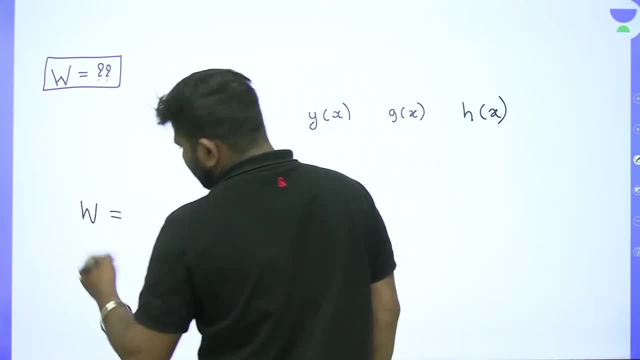 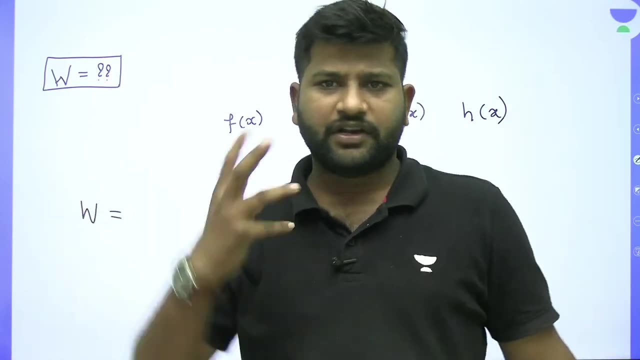 so how will you find out the wrong skin? see the definition of the wrong skin. some mathematical mathematics tells that you have to find it out like this: if this matrix is given by n, by n, matrix like this, all those things. now we will speak in a simple language, in. 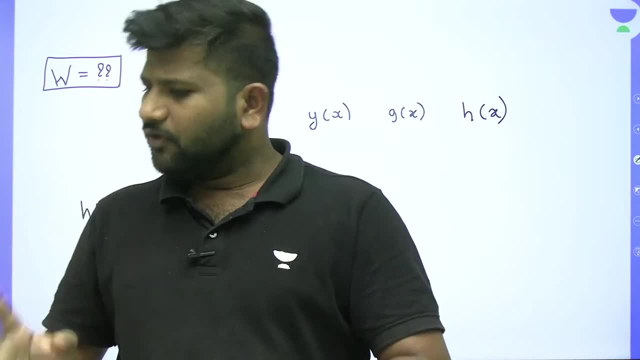 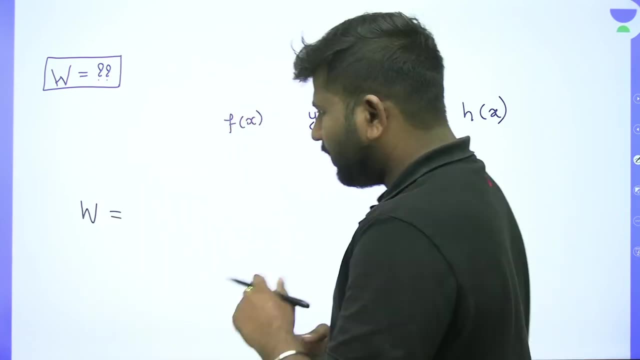 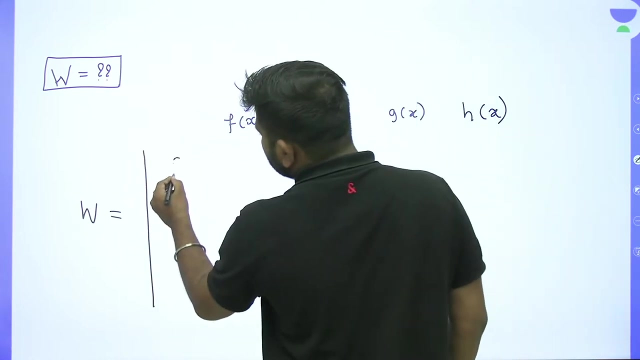 our language we will say what the meaning of wrong skin is. we will keep the language of the book a little aside, because it is important for us to understand and we do not have to write theses. so what will we say in our language? make a matrix here and write all these 4 functions here. 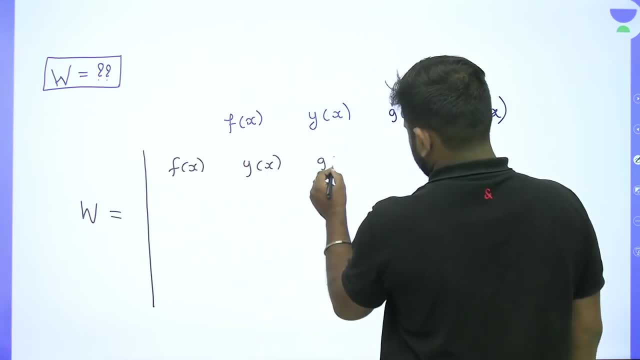 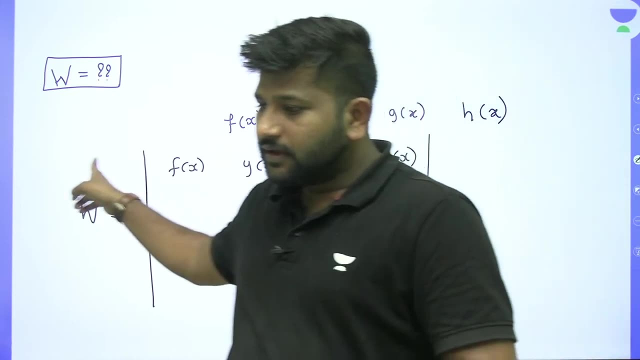 f, y, g, h. we have written this. now what to do? this is your first row. this is your first row. don't do it all by yourself. now what do you do? differentiate these. keep doing it. 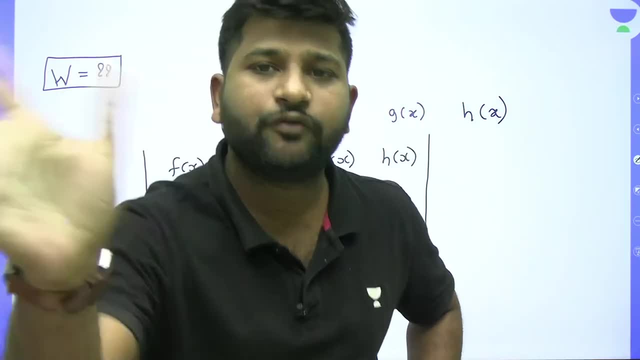 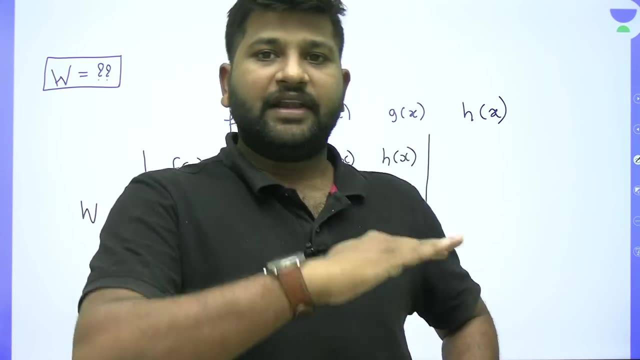 keep doing it. you have to differentiate it until the square matrix never comes. then the talk is over so much that you have to differentiate until the square matrix comes. when the square matrix comes, stop see it, that's it. you will get the wrong skin. 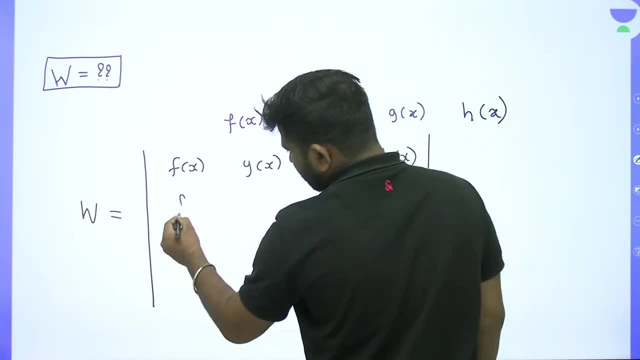 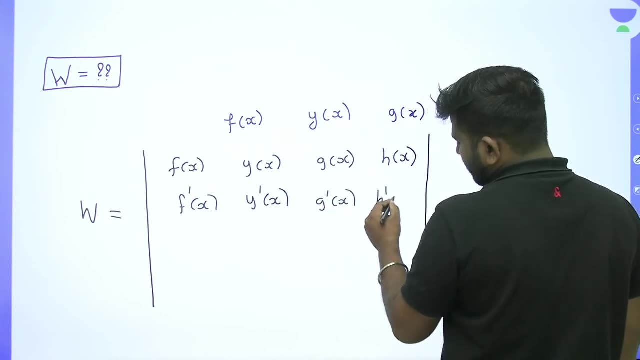 take out the detector. I mean, this is how it will be to help your f prime of x, y prime of x, g of př. x is not at all different. ofstraight grip stick, get out. b section: system De regiment. y plotting of x, derivative derivative h prime of x. is this square matrix happening? not happening? differentiate again. 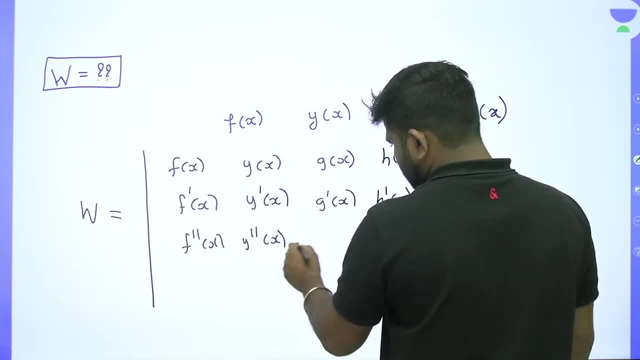 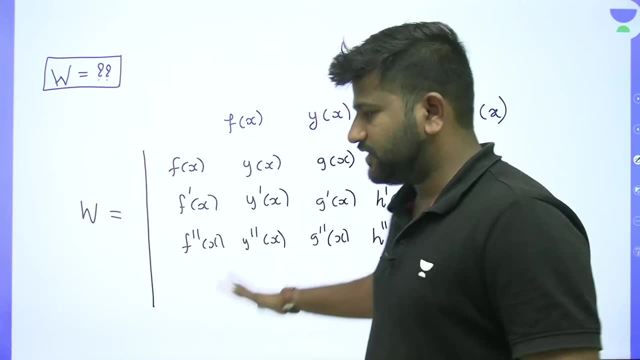 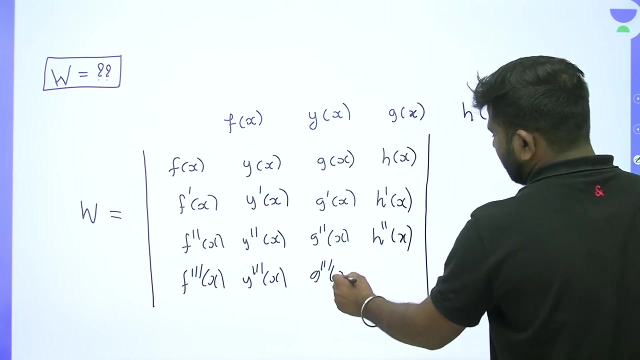 f. double prime of x, y. double prime of x, g. double prime of x, h. double prime of x. is this square matrix happening? not happening. differentiate again: f triple prime of x, y. triple prime of x, g. triple prime of x, h. triple prime of x. is this square matrix happening? stop, this is your. 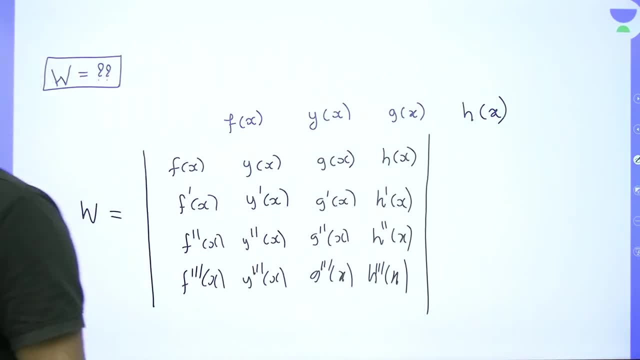 wrong skin. okay, somebody, what is the meaning of the wrong skin? so they go. it's not simple. a a me like a rocker on skinny yoga rockin. that's it as simple as that. okay, but look at our capacity up a jitnada function. a a girl. pass function of a to the topics: the path jitnada. 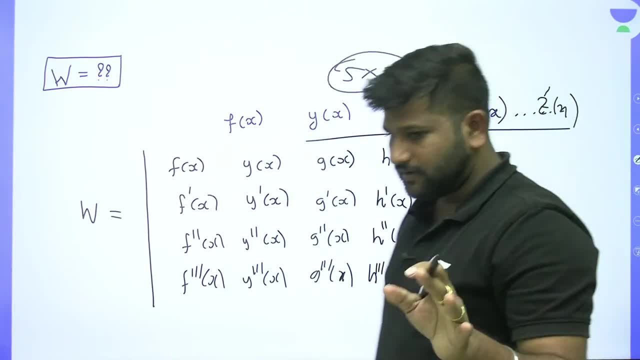 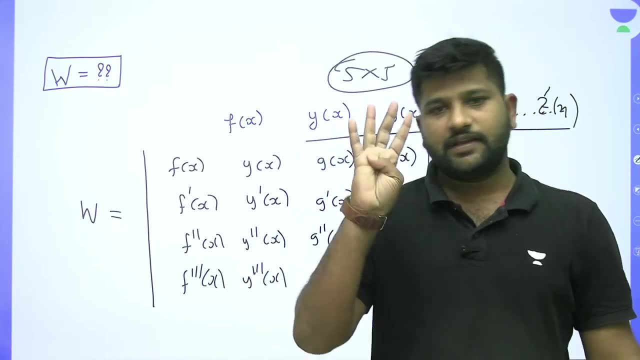 function a with a dimension cap car on piano manera simple: jitnada mission, capca function, jitnada pass. function only with a dimension car. do function at the two by two or three. function of the three by three or four. function a four by four or five, five or n or n by n, or that's it. so what is the meaning of? 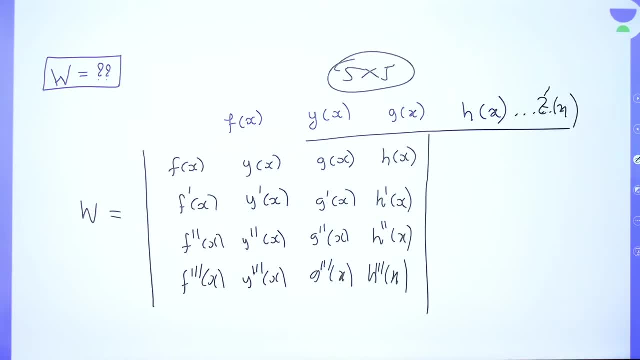 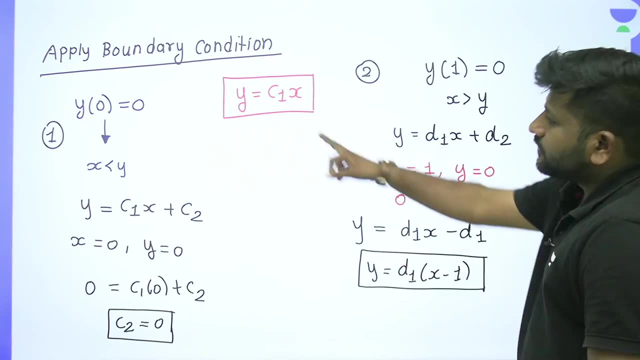 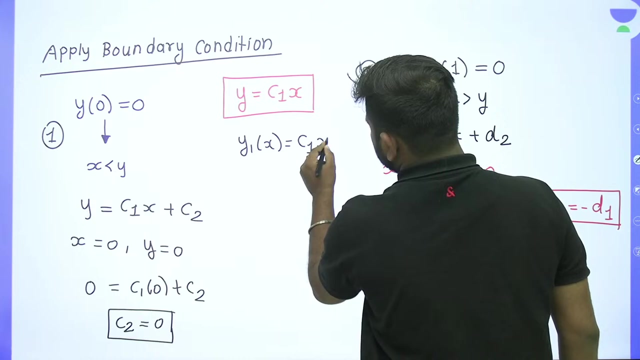 the wrong skin. so here we have to find out wrong skin. so we have two functions here. one is y1 and the other is y2. okay, so this is a y1 and y2. so I will write it like this, that this is a y1 of x. so y1 of x, how much you have c1 of x and this is: 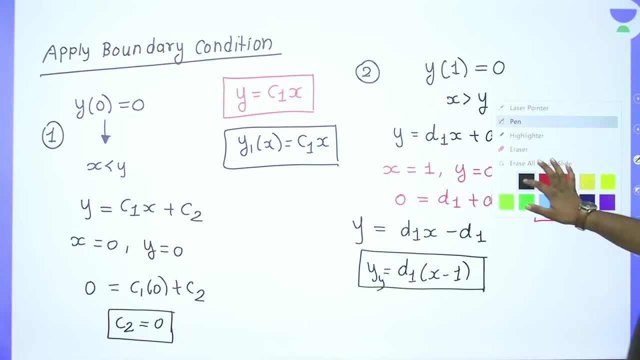 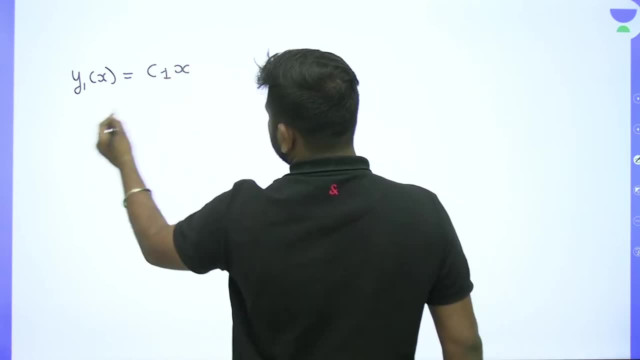 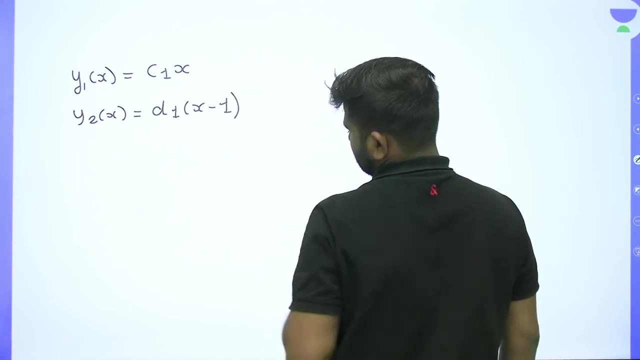 a y2 of x. I will write it on the next page how much y1 of x we have. y1 of x is a c1 of a c1 into x and y2 x is equal to your d1 into x minus 1. this is yours, so you have to. 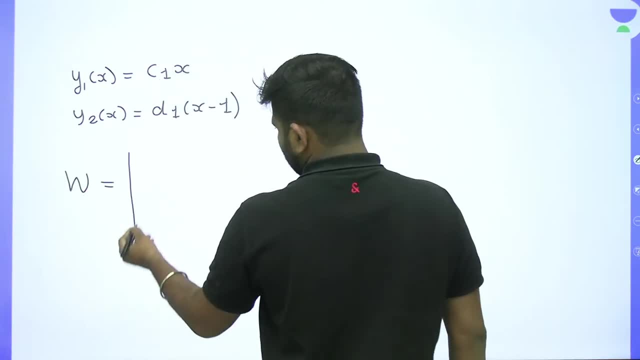 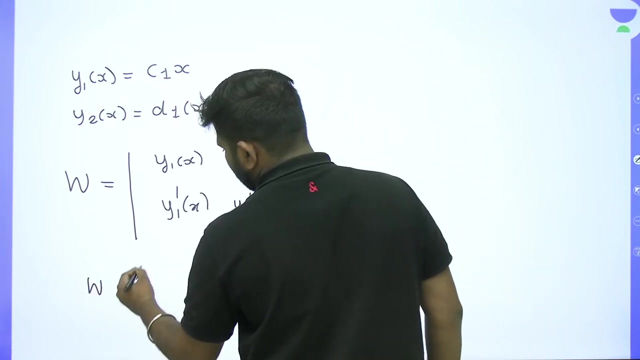 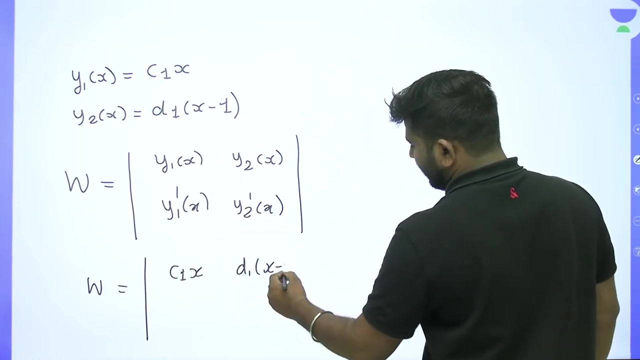 find out the wrong skin. so how many functions are there? wrong skin? there are only two functions, so there are two functions here: y1 of x, y2 of x. differentiate this: until your square matrix is not made here, just leave it, so this wrong skin will be yours. y1 of x is c1 x. y2 of x is d1 into. 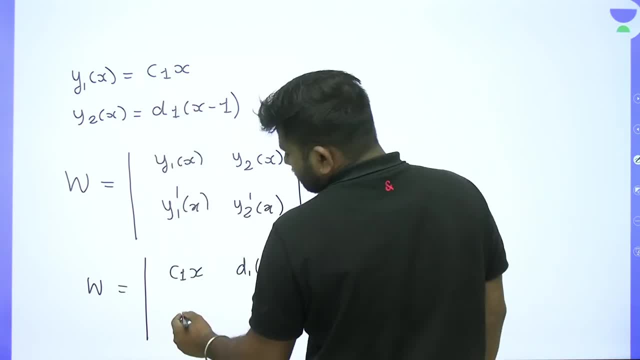 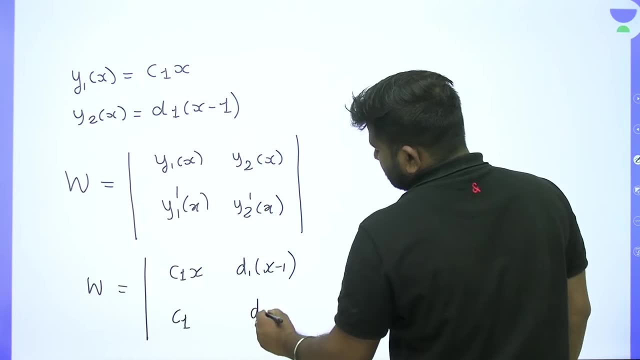 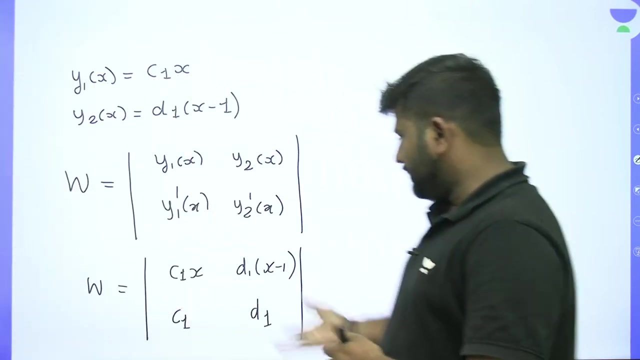 x minus 1 y1, prime of x. so differentiate this, then this differentiation will be c1 and this differentiation? do this, then its differentiation will be d1. correct, yes, this differentiation will be d1. understood, this is a wrong skin, hmm. and then we will simplify this, so it. 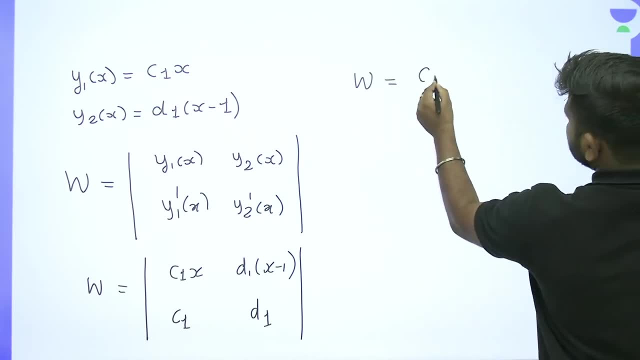 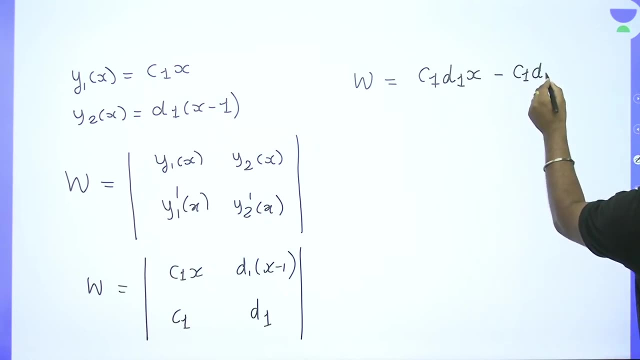 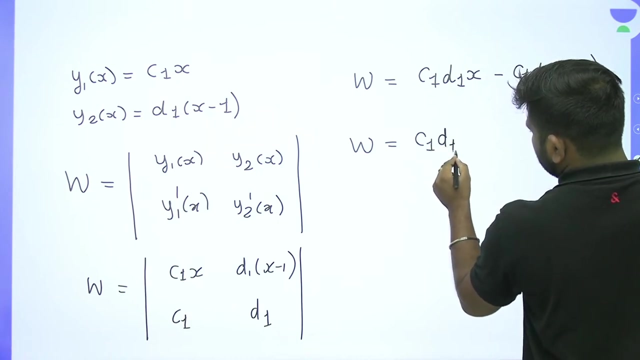 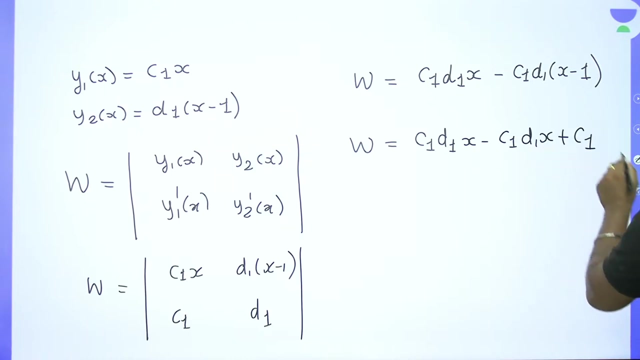 So if you simply by the wrong skin, what is your wrong skin? this is a C1 D1 X minus C1 D1 into X minus 1.. So this is equal to C1 D1 X minus C1 D1 X plus C1 D1.. 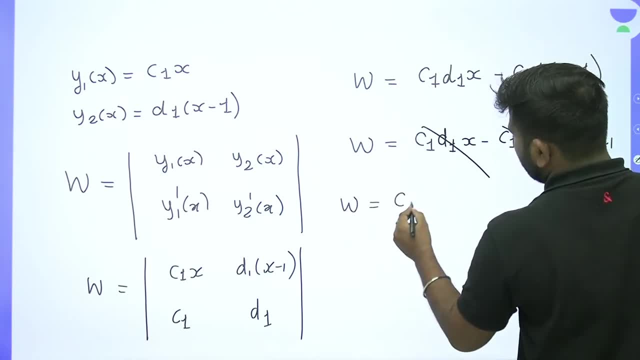 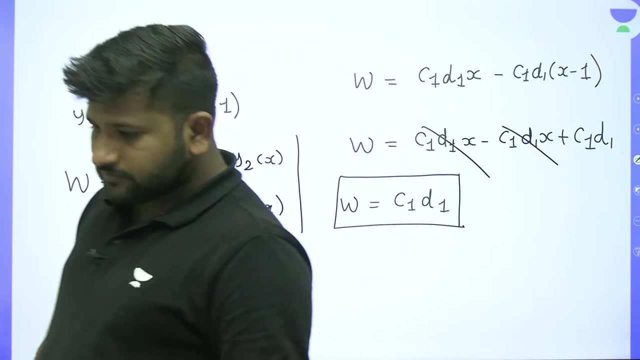 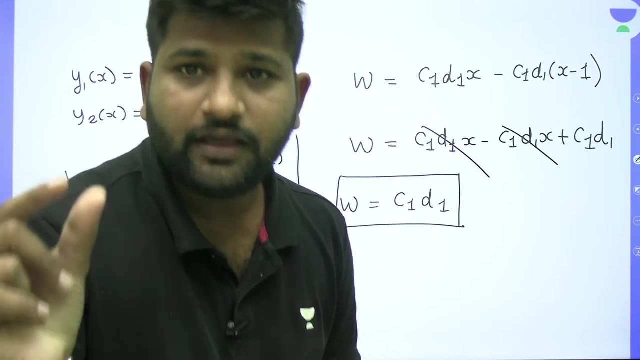 So this and this are cancelled. So what is the value of wrong skin? This is C1, D1.. What is the value of wrong skin? This is C1, D1.. Okay, And remember that if a variable comes in your wrong skin, if your wrong skin contains some variable, 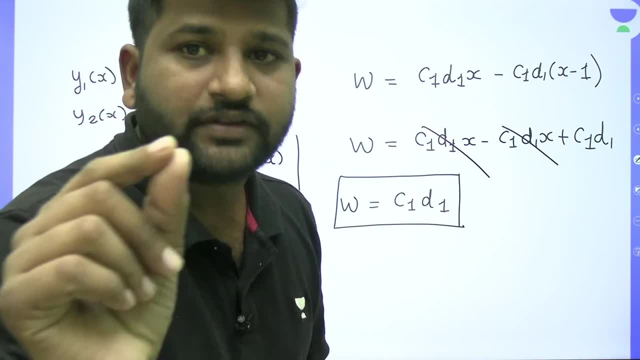 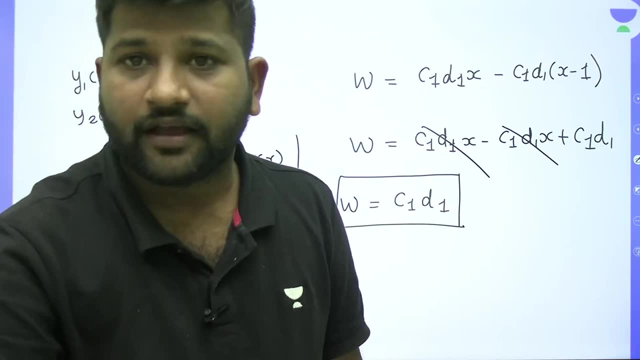 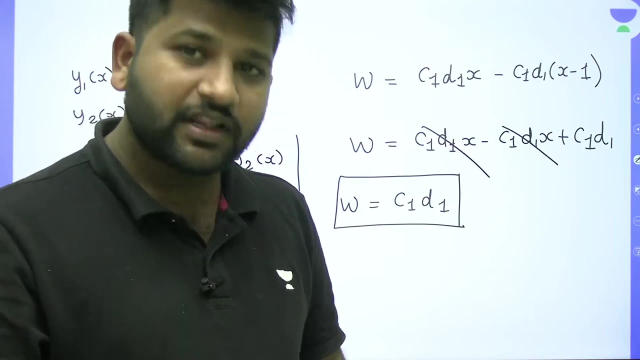 here the variable is X. if a variable comes in your wrong skin, that means somewhere you have gone, That means somewhere you have done some mistake, somewhere you have done some mistake. Wrong skin does not contain any variable. You do not get any variable in the wrong skin, it gets cancelled automatically. 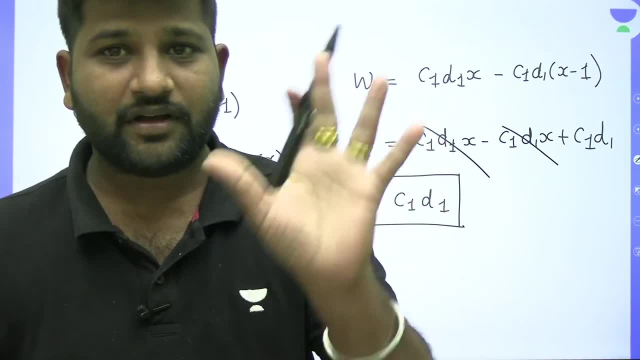 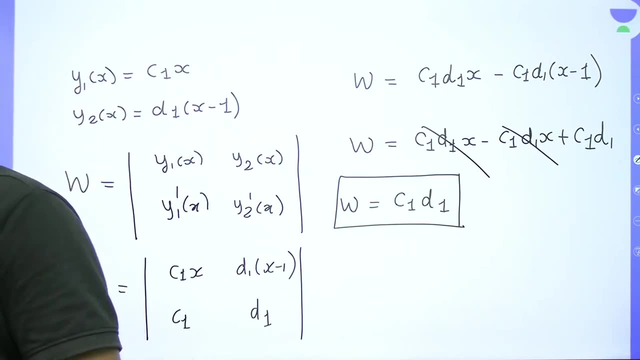 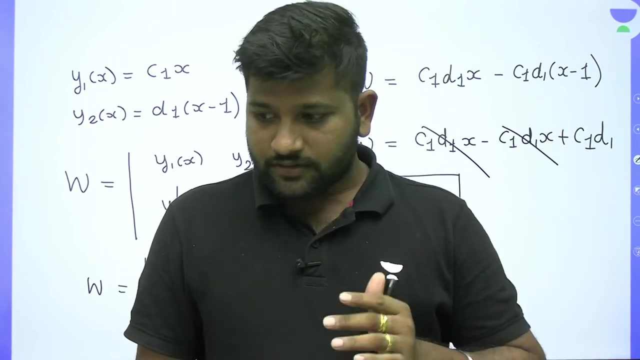 And if a variable is coming in your wrong skin, that means you have done some mistake somewhere. please re-check it. Okay, Is this clear to everyone? If your wrong skin contains any variable, that means you have gone somewhere. Okay, You will not get any variable in the wrong skin. 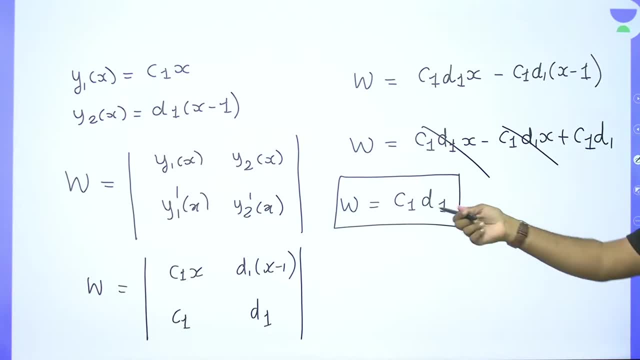 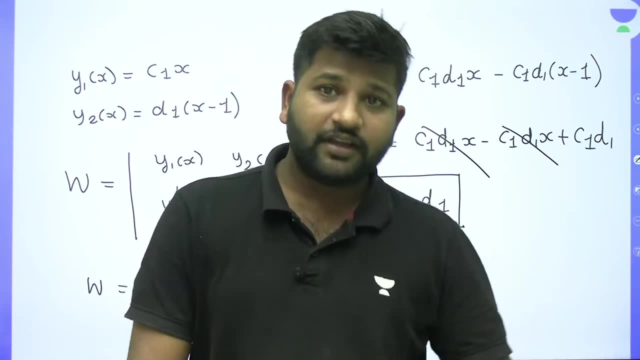 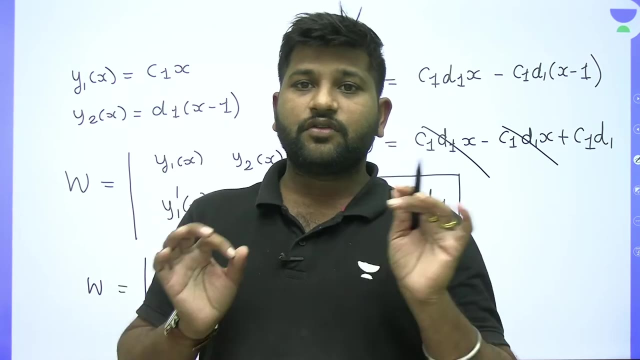 See here, Here, in the wrong skin, AXX will be cancelled, C1, D1 is directly. you will get a pure, constant Wrong skin. there will be no variable in the wrong skin. You write it down in pure Hindi That in the wrong skin, when we find out the wrong skin, there should be no variable in the wrong skin. 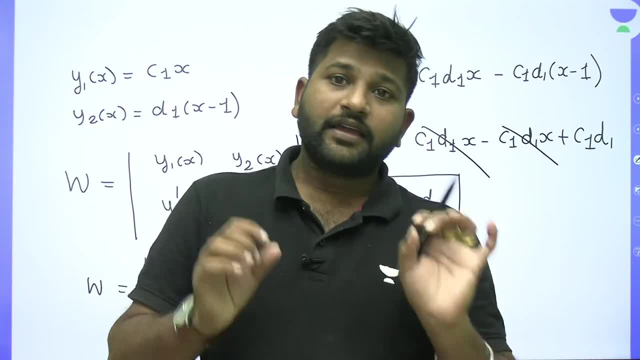 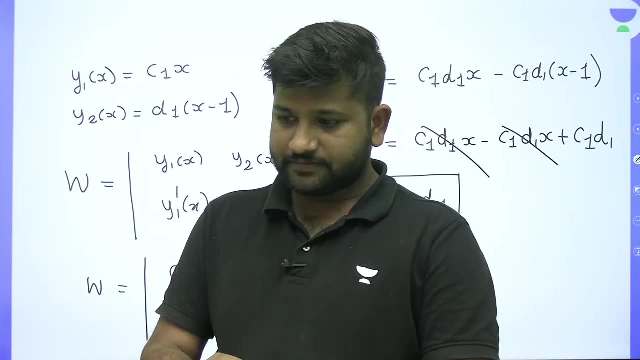 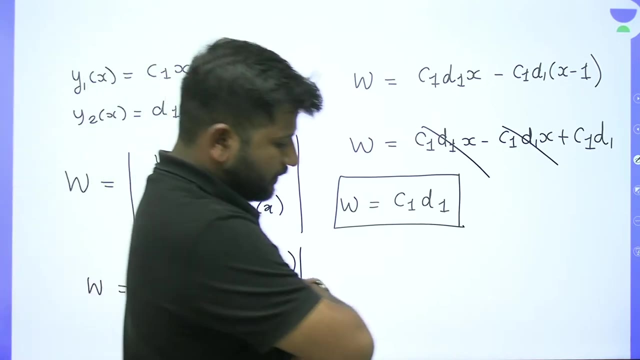 And if there is any variable, that means this means that we have done some mistake somewhere. This mistake is definitely we have done Understand, Okay, Now this is done. now this is also our step, but what is the last step? what is the last step of you? 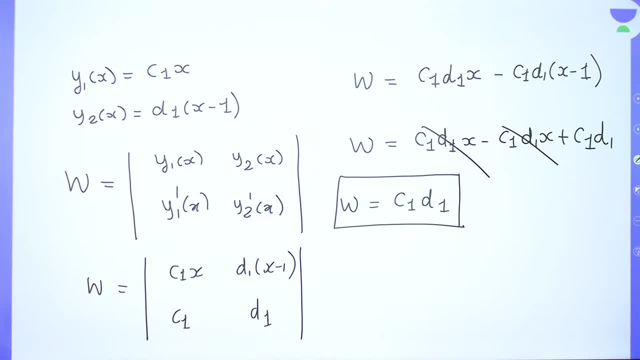 Okay, What is the last step? The last step is to find out the solution. Find out the Green's function. Now, find out the Green's function. that is the last step. We have already got all the things. Okay, Okay. 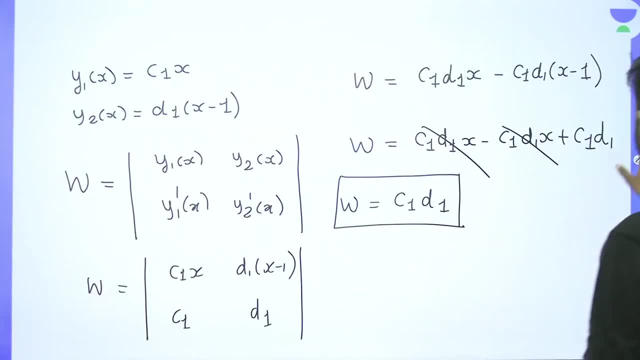 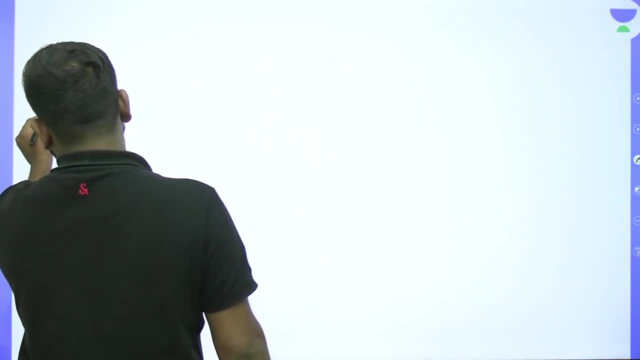 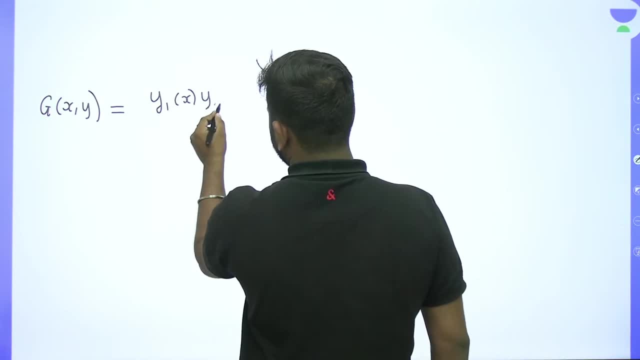 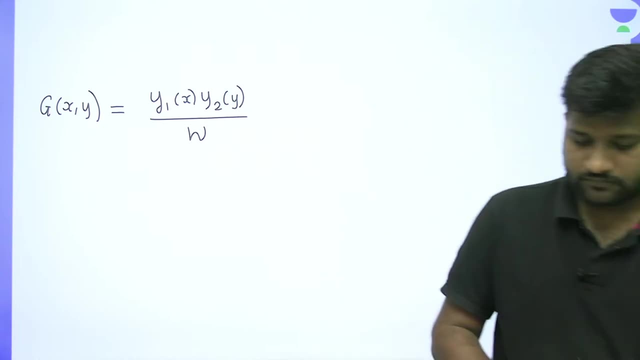 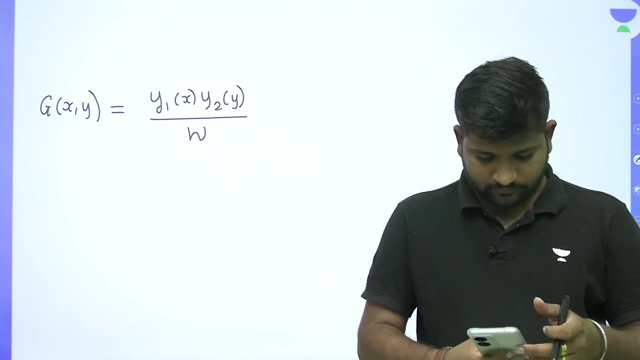 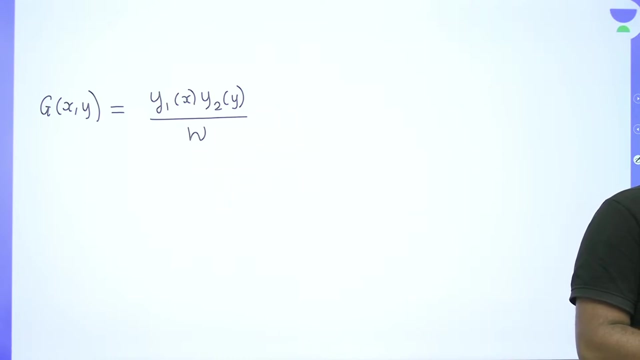 that this would be First x, Second y, divided by the wrong skin: hy y 1. Wait a minute, I am getting a call. Okay, Hey, everyone hit the like button. hit the like button. they are just watching. hit. 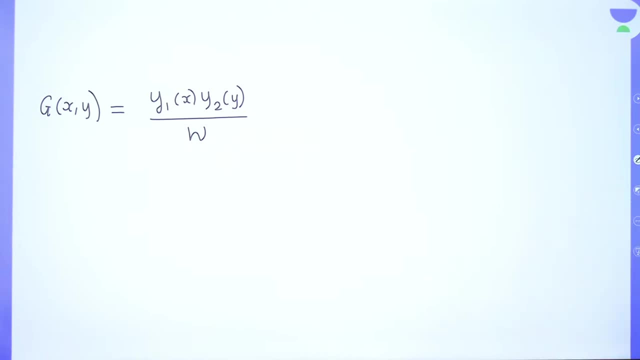 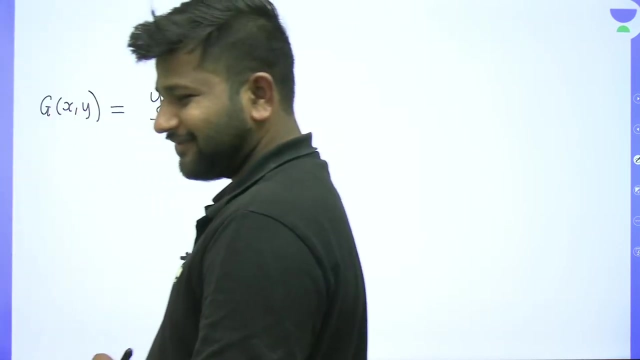 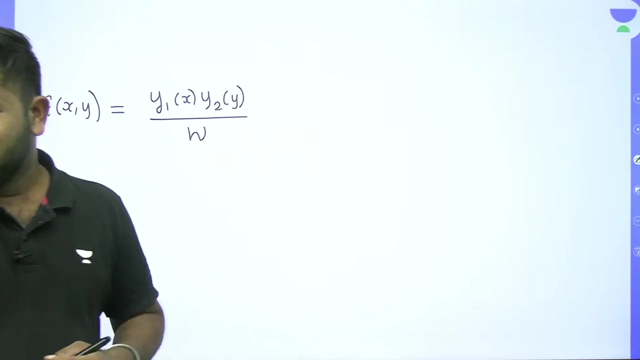 the like button. The likes should be as much as the likes. they are just looking. just hit the like button. everyone who did not do You will be thinking that what is this force, isn't it? I mean, we are watching quietly and we are in the middle. hit the like button. 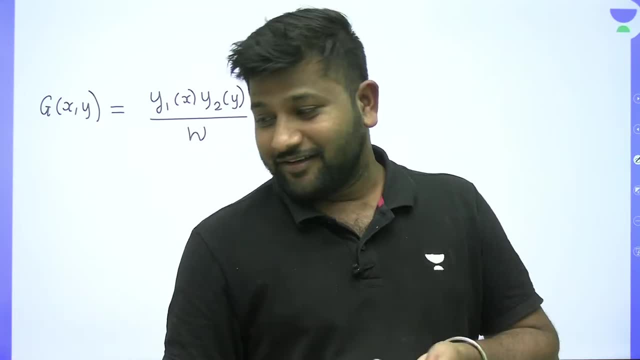 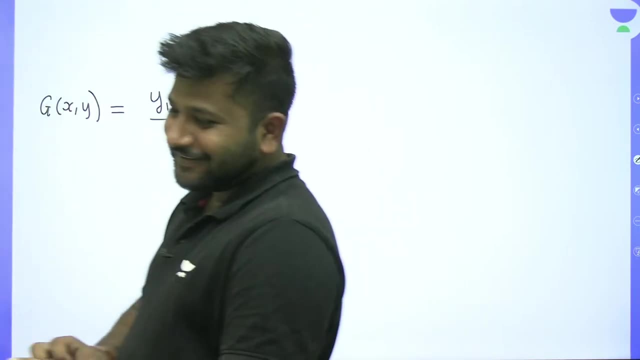 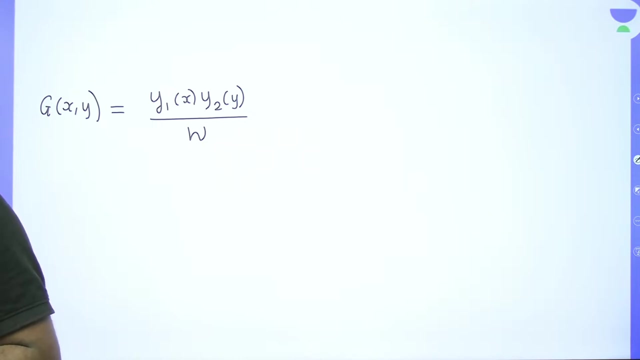 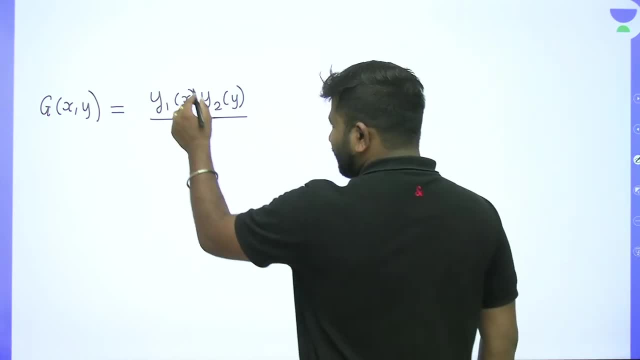 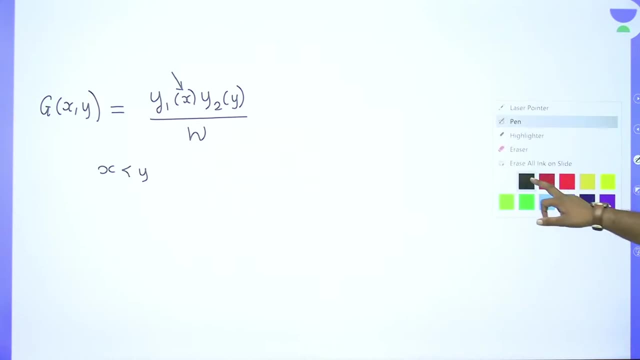 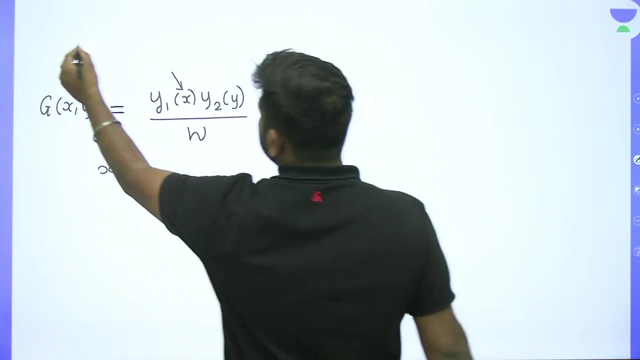 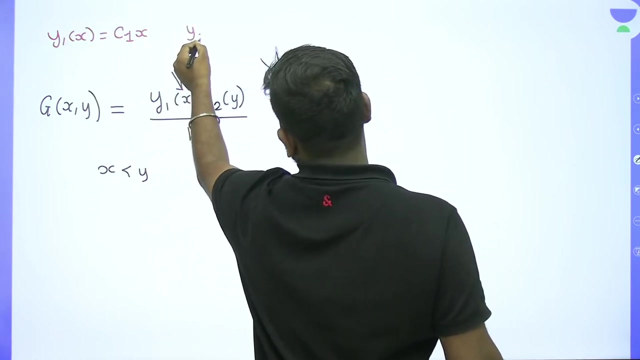 Green's function. so what I have told you here is that this will be small inside. that means this is a solution for x less than y. okay, so what is the y1,? so I write here that what we had- y1 of x, y1 of x is our c1x and y2 of x is our d1 into x minus 1, okay. 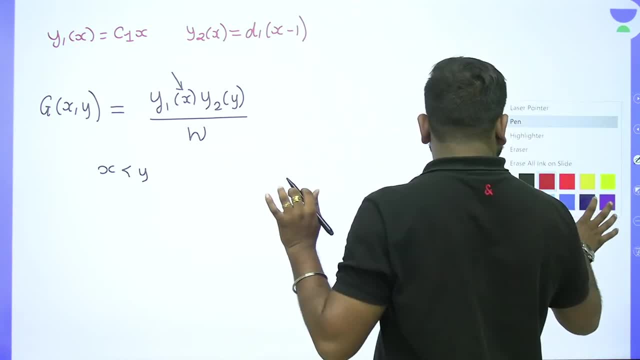 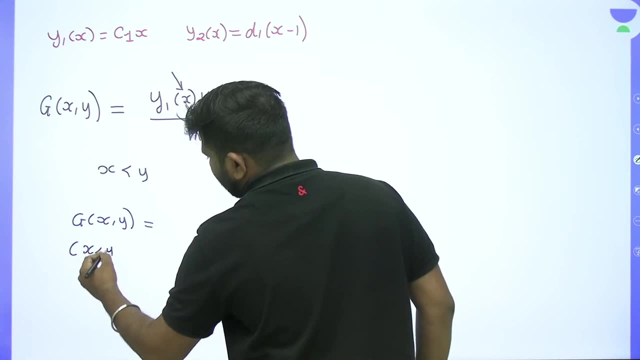 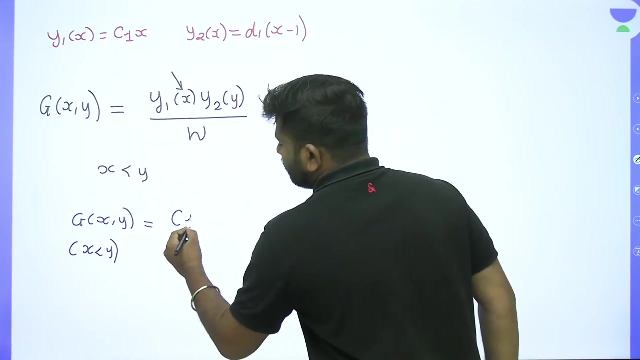 so this is the Green's function. so this Green's function will be ready here. okay, that Green's function. xy is equal to what will be for x less than y. see, this will be y1 of x. that means, put x in y1, put x in y1, that means this will be c1x. okay, and then. 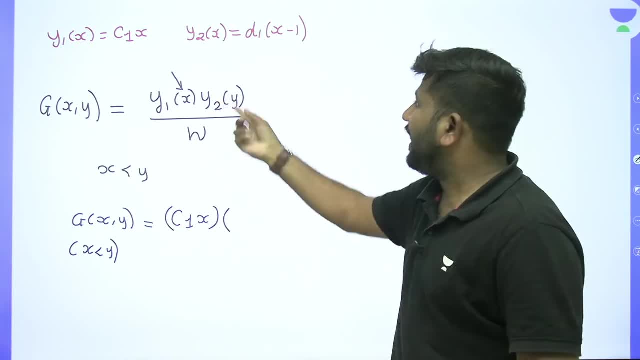 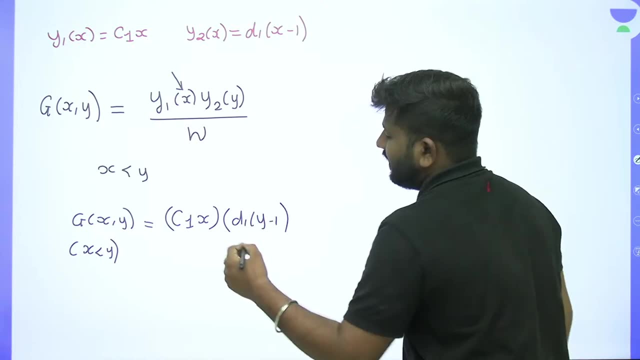 here y2 of y. pay attention, y2 of y, that means y2, put y in that instead of x. so this will be d1, y minus 1, understood and divided by Ronskin, what is your c1, d1, see, this is. 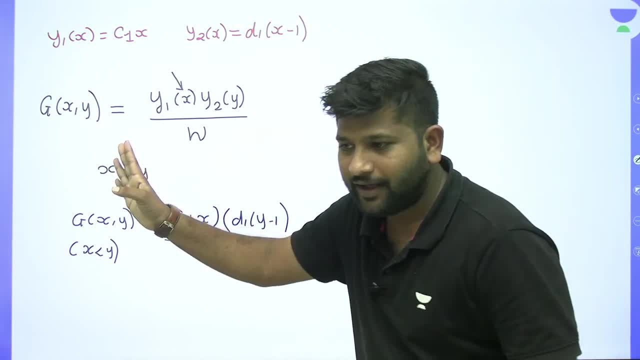 that green's function y2 of x is pretty 12, that is why this green function say: then your bottom is going to be c1d0,, that is going to be c1x. but the next one is here again, it is getting st 형ed. почему? because the ceno. this guy took the ceno here. 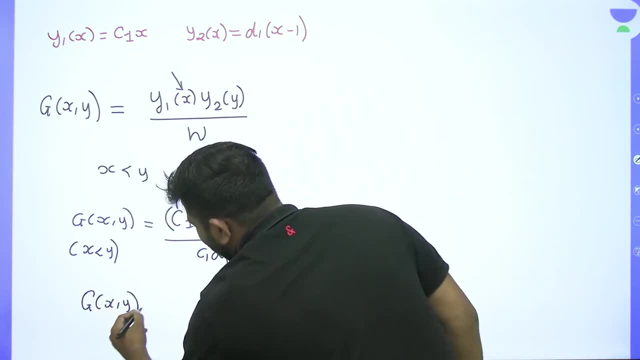 Now you are always saying that again, the exact same thing bought all the time, but it doesn't look that way that bg into g minus one plus b is solving. what we are saying here is that the gfx x is going to be produced by celebrating, because, if it is, 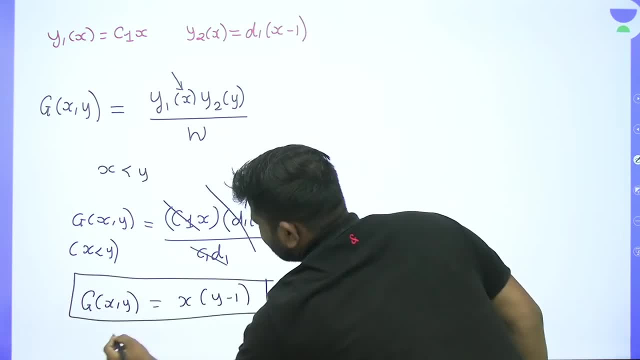 mix with x. once again. that is because if it is mix with xm, so it is for x times, because if we get the useful rule, it is going to be disappear. then we get x. Now come to this situation, that is, we are talking about **** refugees, so let's give. 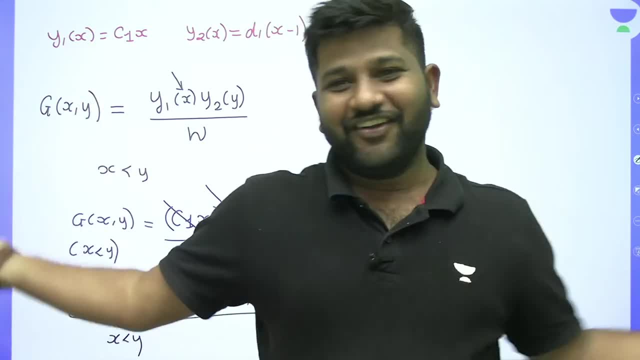 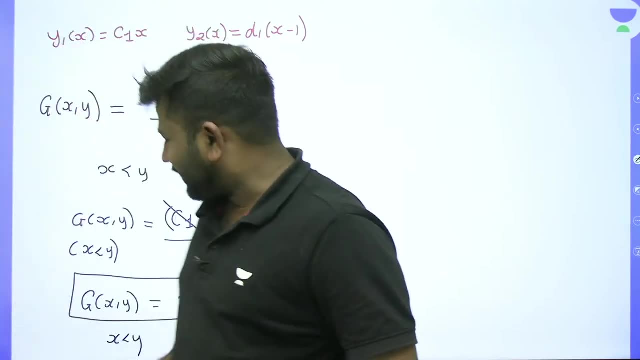 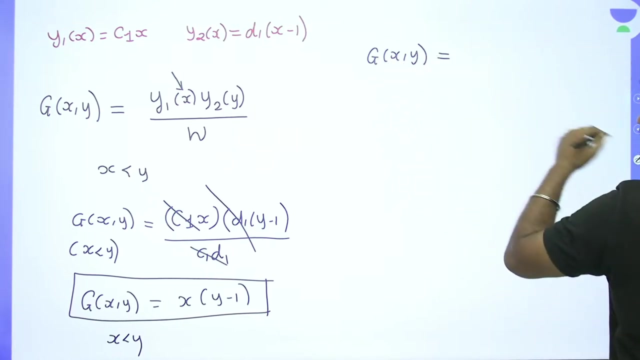 Not that much difficult. the answer is done. that is the Green's function. so your Green's function will be this. that is for this. But if we want for the second region, then g of x- y, then how much will be this g of x- y? 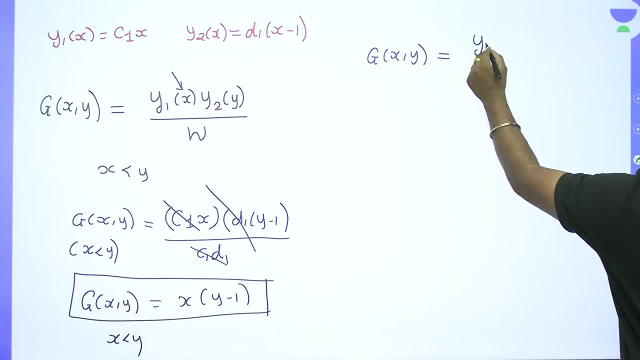 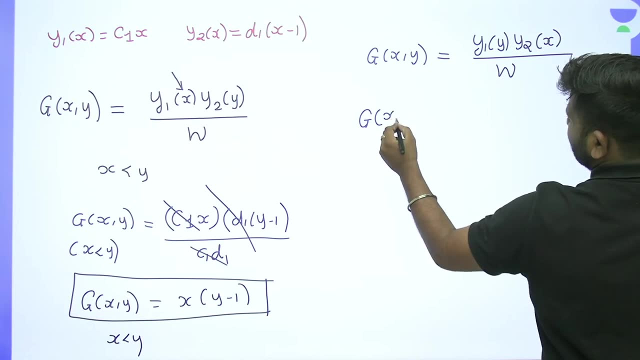 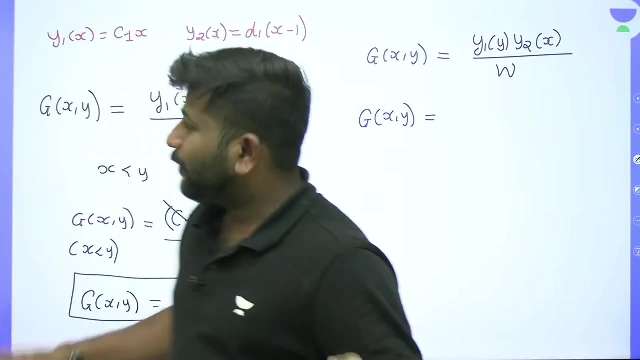 g of x, y will be this: y1 of y, y2 of x, divided by wrong skin. so g of x, y is equal to how much will be this y1 of y? now, what are you saying? y1 of y, y1 of y means y1 is this: and when y is added to x, this will be c1y. 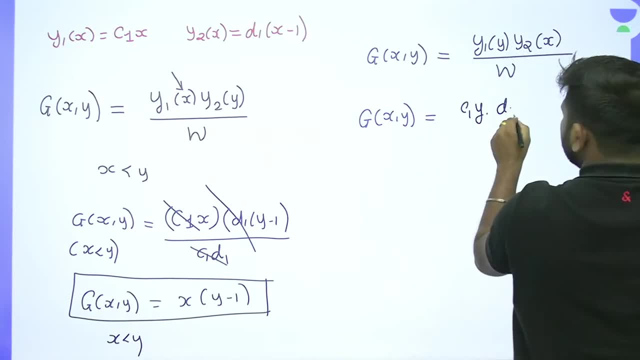 y2 of x. y2 of x means d1, this will be your x-1,. that's it done. So that's it done. So g of x. y is equal to: oh no, w. w is nothing but the wrong skin. 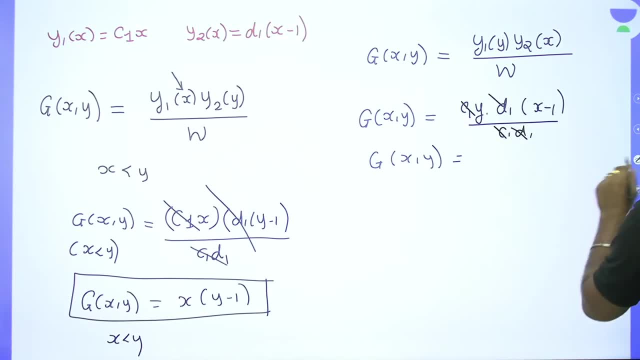 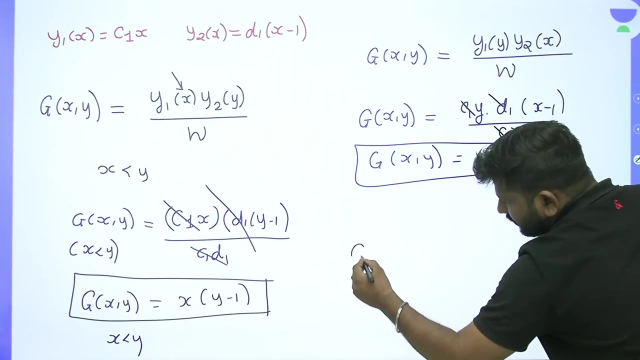 What is wrong skin? You have c1d1, c1d1, And this will be cancelled, so you will have x-1,. who said that the Green's function is difficult? That's it very simple. Okay, that means now I will write that this Green's function, this Green's function, is your. this is equal to this. 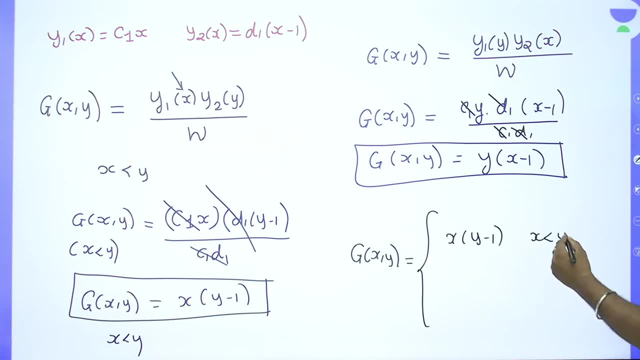 It will be x into y, y minus 1 for x less than y, and this is a y into x, minus 1 for x greater than y. that's it. just follow these steps. this is your solution. just follow the steps. ok, I hope you have understood. 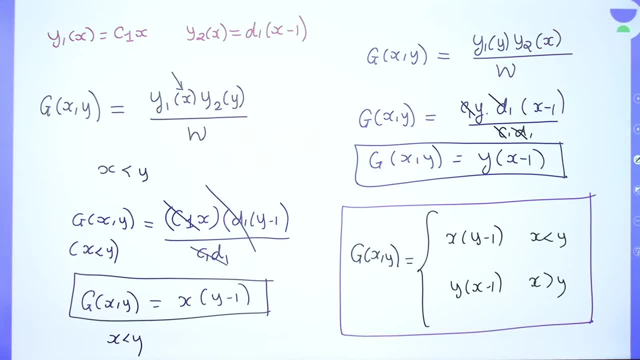 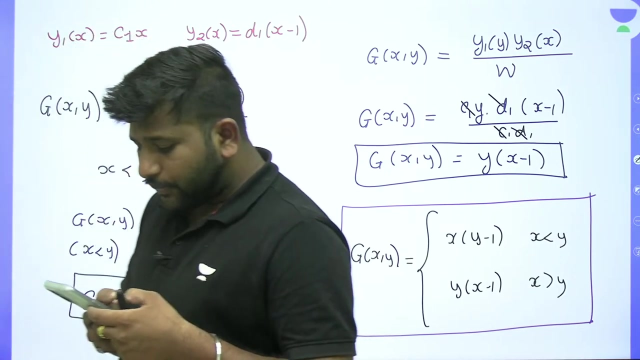 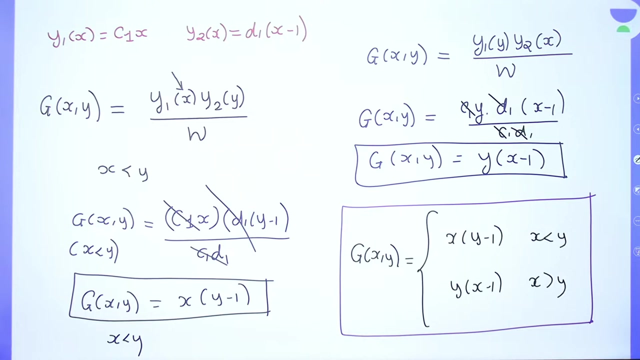 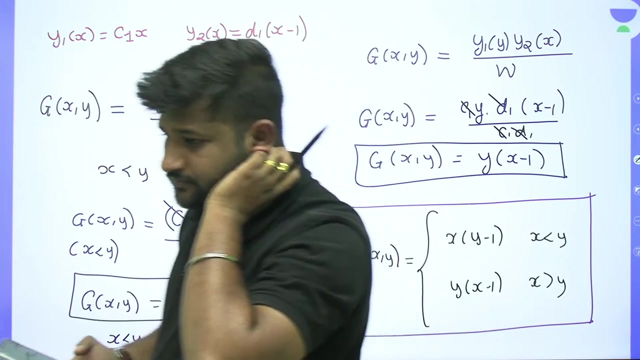 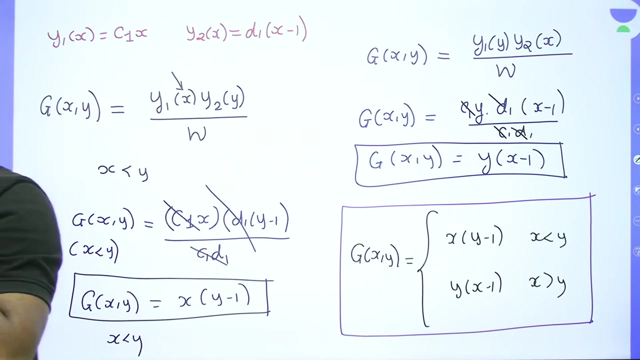 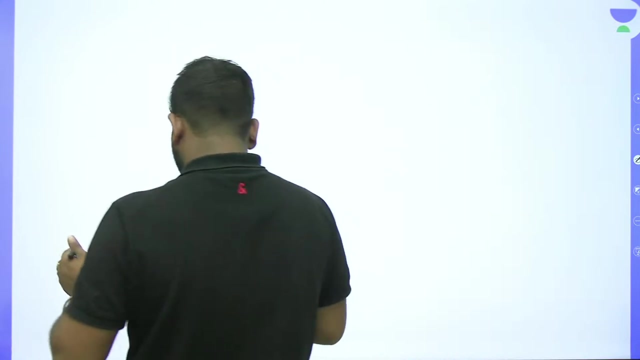 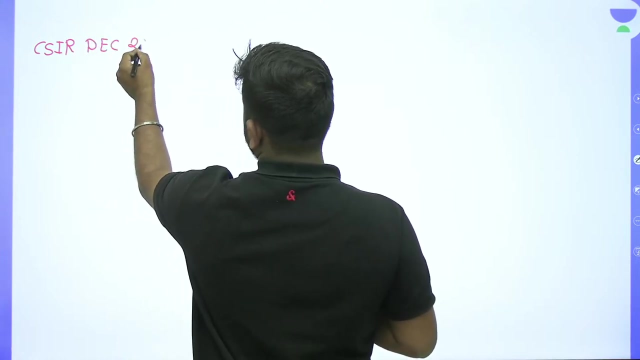 if there is any doubt or difficulty, you can ask. otherwise, let's move forward, ok, ok. ok, is this clear to everyone? ok, next, so we'll discuss the question. okay, is this clear to everyone? so let's go ahead. so let's discuss the question. this question is from CSIR, December 2018. 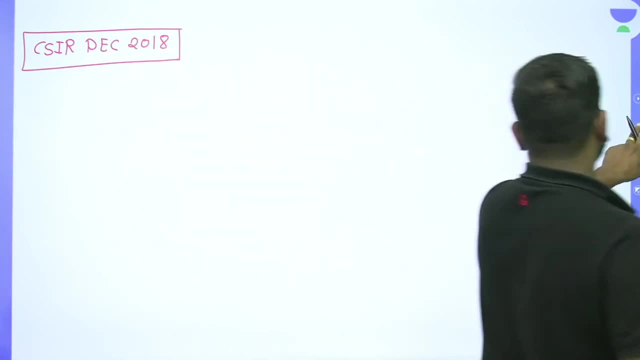 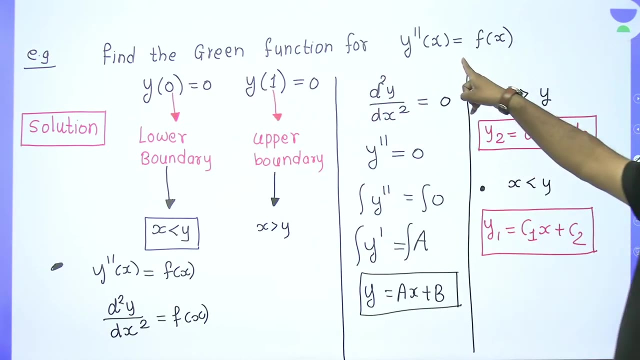 let me tell you once again how to do it. see here: this is your you. this differential equation is given to you. this boundary condition is given to you. put 0 on this side after putting 0, take out its solution. so write this solution for x greater than y and x less than y. 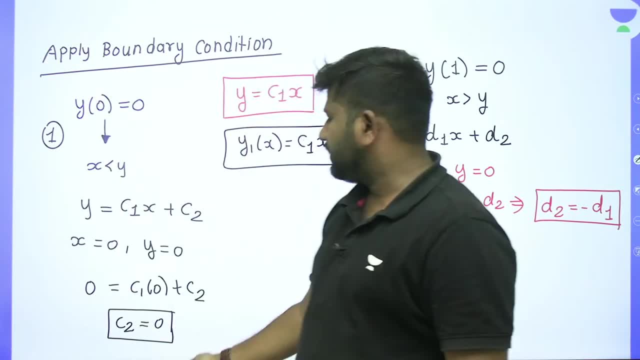 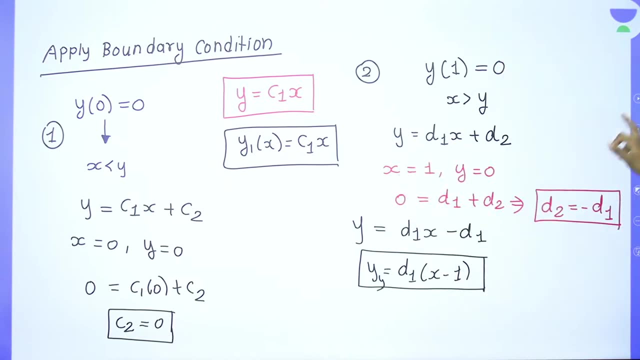 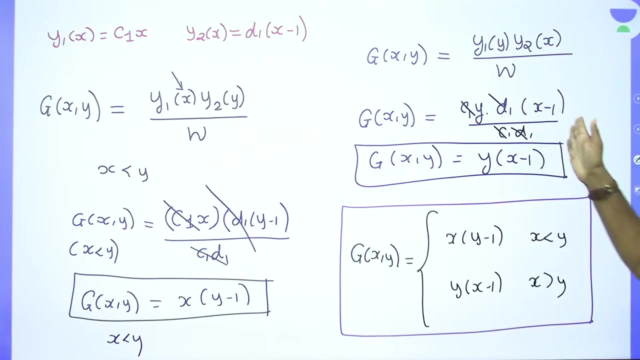 then apply the boundary condition here after applying the boundary condition when your 4 variable is connoted in 2 variable. so from here we will get y1 and y2. find out the wrong skin from this. after finding out the wrong skin. yes, this implies that we can habitually say that. 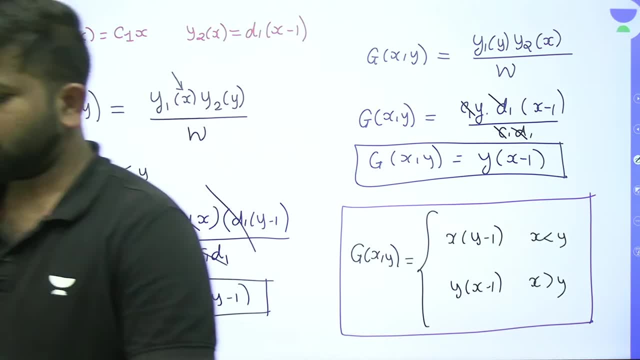 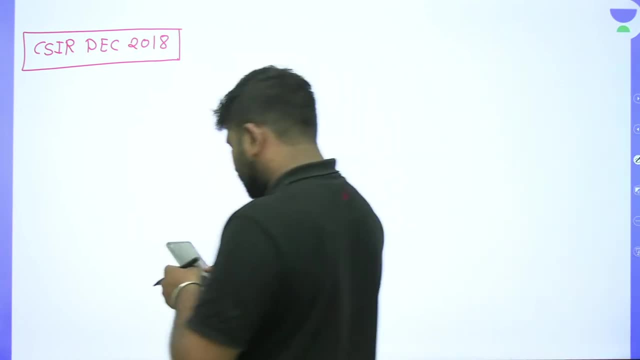 z is just 1 from z, z is just 1 from y, z is just 1 from z. what is this? but what is the boundary condition? there's two parts, so by doing right once, leave z is just 1 pot. now we should write z, is is equal to 1. 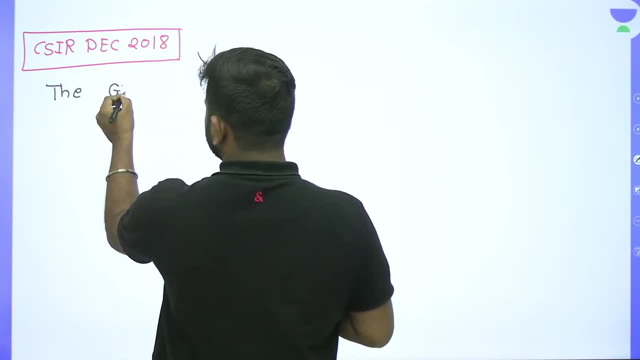 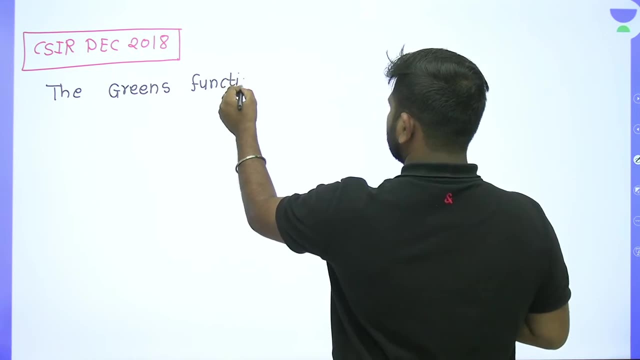 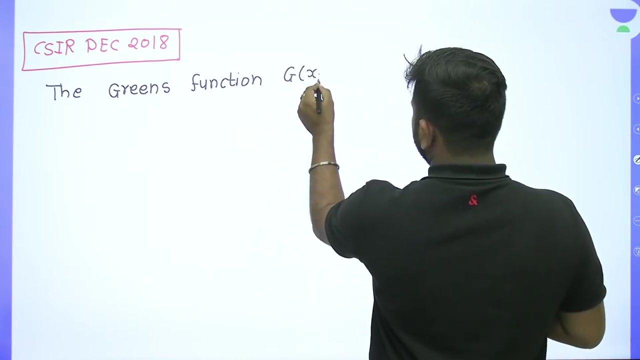 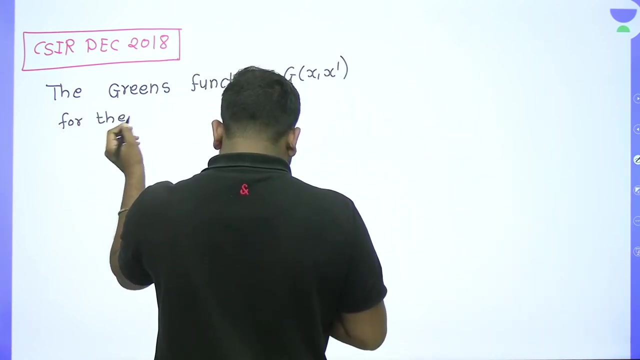 and we will be learnt all other games when we will learn like this. so how come j is equal to 1 and y is equal to 1, so 3 times z is equal to zero, will achieve 10% agreement. Green's function: g of x x prime. g x x prime for the. for the equation for the: 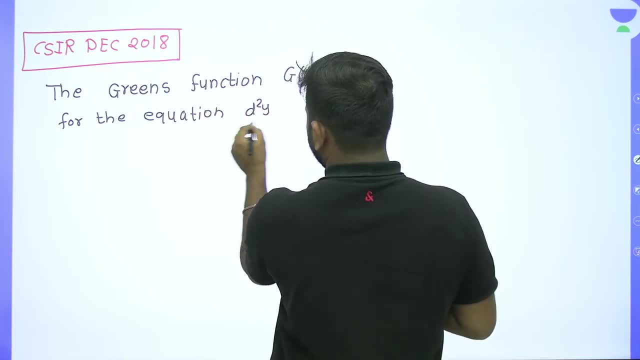 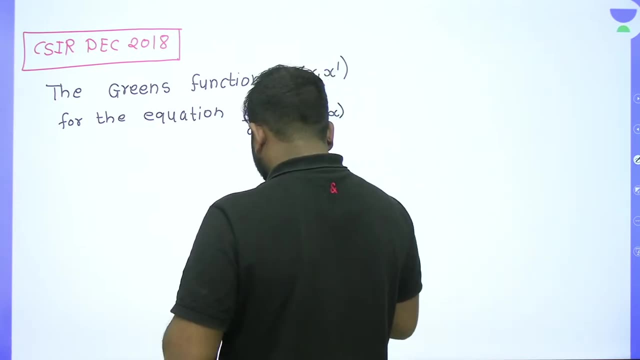 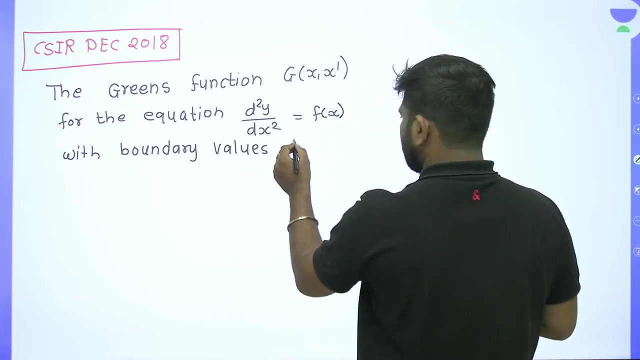 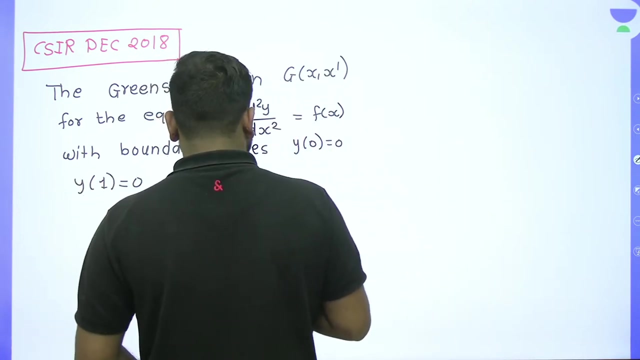 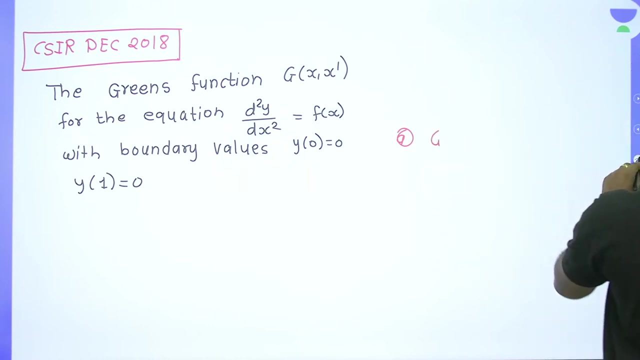 equation: d square y by d x square. d square y by d x square is equal to f of x is equal to f of x with, with boundary values. with boundary values. with boundary values, y of 0 is equal to 0 and y of 1 is equal to 0. okay, so this was given to you, and your options. they are: 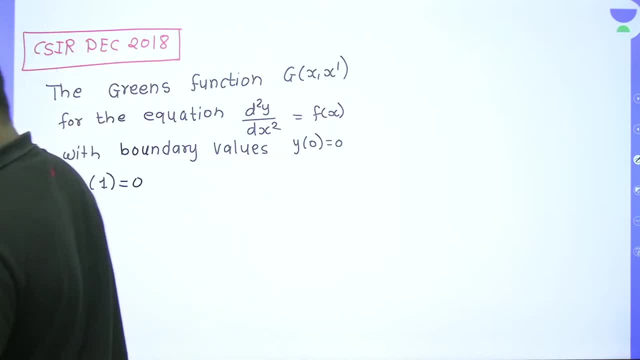 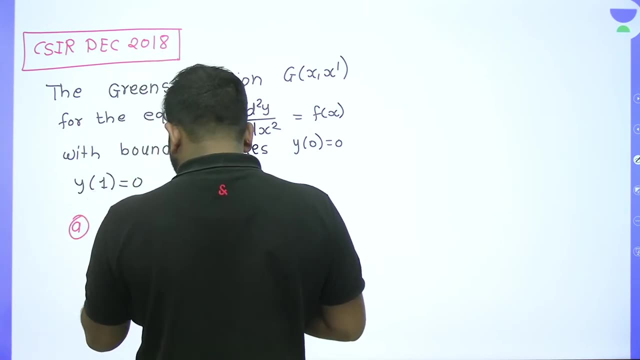 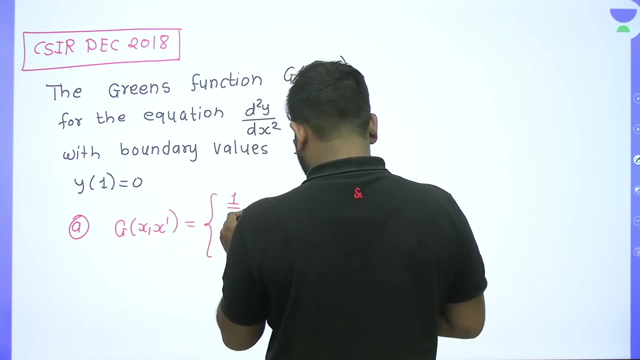 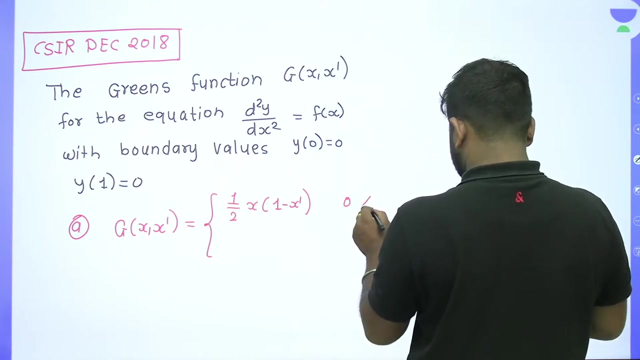 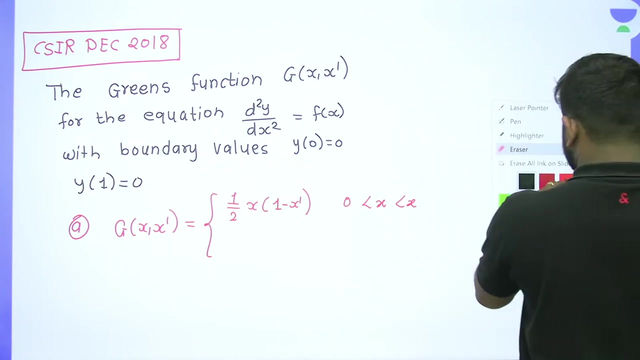 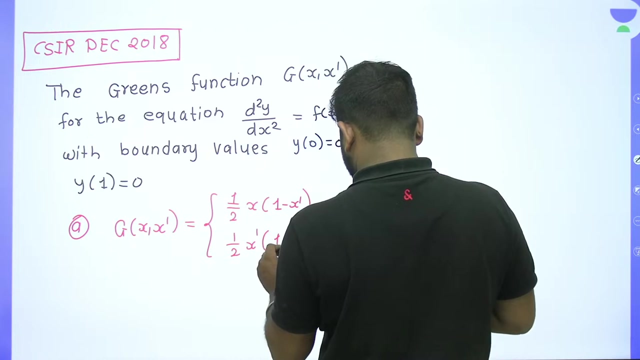 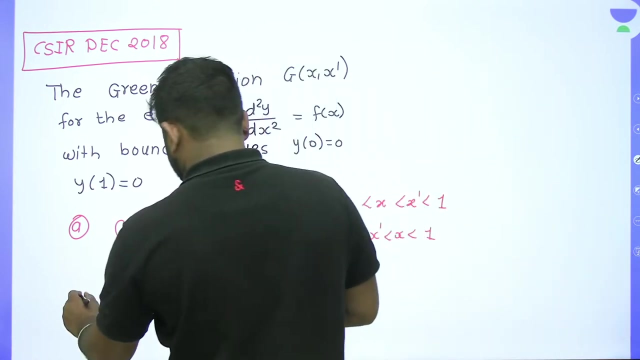 given to you. option a g, x x prime is equal to, you will have. this is a 1 by 2 x into 1 minus x prime. this is for 0 x prime 1. this is one by two x prime. 1 minus x zero x prime x: 1. option b g of x x prime is equal. 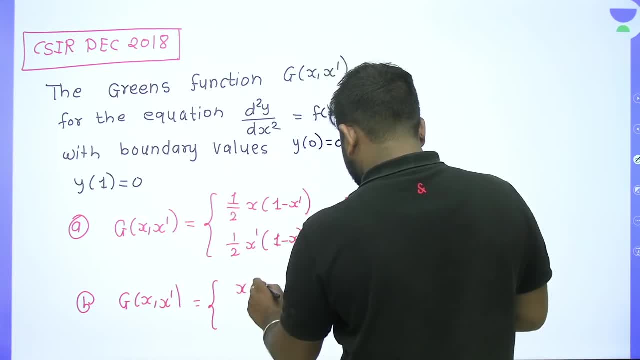 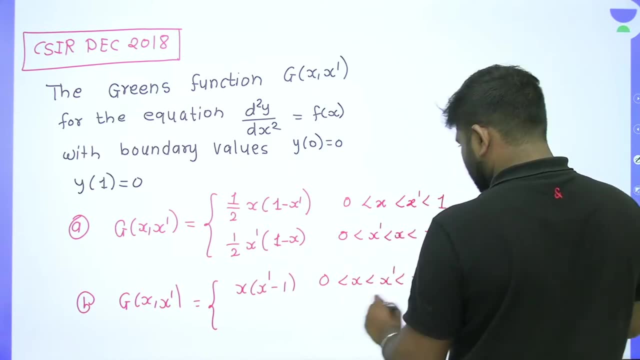 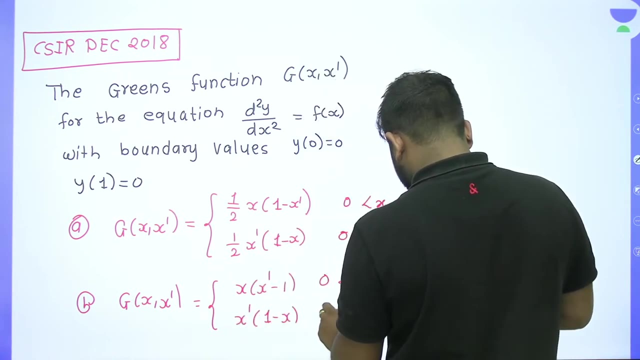 to you have given. this is a x into x prime minus 1, this is for zero x x prime one x 1 x prime 1 and this is for x prime into 1 minus x. so you got 0 x prime x 1, so this was your option. 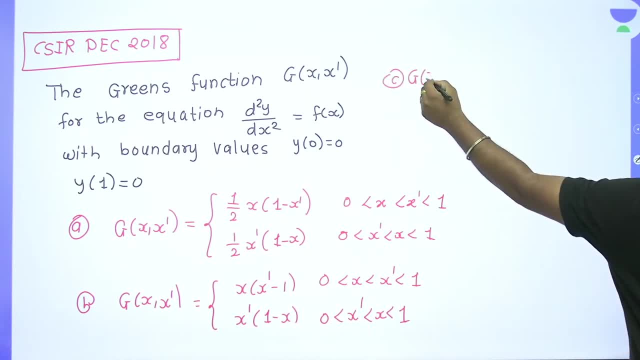 option c, given g x x prime is equal to minus one half into x into 1 minus x prime. this is your 0 x x prime. 1. this is a one half x prime into 1 minus x. this is for 0 x x prime. 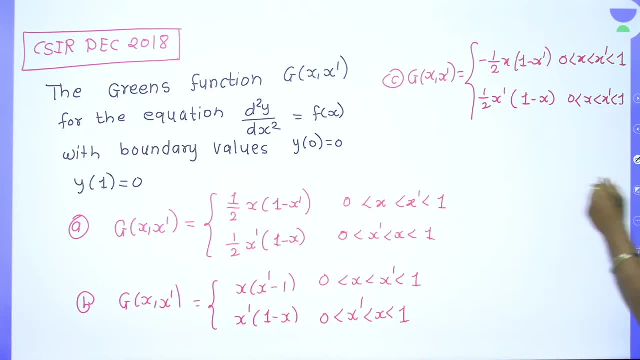 1. okay, this is given to you, and option d, given g of x, x prime is equal to, this will be x into x prime minus 1. this is for 0 x x prime 1 and x prime into x minus 1. for 0 x prime x: 1: okay. 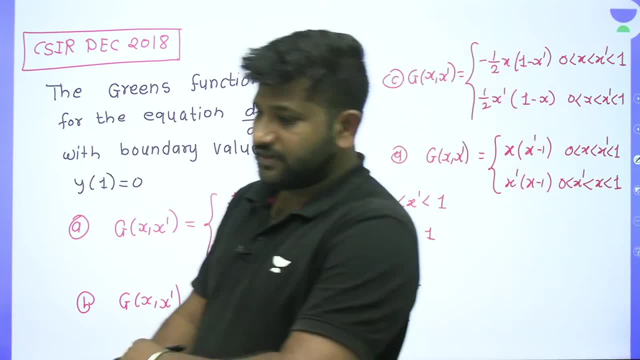 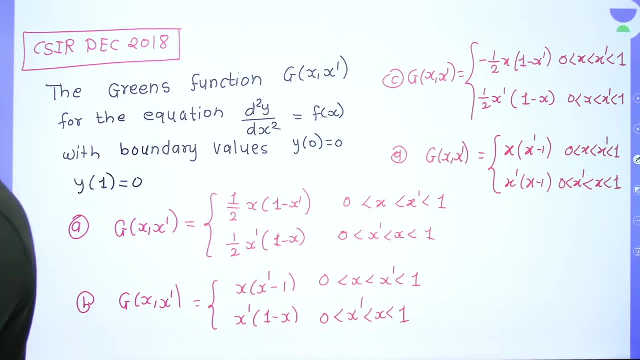 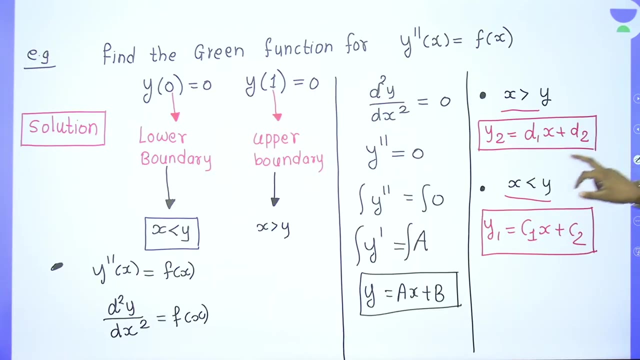 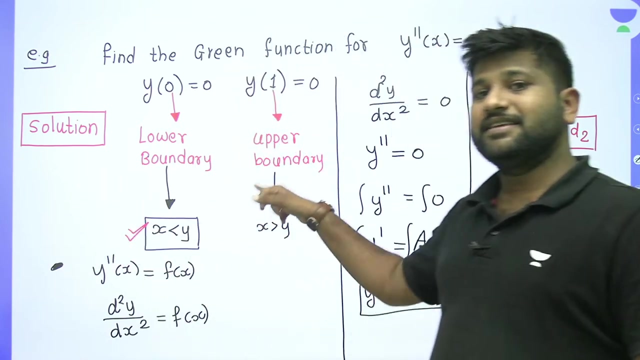 so what is the answer of this? so low boundary or lower value? yes, lower boundary is not for lower value, only take it for lower boundary. lower boundary you have to take for the x less than y source dollars. lower boundary is for x less than y. God is a over already. 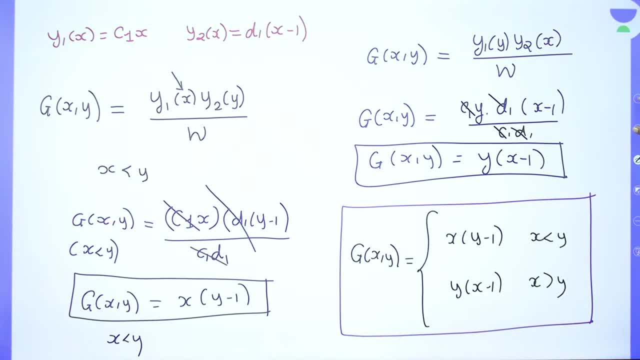 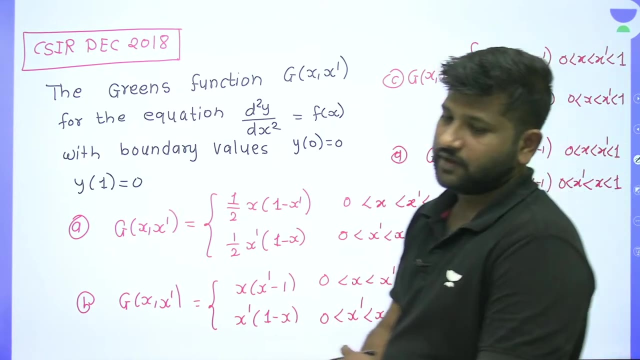 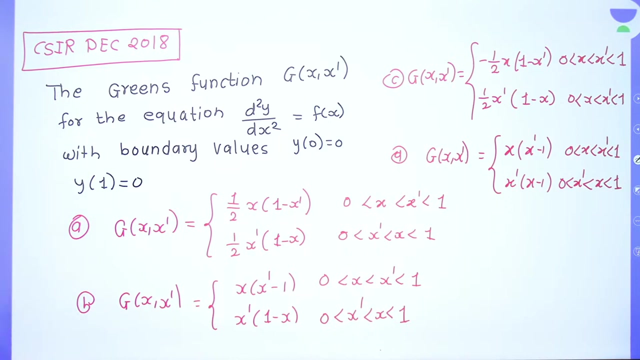 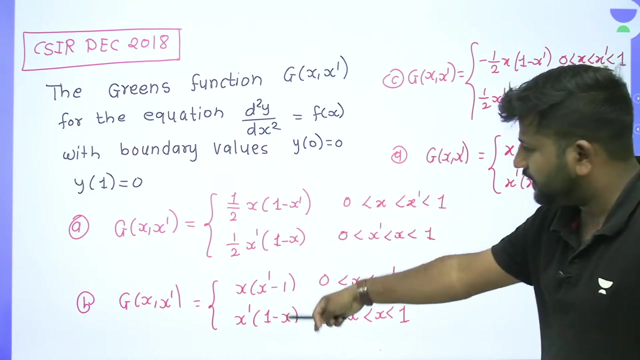 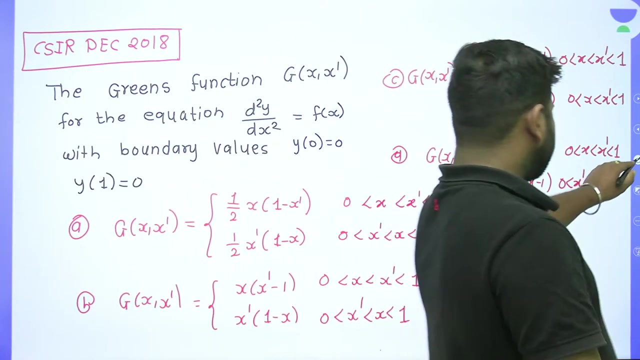 you have to take it. see what is the answer. see what is the answer. see, there is not a scar here. What will be the answer to this? any idea? what will be the answer to this? option D, option B, A, B, C, D: What's the option at this very moment? you will get question of 5 marks. 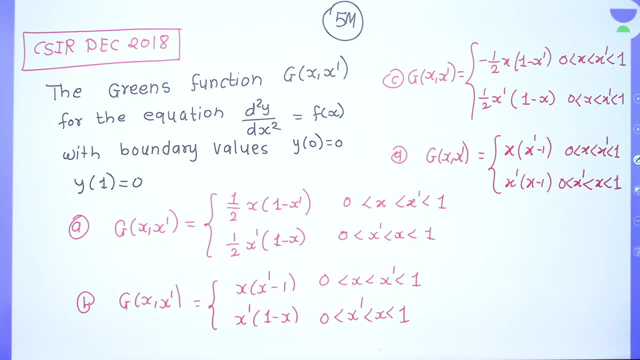 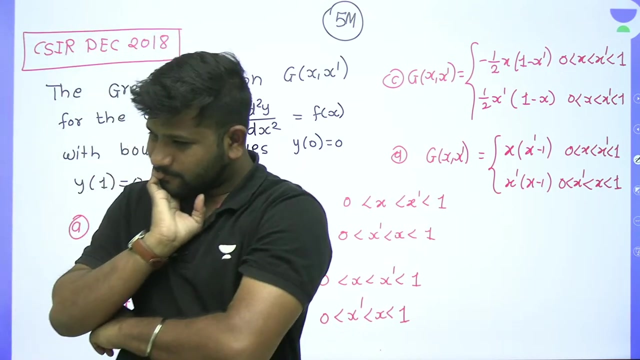 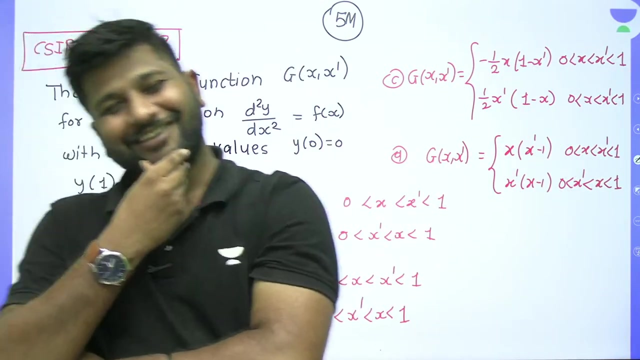 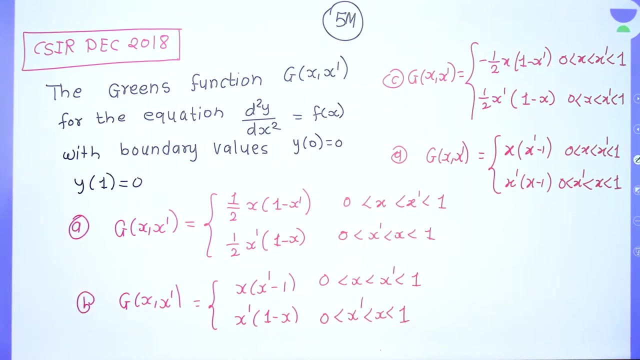 with this function and what will be the answer for this? what will be the answer to this? hmm piace, what is the answer of this? not that much difficult. this is the last problem. this is the last problem. what is the answer? what is the answer for this? 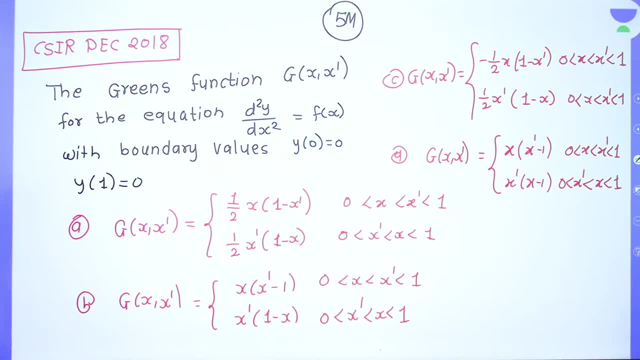 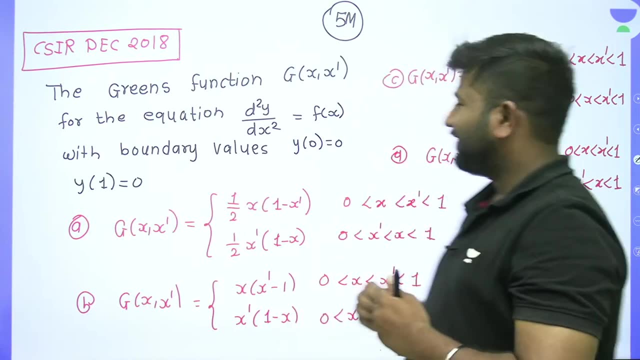 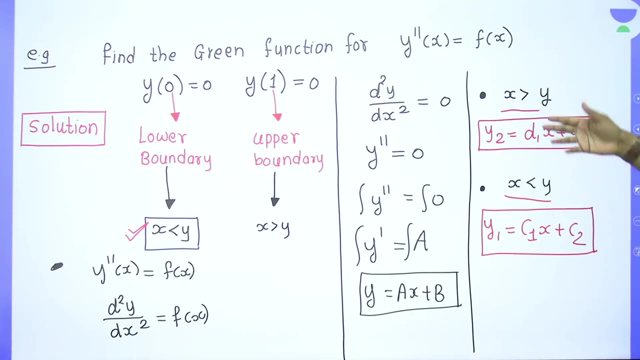 how is this not right? this mistake is not trapped on the will of the teacher. see, this question is same. this is the question given to you. the boundary condition is also given, is not? it is the same as it is now here. we have taken the greens function, so what? 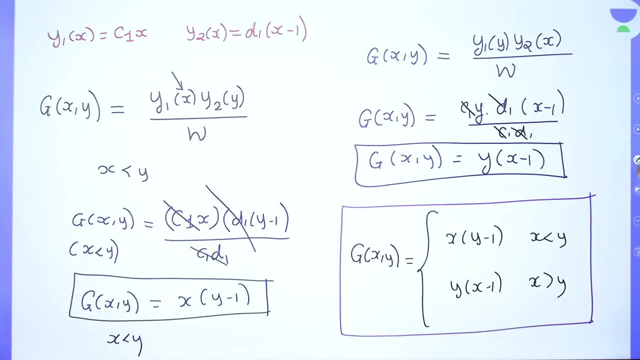 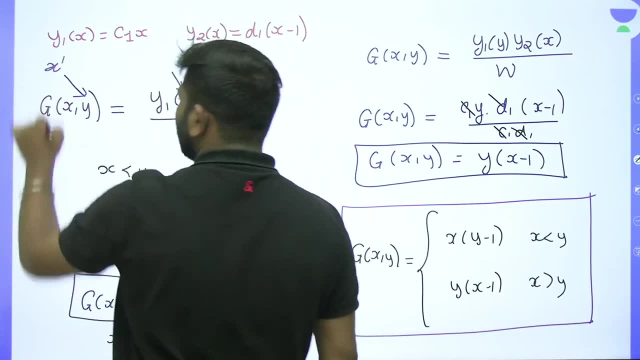 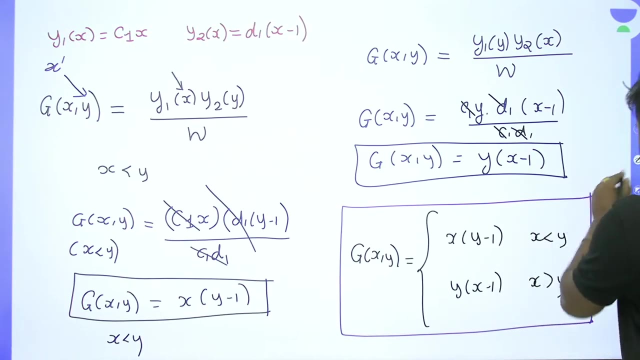 is the green function. so the green function here j of x, y, is not it. what have you taken in place of y? x prime. so put x prime in place of y. So let's say i'll put x prime here, so it will be x prime. put x prime in place of y. 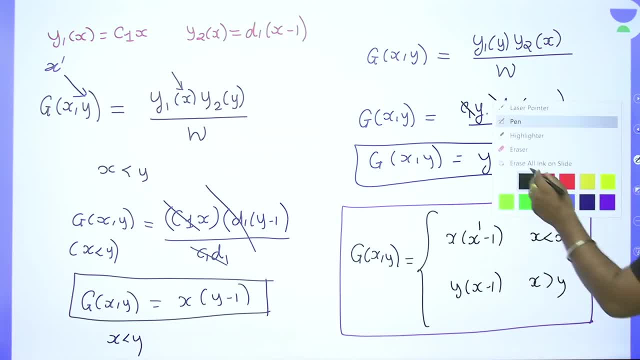 put x prime in place of y, so let's say the resp communities, ok, Ok, Ok, There is a question here. well, here, if instead of y put x prime, right now, this is the same problem. so here are we getting one half, are we getting one half? 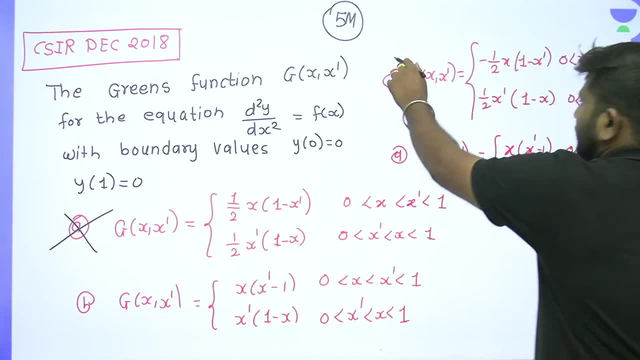 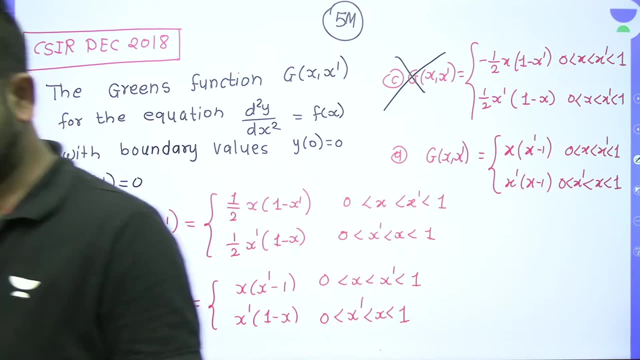 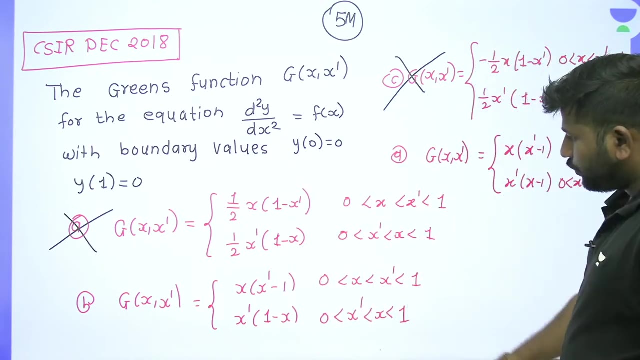 no, here is one half. so this option can't be done. so option a and option c can't be possible. understand: option a and c can't be possible. if it will be, then this will be now in both. all the things are same. see, this and this are same. 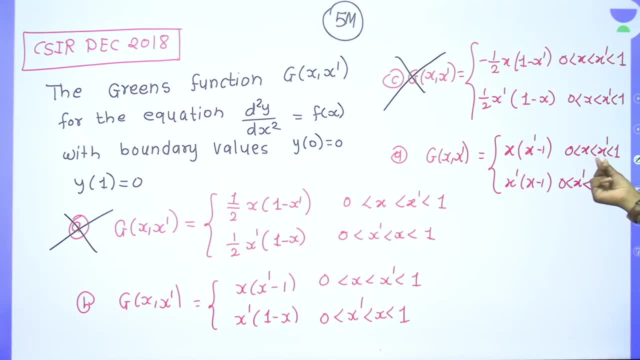 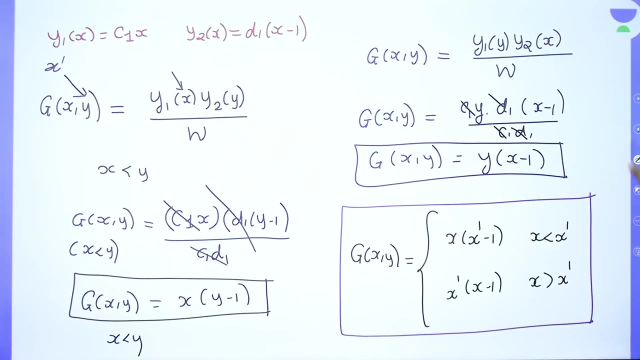 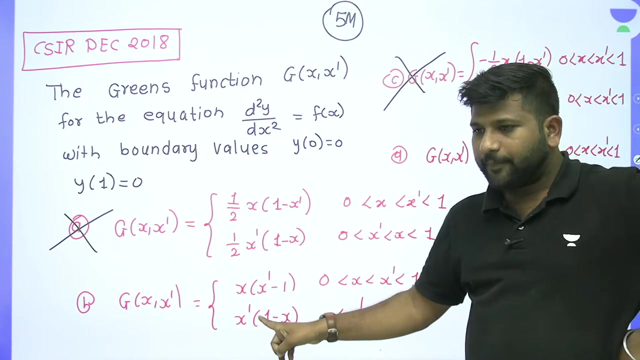 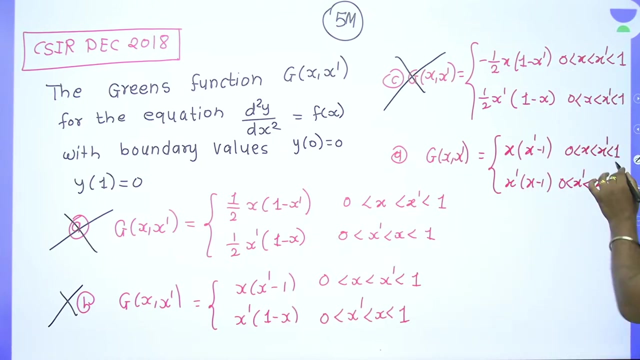 right, is this also same? no, it is upside down now. here see this: x x prime minus 1 so x. what should come in this? x minus 1 so x minus 1. here you can see upside down, see there are times who people. 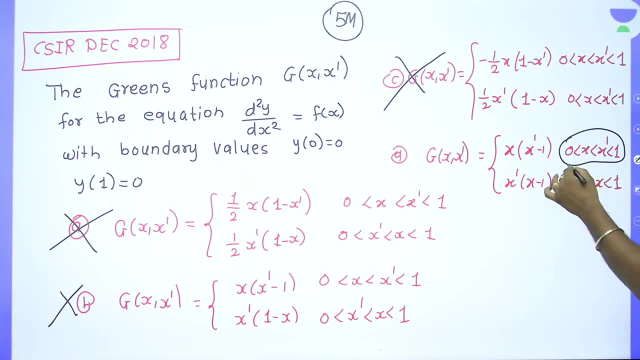 will see here. but there will be two sides. one is behind, the other is in front, so one is moving the number of points. now it will also be its value, because if it's negative, so it is the integral value and the result is negative, so it's a solid white. 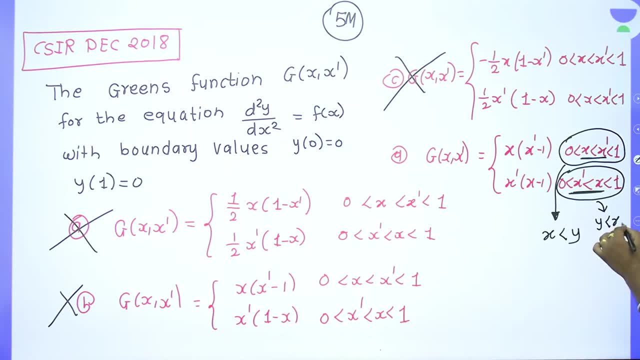 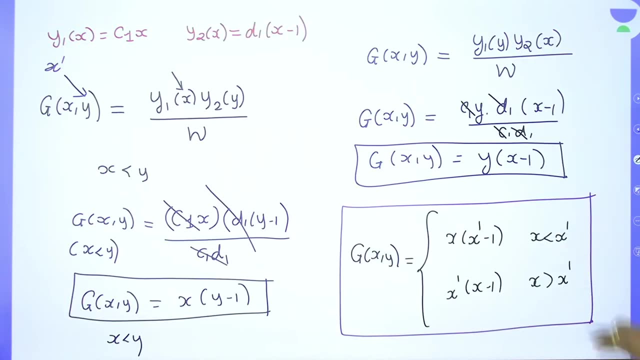 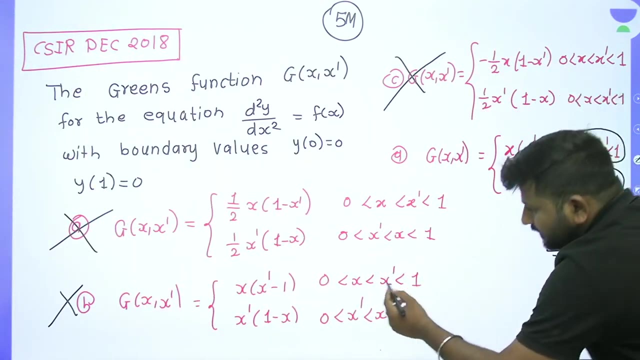 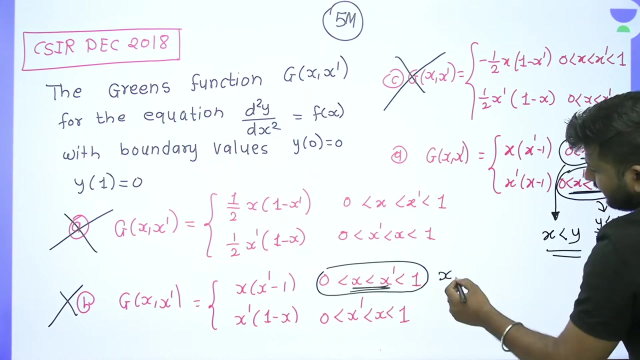 so we will choose like this for this. so here, here is your value, here, understand, ok? so see, here I erased. understand what I am saying, right? so what is the meaning of this? you will think, sir, what is this big? see this middle? so x means x and this x prime means y. 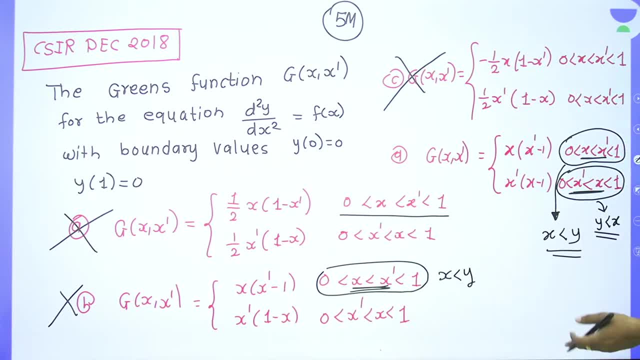 so this is. it means they have given so big confusion, but no need we know this. see, this means this is x, prime. that means this y and x. this is what I gave you, what I did here. understand everyone. is this clear to everyone? move forward. ok, is this clear? 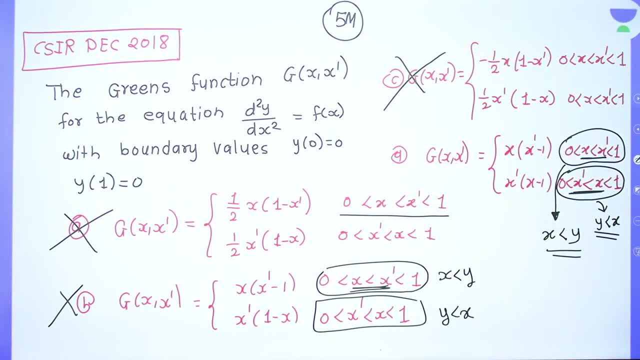 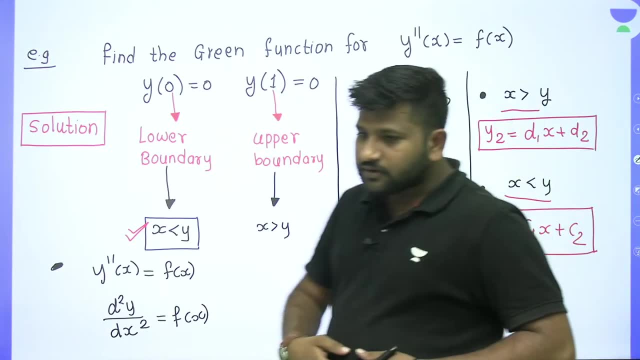 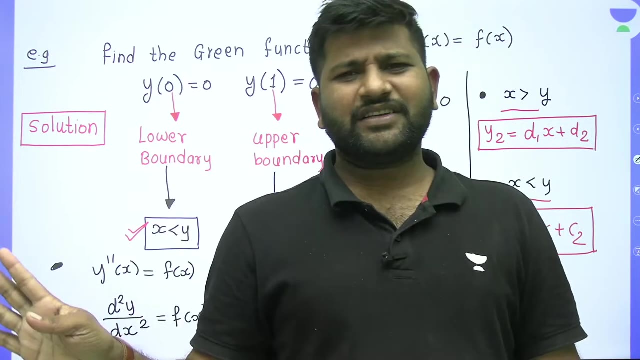 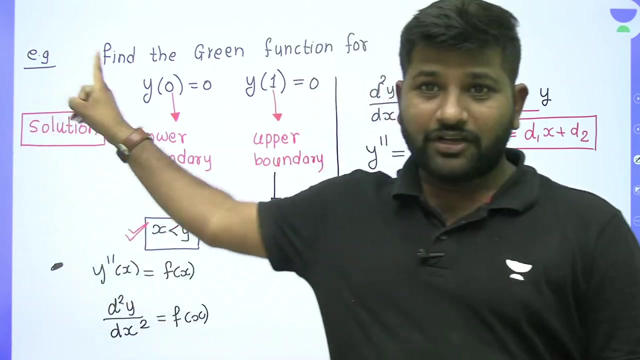 to everyone. see, the procedure is very simple. if you tell the procedure that it is difficult, that means no, it is not difficult at all. it is simple. follow the procedure. see here. only this much is there in the green function, nothing else. now this question. see carefully. we solved this question with so much procedure. 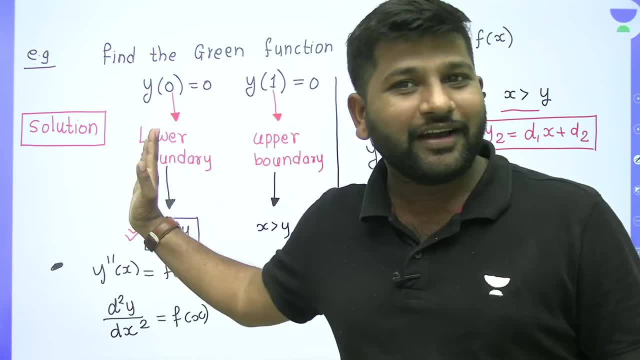 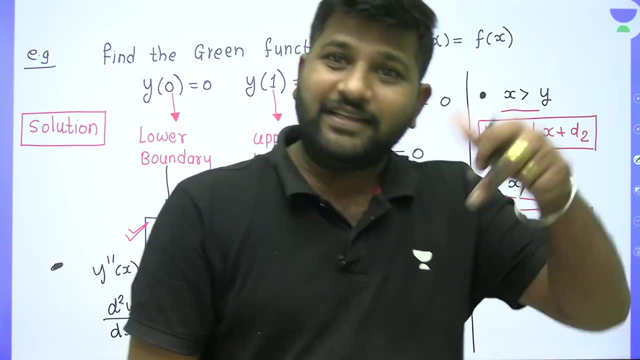 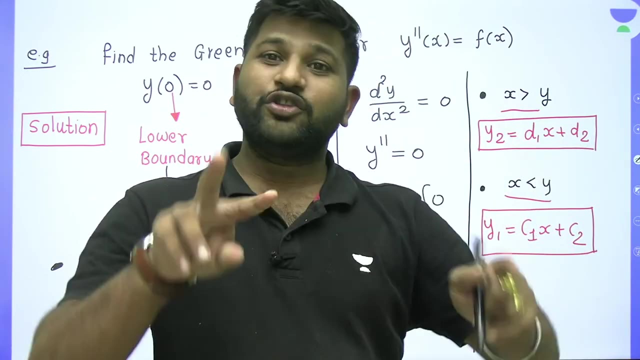 there are some more methods in this to solve this. this is a normal procedure if we have some more conditions. there are some properties of the green function with that property. we can tell which option will be right in this by using the property of the green function. but if 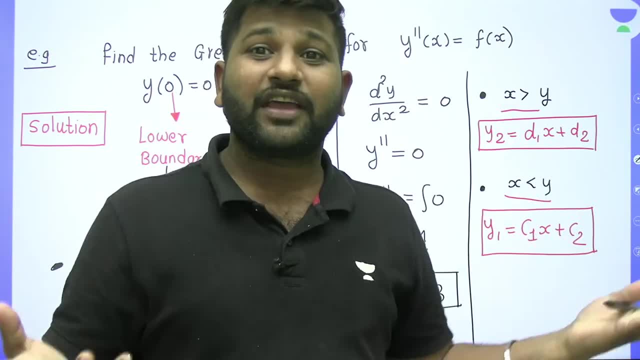 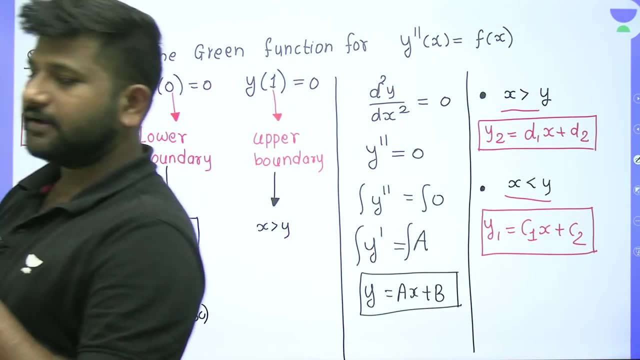 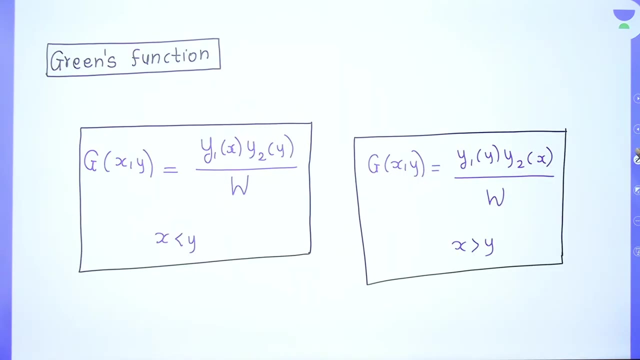 two options are there. if both are satisfying the properties of the green function, then what will happen? then? we have to follow this procedure. ok, we are going to discuss that. I hope you understood this, that I need to explain it again. I don't think it will happen. 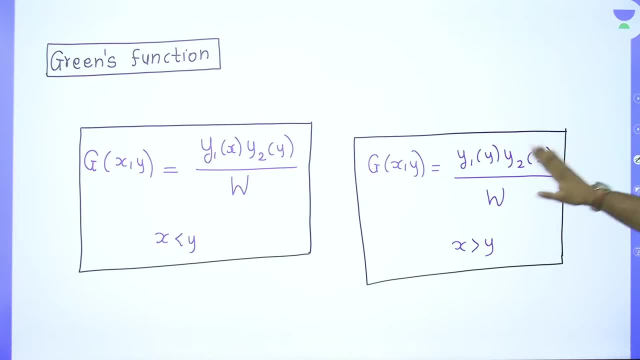 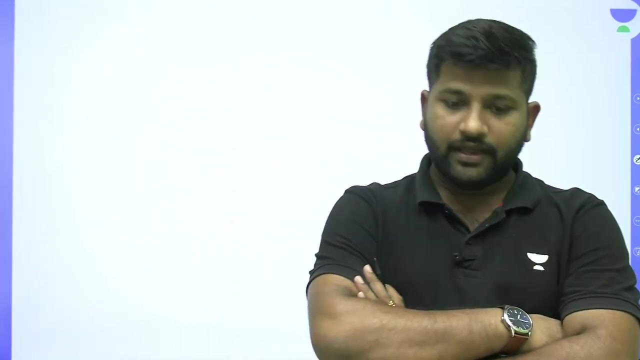 because it is simple. I discussed this yesterday. this is your procedure. move forward now. so what is the green function? again, we come to the green function. so what is the green function? it is used to solve the differential equation. so if we want to solve differential equation, then 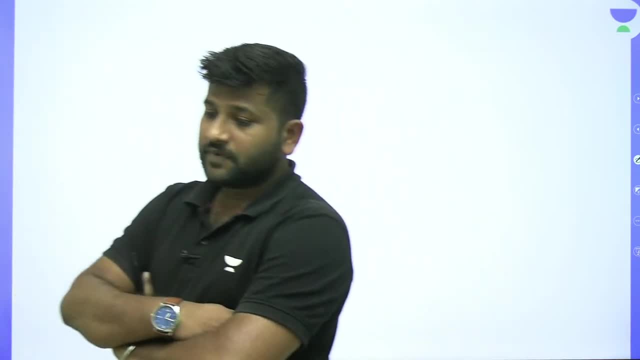 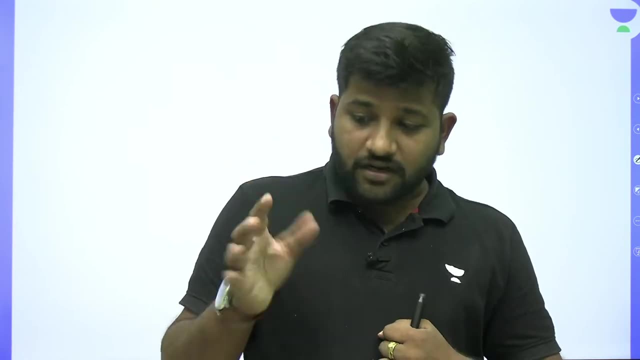 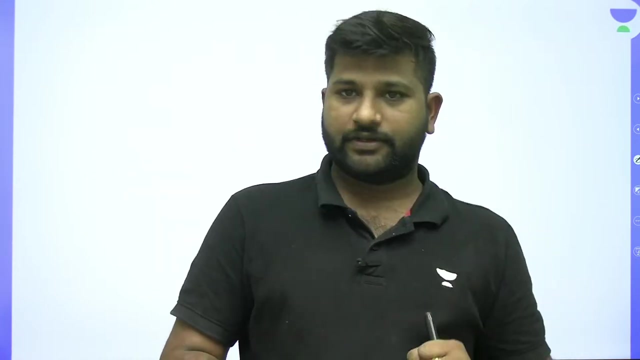 we need the green function. ok, now this differential equation. should the differential equation be second order only or not necessary? third order, fourth order, fifth order, whatever it is, all the differential equations- you can find it out by using the green function. it is not like the green function is only for second order. 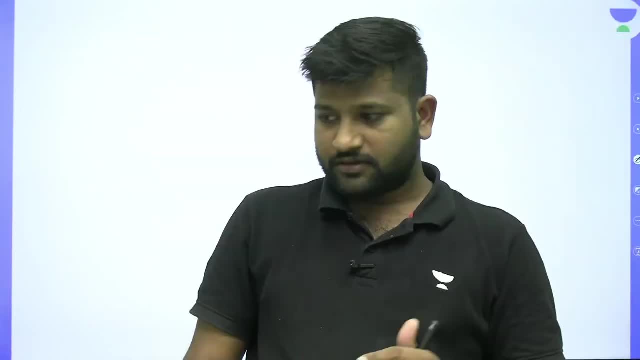 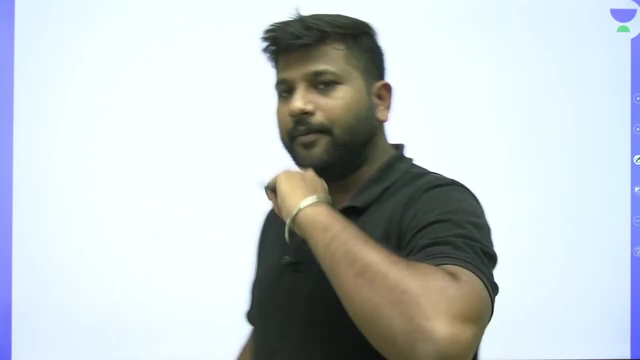 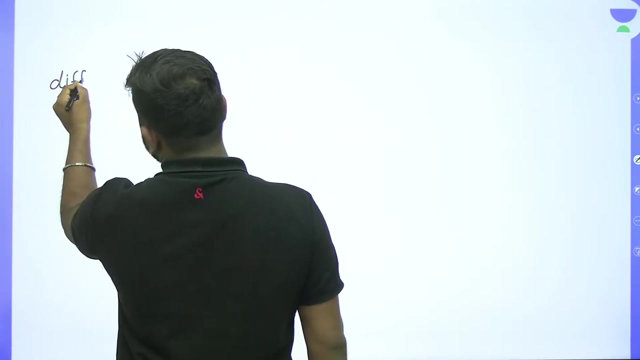 no, it can be used for any higher order, ok, ok, I hope you understood this. now we come here. we come again on differential equation. we are solving differential equation, so differential equation, we take a second order. differential equation, because in examination we take differential equations only up to second order. 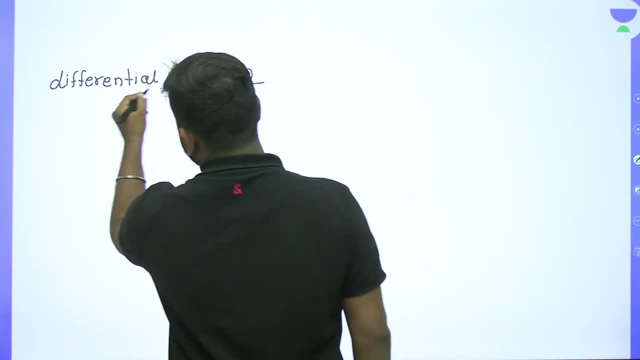 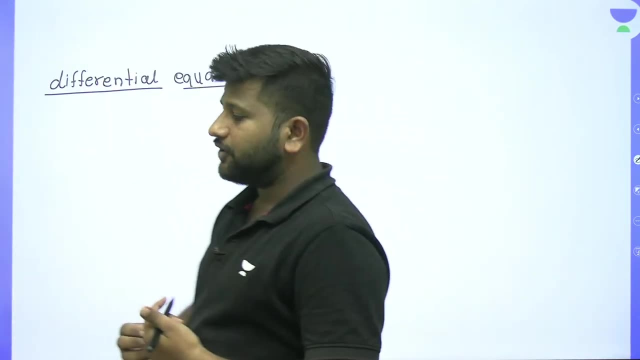 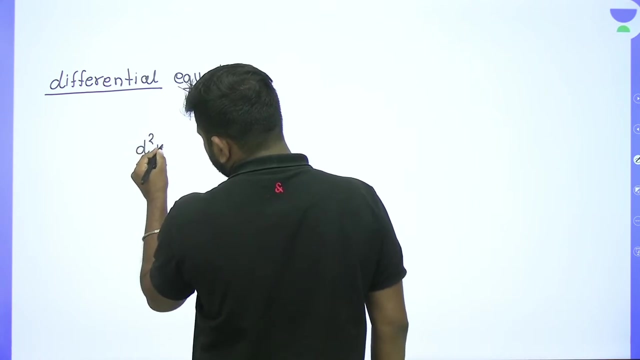 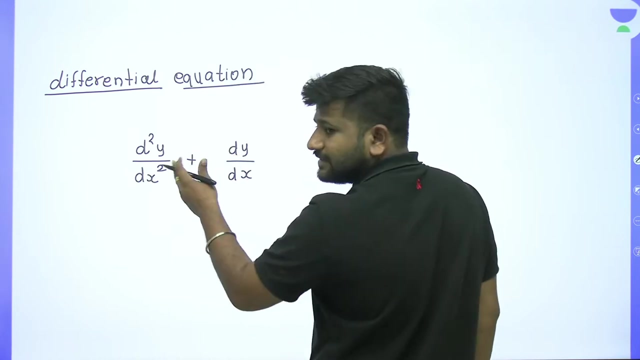 so you find it better to talk about second order? ok, we talk about how second order differential equation is used. now it is not necessary see here, this is theracialitt order. that is, a d square y by dx, square plus dy by dx. this is a second order differential equation. 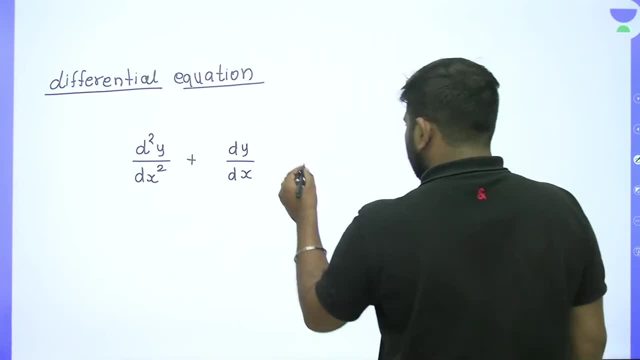 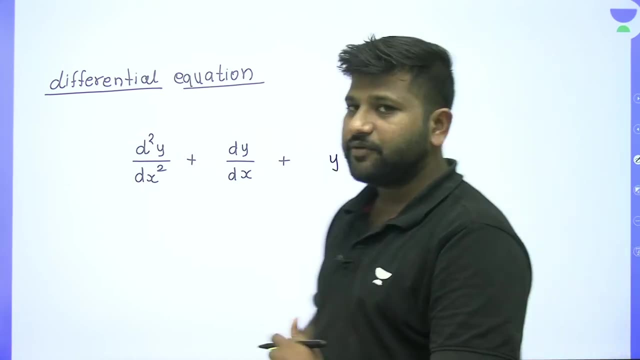 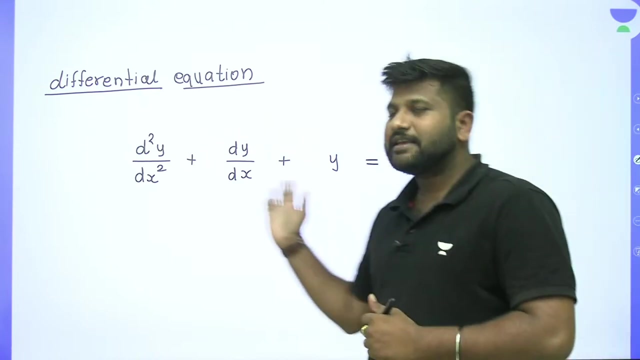 i am just writing: okay, plus something into y is equal to, let's say, f of x. this is your differential equation. okay, you will think that, sir, why did you put space in between? because it is not necessary that your differential equation will be like this. your differential equation can also be like this: this is alpha 1 of x. 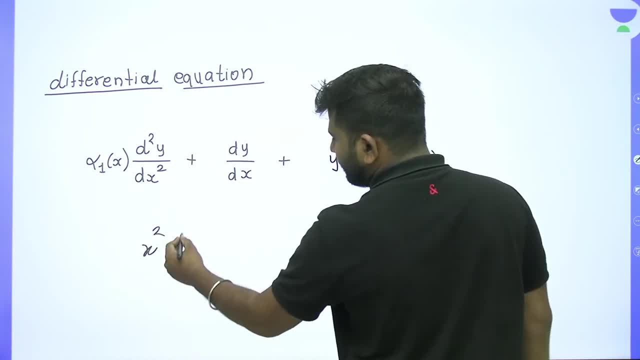 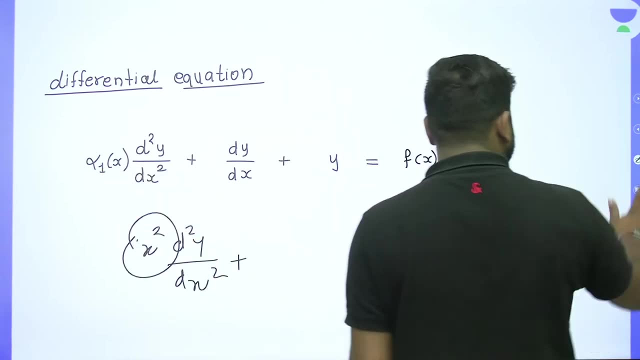 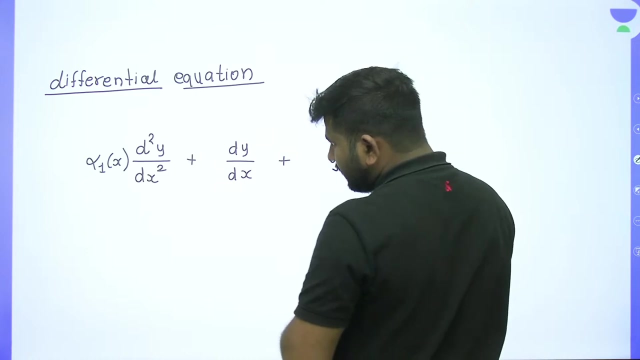 means here. this is also a differential equation: d square, y by dx square. so this can be anything. this can be 1, this can also be this. that is why we write it like this: that this differential equation can also be like this. sorry, 0, 1. 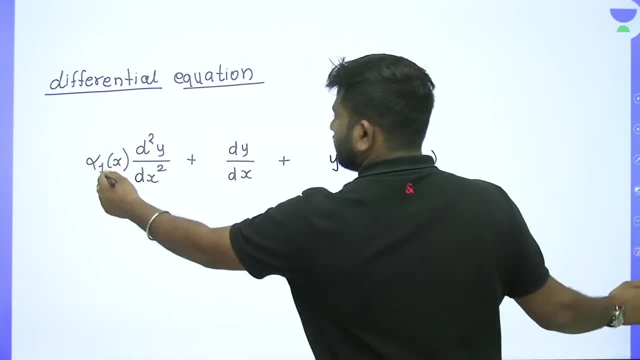 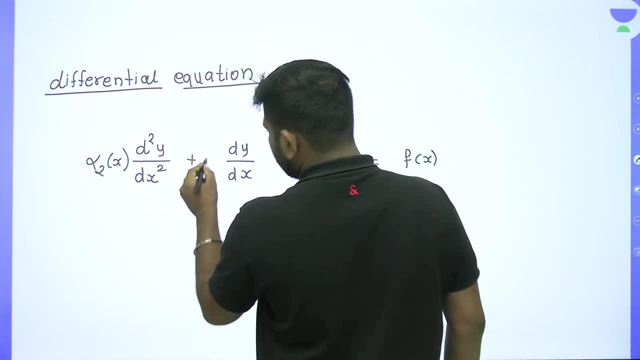 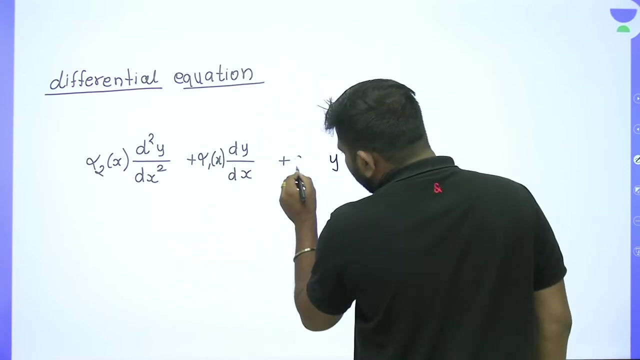 0, 1, 2. this is a 2. this is a alpha 2 of x. this will be your alpha 1 of x, are you understanding? and this will be a naught of x. so this is your differential equation. this is your differential equation. 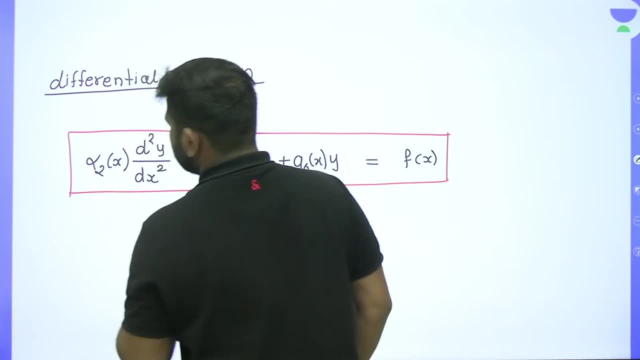 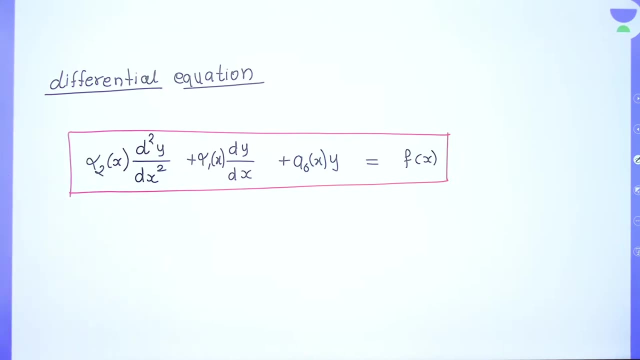 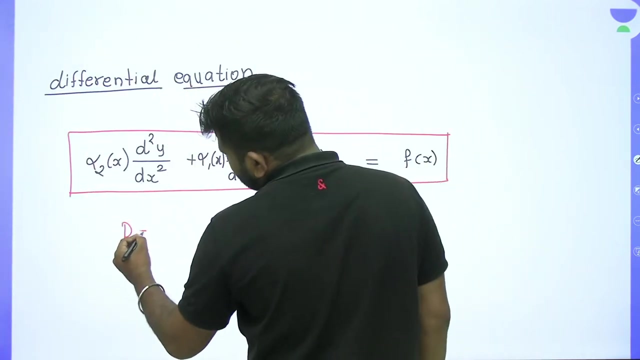 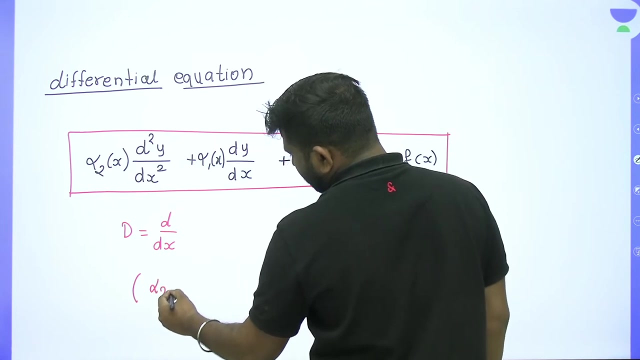 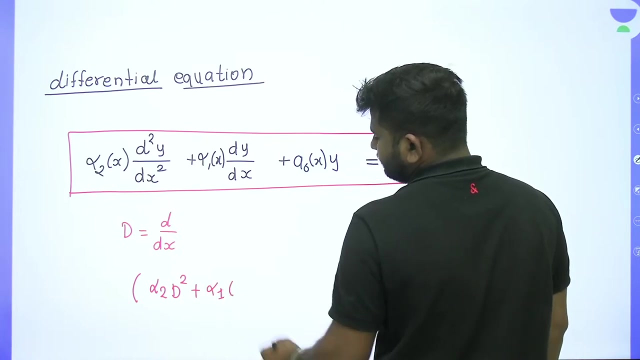 and this differential equation we have to solve by using the green's function, so green's function, so green's function. we have to simplify it, okay, so i can put it like this: that this d is equal to d by dx. if you substitute, that means how much will be your differential equation? alpha 2 into d square, plus alpha 1 into d, right? 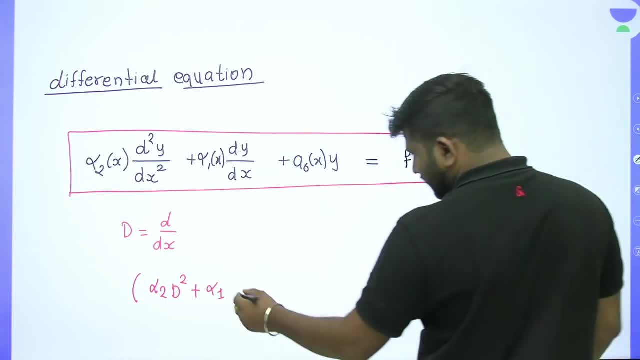 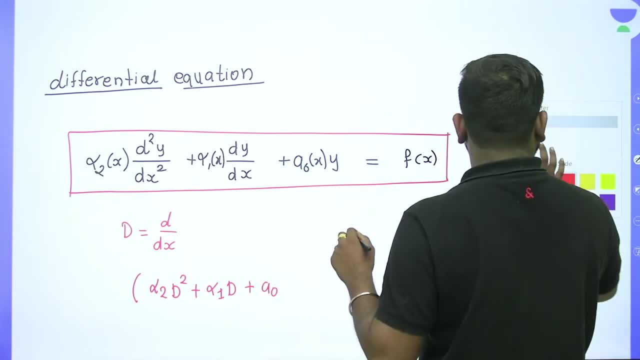 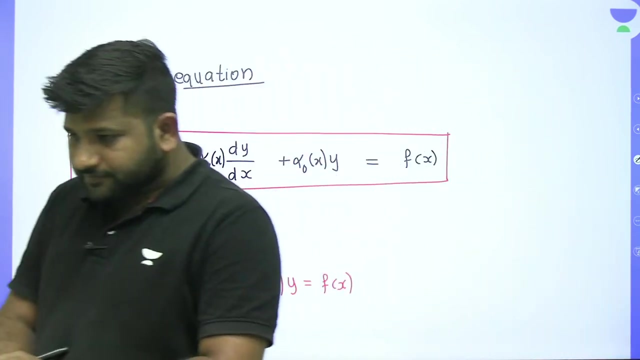 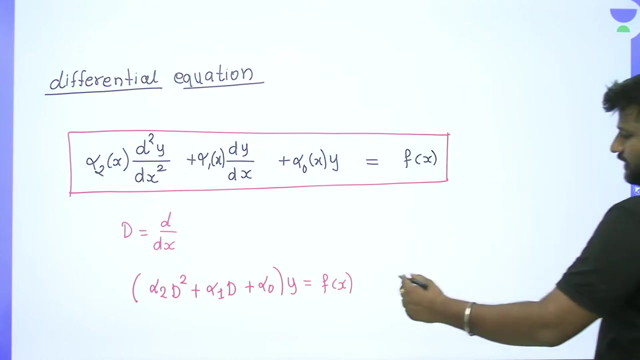 right alpha 2 into d square plus a by 15, by 15. so you write it as this, so like this, and you can write it like this. you write it like this, and you can write it like this: differential equation is this differential equation. 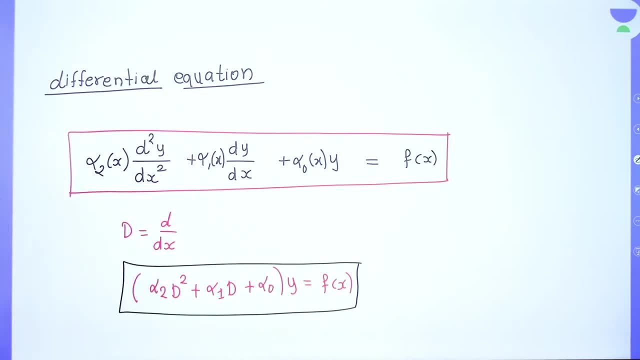 we can write like this as well. Okay, That means here we can see that this is our L of y of x is equal to. you had f of x. if you remember the first lecture, That means here L will be your alpha 2. 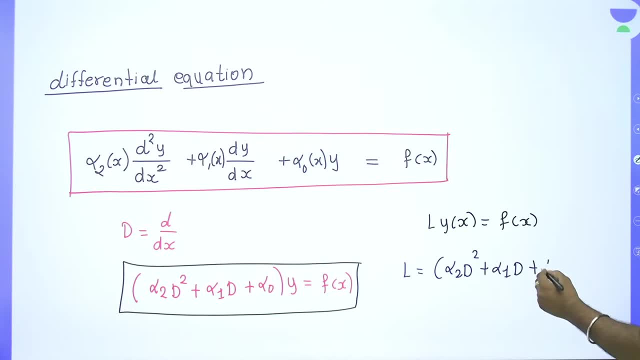 d square plus alpha, 1, d plus alpha. naught Right, This is your L. you can inverse it. That will be your Green's function. Okay, Sir, what are you trying to say? Just see what I am trying to say, Okay. 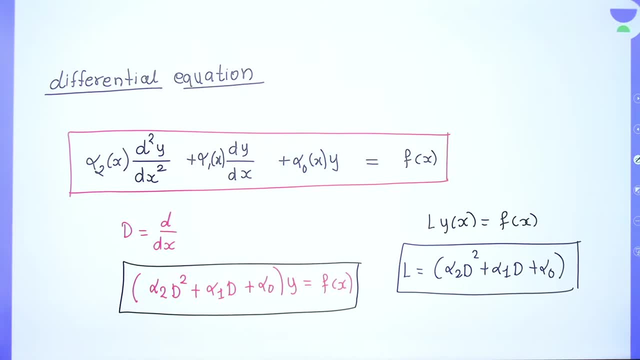 Now to solve this, we will use Green's function. So now, here we are going to discuss that, this Green's function. what are the properties of this Green's function? What are the properties of Green's function? Okay, What are the properties of Green's function? 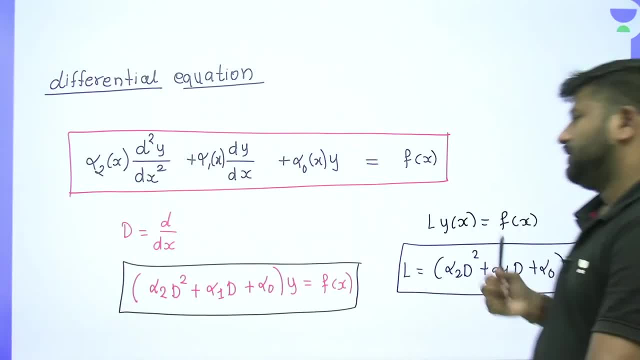 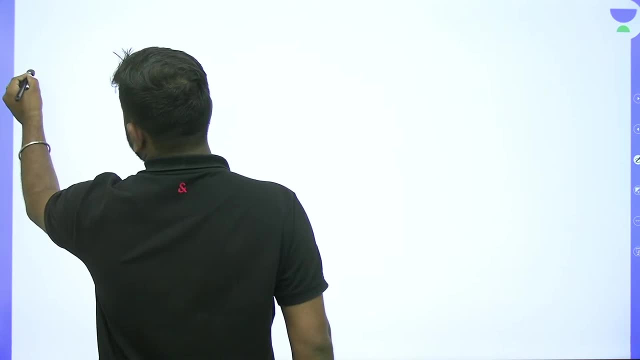 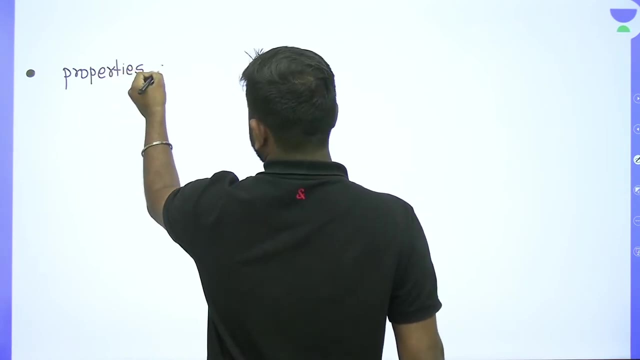 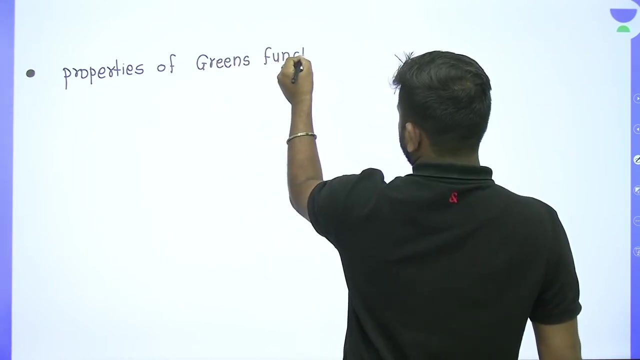 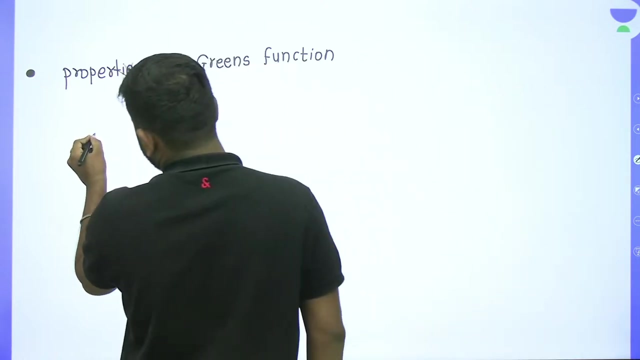 That property we are going to discuss now. Okay, So properties of Green's function, Because from this property you can find out properties of Green's function. Properties of Green's function. So there are some properties of Green's function. What are those properties? 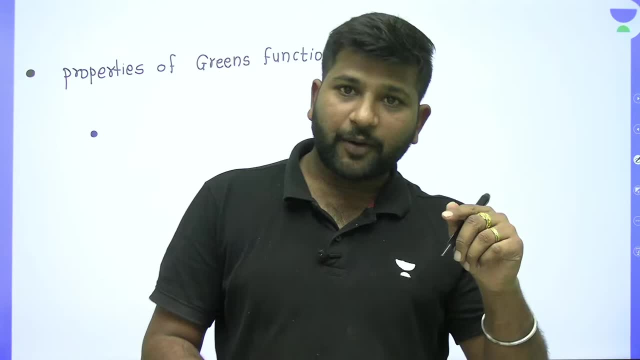 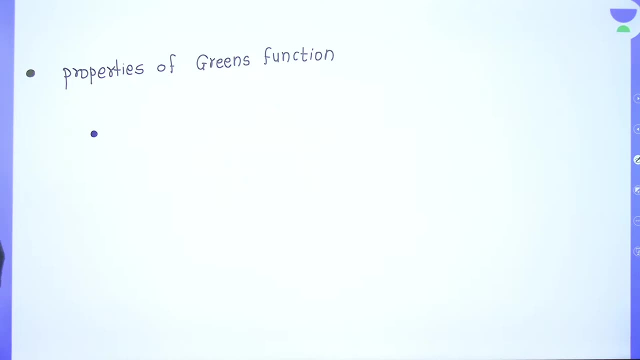 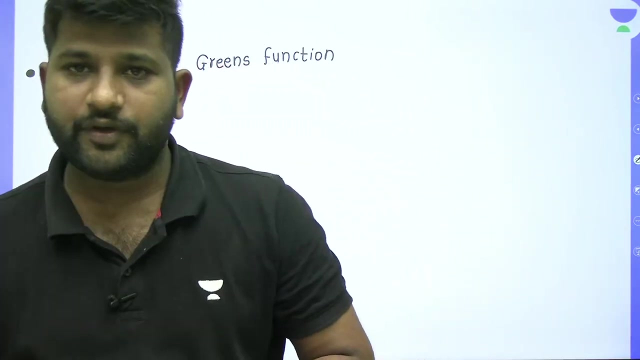 We are going to discuss here. So from that property we can directly find the answer. Okay, So this Green's function is: when you have been given a differential equation, So that differential equation is given in that, In that boundary conditions will be given to you. 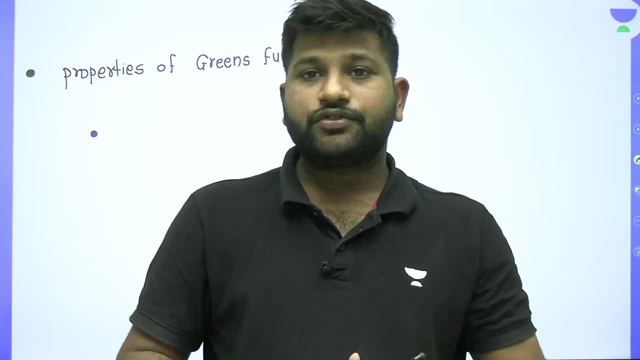 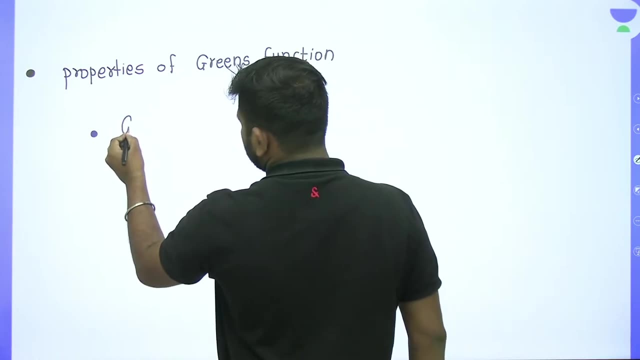 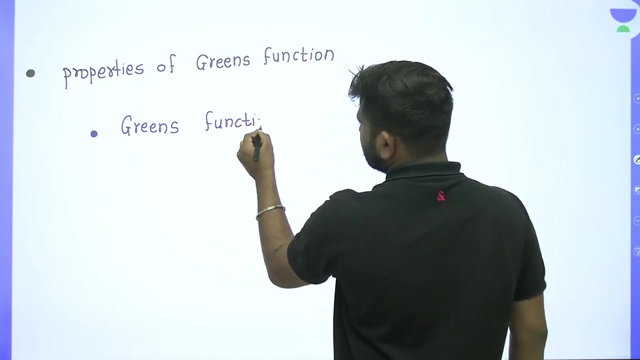 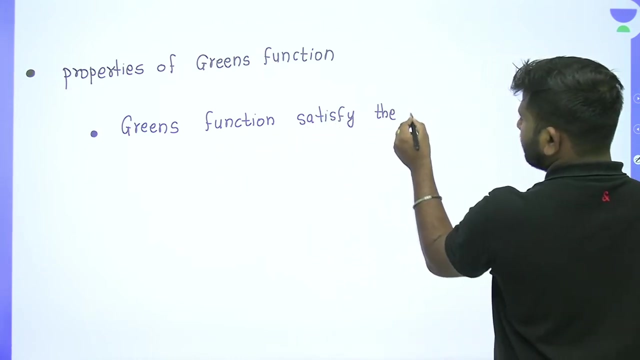 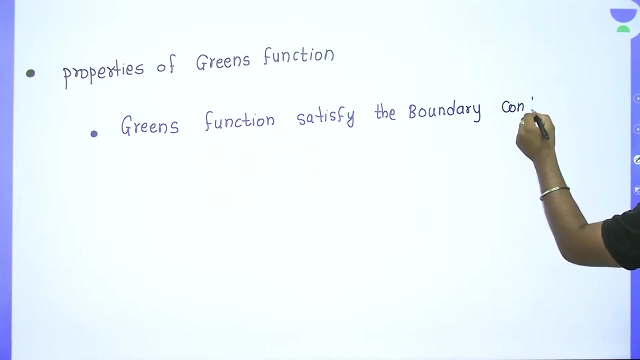 So if you are given the boundary conditions, So whatever green function you will get, Whatever you will get green function, This green function that you will get, Green function, satisfy The boundary conditions. Green's function also satisfies the boundary condition. Green's function satisfies the boundary condition. 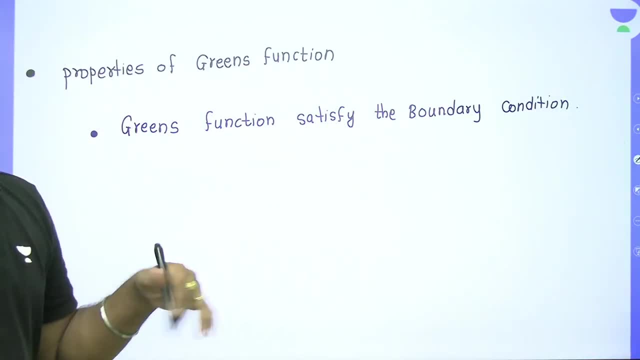 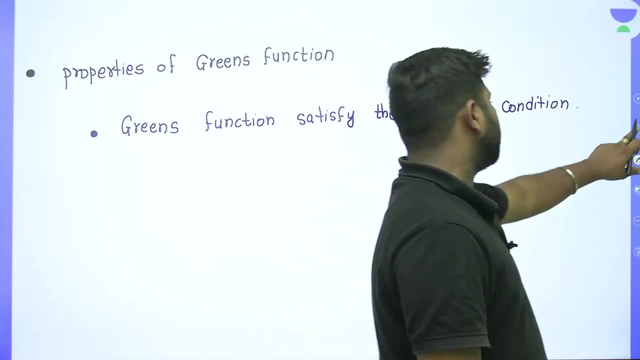 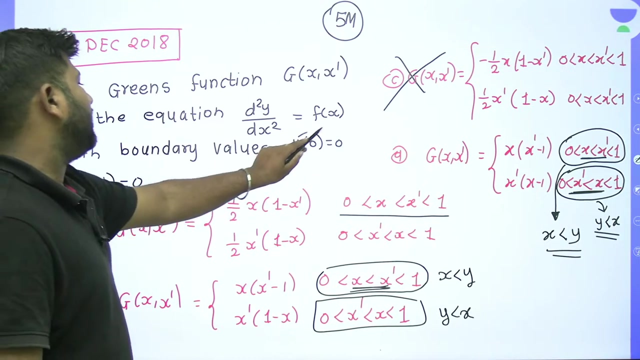 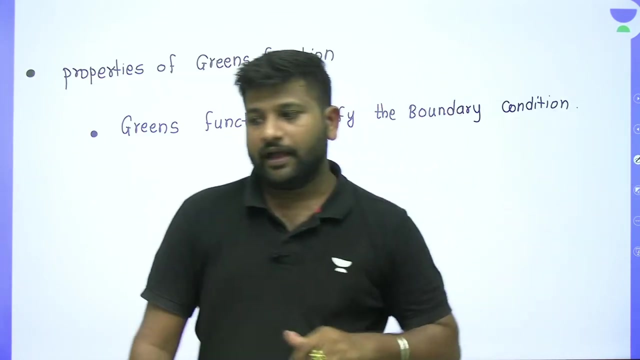 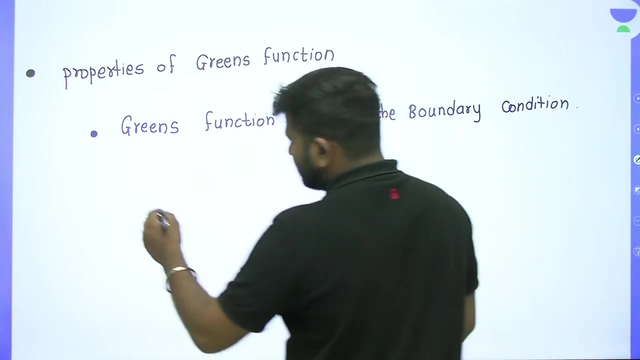 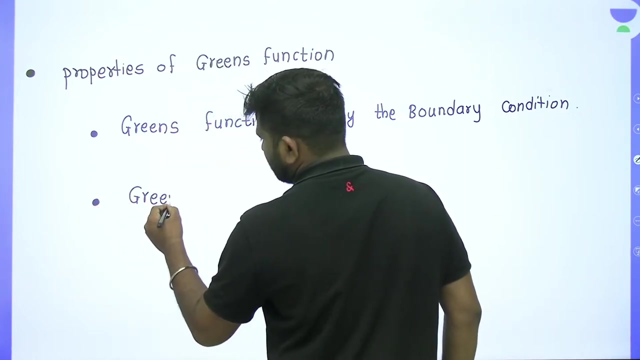 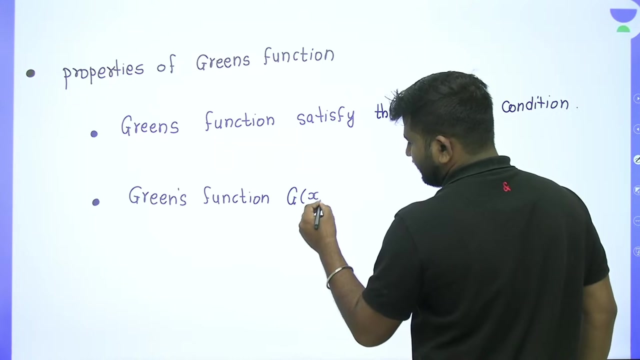 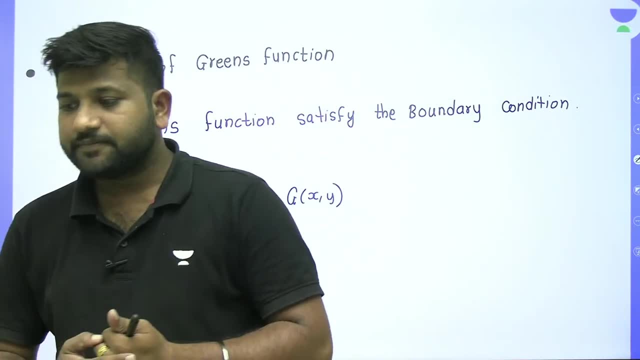 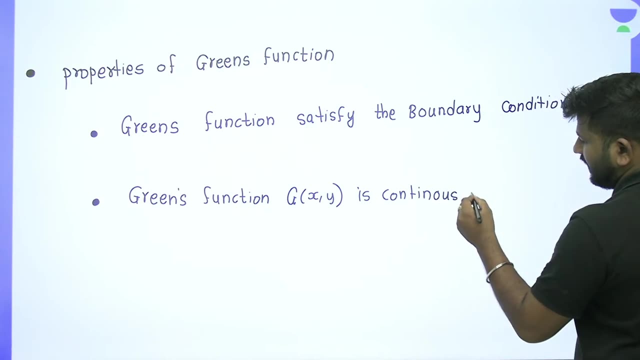 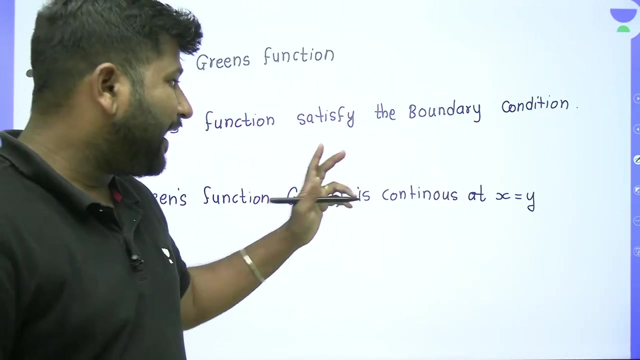 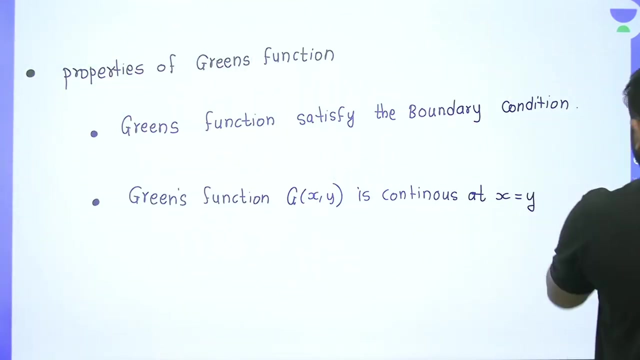 This Green's function- This Green's function is continuous- Is continuous at x is equal to y. So Green's function will be continuous at x is equal to y. Ok, Means See here. This means This is your y, This is your y. Now you will approach this region from here. 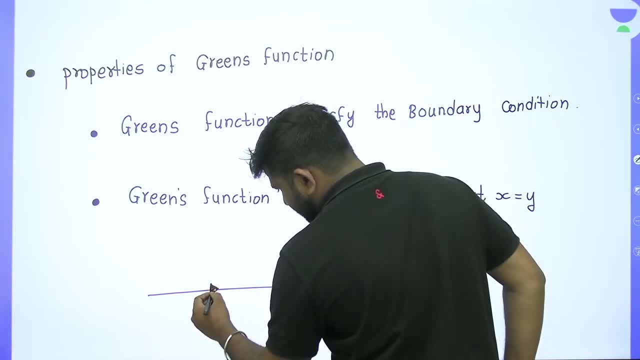 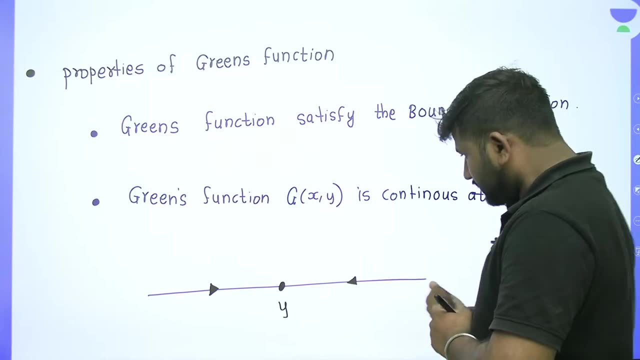 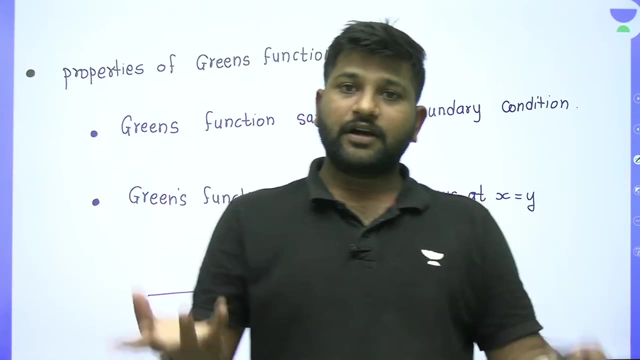 And here this region, you will approach from this direction. That means, If you approach this Y through this region, Or from here Or from this region. So what is this Green's function? It is continuous. it means that its limit should definitely exist. If any function is continuous, it means that its limit will exist 100%. 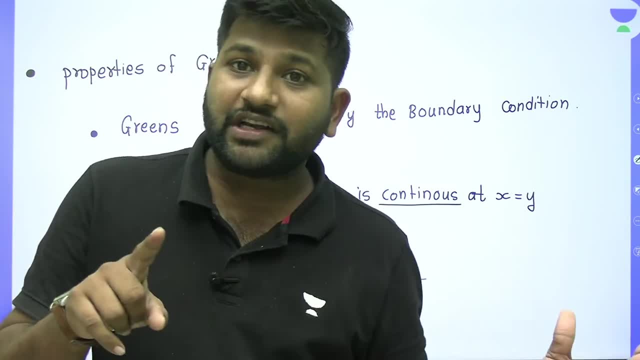 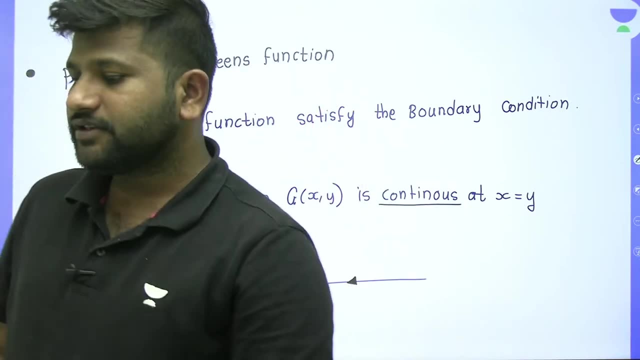 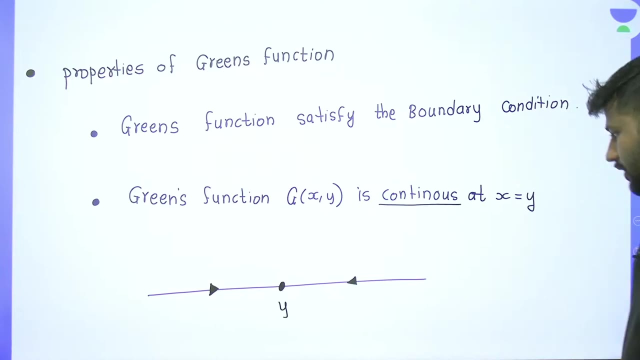 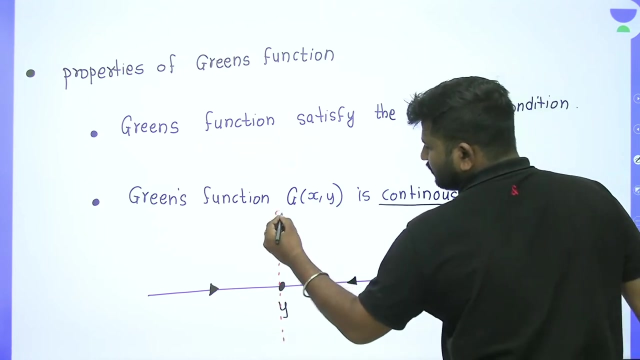 If the limit exists, then the function will be continuous, but if the function is continuous, then the limit will exist 100%. Everyone knows this right. So what is this region? If I look here, then this is y. let's say y is equal to 3. 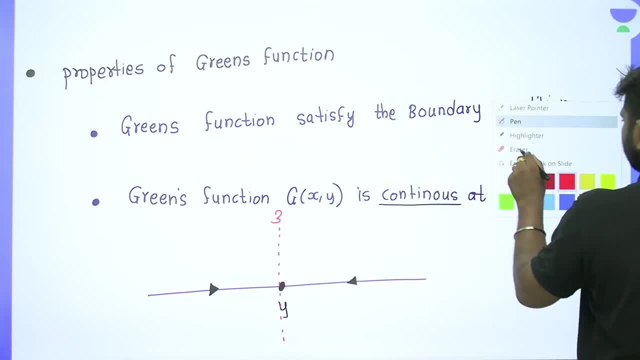 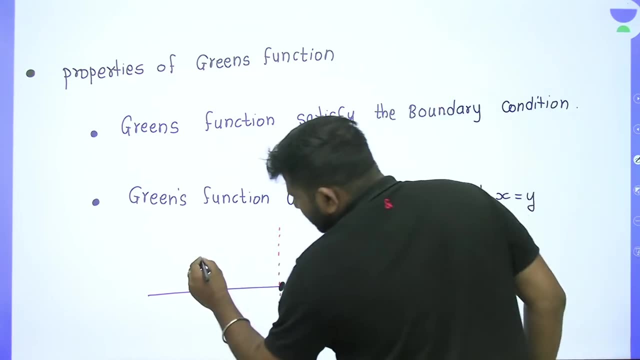 If I take x here, then what will be x? It will be more than 3, that means x is greater than y. What region is this? This is x greater than y and this region is x less than y. And if you take the Green's function, 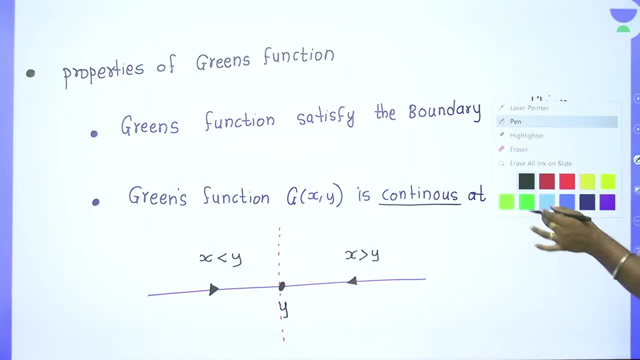 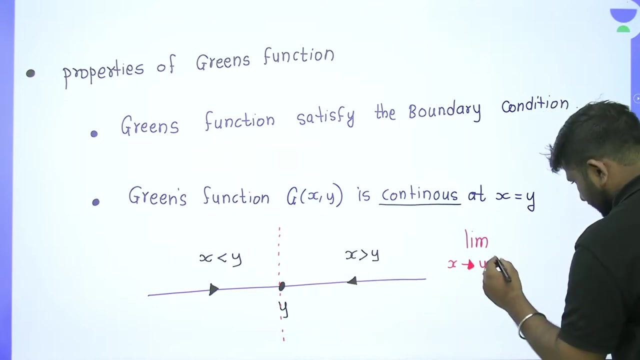 So if you take the Green's function, then what is this Green's function? It is continuous. Green's function is continuous at x is equal to y. This means that the limit x tends to y. If you are going from this direction, let's say this is y plus of g, of xy. 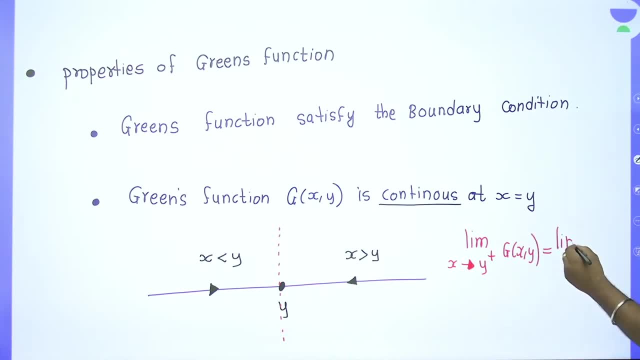 It should be equal to the limit. x tends to y minus. y minus means If you are going from this direction, it means that the limit should exist in the opposite direction. So we will give you in the example or in the question that find out the Green's function and give four options. 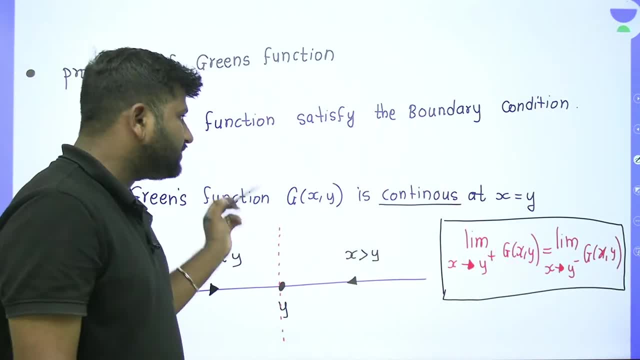 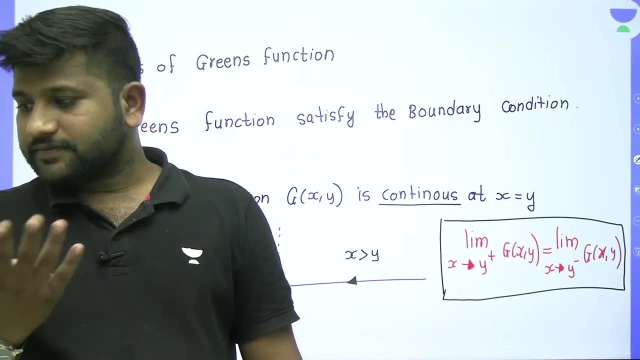 If you do not know how to find out the Green's function, then just use this condition: See if the limit is existing or not. Do you understand what I am saying? Green's function, as you have given four options here. Green's function, as you have given four options here. 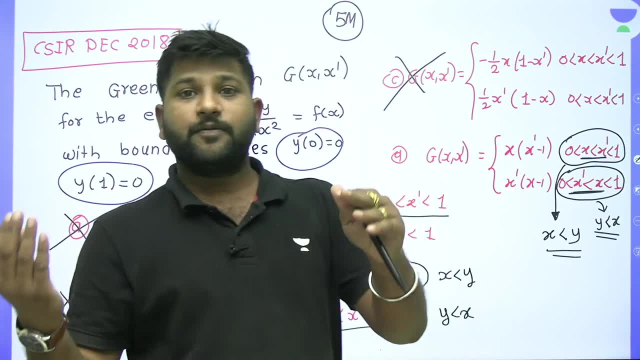 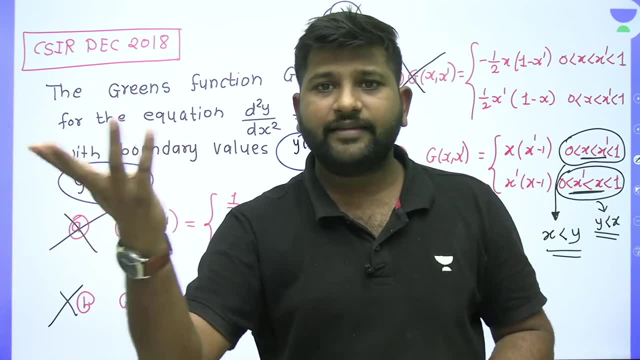 In these four options. you don't even know how to find out the formula of the Green's function. You don't have any idea. You have no idea how to find out the formula of the Green's function, But you know what the properties of the Green's function are. 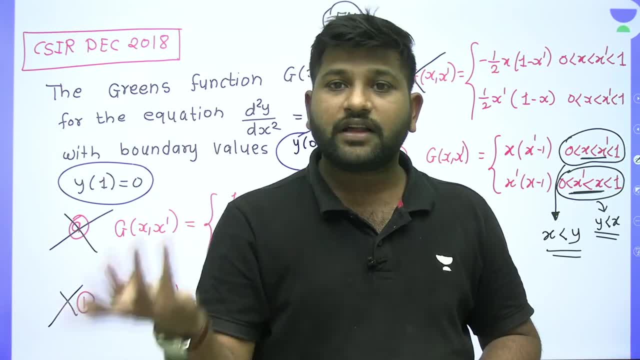 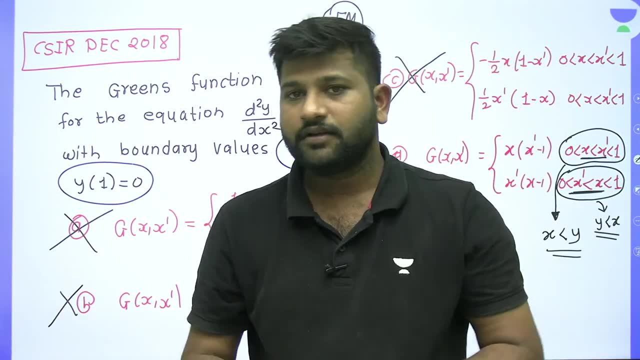 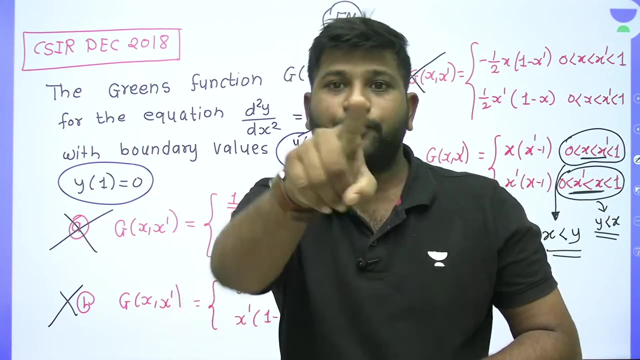 So check which option is satisfying the properties and which is not. The property that is satisfying will be the Green's function. What is not doing will not happen at all. That's it. You can do it in two ways. Even if you don't know the procedure, you can find out the answer. 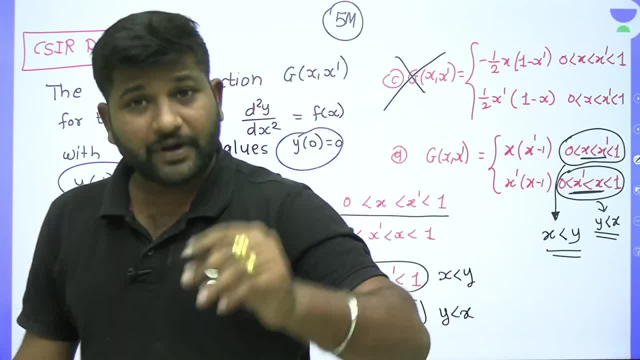 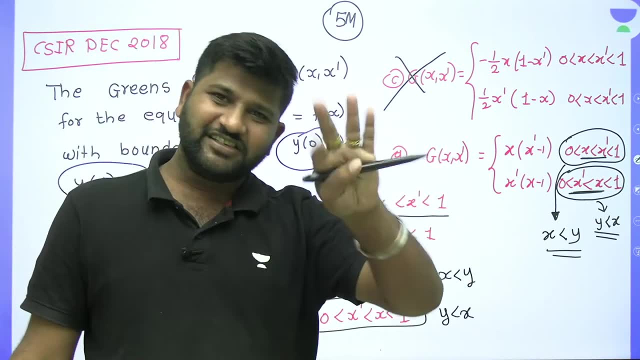 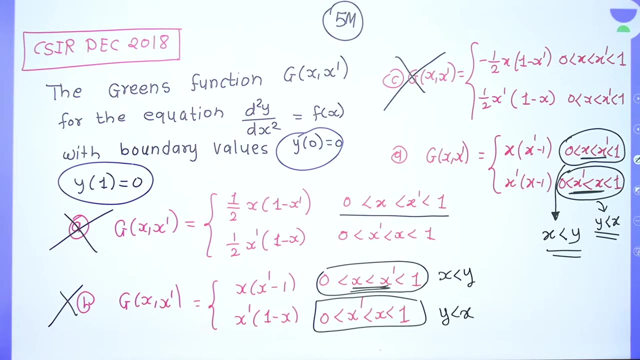 By using, with the help of the properties and with the help of the options. This is applicable for all Green's functions. Any type of Green's function is applicable for all types of Green's functions. Do you understand? Is this clear to everyone? 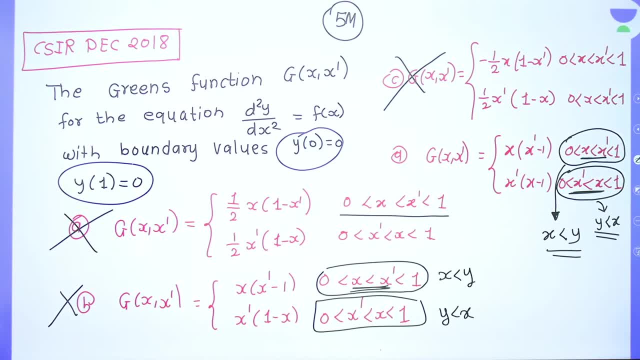 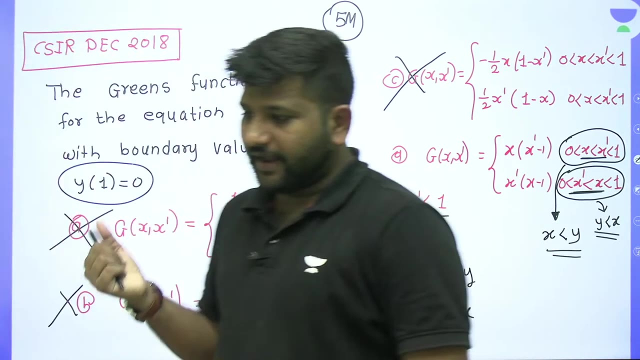 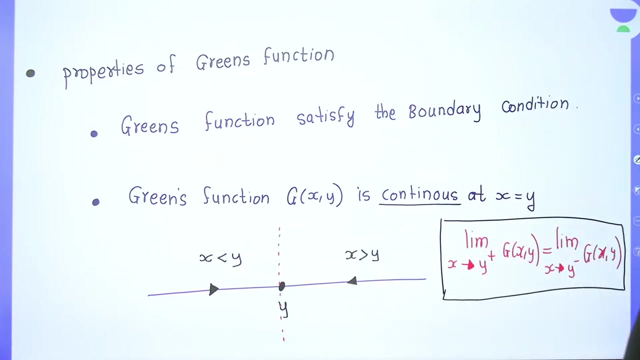 Yes, it's applicable. Does anyone have any doubt or problem? Okay, Let's move on. This is the property first and second And a third property, Because it can happen that you have four options. They have given four options to you. 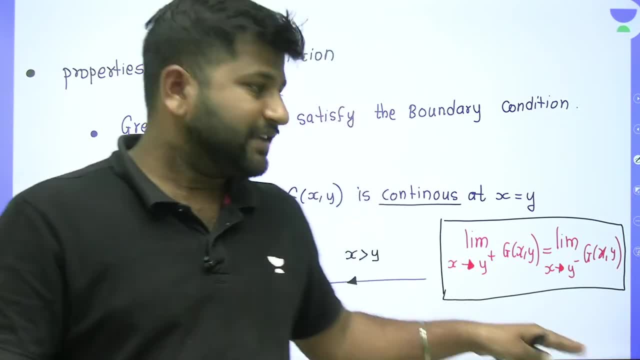 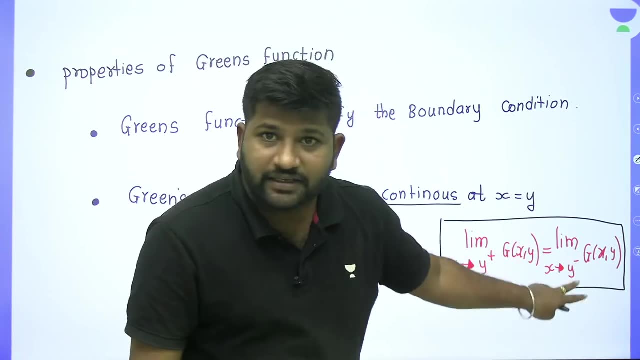 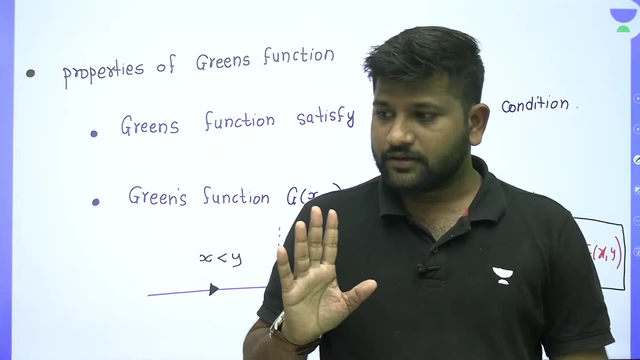 And in four options, only two options are not satisfying, But two are doing So. which Green's function will happen? Means, even after this condition is satisfied, you can't know which Green's function is. Do you understand? Okay, So for that there is another condition. 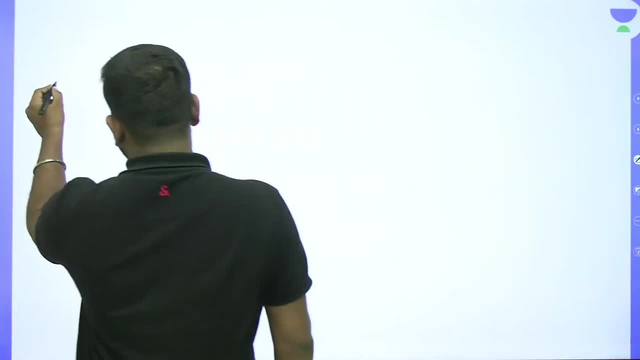 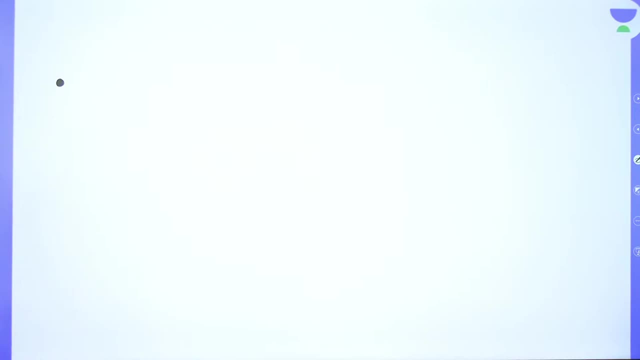 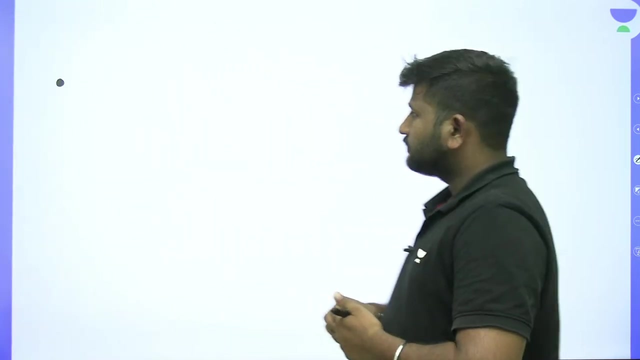 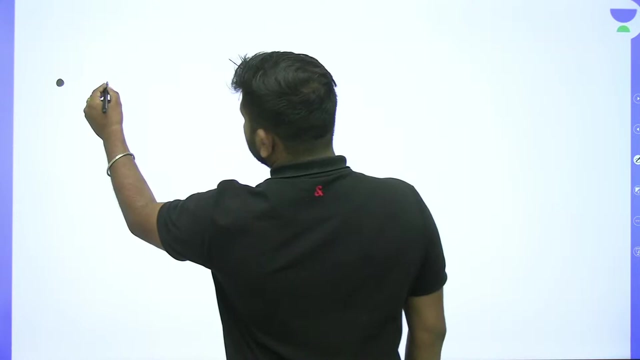 That is the third one. Means, there is no condition. Means, there is no condition. There are properties, Properties of Green's function. Okay, So what is this Green's function? It is continuous, So differentiate it. So the differentiation of Green's function. 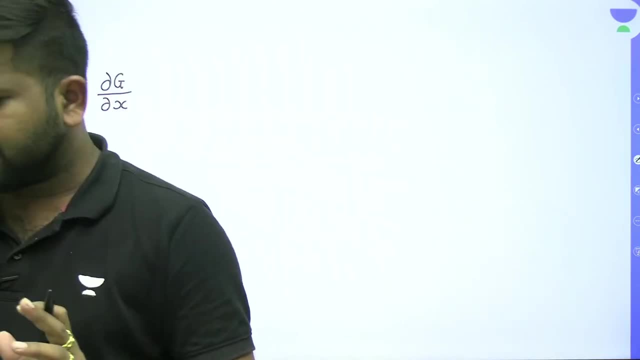 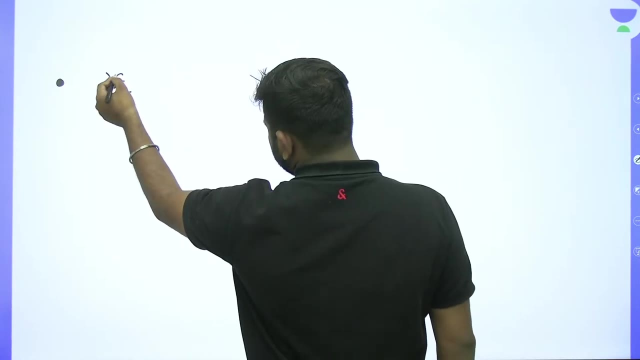 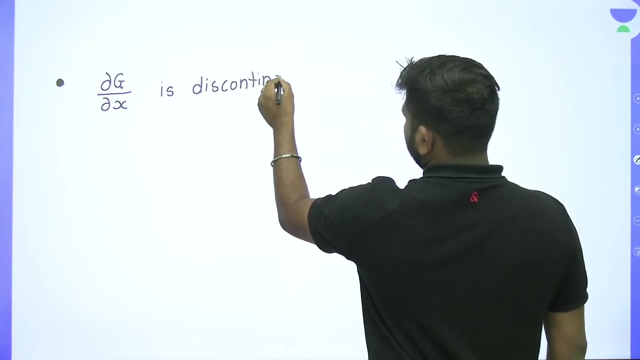 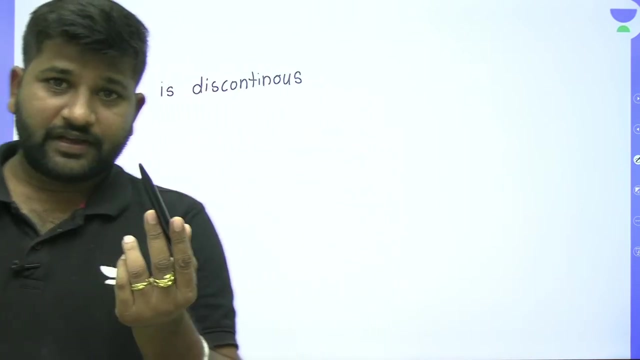 Right: Differentiation of Green's function. Look carefully: Differentiation of Green's function is a discontinuous Differentiation. That is, del G by del x is discontinuous. That means if you differentiate the Green's function, then what is its differentiation? 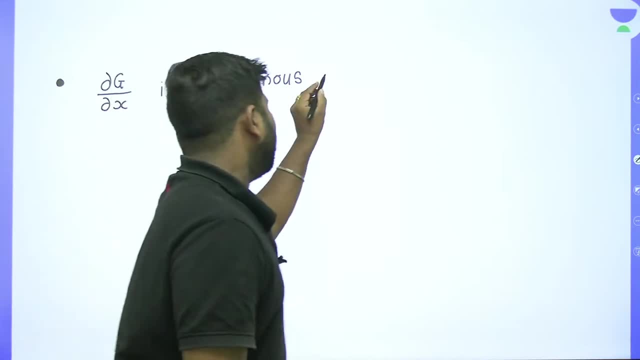 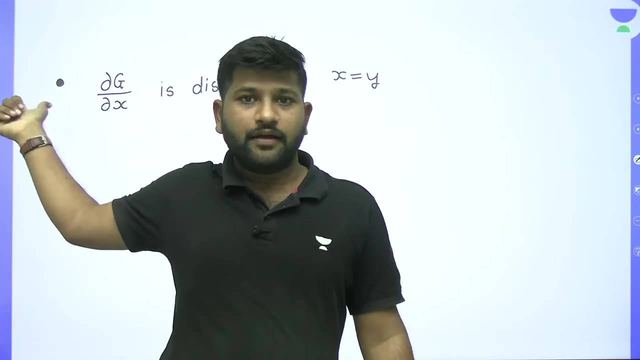 It is discontinuous. Where At x is equal to y, At x is equal to y. At x is equal to y, Your differentiation will be discontinuous. at x is equal to y. What does discontinuous mean? There will be amount of discontinuity. 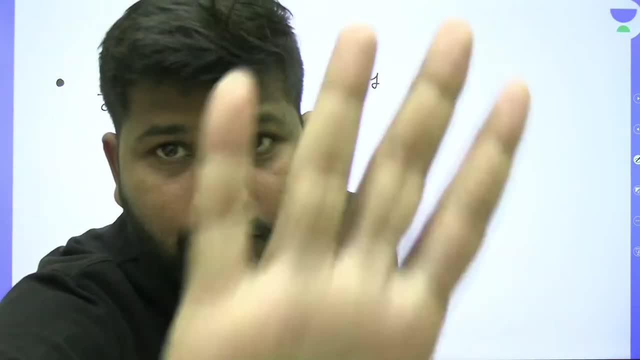 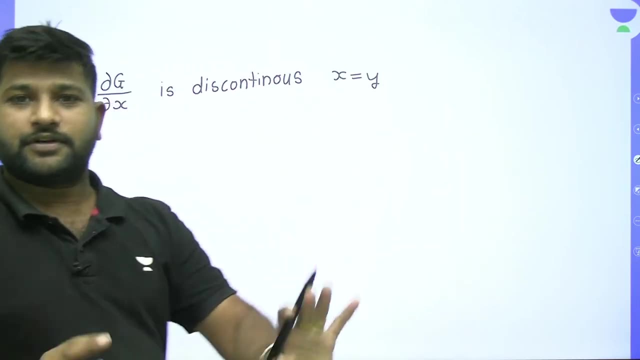 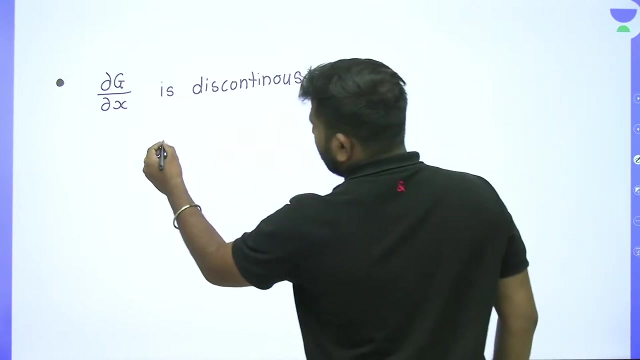 What does function? discontinuity mean There will be amount of discontinuity, And what should be that amount of discontinuity? That is the most important question, Isn't it? So the amount of discontinuity is That amount of discontinuity, And 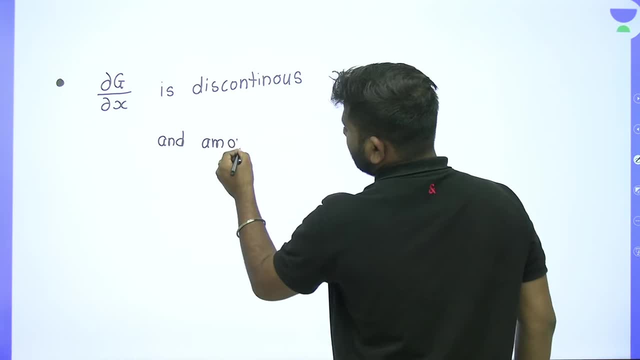 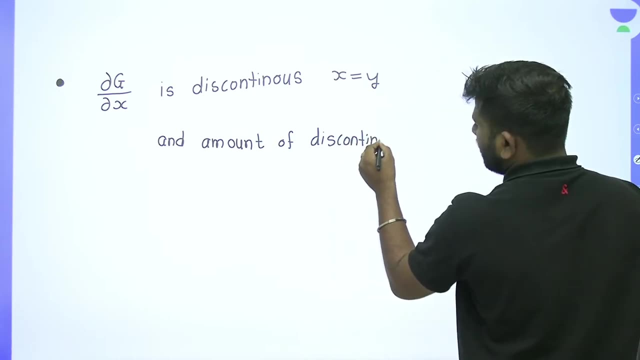 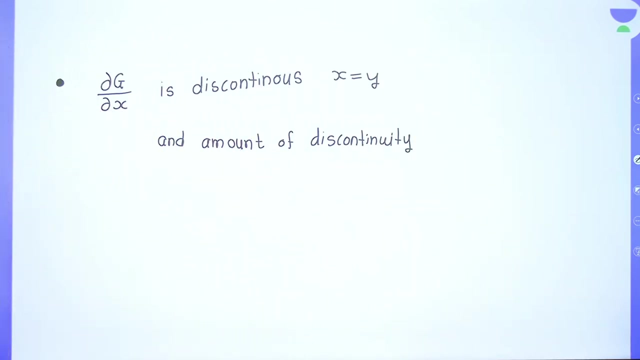 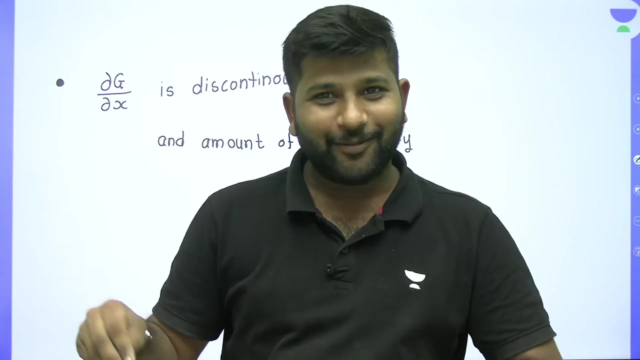 And Amount of discontinuity. Amount of discontinuity: What is the amount of discontinuity: RHS minus LHS? Did I tell you, Yes, we are going to solve the problem with the property itself, Isn't it Because the next problem will be solved with the property itself? 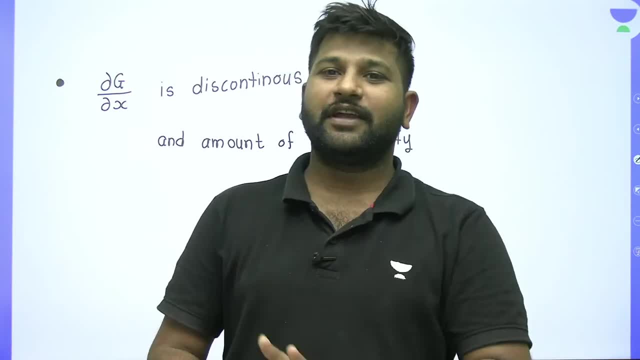 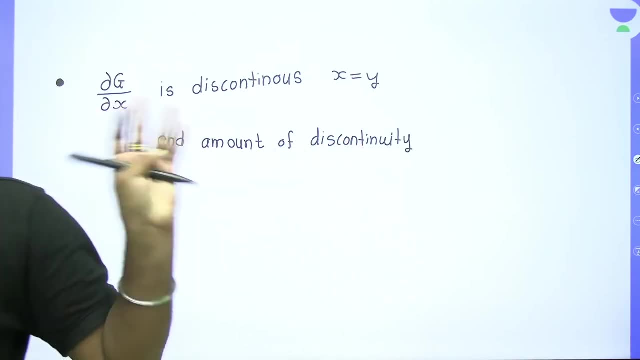 Because if we follow the proper method, then it will take a very long time. We are going to solve it with the property. also, Just be patient. First understand the property. I will discuss, Don't worry about this. Okay, Okay. 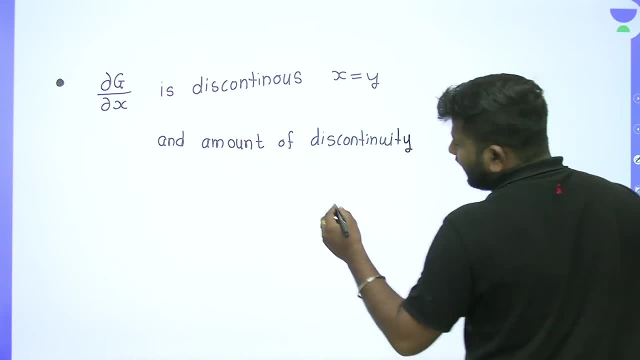 So see here What is the amount of discontinuity? Amount of discontinuity means what? Right hand limit minus left hand limit, Don't you know? Limit Like you have this Right. Let's say this is x is equal to zero. 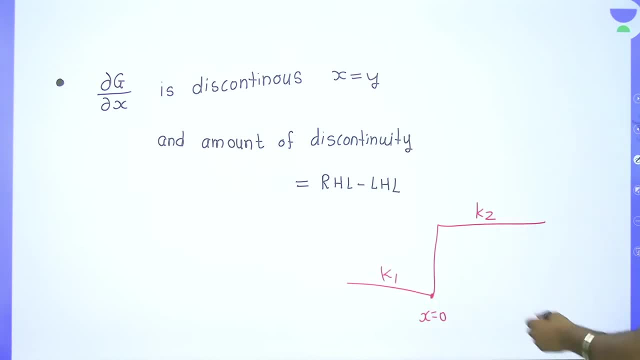 So let's say here is k1 and here is k2.. So here your discontinuity is: x is equal to zero. So what is the amount of discontinuity? k2 minus k1. This is called the amount of discontinuity. So here also the amount of discontinuity will be the amount of discontinuity when you take the first derivative of the Green's function. 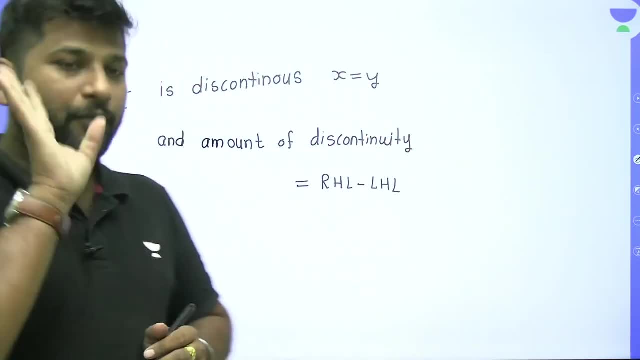 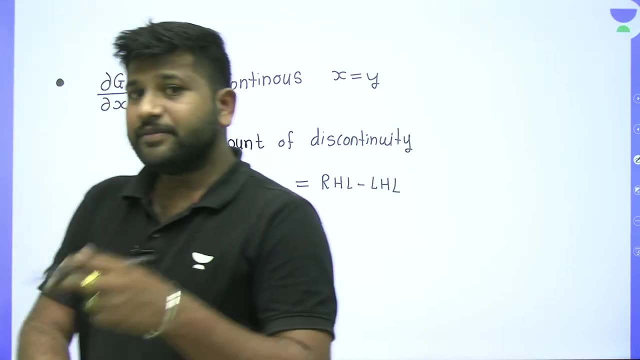 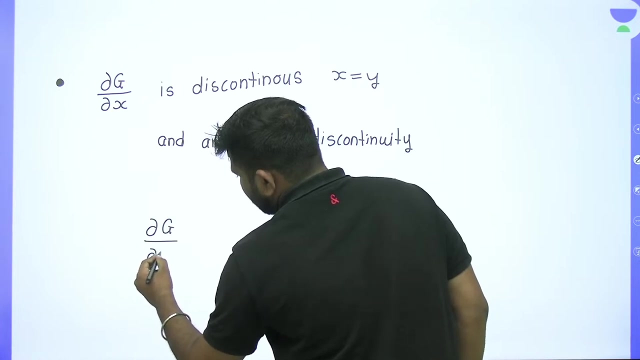 And that amount of discontinuity is the amount of discontinuity RLH minus LHS. Is it correct or not? Okay, That means what? What is the meaning of this? So see here. So that means this: del g by del x. 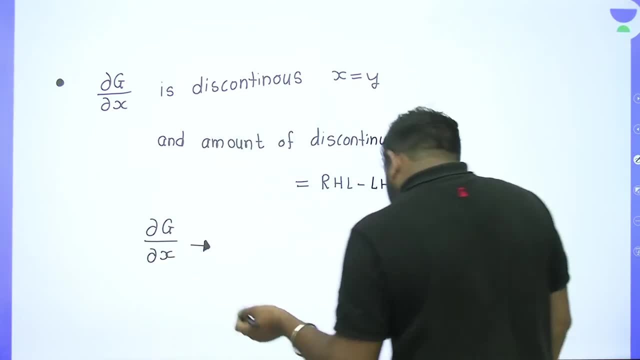 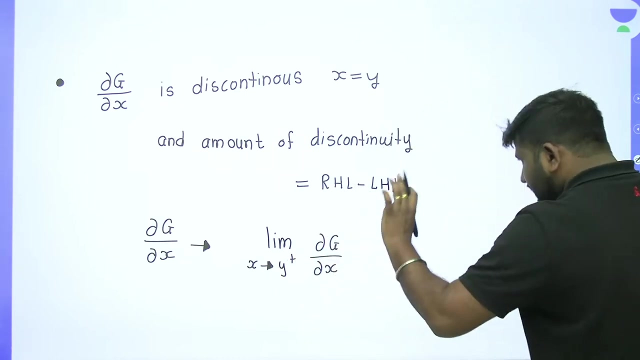 This is the amount of discontinuity. This amount of discontinuity, What does it mean? See That limit x tends to y, plus Right Del g by del x. Amount of discontinuity: This is what is called Right hand limit minus. 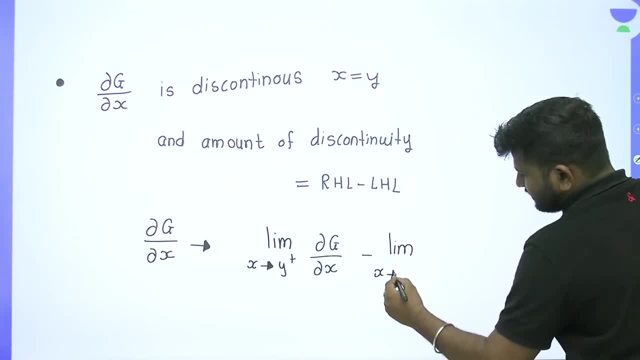 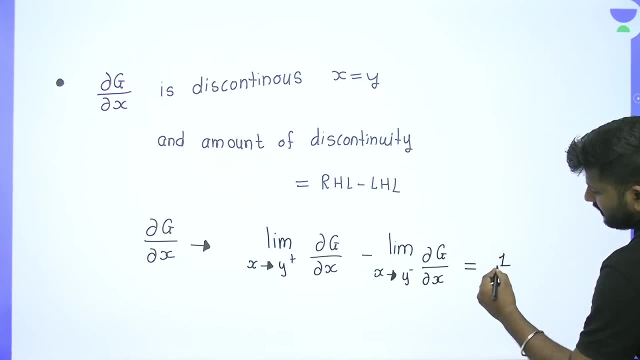 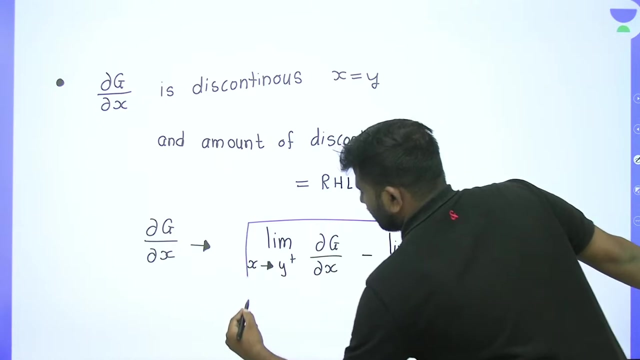 Limit x tends to y minus Del g. by del x, This should be 1 divided by alpha 2 of x. What should be Alpha 2 of x. This should be the amount of discontinuity And In CSIR. 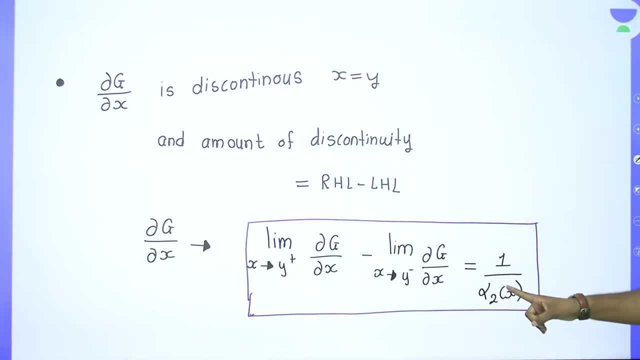 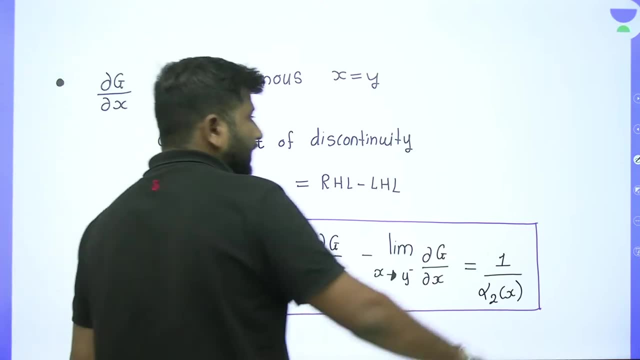 In CSIR You always This alpha 2 of x. This always gives you 1.. All the questions of the previous year They have. This is your differential equation. This is the coefficient of this. You have always given 1.. 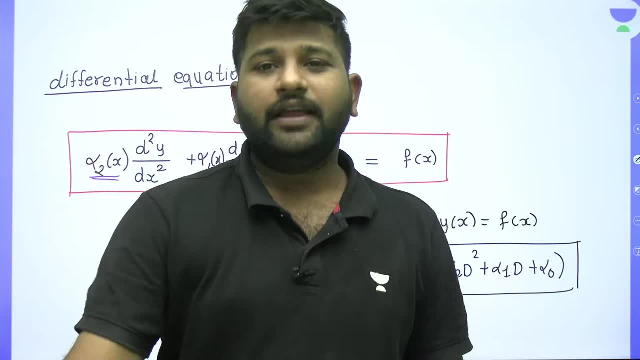 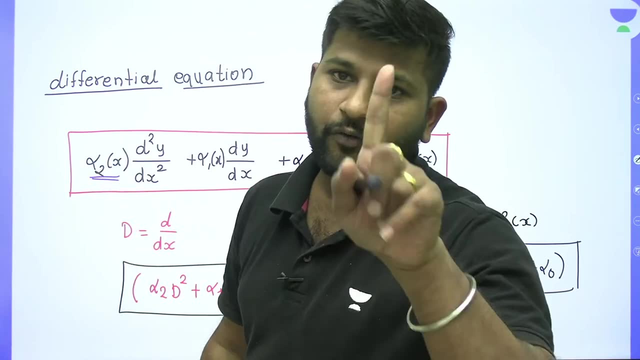 But this will always be 1.. It is not like that It can be anything. You have in every CSIR, This alpha 2 of x. This has given you 1.. But it is not like that. This will always be 1.. 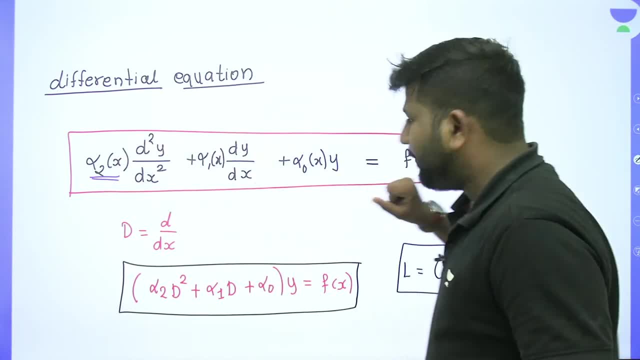 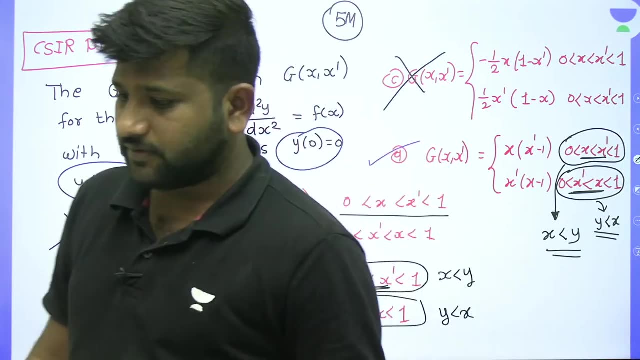 No, Now here it will always be 1.. Now, this property, This property, You solve for this. This is for option D, Four of the four properties, Which is It will satisfy. We will also discuss about it First. look at this. 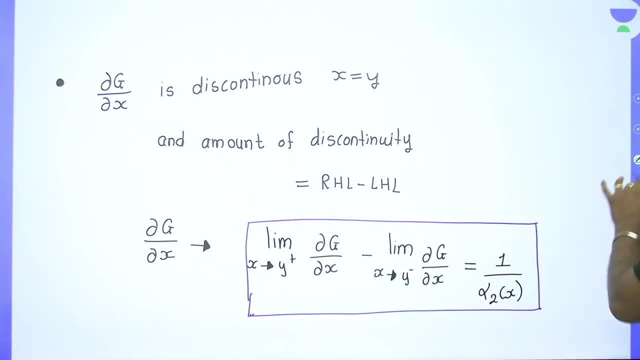 This is the amount of discontinuity. So many times What does it give you That in CSIR Alpha 2 of x, 1 is given. That means Amount of discontinuity. What is this amount of discontinuity? 1.. 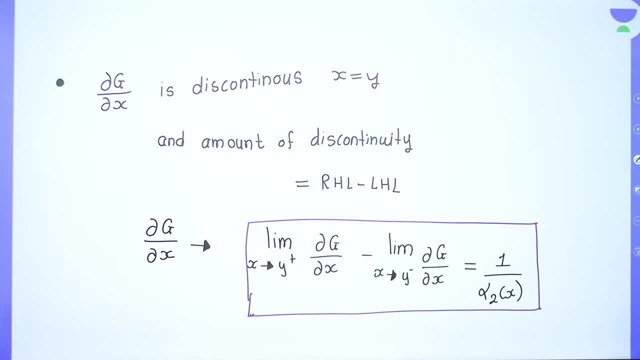 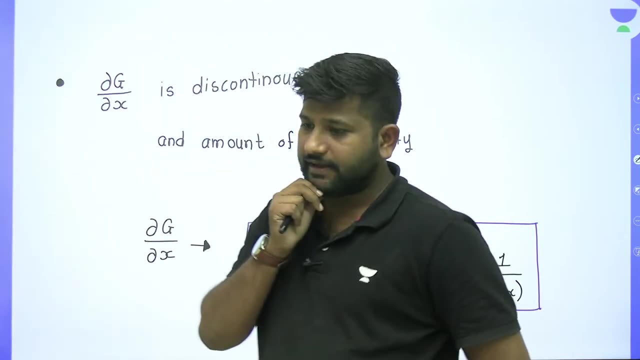 Got it My thing. How will you solve this? 1. Ok, 2. How find it? 3. Where is this? 4. 2. What is this? 5.? What is this? 6. 7.? 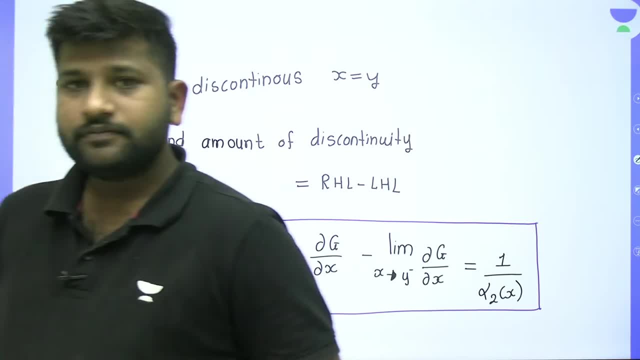 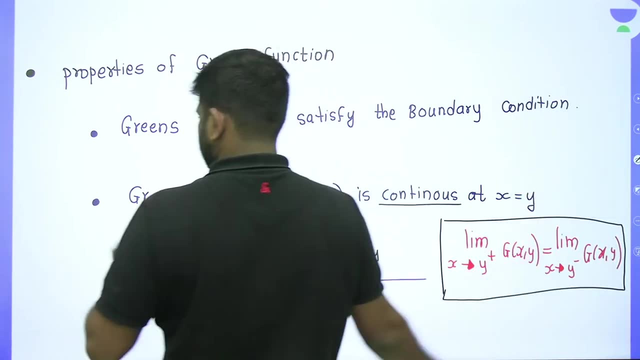 Ok, There is 8.. There is 8.. Ok, I will tell you If you understand this all, If you understand, If you understand, So Only that, Okay, So How will you solve this? Ok, Property is very important. 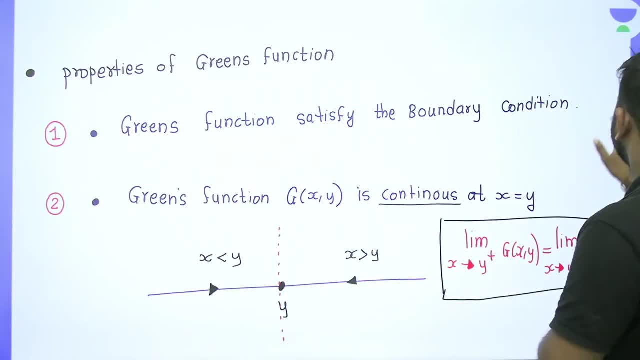 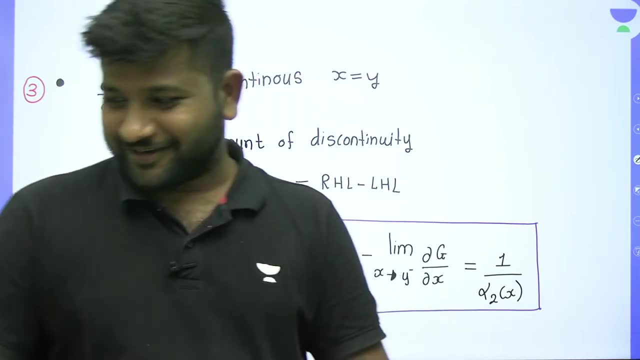 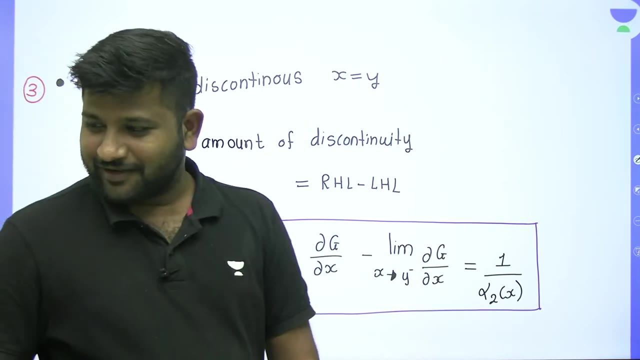 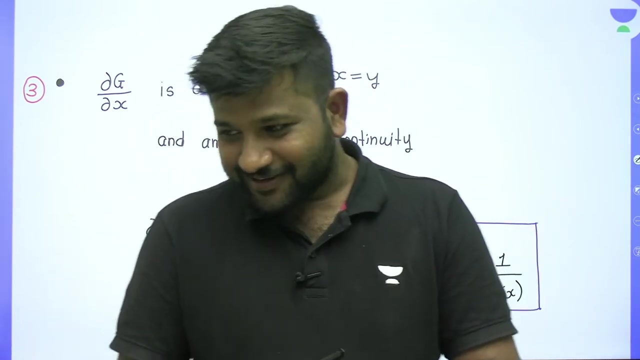 Isn't it? This is second. This is third, Isn't it? Property is very important, No matter what it is, Isn't it? Isn't it? If it comes after marriage, then it is also needed for that, Isn't it? 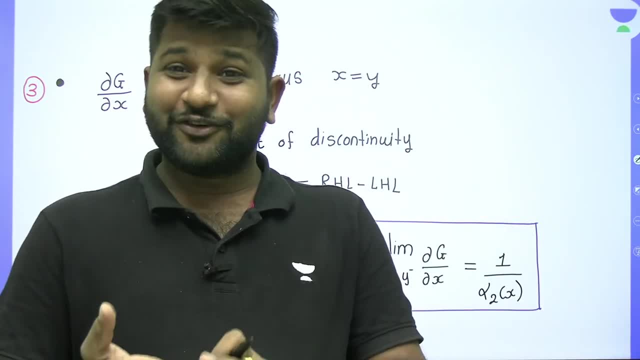 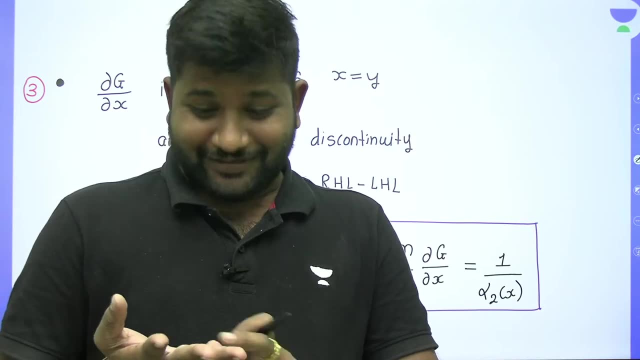 If a girl gets a good husband, then she will get a good husband. What do boys want? They want a good husband, They want a good job, They want a good earner. All these things should be there, Isn't it? 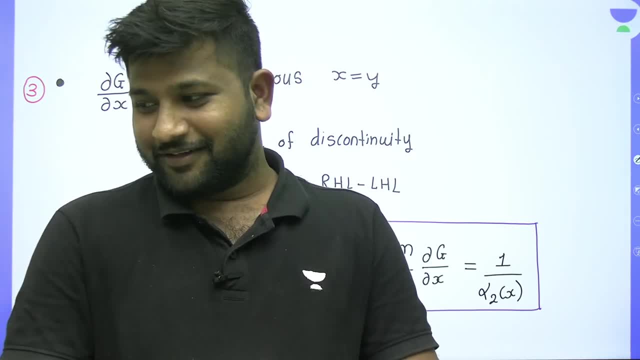 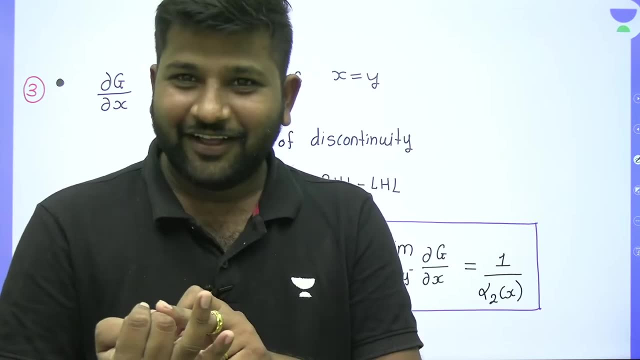 So pay attention to this. This is very important, Isn't it? If we get a good husband, then we will not get a good wife. We will not get a good husband, We will not get a good wife. We want a good job. 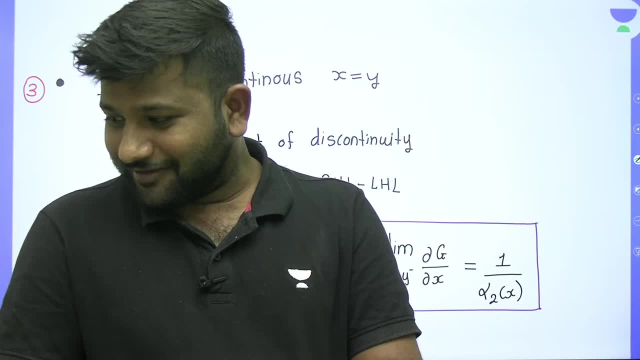 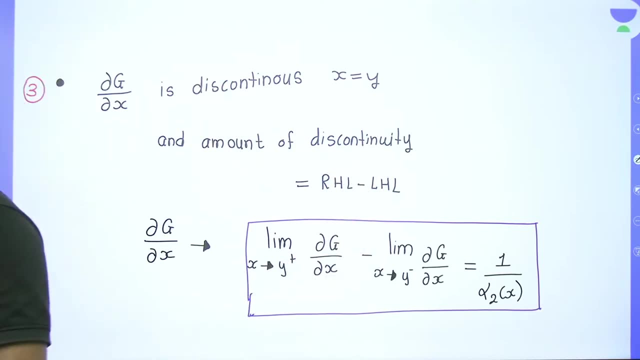 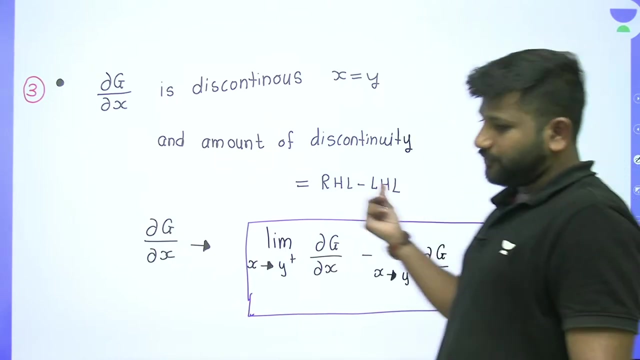 We want a good job, We want this, So property is very important. If you know property, then all these things are possible. Come on, I hope you understood this. I hope you understood this. These are the properties. These are the properties. 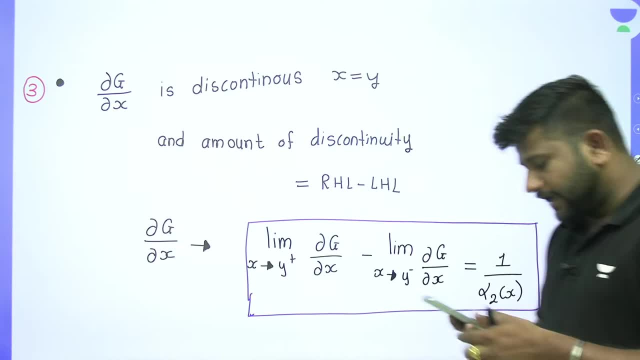 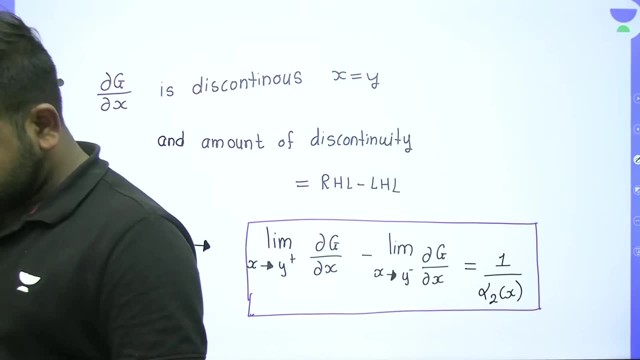 So let's solve this question on this property. Let's solve this question on this property. Let's take the question of CSIR So that you get a good idea of this property. So that you get a good idea of this property. 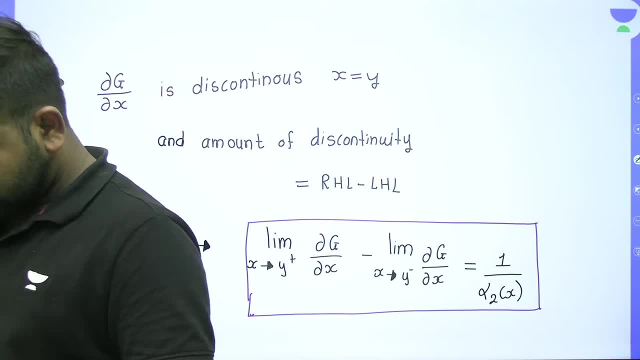 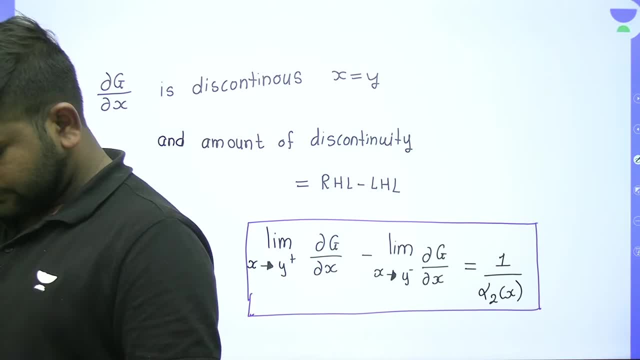 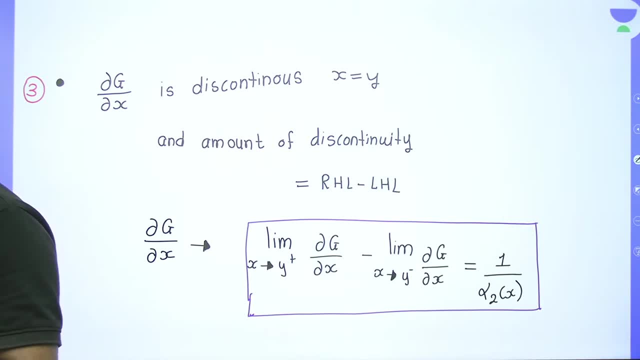 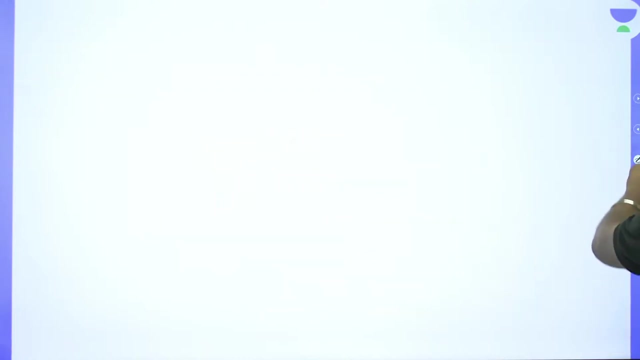 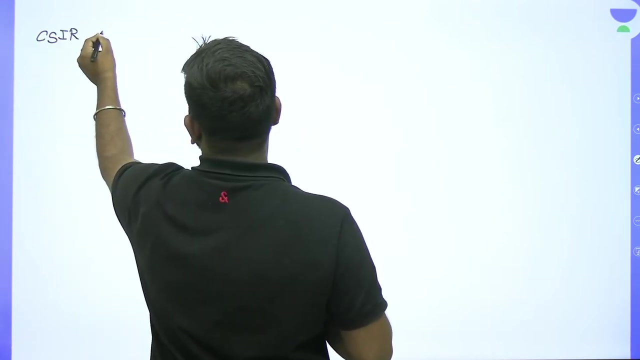 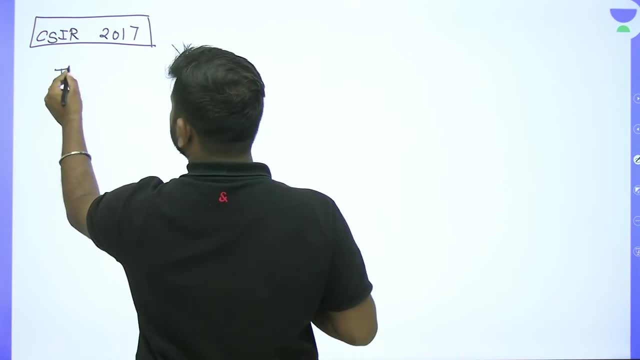 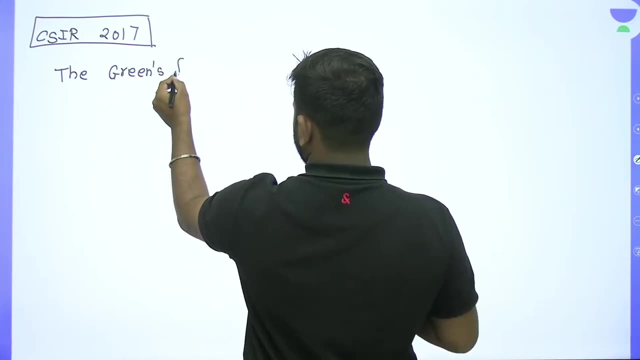 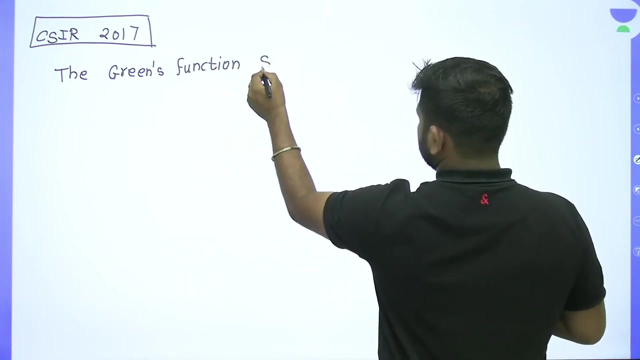 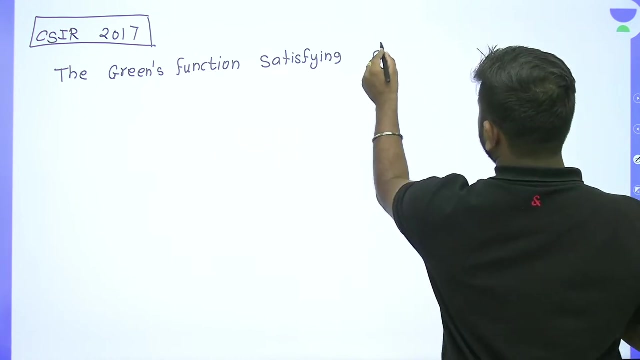 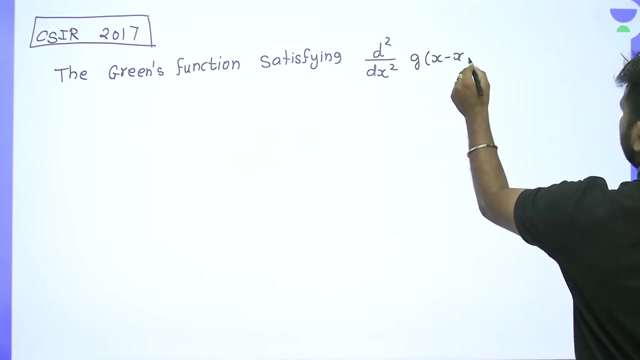 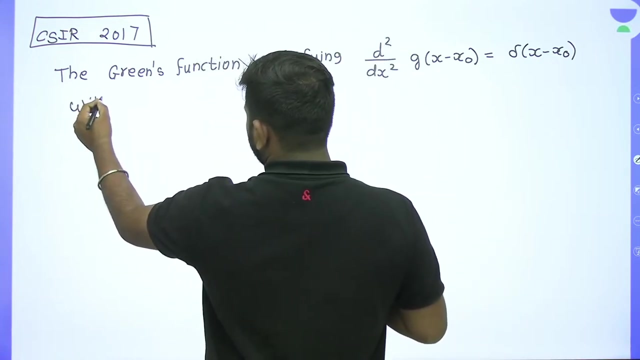 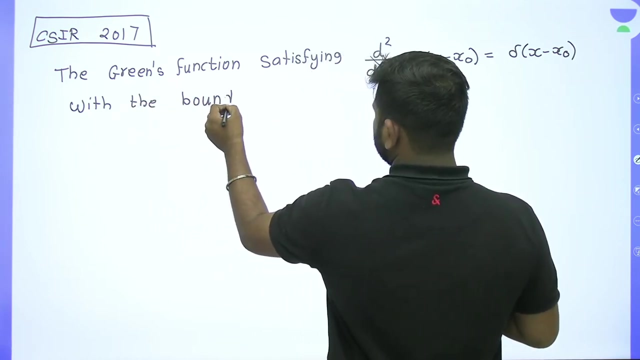 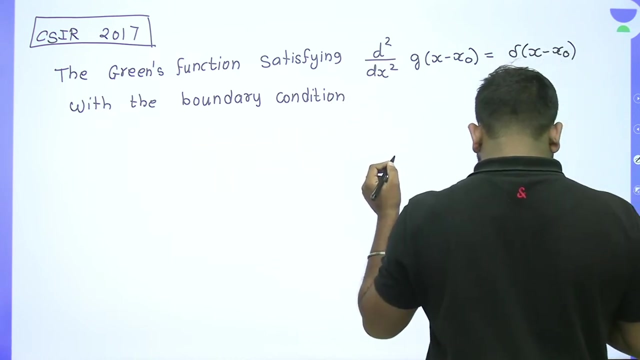 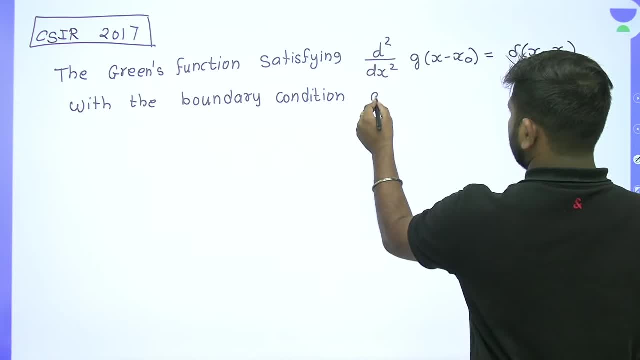 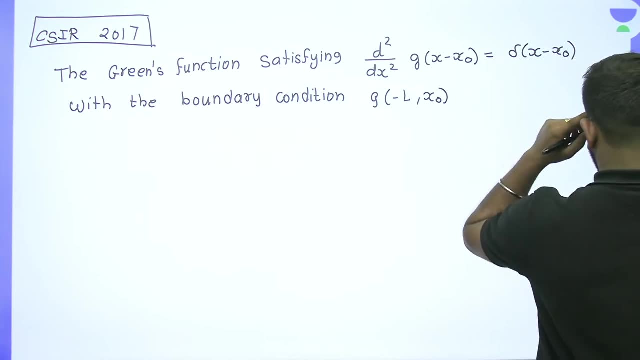 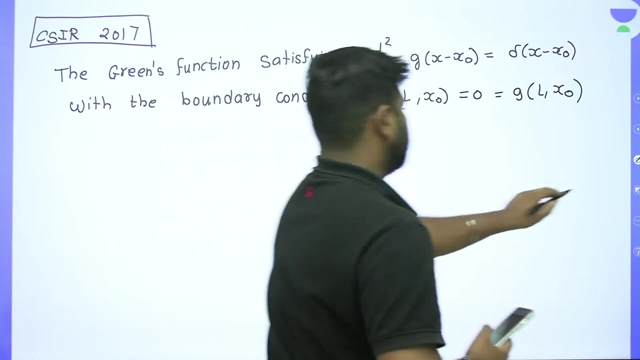 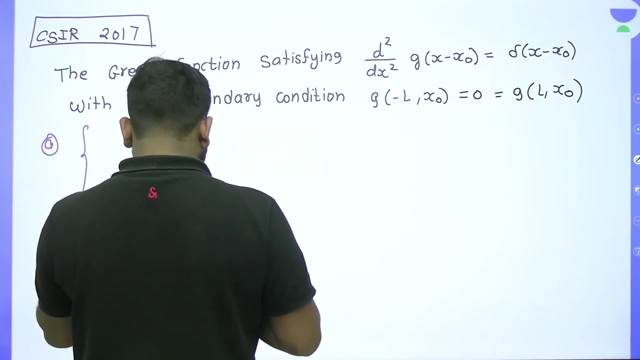 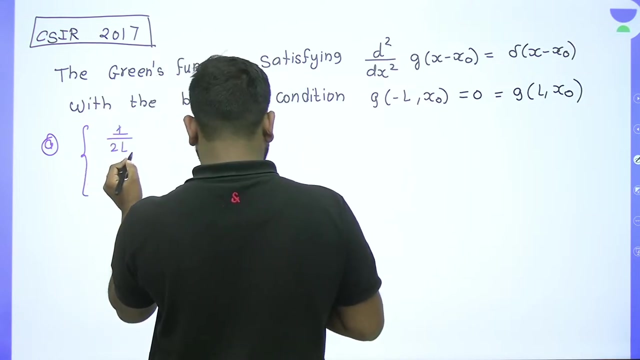 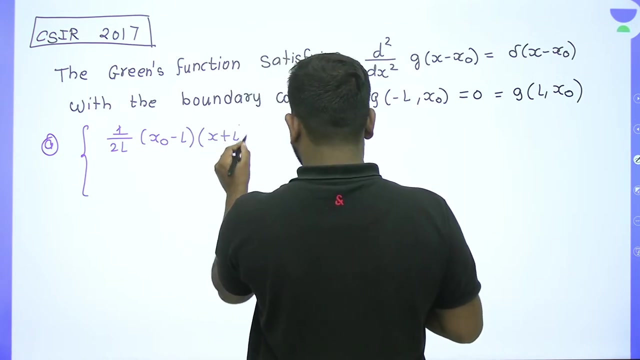 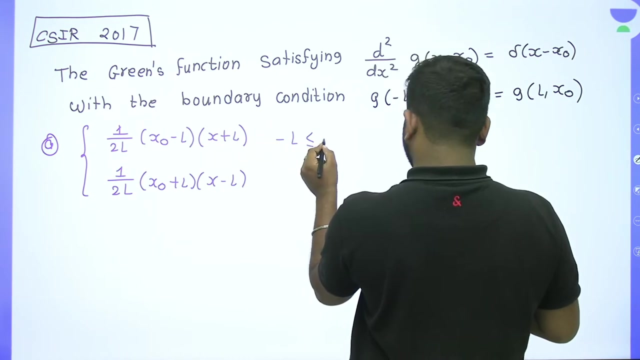 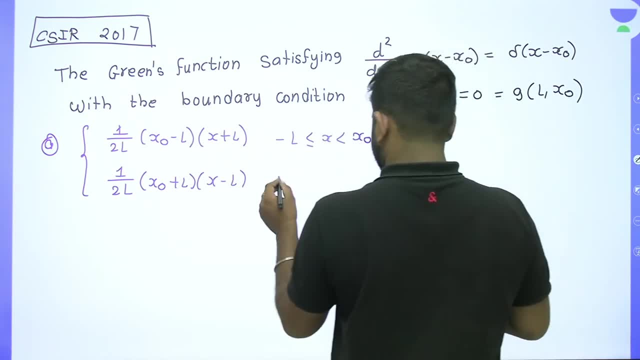 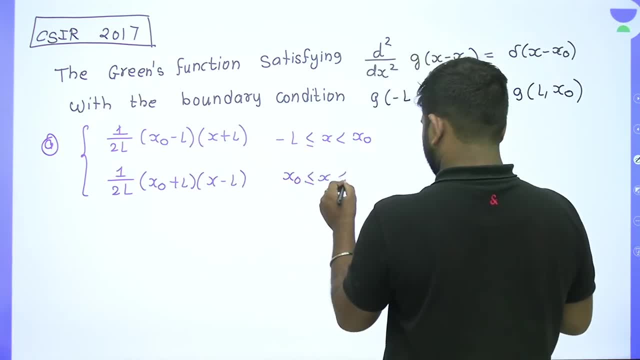 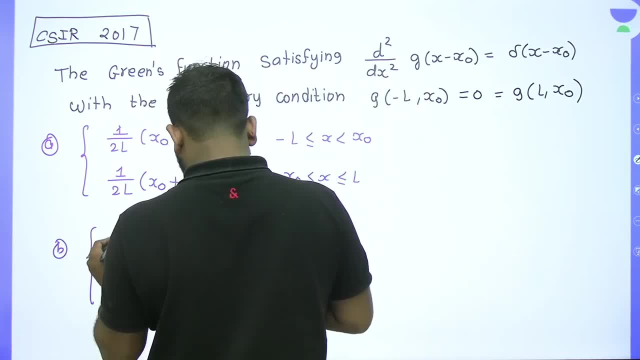 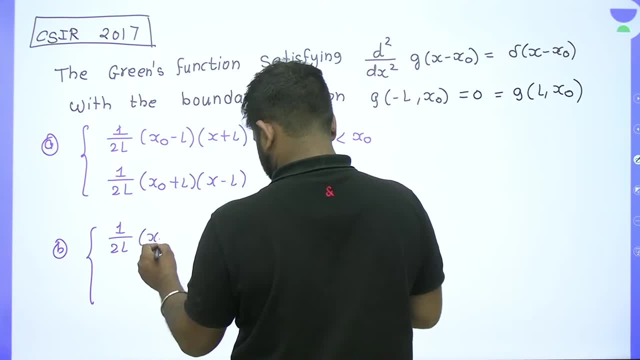 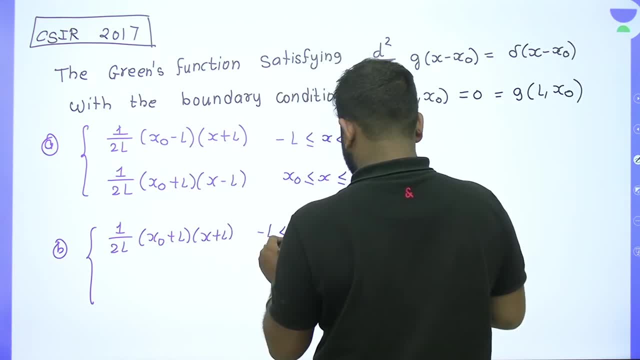 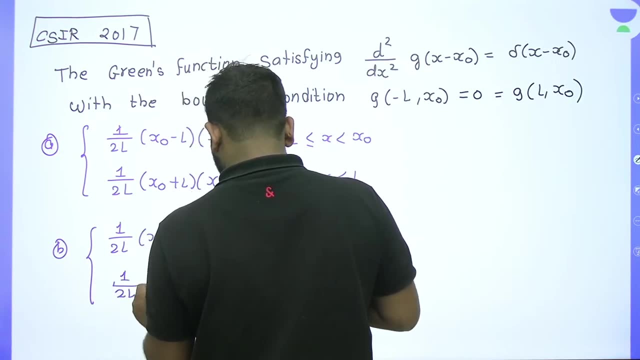 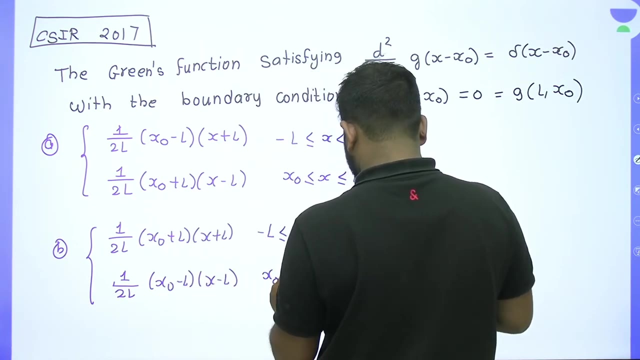 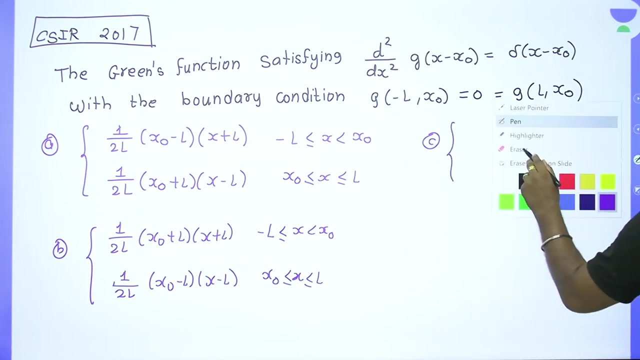 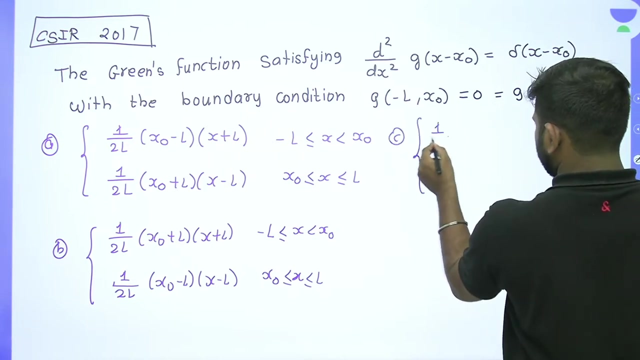 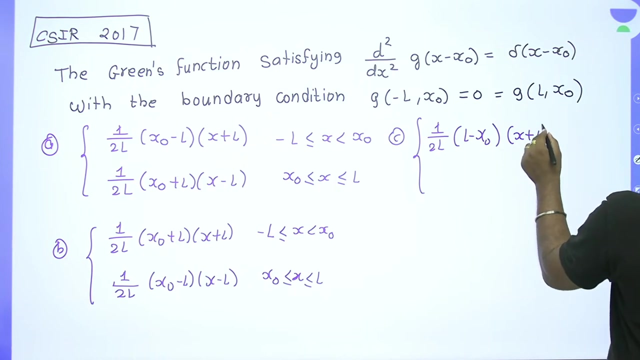 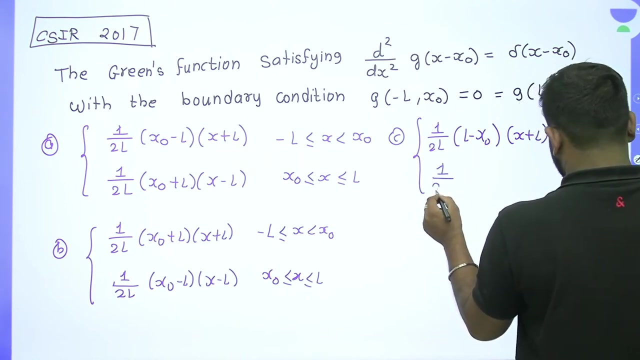 which video is 17 or 18,, I don't know. let's see: minus l x x naught 1 divided by 2 l. it's not minus l x minus l x naught. option b: option c: 1 divided by 2. l l minus x naught x plus l. minus l x x naught 1 divided by 2 l. 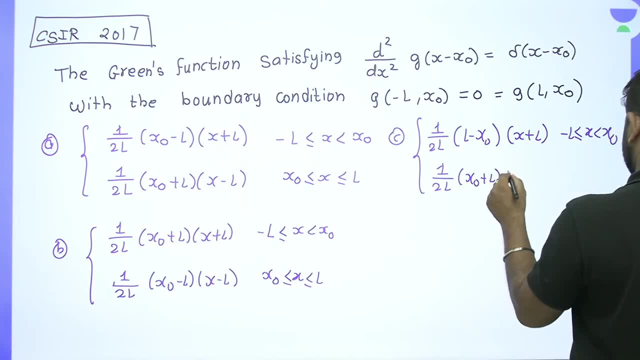 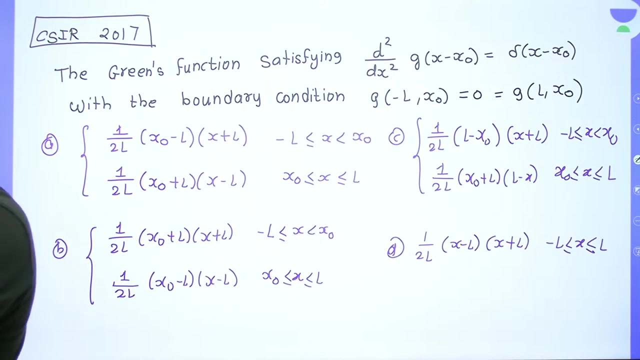 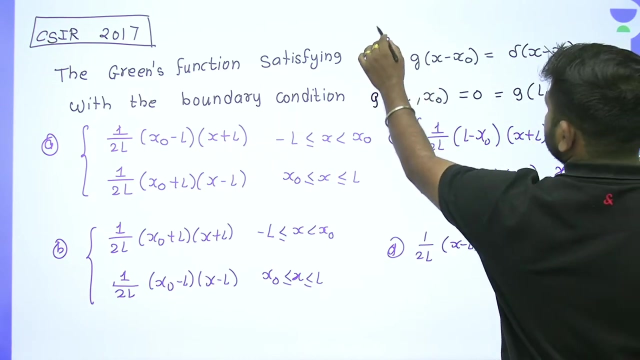 x naught plus l l minus x x naught x l and option d: 1 upon 2: l x minus l x plus l minus l x l. so what is the solution for this question? any idea? so this is the thing, but look, this is L. 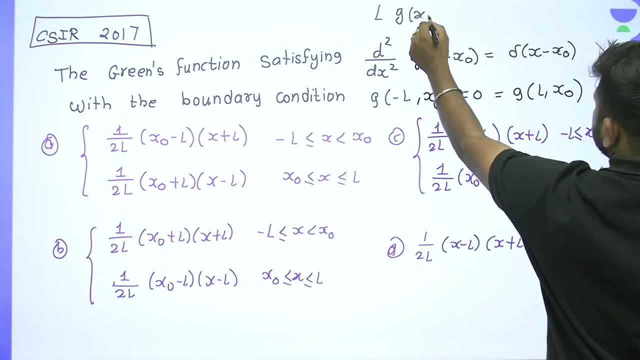 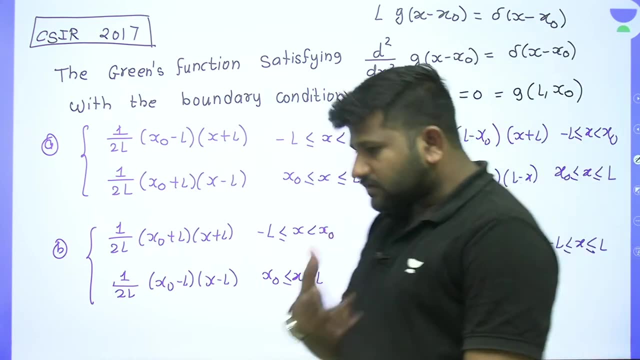 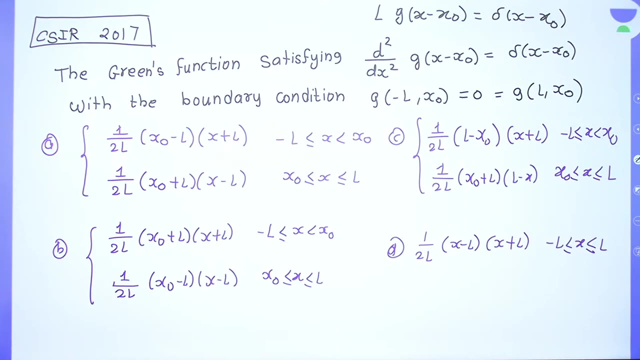 L and G of X minus X naught is equal to direct delta: X minus X naught. just Y is called G. that's it, ok. what will be its solution? ok, so what is its solution? wait, this is direct delta. so wait, this is direct delta. so this is L. 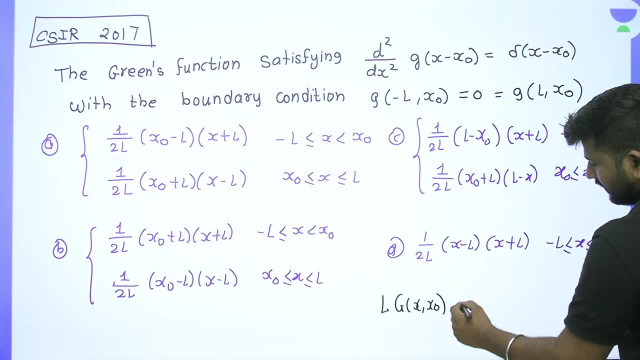 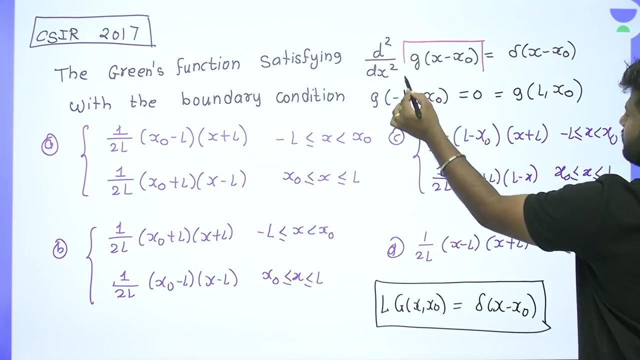 G of X, X naught is equal to direct delta: X minus X naught. ok, so this is direct delta. ok, that means here the Green's function, this Green's function is your E, this is your Green's function, and here the value given to you, this value given to you, is their. 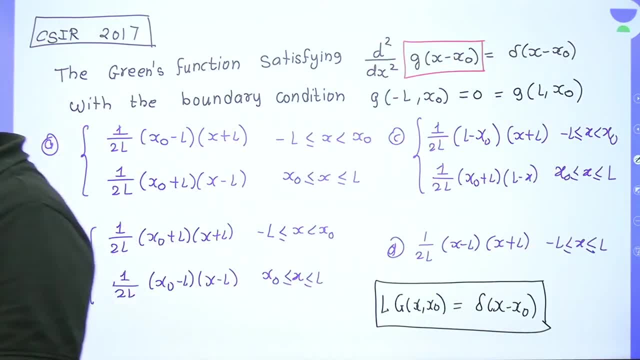 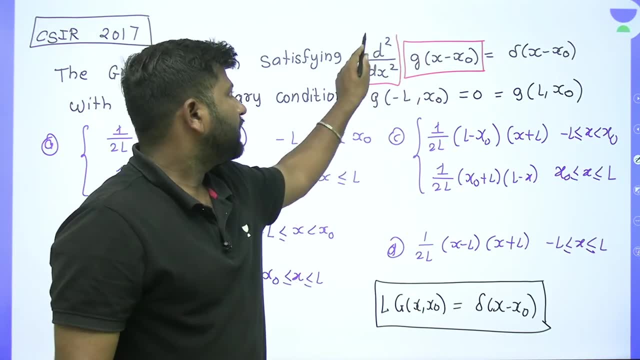 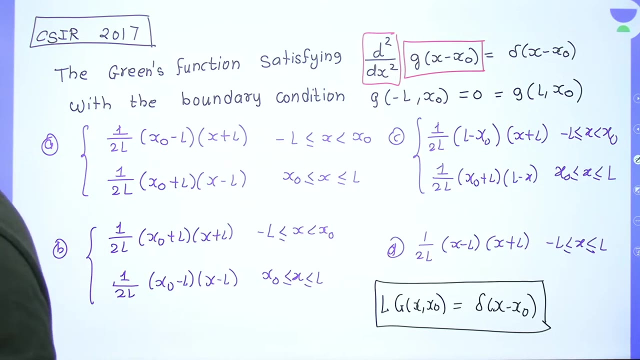 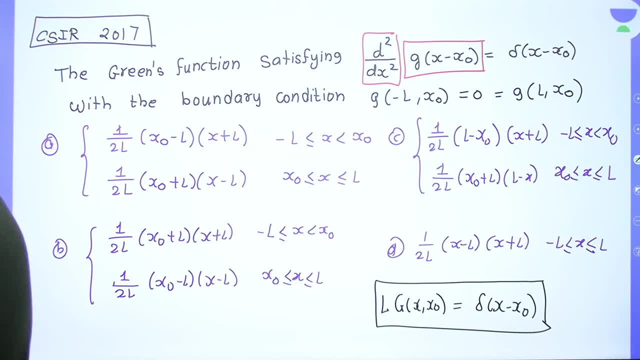 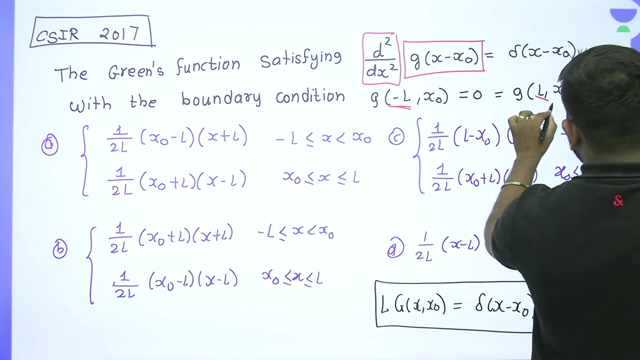 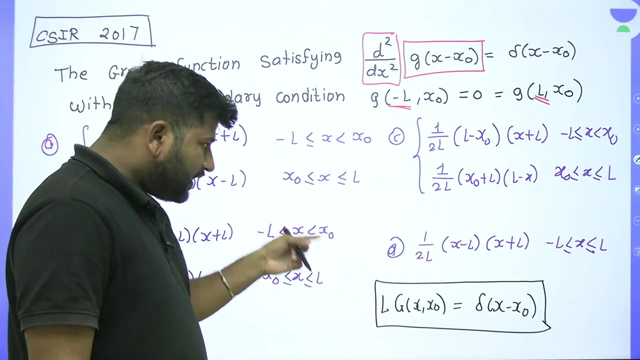 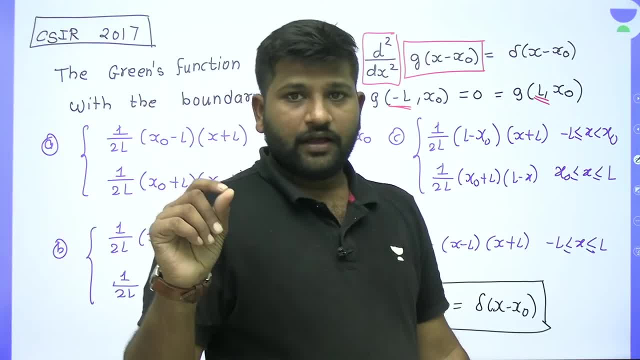 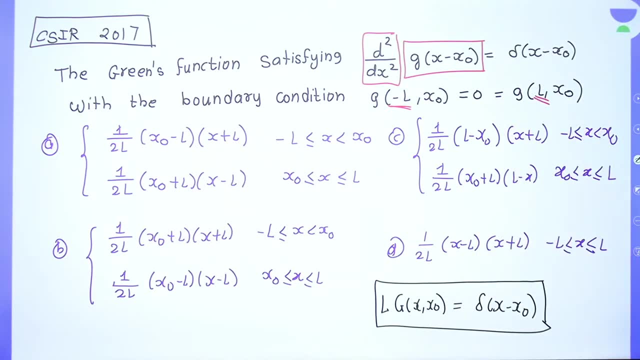 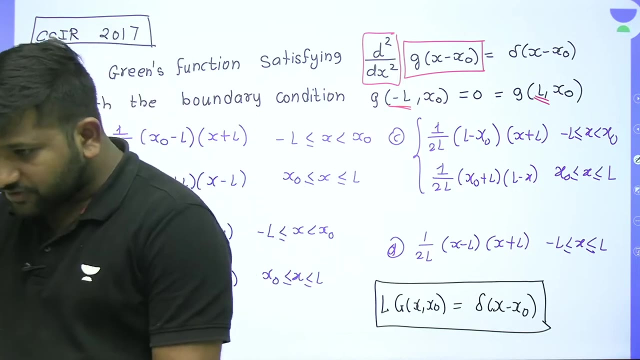 what is this Green's function and what are the properties of the Green's function? so the Green's function, this Green's function property, this Green's function, it should be continuous means. their limit should exist as limit, their limit should exist as limit. so let's check this. 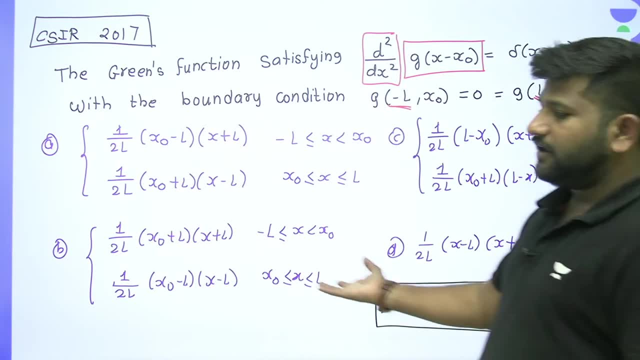 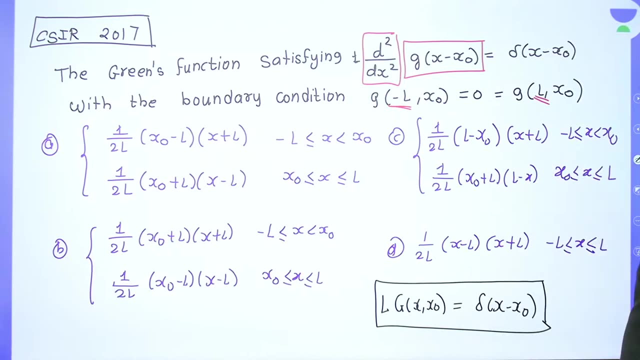 that how? now they have to check that whose limit is existing and whose is not. and now you can see here that this Green's function is L. what is its coefficient? it is simple: 1, so the amount of discontinuity will be 1, that's it. 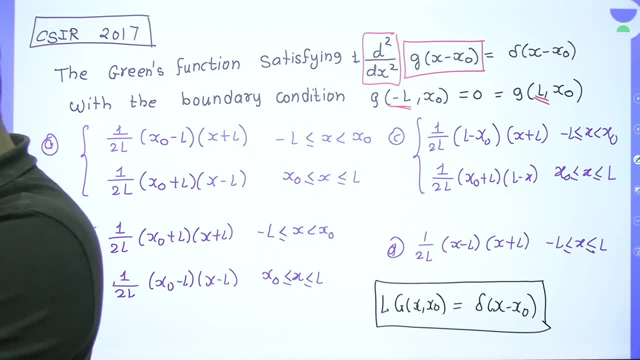 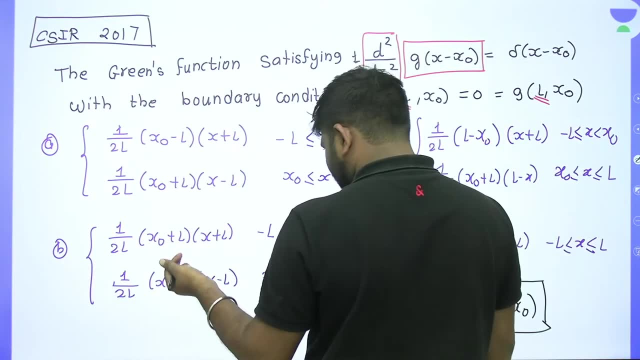 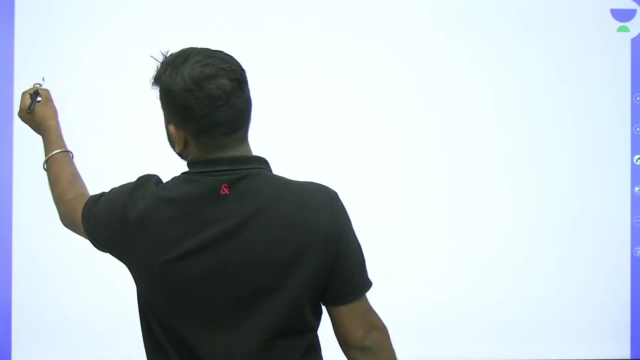 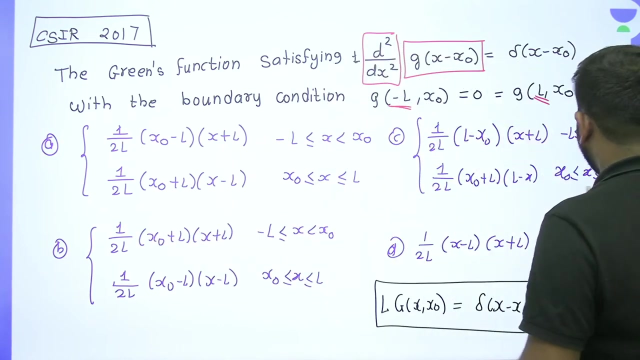 ok, ok, ok. so now let's say: its option is A and option A is correct, so let's take option B. means for: to explain, let's check second option, let's talk about second option. because option A is correct. so here it is ok. now see here: 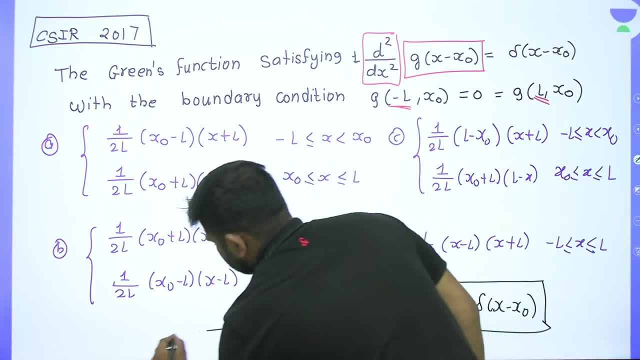 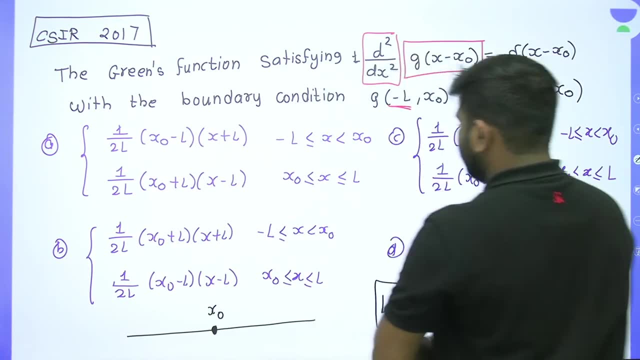 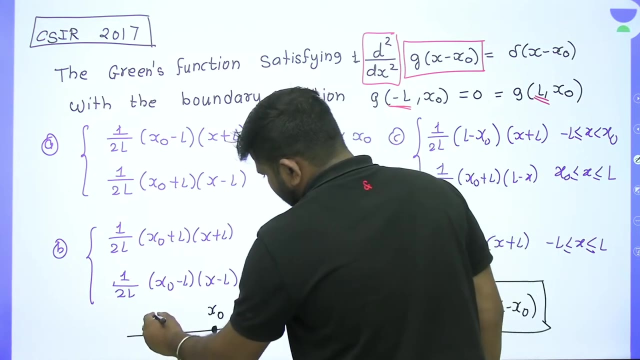 that this is your, this is the thing, this is your. let's say: this is your X naught, this is your X naught, ok, and we have to approach this. we have to approach this X naught so we can approach like this and like this. here is minus L. 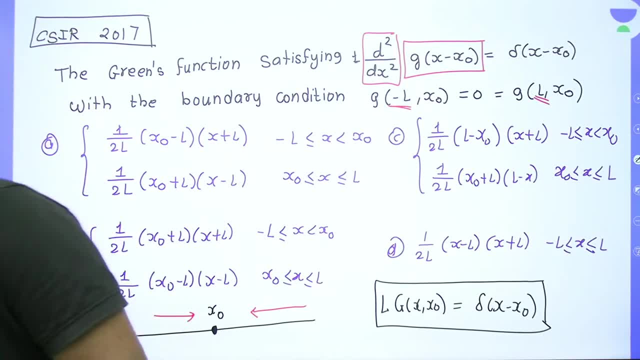 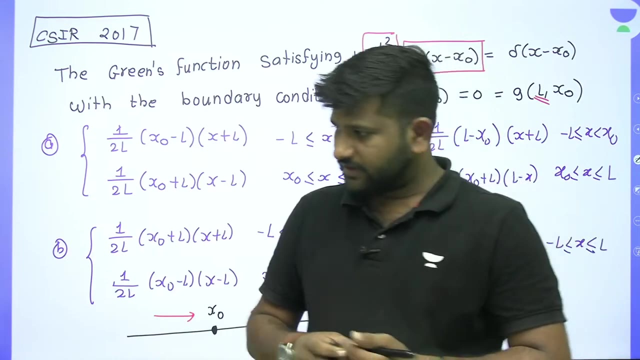 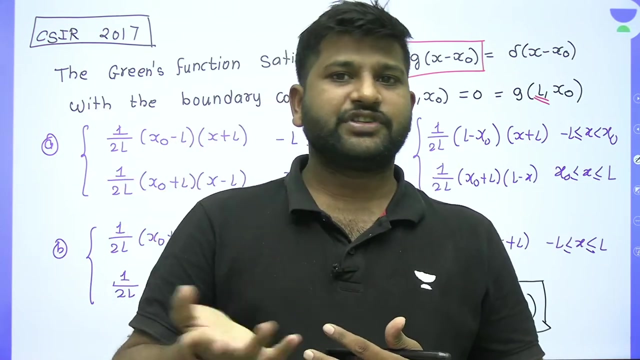 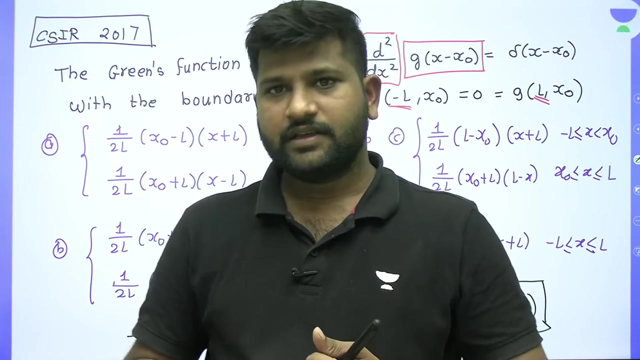 here is plus L, right. so here you ok, Mr Udesh Mishra. full mathematical means mathematics. hmm, numerical analysis is taught, in which interpolation, extrapolation, extrapolation. this is saved. Euler's method is also saved, so he didn't take it because you have, so that is saved. 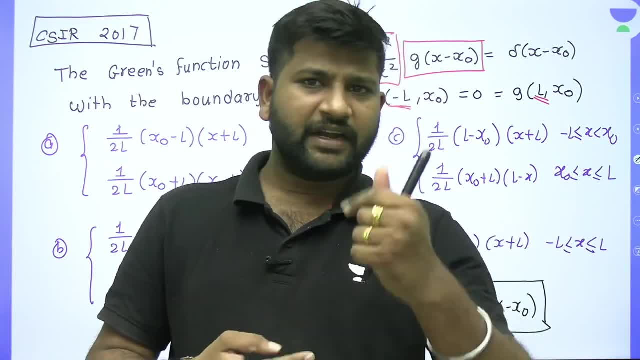 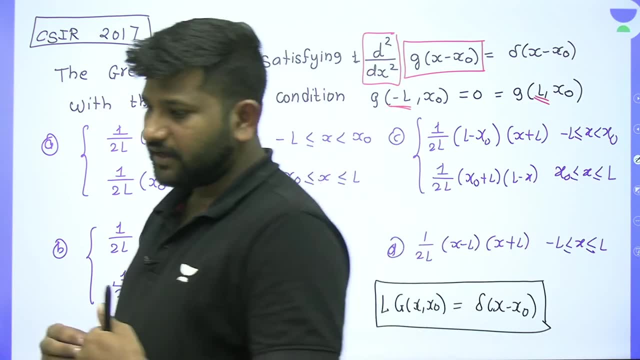 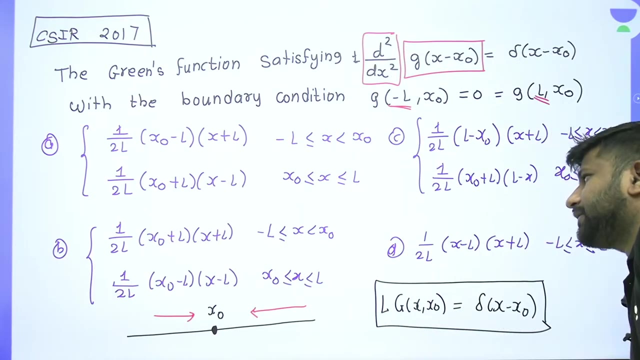 but I will take later on in mathematics matrix, which is special in classes, complete matrix, complete complex analysis. also I have taken in special class. ok, ok, let's move ahead. ok, let's move ahead, ok, ok, ok, ok, ok, ok, ok, good, ok, so you are opting b. 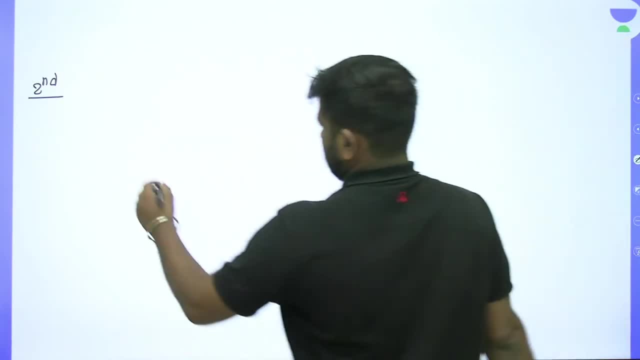 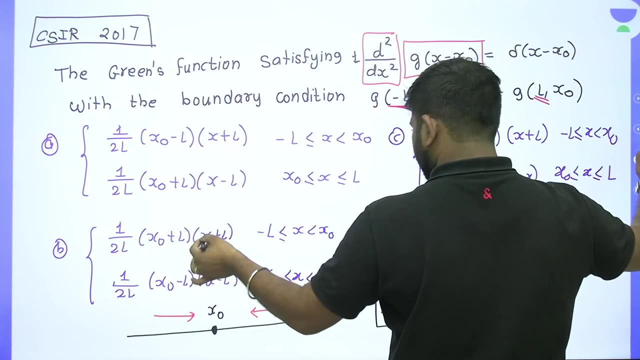 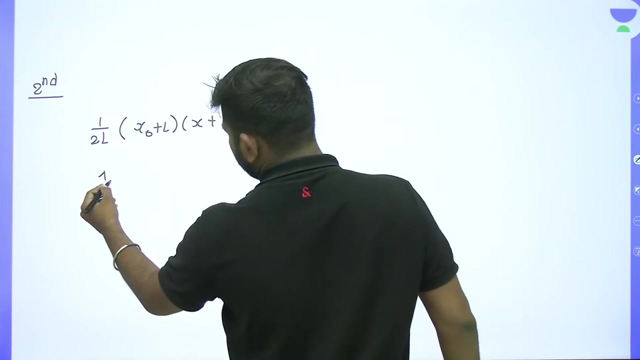 option b or option b. you see what is option b: 1 upon 2 L, so this is the one upon two L into this what is X naught plus L, X plus L and one upon two L by x naught minus l, x minus l. 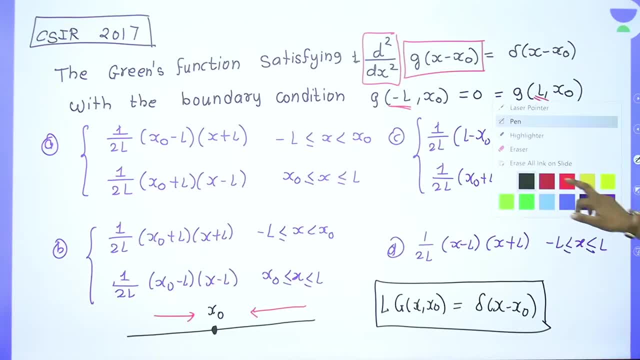 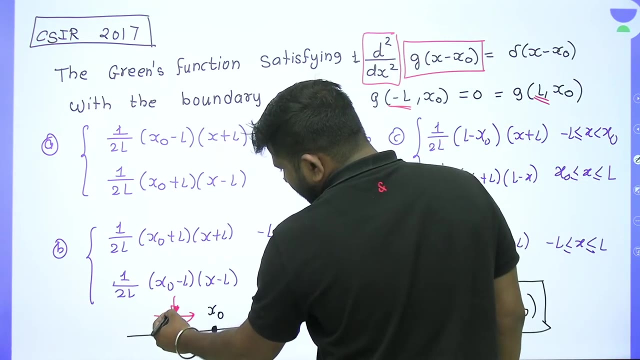 this is so. this is for two reasons, if you see here. so this is x less than x naught. this is x less than x naught. that means x naught is more. so which region is this talking about? this region is talking about understand this region. 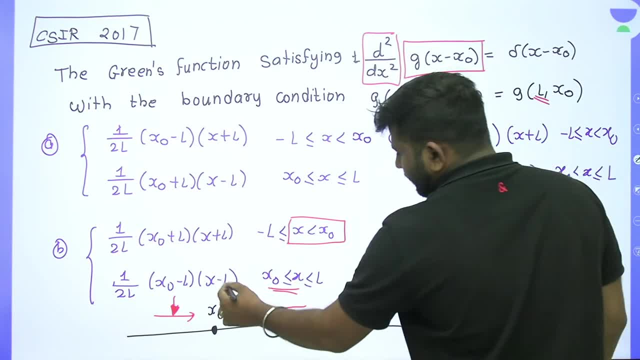 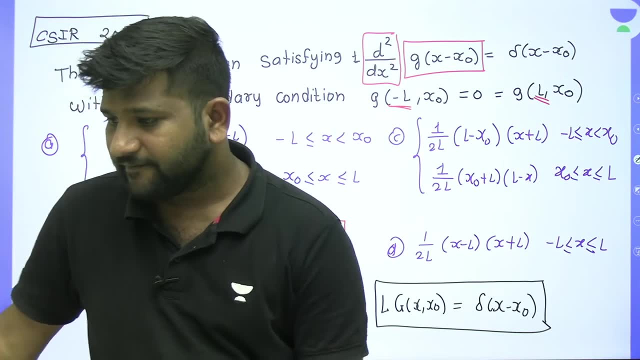 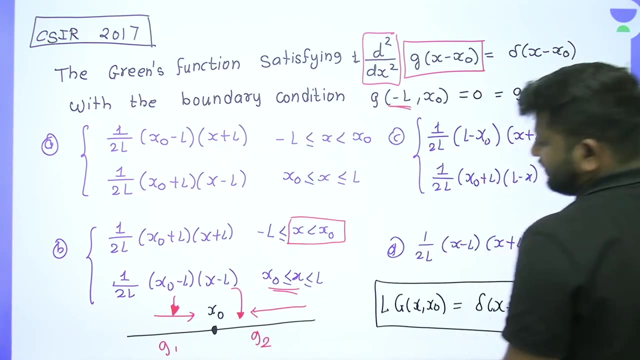 and here, what is this? is this? that means x is big. that means this region is talking about this region. understand this, ok? so this one you will say this is a Green's function in this region- is a g1, and Green's function will be in this region, g2. 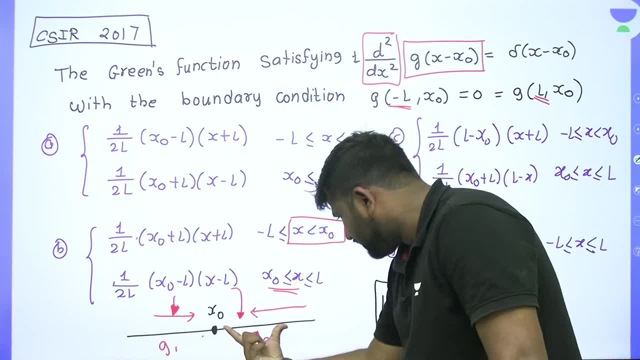 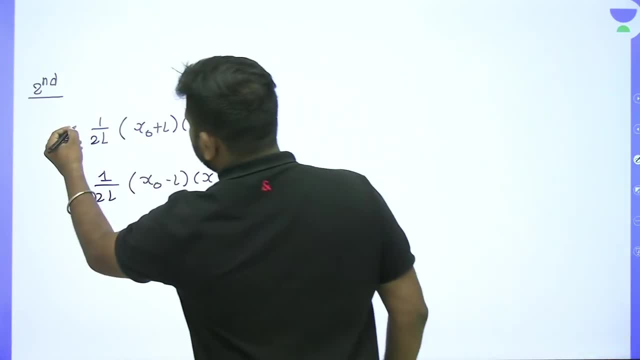 so in this region, Green's function will be this. this region, Green's function will be this. so in the first region, Green's function is so: in the first region, this is your Green's function. and in the second region, first means first in that region, and this is your Green's function in the second region. 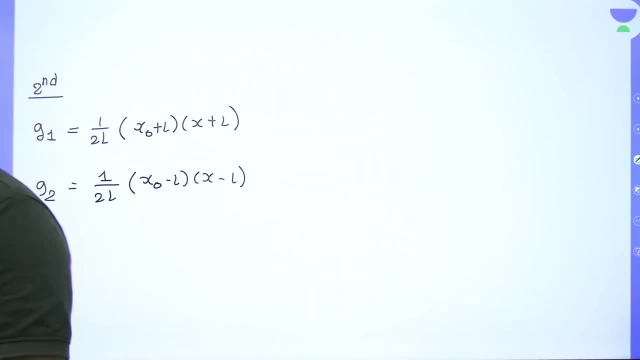 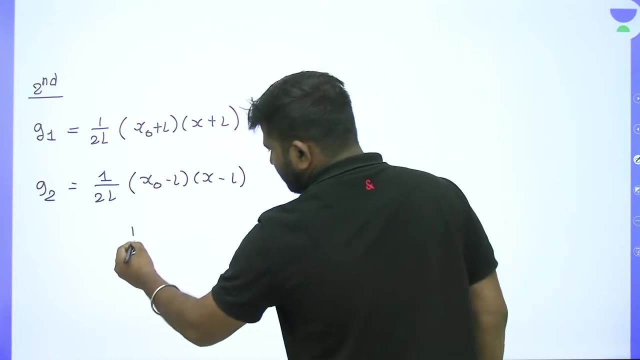 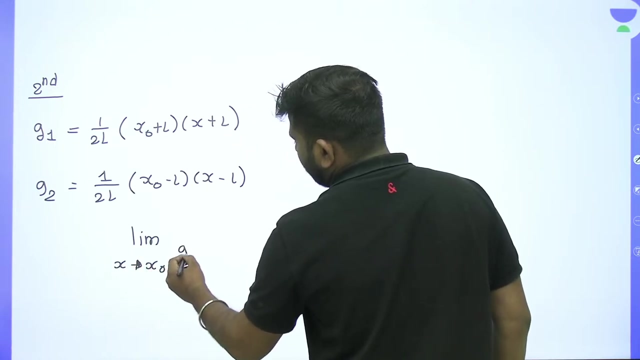 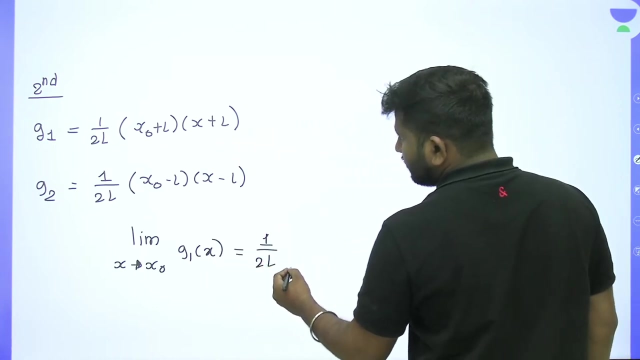 are you understanding what I am saying? ok, isn't it? now see, check its continuity. that means limit. this x tends to x naught. find out g1 of x, which is equal to. so you got 1 divided by 2L. this will be your x naught plus L. 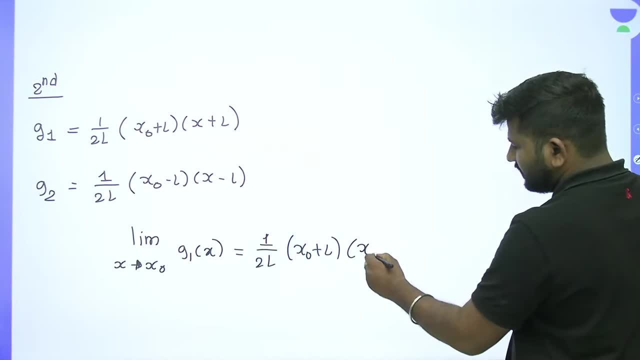 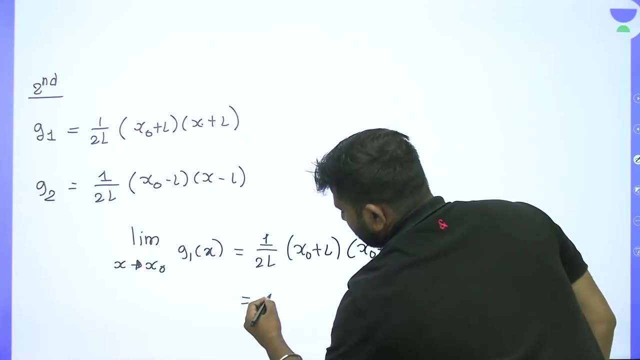 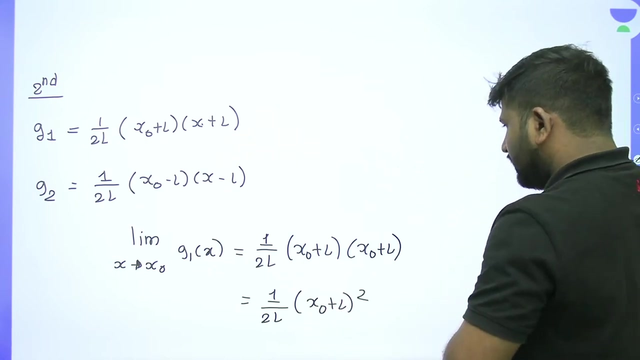 and x tends to x. naught means this will be x naught plus L, isn't it? put x naught in place of x. yes, so which is equal to 1 upon 2L into square of x naught plus L. this will be ok. 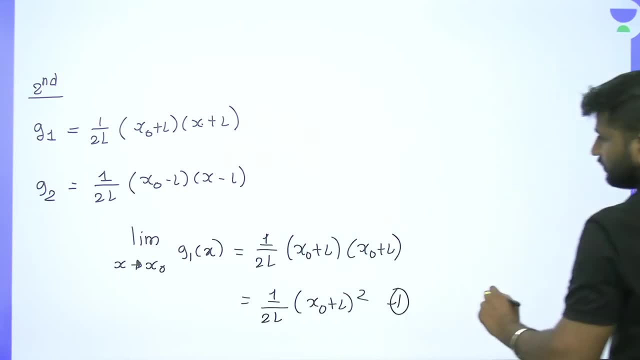 if you see the second, so consider this equation as 1. if you see the second, that limit, x tends to x, x tends to x, naught, isn't it? x tends to x, naught, if you did, that is g2 of x, because limit should exist. 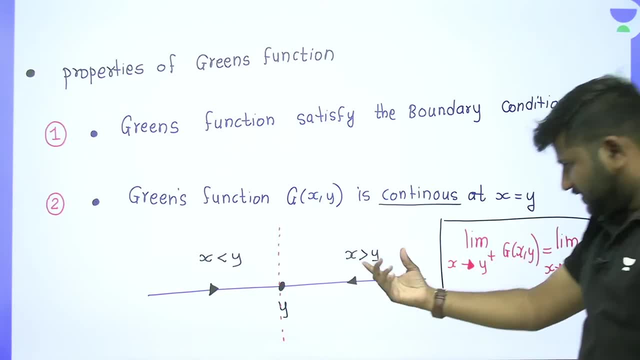 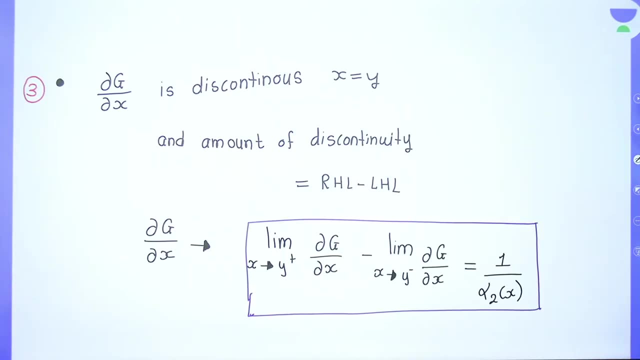 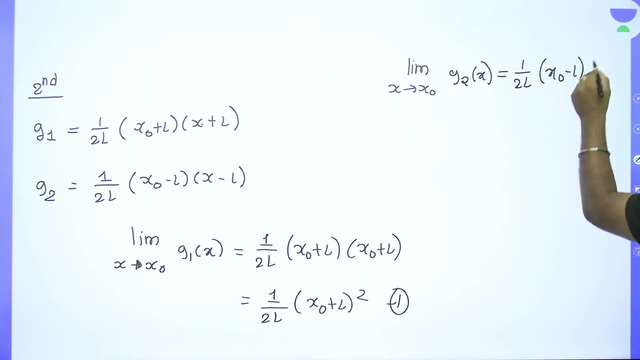 see, I am talking about this property, this, this Green's function, this region's Green's function, this region's Green's function. their limit should exist. so if we are doing this here, then how much will it be? 1 upon 2L in bracket x, naught minus L. 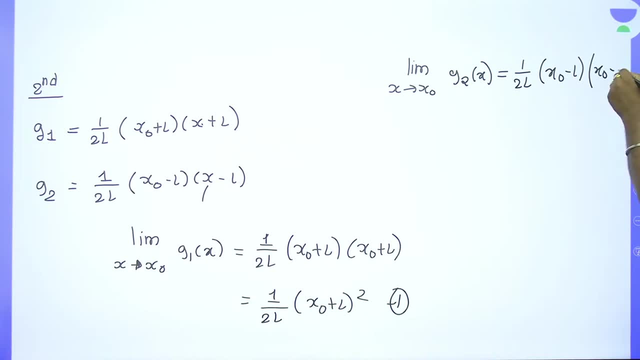 and limit x tends to x naught, so we will put x naught in this and x naught minus L. so from here you can find out that limit x tends to x naught. g2 is equal to how much 1 by 2L? 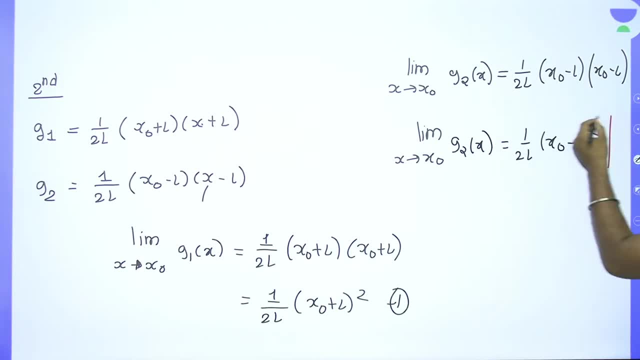 square of x, naught minus L. are these two same? is this two are same? no, here, 1 by 2L is, 2L is x, naught is x naught is. but here is plus, here is minus, here is minus. so this is your option. 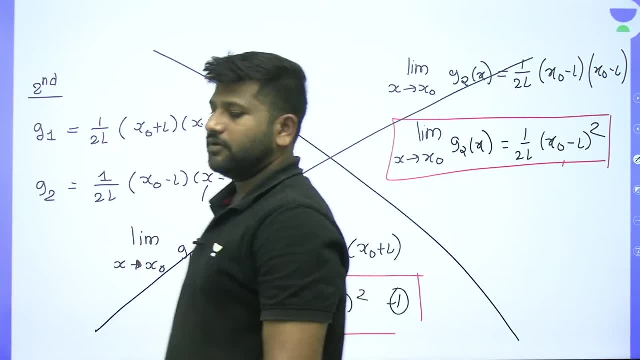 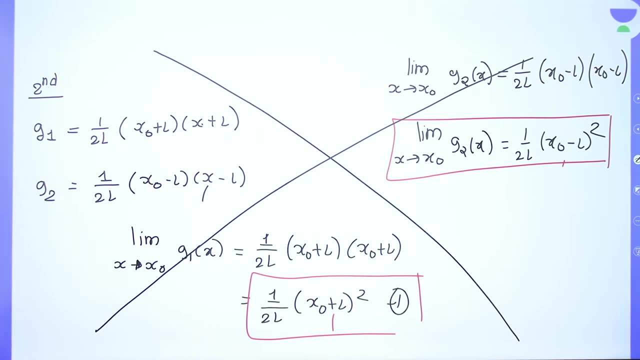 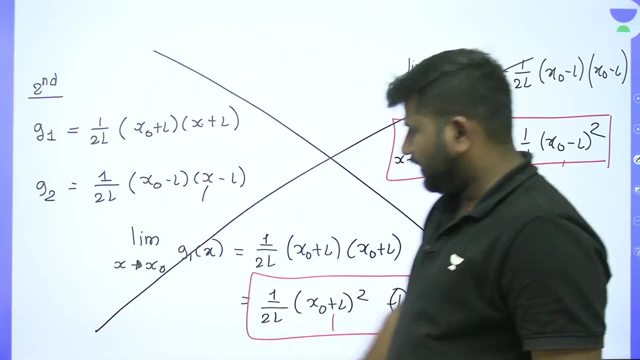 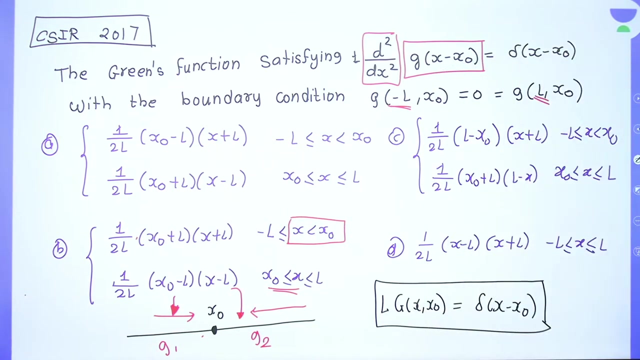 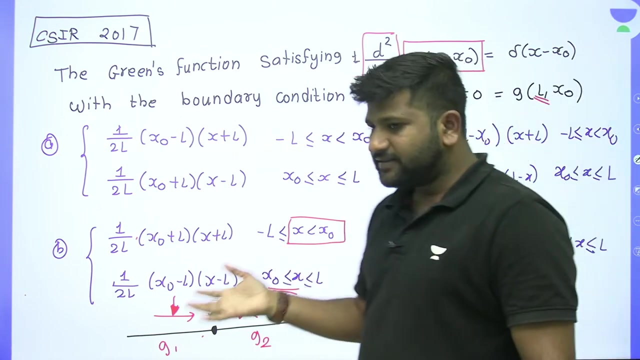 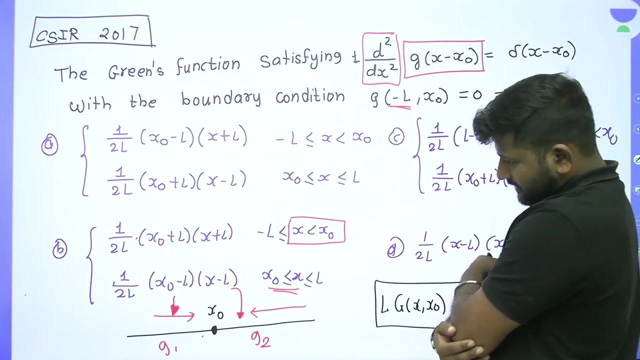 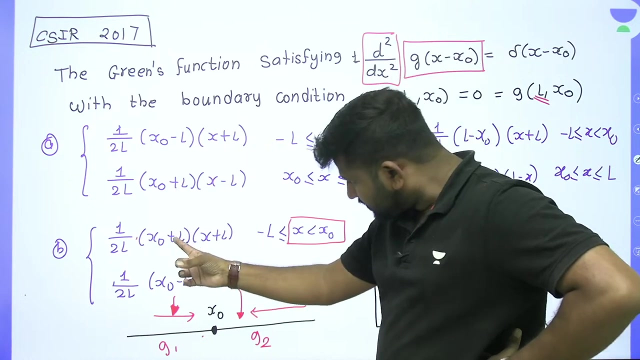 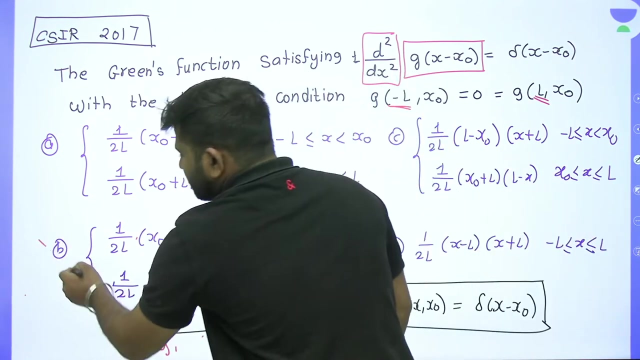 this option is also not correct, understood or not understood or not. ok, I hope you have understood this, ok. ok, by the way, here here you can directly with option. you can do with option check. See, I told you that there is no need to do so much calculation in the exam. see, if I look here, then it is approaching x is equal to x0, so if I put x0 here and put x0 here, then I can see it directly that this x0 plus this will come. this will also come. x0 plus this will come. this x0 minus this will come. this x0 minus this will come. I cut it from here, it did not happen. 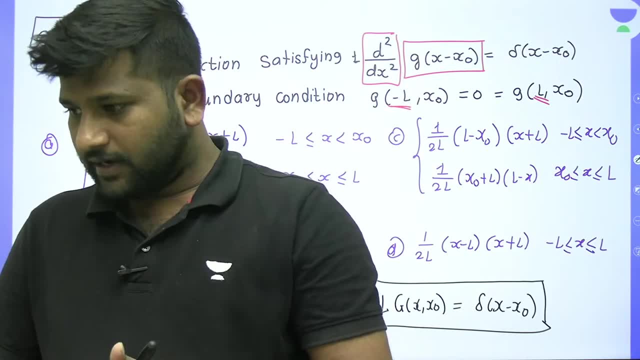 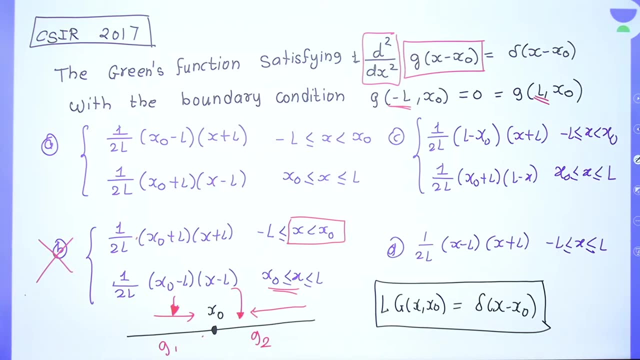 I hope you understood this. If you look at it in this, it is the same here. then put x0 here, put x0 here, put x0 here. okay, so what is happening here In this option? so x plus L, x0 plus L- same is here. 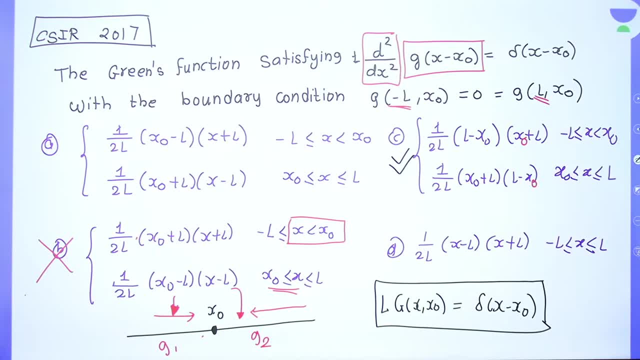 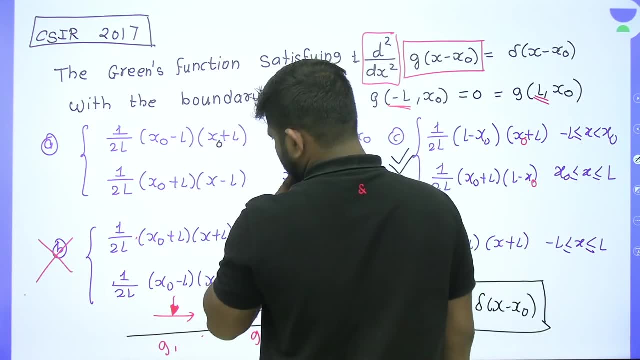 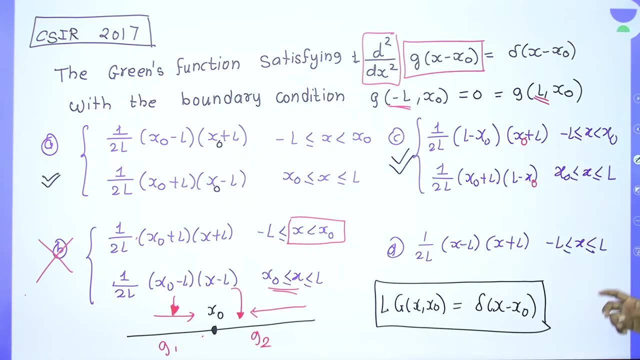 this is also possible. this answer is also possible in this: x0 put x0 instead of x. I put x0, x0-l, x0-l. same same. this also answer is possible. you are understanding right? ok, this is also possible. this is also possible. this is also possible. 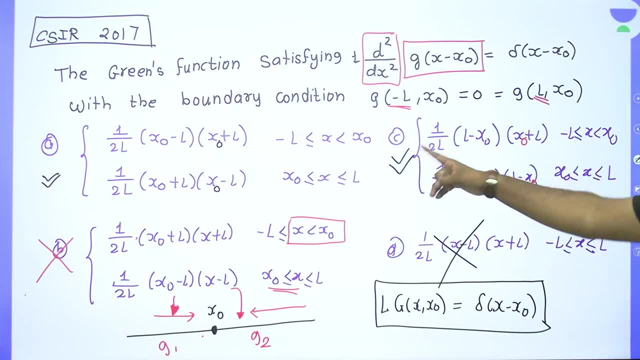 now in this option a and c, what is the limit of all this? limit is existing. if limit is existing, then what is your next procedure? what is the next procedure? what is the next procedure? amount of discontinuity. how much amount of discontinuity should be? what is the amount of discontinuity? 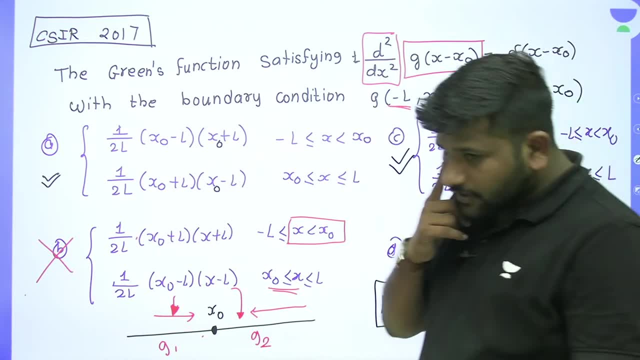 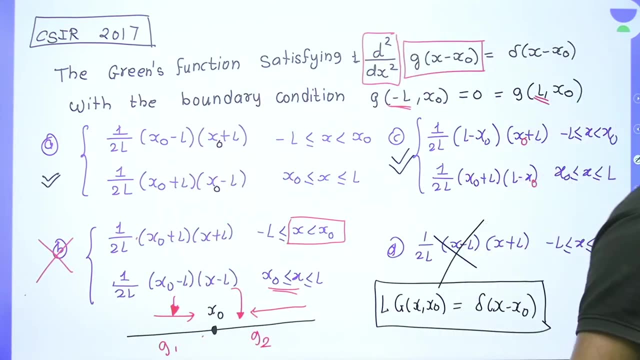 amount of discontinuity should be one. how much amount of discontinuity should be one? now check in option a and option c. now check in option a and option c. now check in option a and option c. how much amount of discontinuity in option a. how much amount of discontinuity? 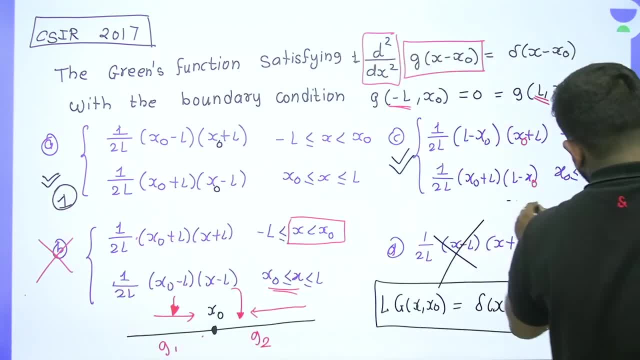 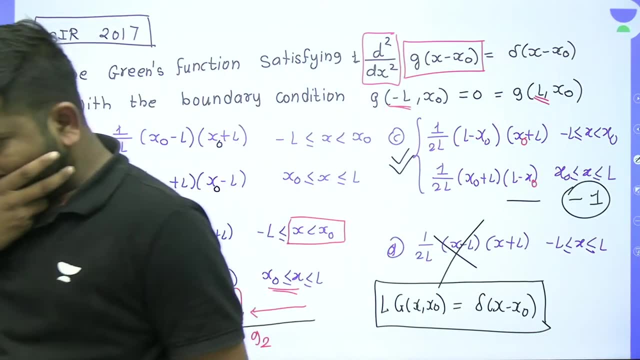 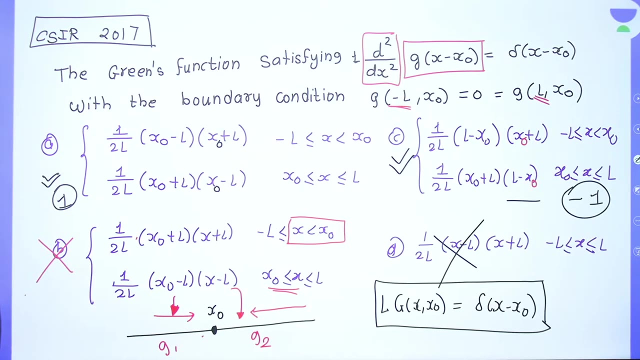 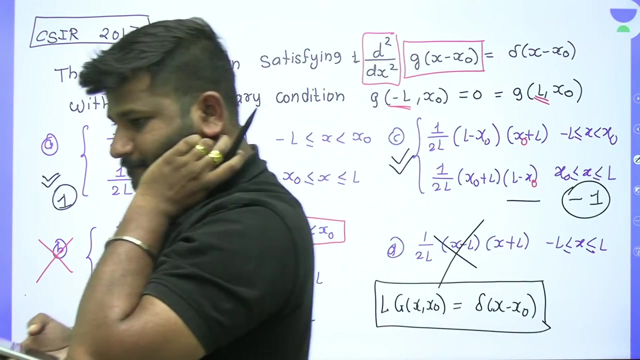 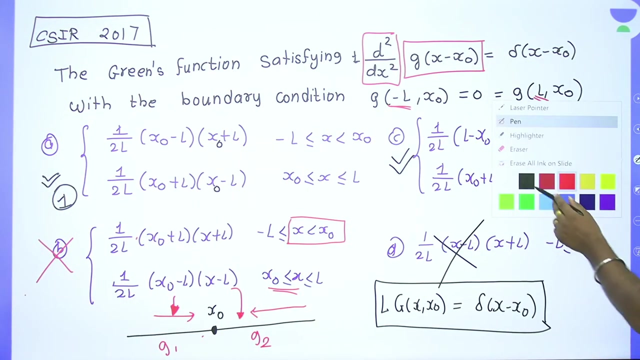 you will get one. and in option c, amount of discontinuity, you will get minus one. but amount of discontinuity plus one should be ok. ok, do you understand why option d will not happen? because if you take del g by del x, then del g by del x will be continuous at x is equal to x. naught, do it, do it, do it. 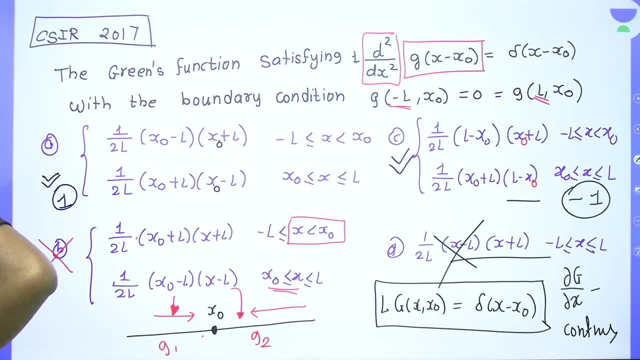 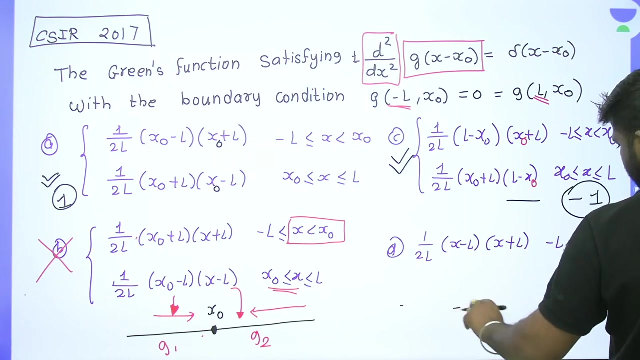 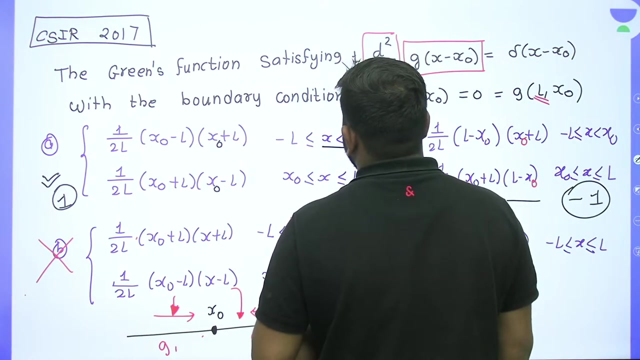 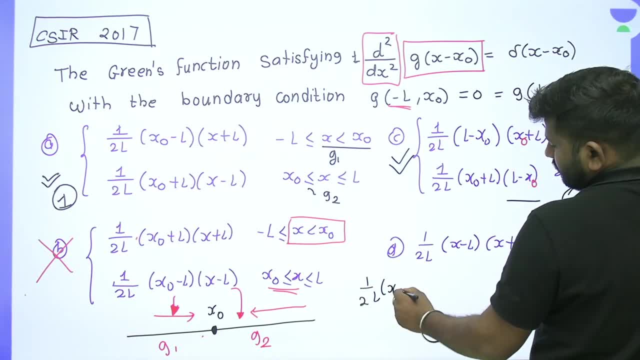 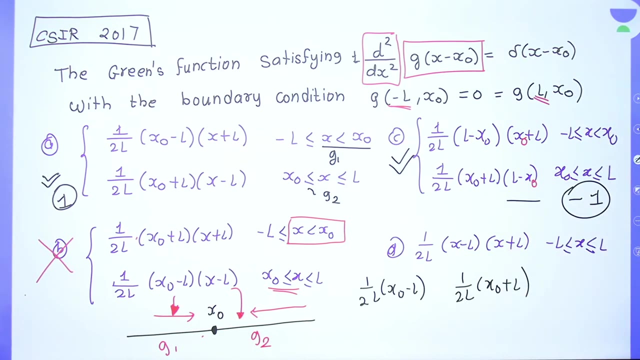 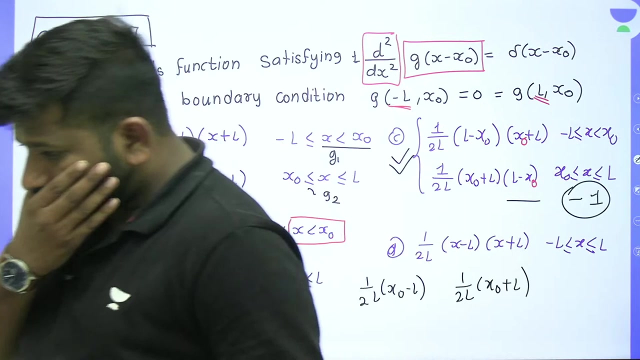 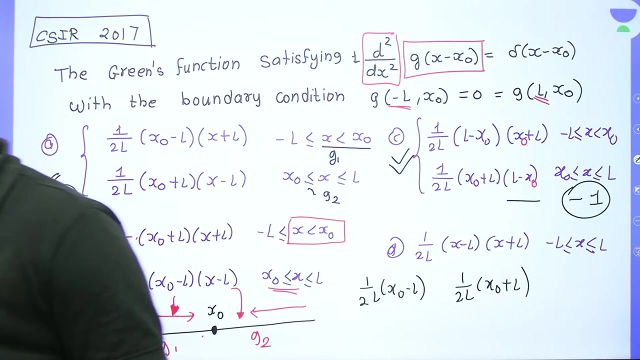 so what is the differentiation of this 1 divided by 2l into x0 minus l, and what is the differentiation of this 1 upon 2l into x0 plus l? and what is the differentiation of this 1 upon 2l into x0 plus l. 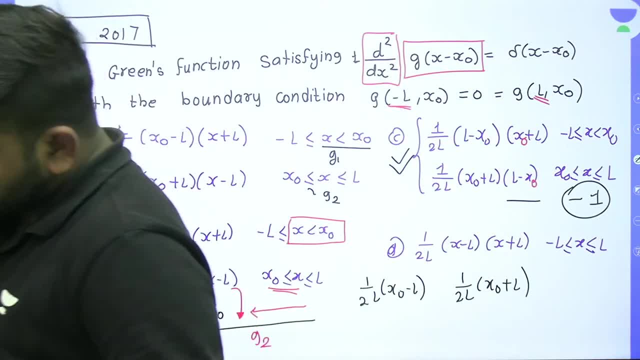 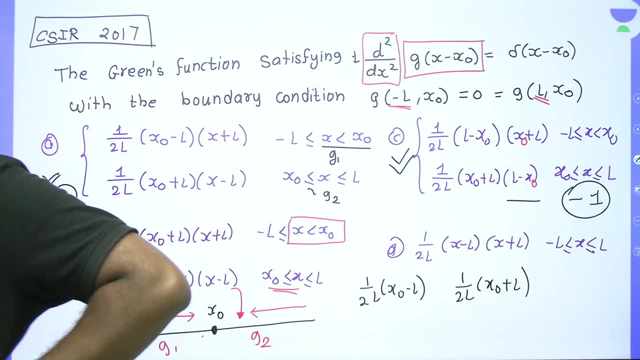 in both the regions. the Green's function is same. it may or may not be. it depends on the function. it will also depend on your function. what is your function? but most probably it does not happen. most probably 99%. some functions are such for which it may happen, but 99% it will not be the same. 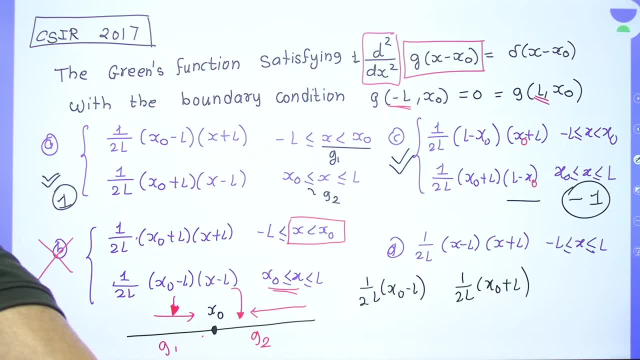 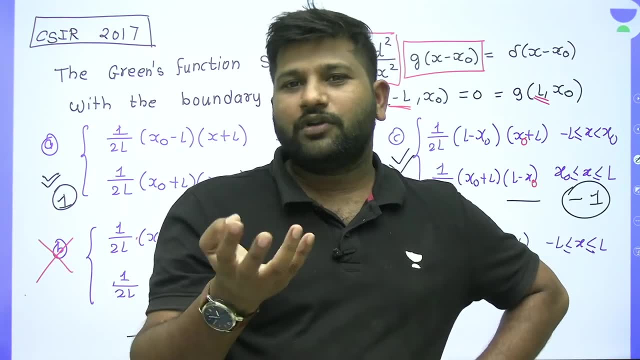 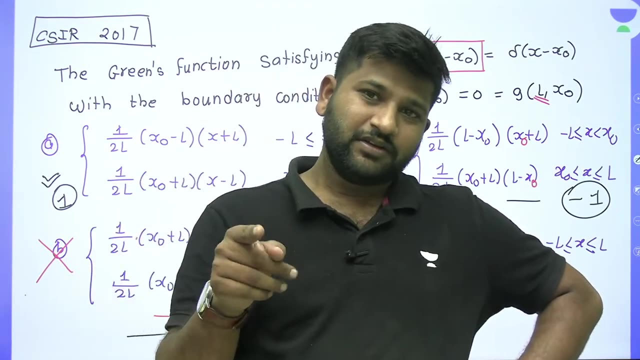 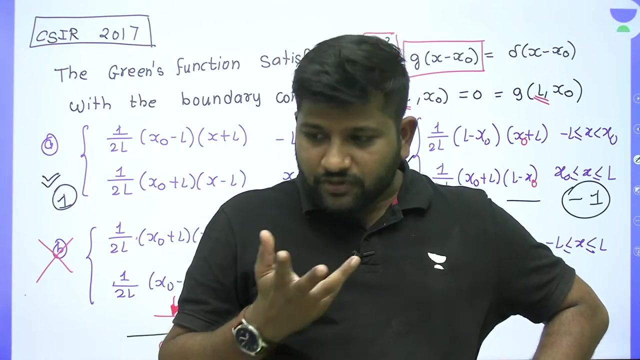 that means it is not the same. if it is the same in both the regions, then the amount of discontinuity will be 0, and if it is 0, then the coefficient of the second order derivative is 0, so your second order differential equation will not happen. 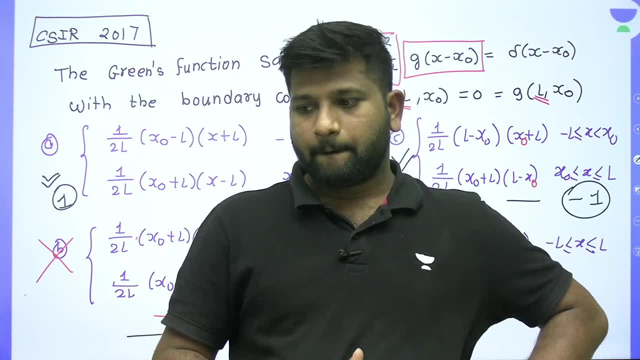 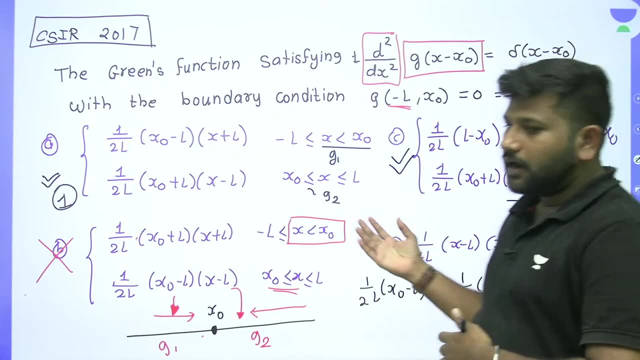 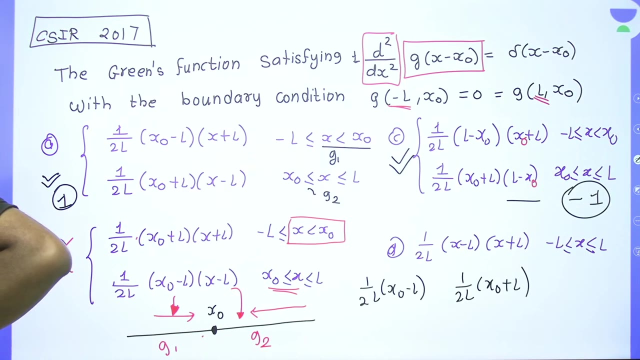 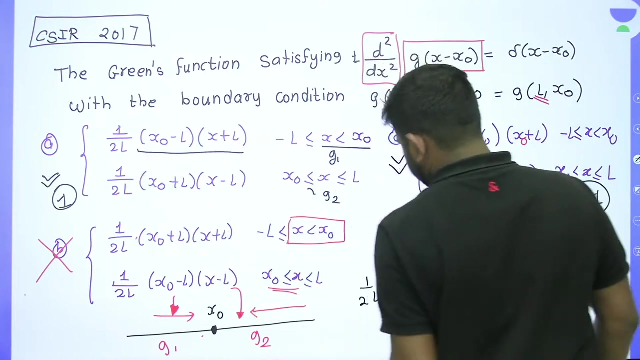 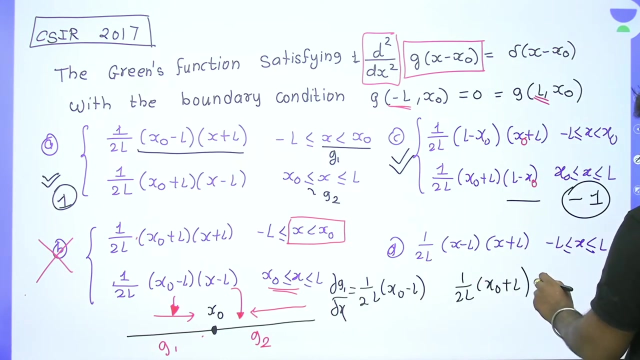 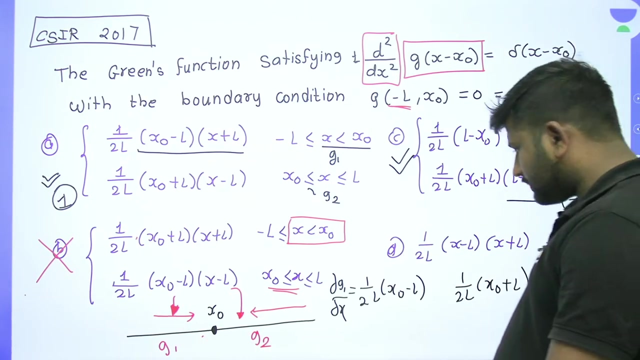 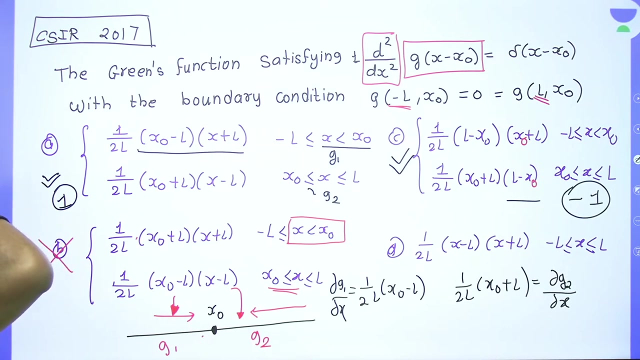 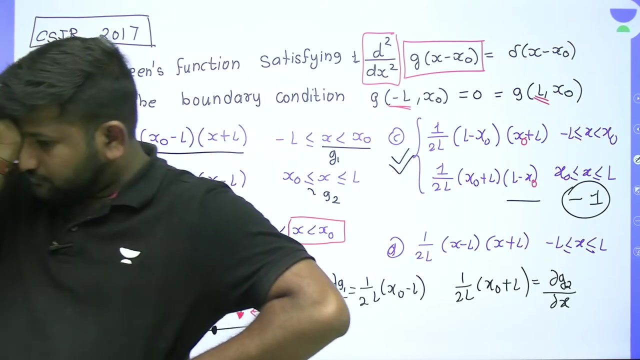 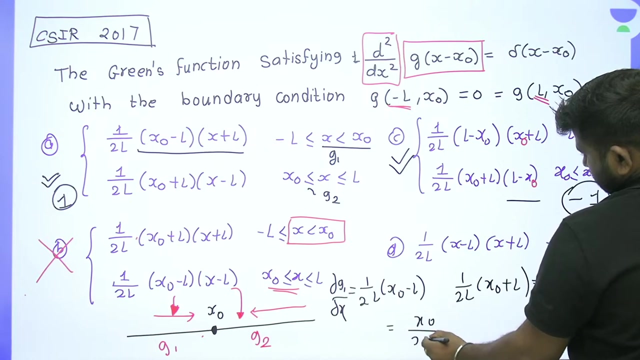 it will be your n minus 1. differential equation: continue a lost. there is some more fine. what is this? this is the del g1 and this is your del g2. by del x minus l upon 2l minus x, naught divided by 2l. 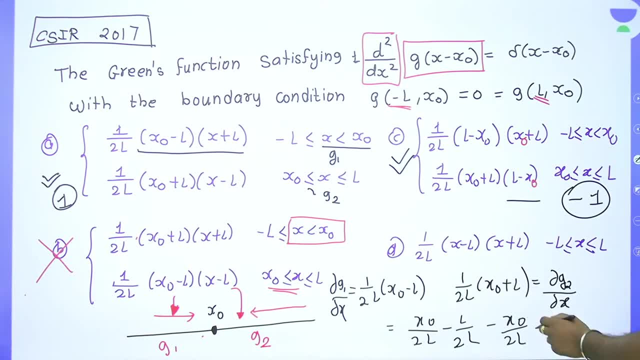 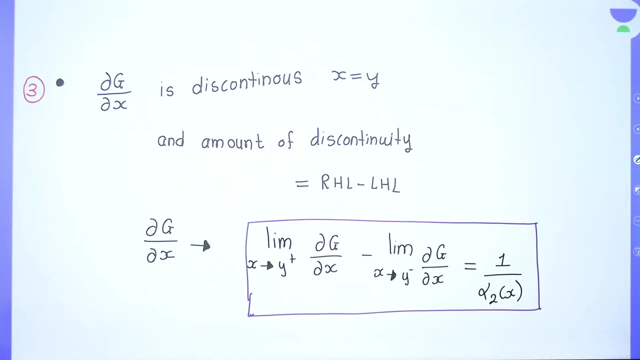 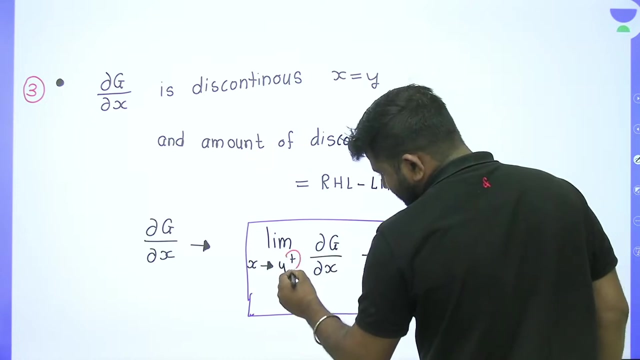 minus, because this is a minus. so this is l upon 2l, so this will be cancelled. is it getting minus? is it getting minus? is option a getting minus? no, it should be g2. this is a y plus. y plus means g2. 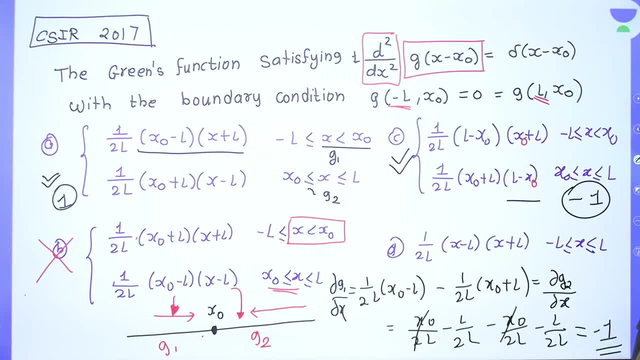 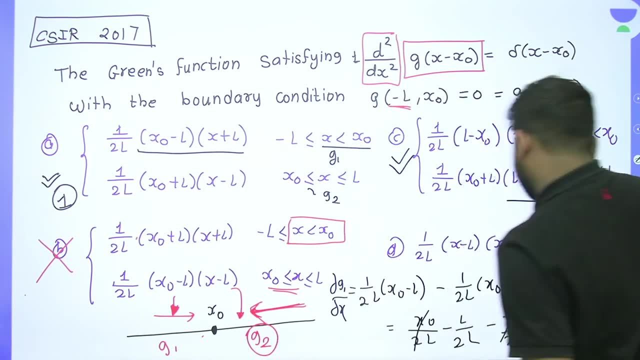 minus. sorry, here is g2, because this y plus means this one. this is y plus and we have called it g2, so it should be g2, g2 minus g1. so when we differentiate this, so when we differentiate this, we will differentiate g2. so g2 is this. 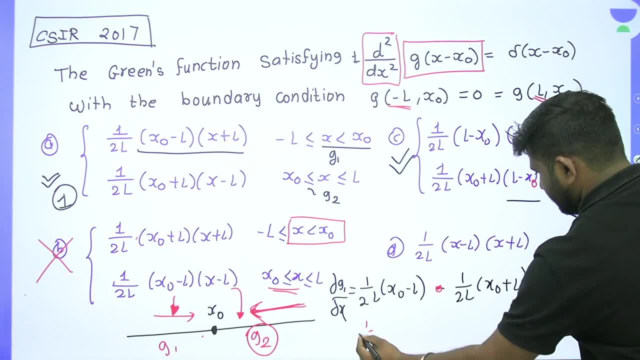 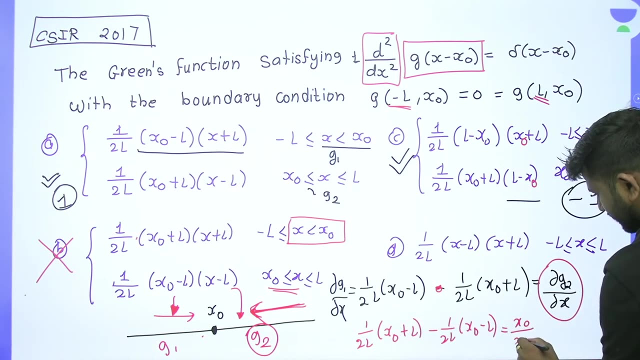 so what is this? this is 1 divided by 2l into x naught plus l minus g1. g1 is 1 divided by 2l into x naught minus l, so this will be: this is x naught divided by 2l. 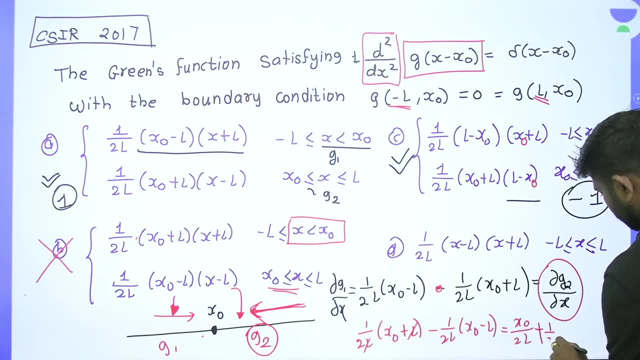 plus l upon l will be cancelled. 1 by 2 will be minus x naught divided by 2l, minus x naught divided by 2l. plus x naught divided by 2l. yl will be cancelled, so 1 by 2. 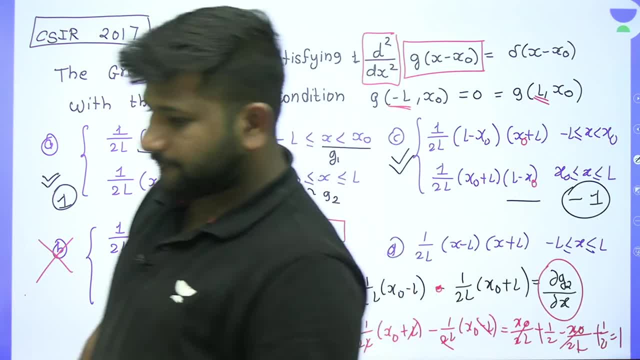 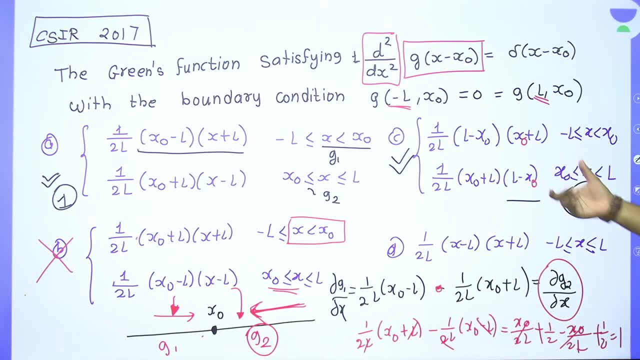 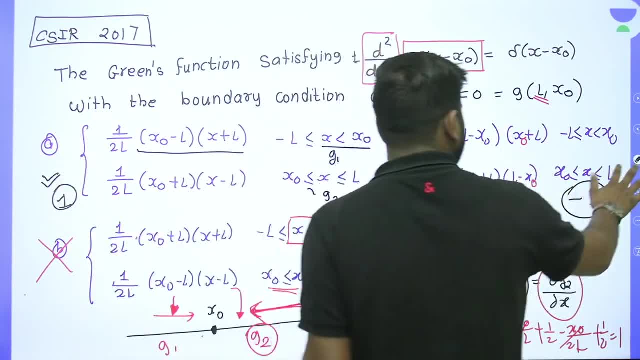 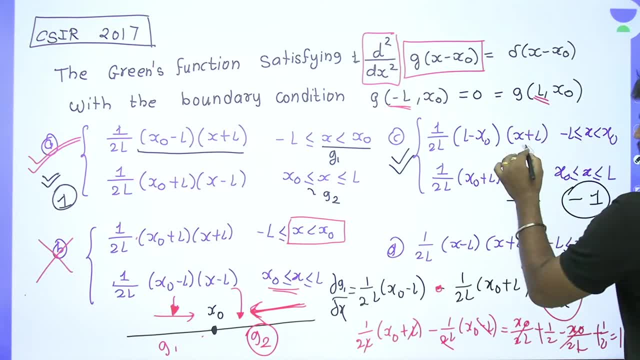 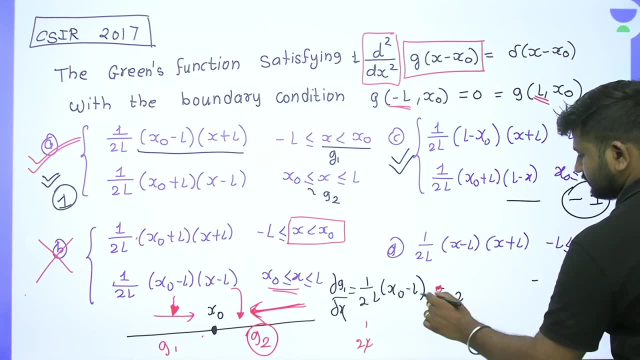 1 by 2 is 1. 1 by 2 is 1. Let's check for this. what is coming for this? I am erasing this right now. you must have written this. How much will it come for this? see now: this x is less than x0,. this x is less than x0,. 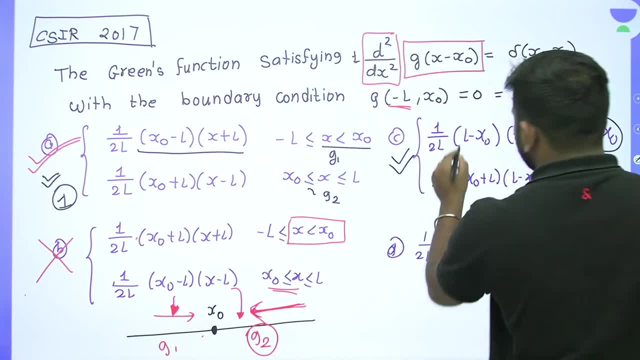 means which region is this? if x0 is greater, then this is g1,, then this will be your g1,, this is your g1, it is very important to understand that. what is g1,, what is g2, right? 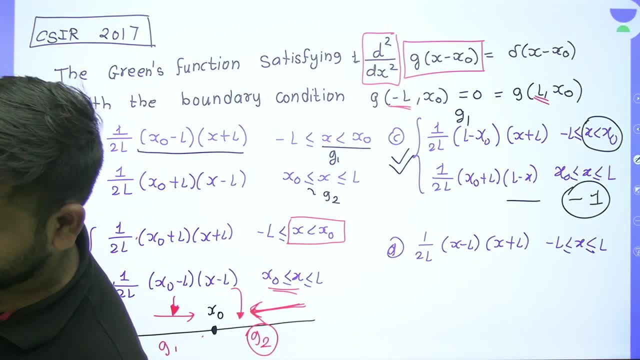 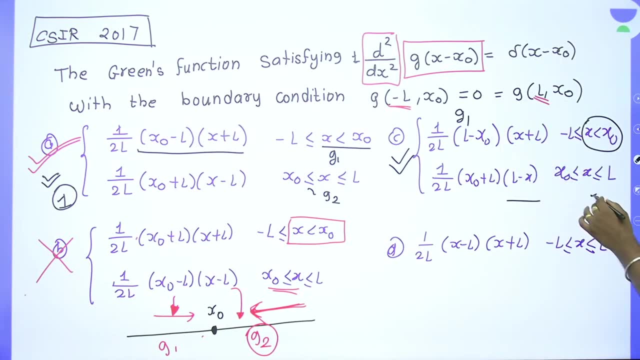 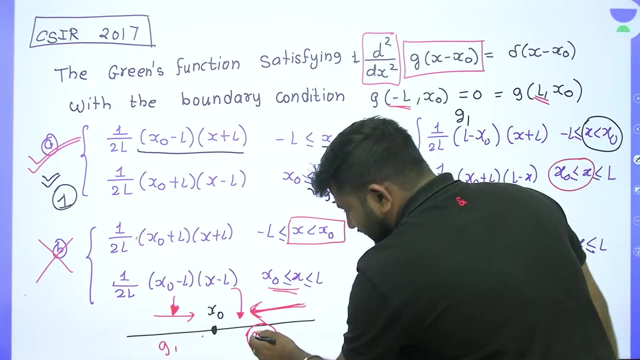 So, Nalai ji, good evening. it's late, the lecture is about to end. come on, still good evening now. if you look here, then this will come, and if you look at this one here, x0 is small. x0 is small means this region and what we called this region g2,. 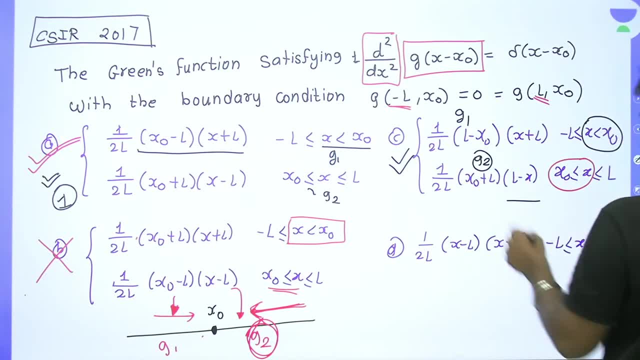 so this will be your g2.. So if you differentiate this, then how much will be its differentiation? Because g2, so del g2 by del x. if you differentiate this, then this will be your 1 divided by 2L, x0 plus L. this is constant. 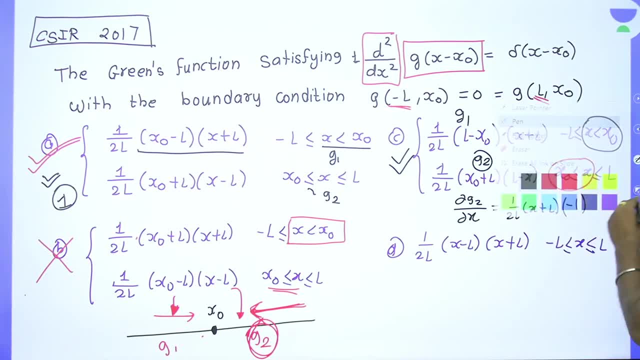 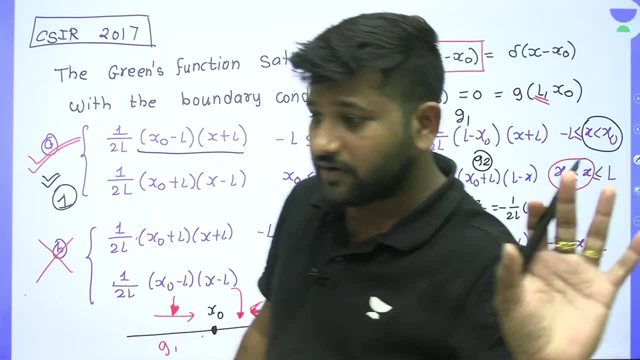 the derivative of L will be 0, minus 1, so this will be minus 1, that means I will write this minus 1 here. I will write minus 1 here. hope you understood this. Everyone is clear. See, here there is no need to find out the Green's function. you can directly find out from the limit, right? 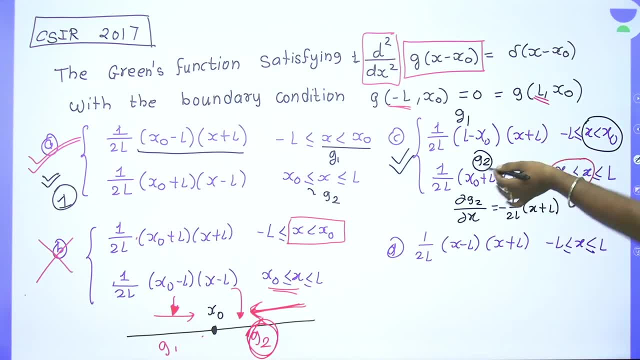 Come on, now this is done, and do its differentiation. so del g1 by del x. so how much will be its differentiation? So this is constant. that is, 1 divided by 2L is a constant L minus x0, this will be constant and its differentiation will be 1, L will be 0, that's it. 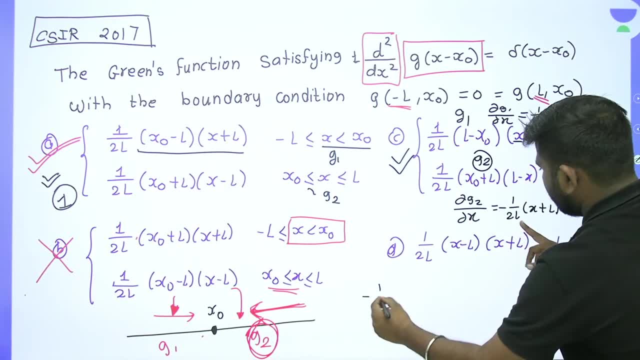 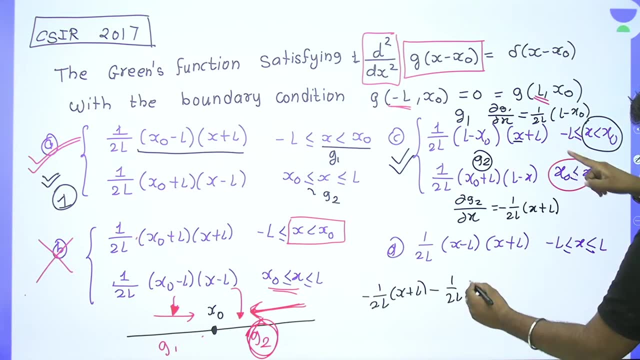 So you subtract these, that is, 1 divided by 2L into x plus 1.. 1 divided by 2L into x plus L minus g2 minus g1,. 1 divided by 2L into L minus x0, okay. 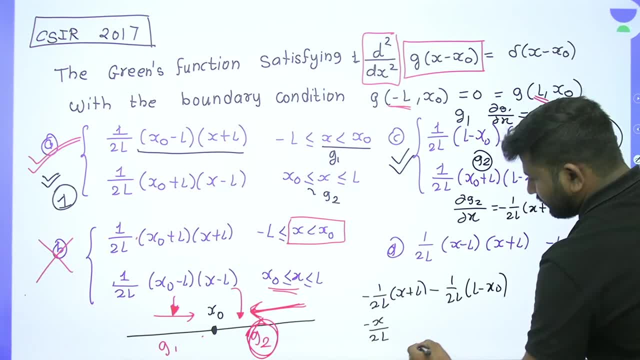 So minus x upon 2L. now this L will be cancelled minus half. okay, This L will be cancelled minus 1 half, and this minus minus plus will be x0, x0, right, x0.. 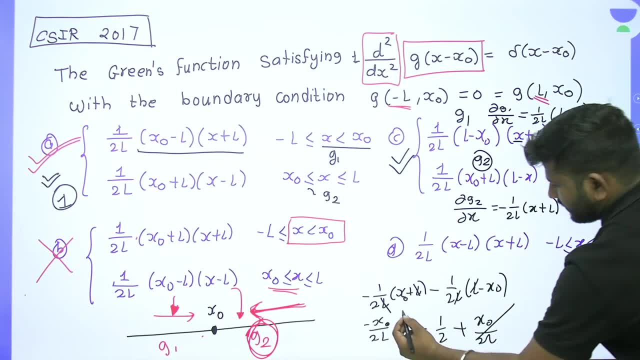 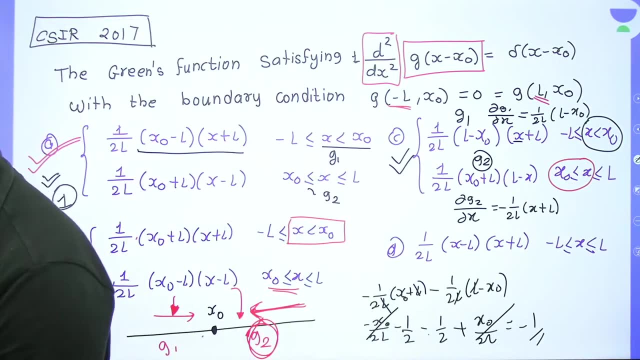 So x0 by 2L, x0, x0, cancel, x0, x0, cancel. Minus half, minus half, minus 1.. What amount of discontinuity. How much should it be Plus 1.. 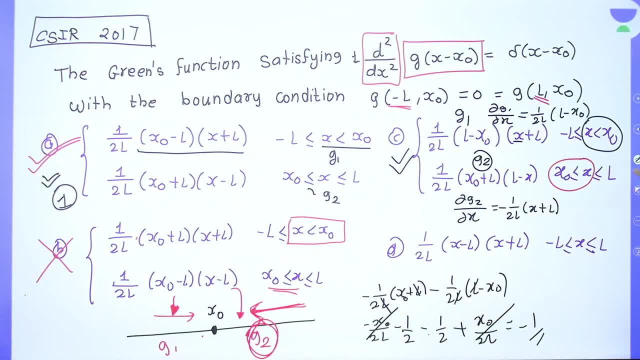 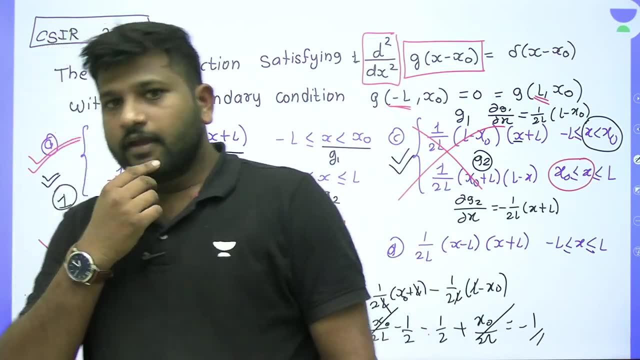 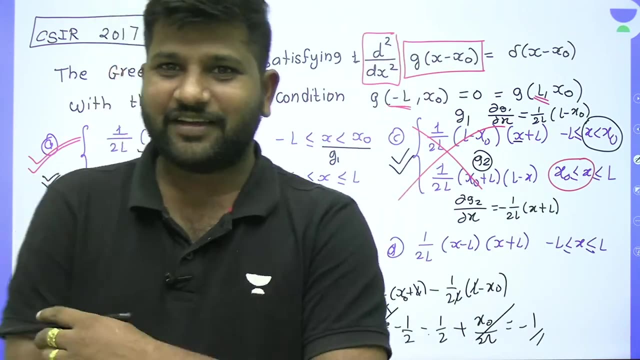 Okay, How much should it be Plus 1.. How much is A Minus 1.? Will this be the answer? Absolutely not. So this is also gone. Okay, Now don't do A. I will give you a homework. do it after CSR, don't waste time in it. 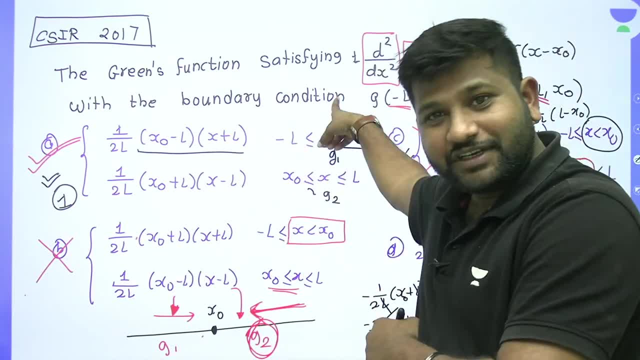 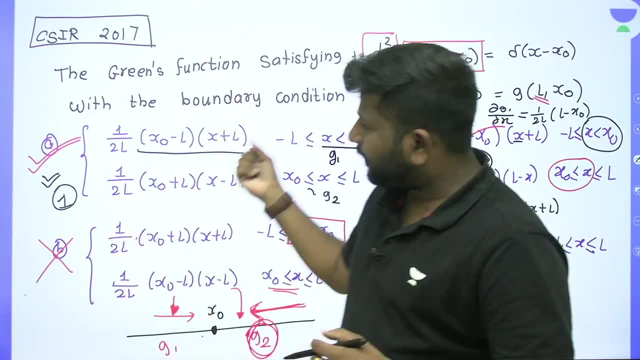 These when we did the procedure right. Solve it with that procedure? Your answer will be A Okay. Solve it with your method? Your answer will be A. The method we did before. 4,, 5, 6 steps. problems can be solved. find out. go, go, go go. 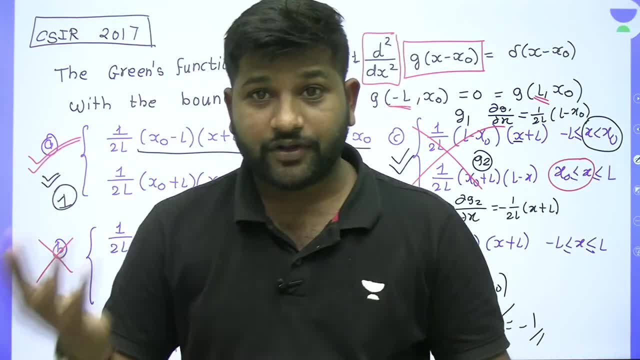 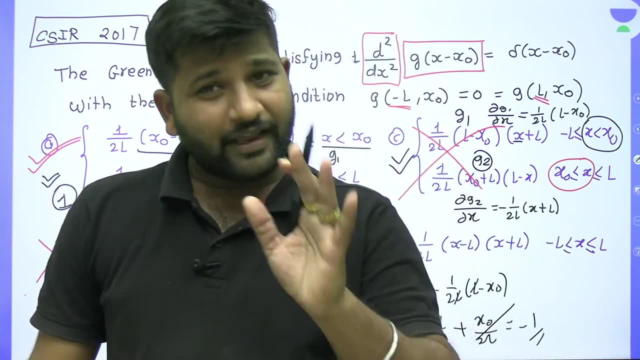 You will think that, sir, this condition you have used, it took so much time. You don't have time at all. If this question comes, then see how much time it will take to solve this question. I say: how will this question be solved? 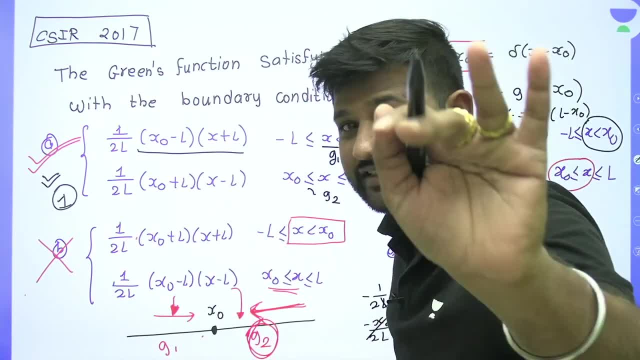 See, this question came in CSR. so what will we do? We know the limit should exist, so it is necessary to solve it. It is also visible from here. If you put this, then this limit should also be solved. See, this is the limit. 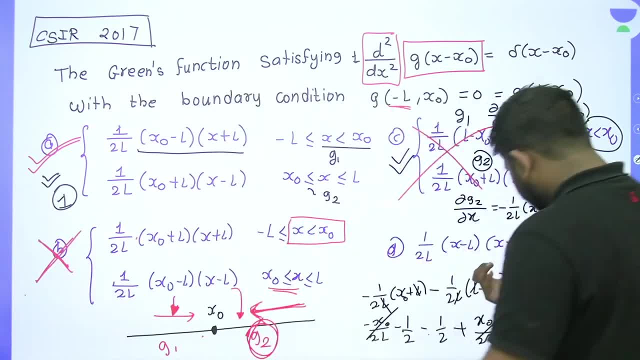 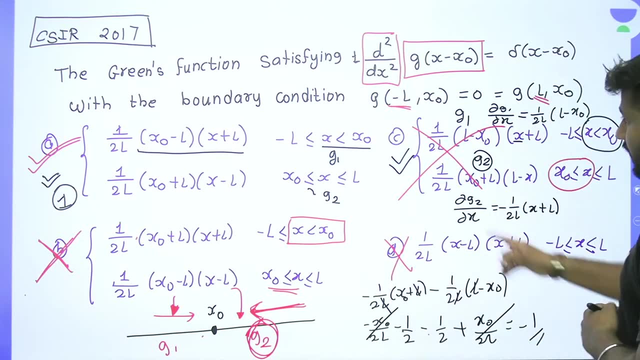 If you put this, then this limit does not exist. This answer went here. If we did its differentiation, then its differentiation. what will be our differentiation? It will be continuous here. So this option will not be there. And as for the option C and D, we will check the limit. 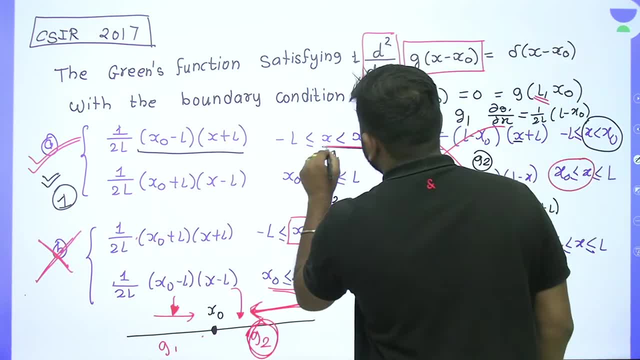 If we put X to X naught, if we put X naught, then RIS is coming. So from here we will think that this is it, this is it. So its differentiation happened quickly, in 2 minutes. How much time did it take? 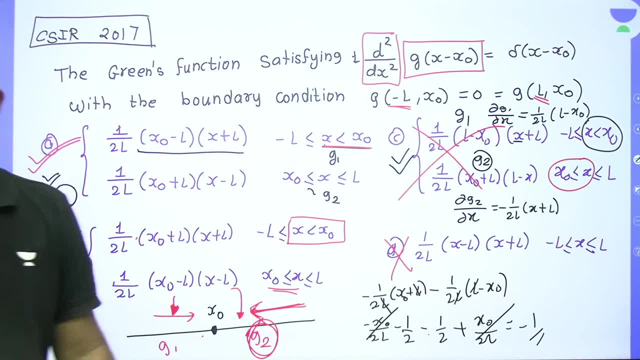 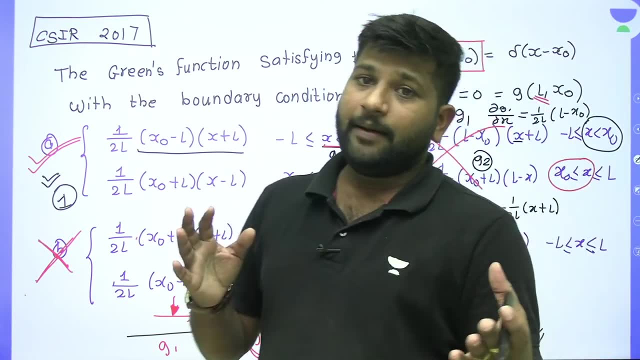 I think this answer will be there in 30 seconds. Who said Green's function is difficult? No, not difficult, Very simple, But I hope you understood. Okay, I hope you understood this. With this, you can also find out from the properties of Green's function what your answer will be. 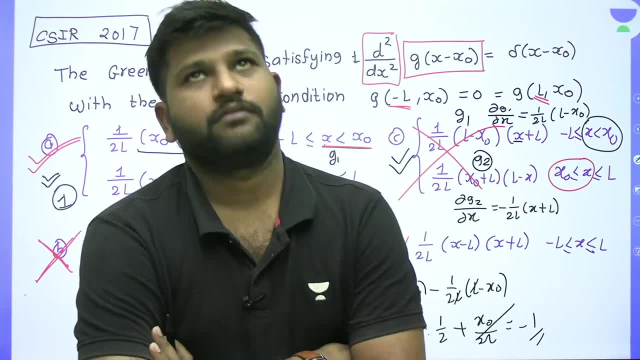 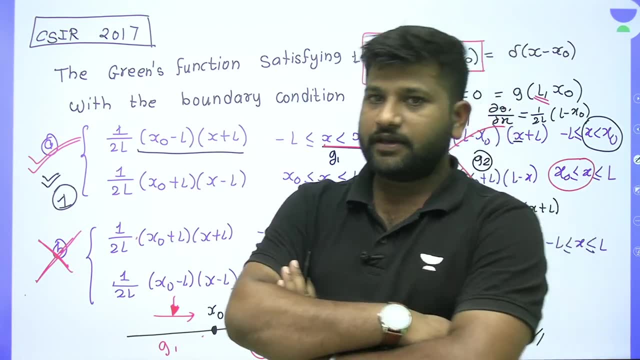 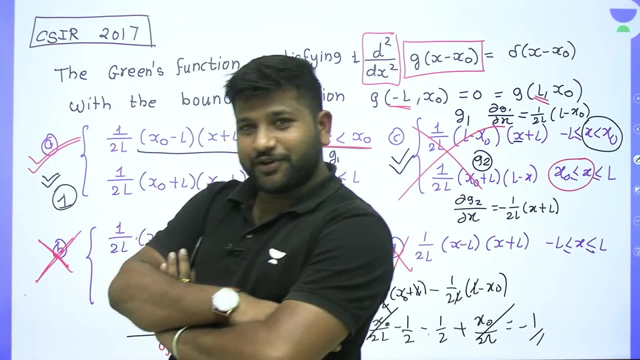 With the help of properties of Green's function. Is everyone clear, Any difficulty? If anyone has any difficulty or doubt, then you can ask: Okay, Now this is Green's function If we want to find out the solution of this differential equation. 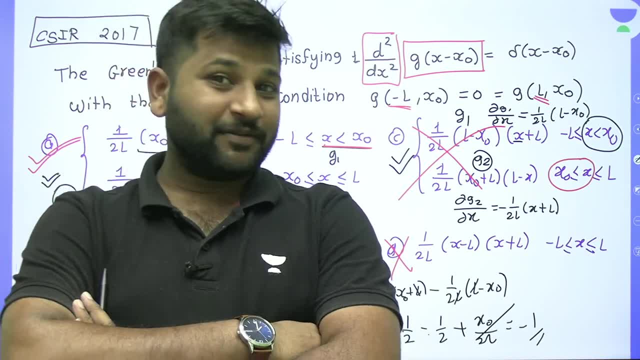 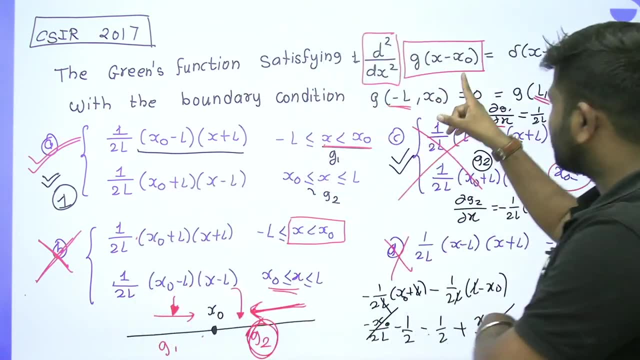 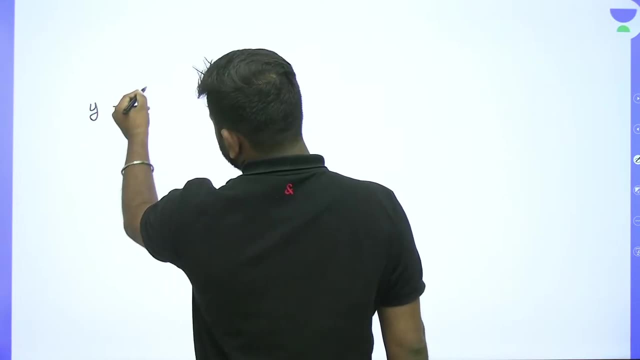 Then we have to find out the solution Now. how will we find out? If you want to find out the solution of this differential equation, Then for the solution of differential equation, let's say Y, So which is equal to your integration. Here is your Green's function. 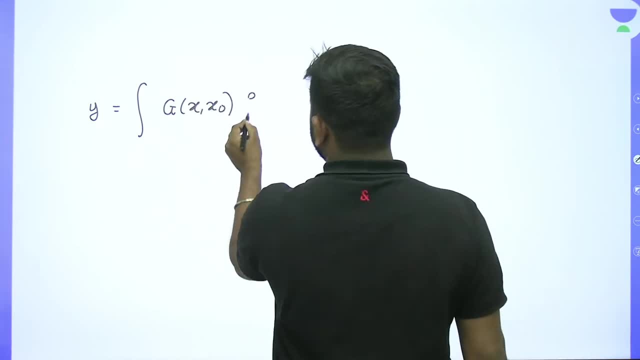 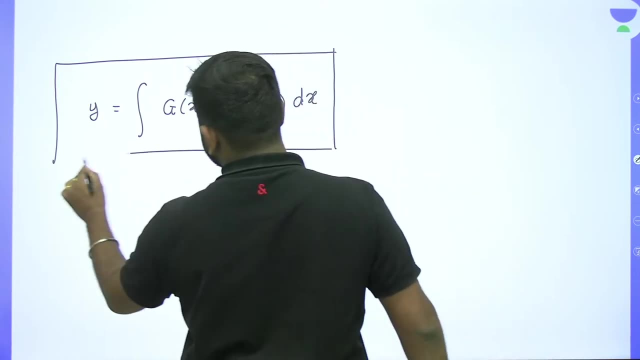 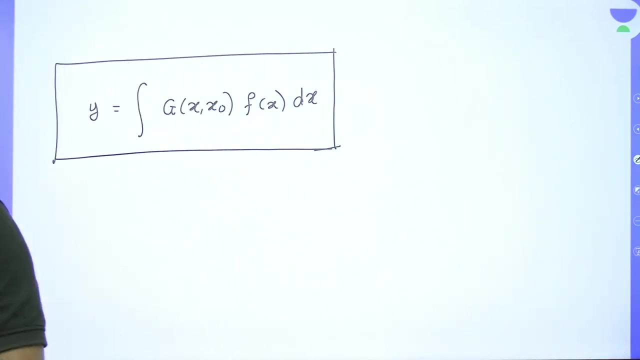 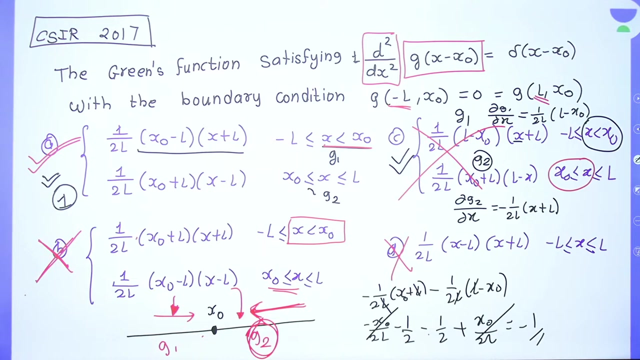 And your f of x is your f of x into dx and solve this integration. that will be your solution. ok, and this is the solution from the general method. one minute? no, it will not happen from the general method, because here, directly, they have given you the greens function. ok, you understand what is happening. 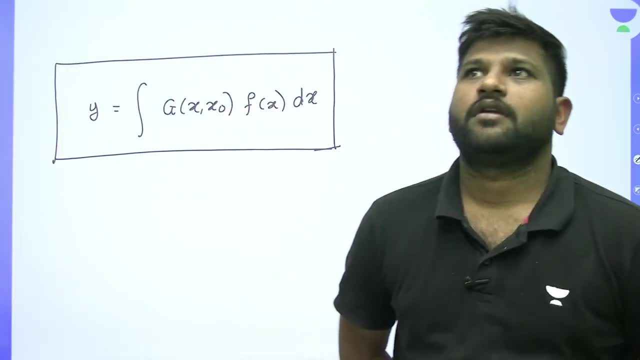 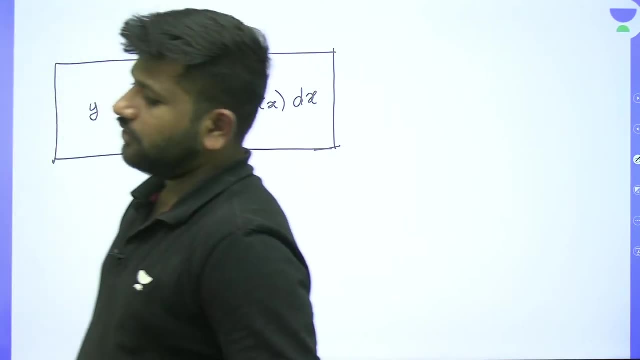 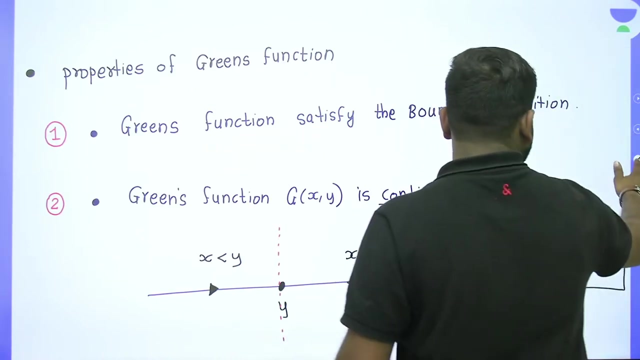 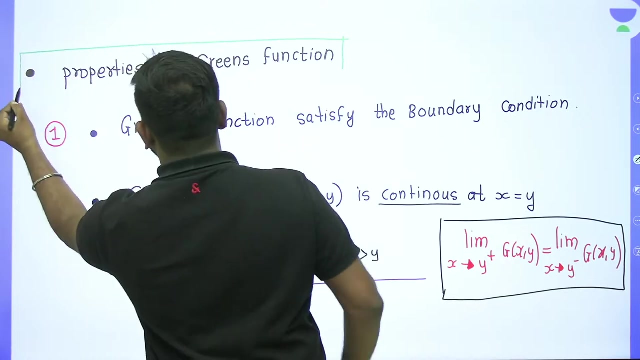 no, because why not? given understand everyone, then keep an eye on them. this is, according to me, this is a very useful thing. that is, the properties of greens function. so the properties of greens function is a very important thing, because from here you go to the question. 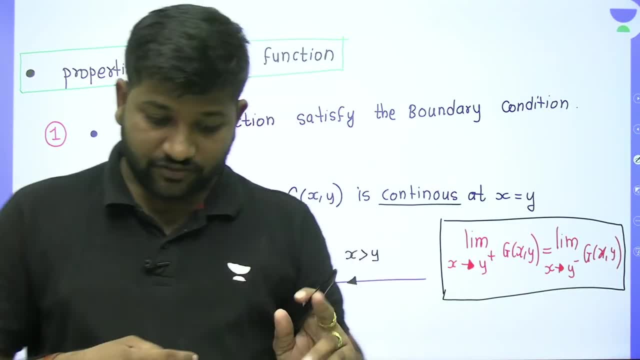 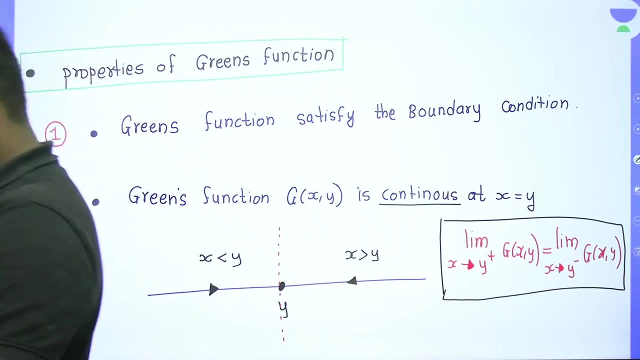 you can save it quickly. so these are the two types. ok, so this is the first method from which you can find out that this is someone else. free doubt. so why not take this? then we'll stop here and we'll have one more session on greens function tomorrow, speaking. 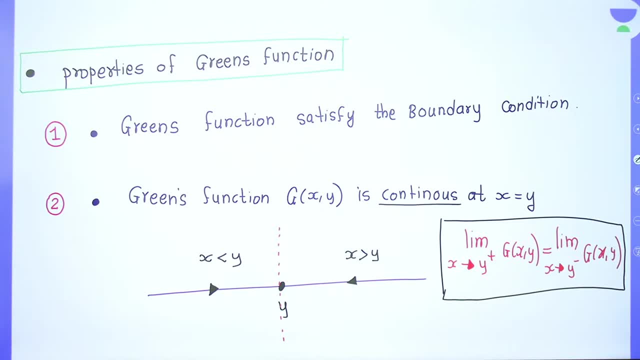 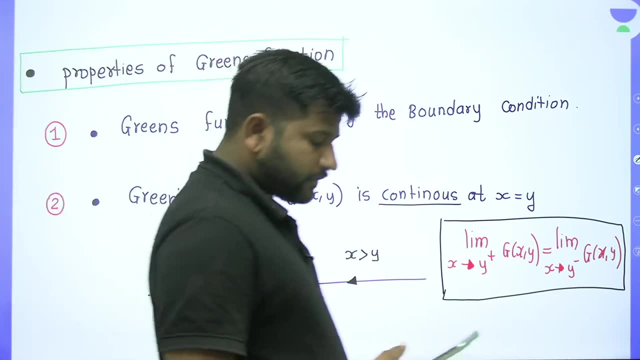 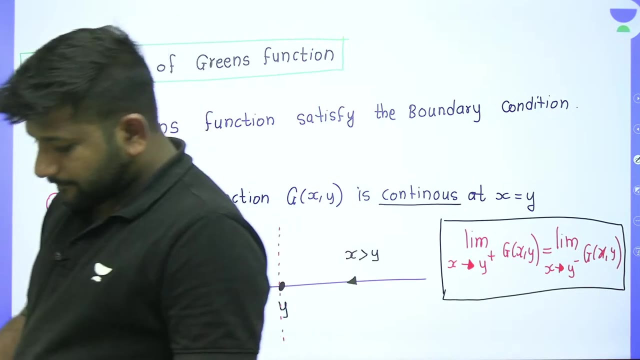 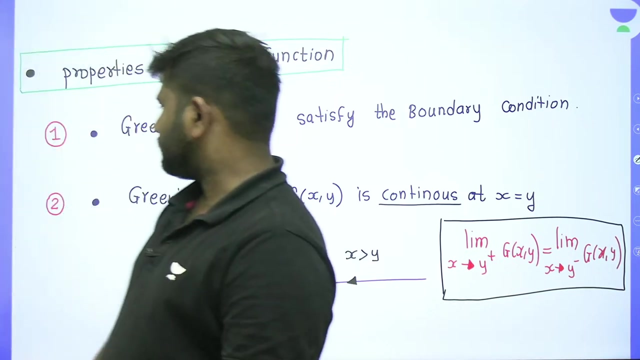 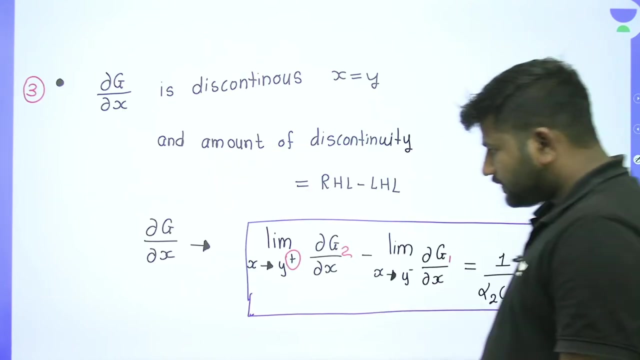 to do our session the way it is done, it is enough to do the same thi y. so this is our session. Byeرة App-Future viewers tomorrow 6 pm. and this is a condition. so should I write here that this is for the x? 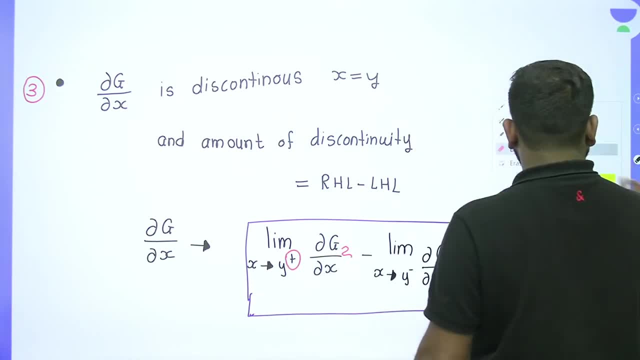 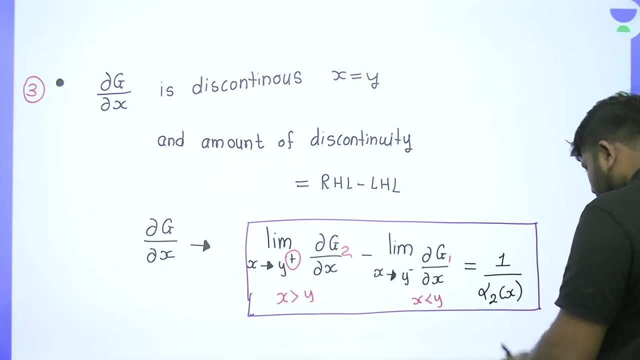 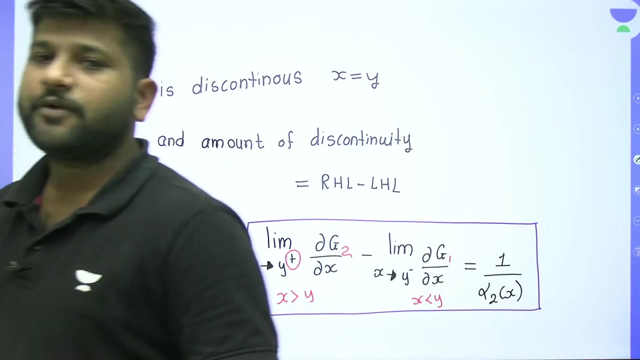 greater than y. if you are getting confused, because here only this greater than and less than is a game. this is x greater than y. this is x less than y. the amount of discontinuity should be this much. ok, we will solve the solution problem now: how to find out the solution of. 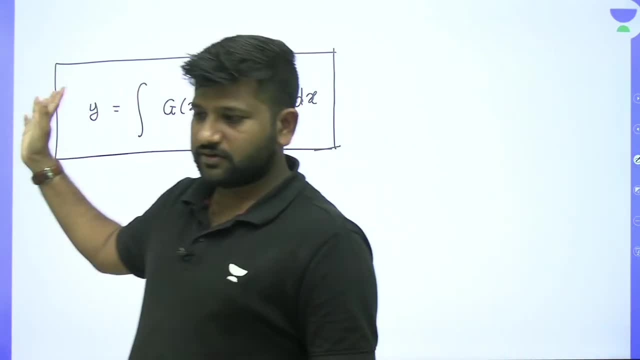 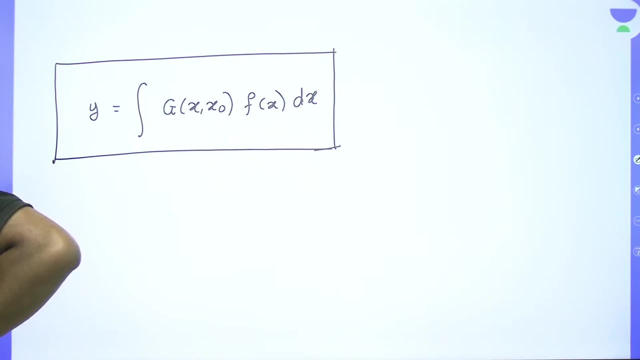 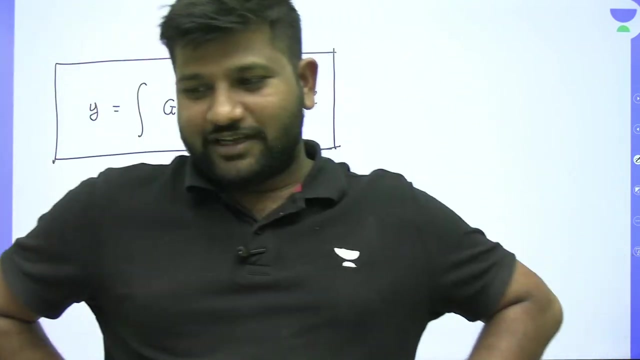 the different green's function. we will discuss tomorrow how to find out in the green's function. ok, if anyone has any problem or any doubt, right, because csn is a function of x greater than y and if it comes to its 5 mark, then it will be good. right, you will also get 5. 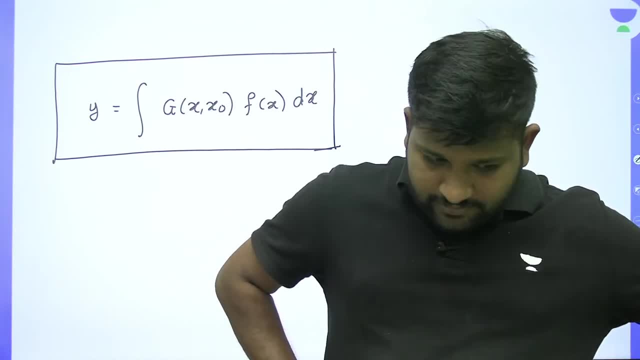 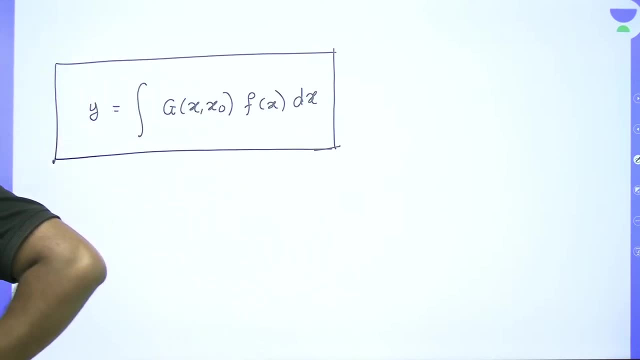 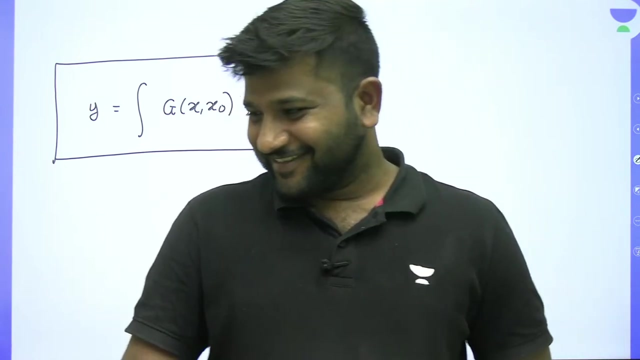 marks. i am also happy the math physics is just a little big, ok, but numerical analysis and green's function. you will definitely get one 5 mark question from both right, and I hope everyone's preparations will be going well. everyone will be feeling pressured, right, right. so if any of you are doing good, then I would recommend this tutorial for everyone. OK, bye. 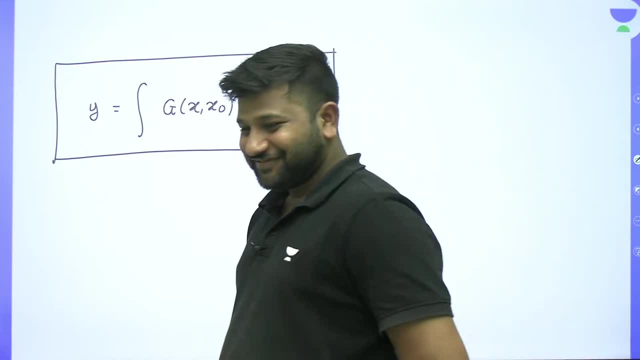 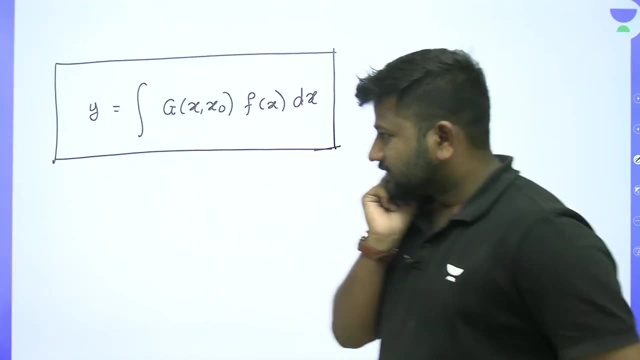 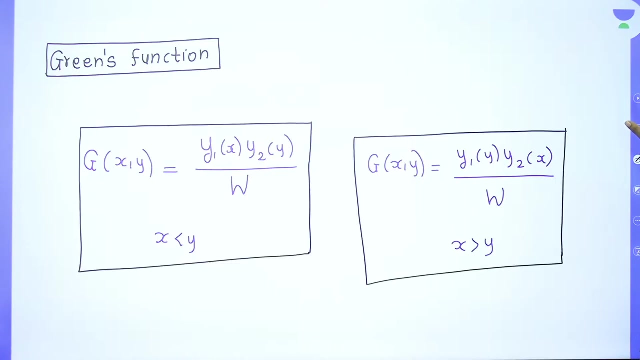 bye, don't worry, don't get tensed. hmm, hmm, ok, so that's it. we will discuss this much in today's session. the rest we will discuss in the next session. so in the next session we will discuss the rest. I hope you understood this. revise these notes. 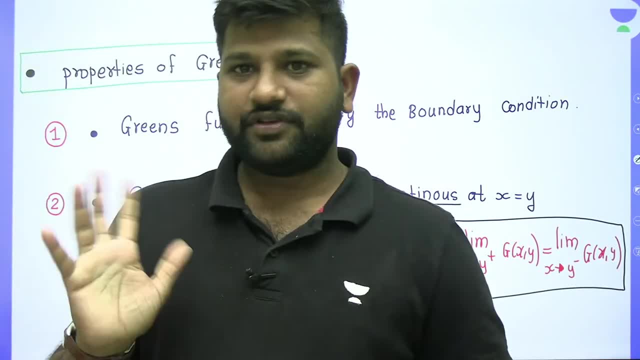 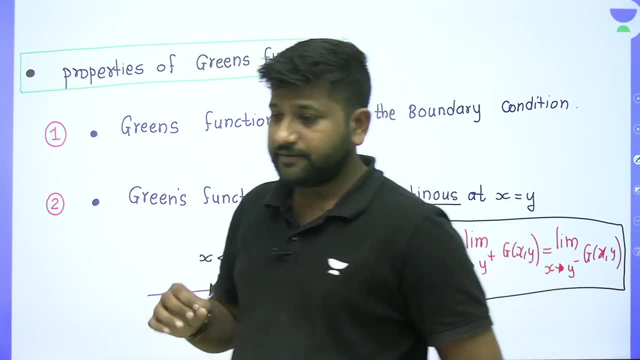 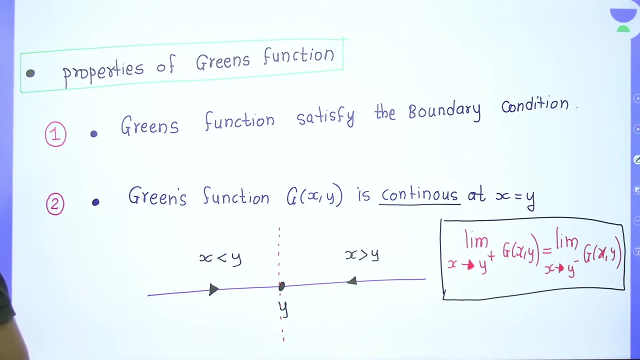 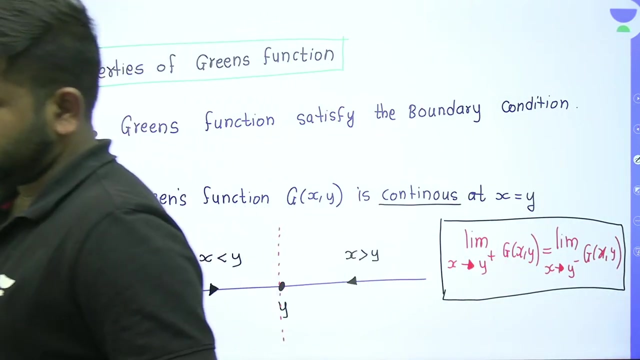 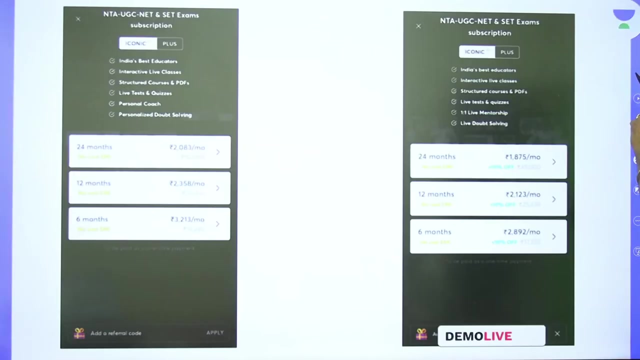 because revision before exam is very important. so the revision you do, don't leave the revision. if you revise, then only all things will be possible. ok, anyone has any doubt? ok, that's it. so we will stop here for today. in the next session- hmm, we will discuss the rest. 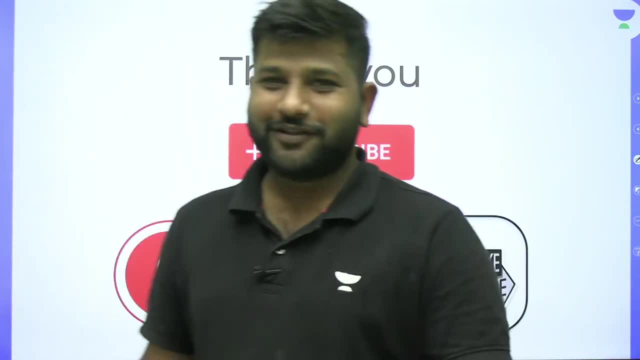 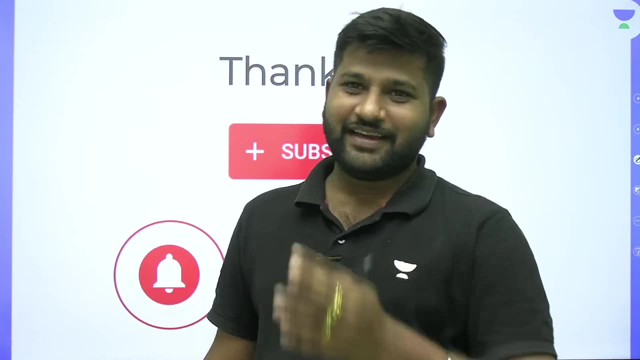 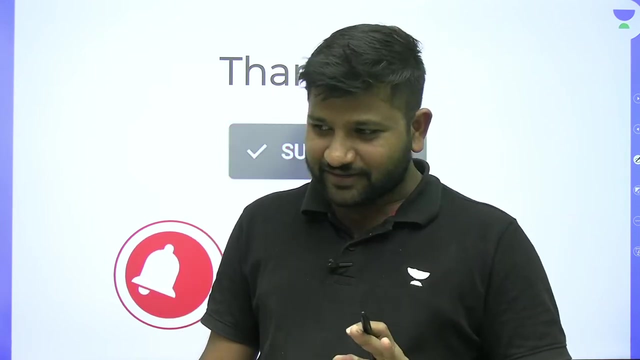 and all the best for your exam. for your exam, give good exam and revise all the subjects as much as you have studied and don't feel pressurized. do it as much as you have studied. hmm, to qualify for CSR, you don't have to know all the subjects. 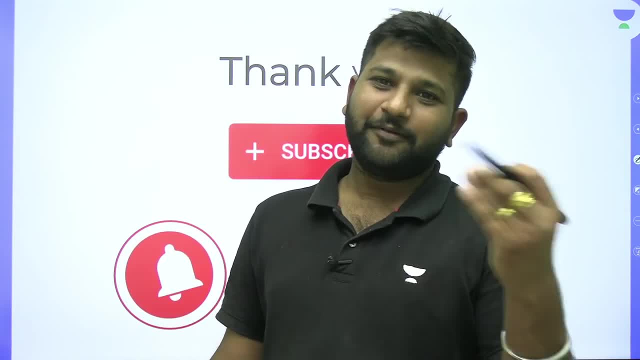 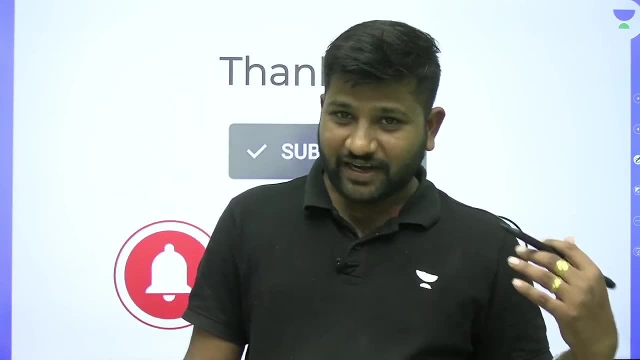 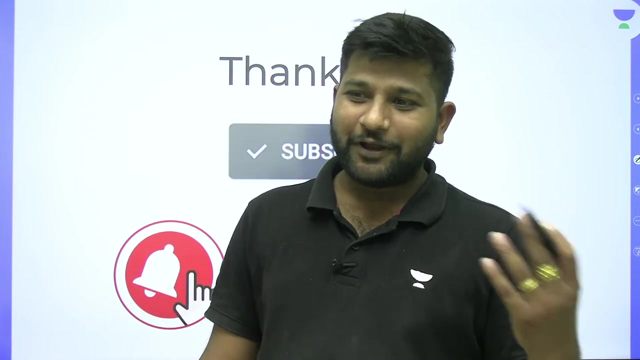 not necessary. if you are good in 3 or 4 subjects, including part 8, then it can be done easily. revise all the subjects, let's say you don't have to feel pressurized. hmm, you know, it's like before the bump comes up, you have the same. 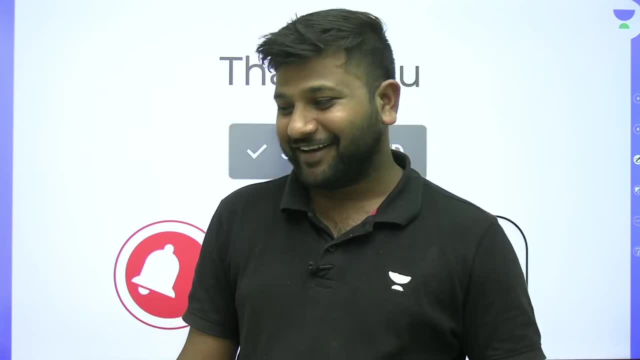 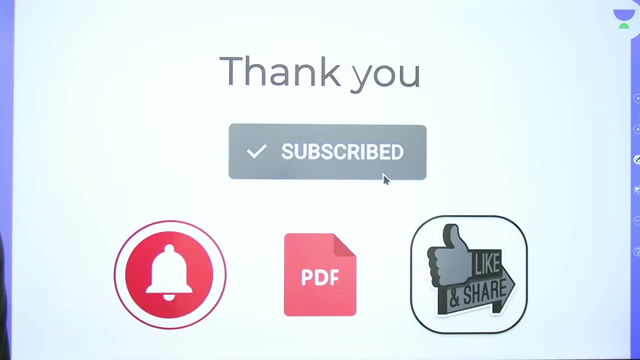 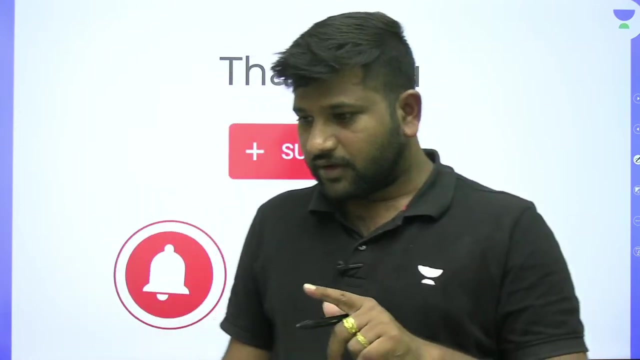 if you qualify, then the bump will come up. so believe in yourself. believe in yourself. there are 2 and 3 in the boundary condition. so, yes, if there are 2 and 3, then 2 is lower boundary and 3 is upper boundary. hmm, 2 is lower boundary and 3 is upper boundary, correct? 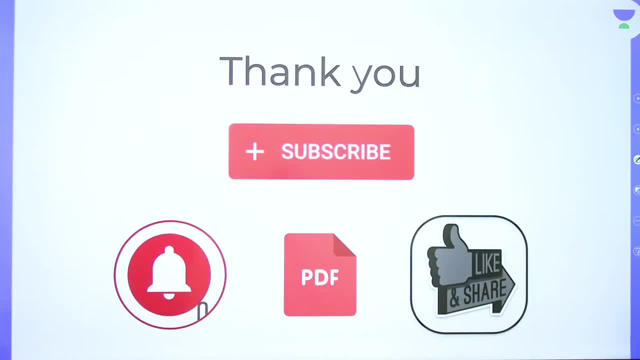 ok, hmm, ok. so if anyone else has any other doubt or problem, then ok, or else we will stop here. ok, bye, all of you, take care, bye, all of you, take care, bye, all of you, take care, bye, bye, bye, bye. 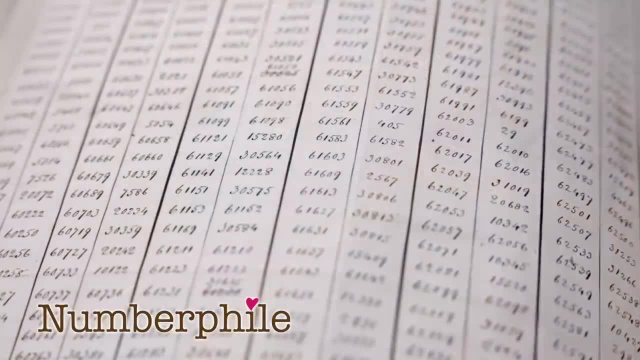 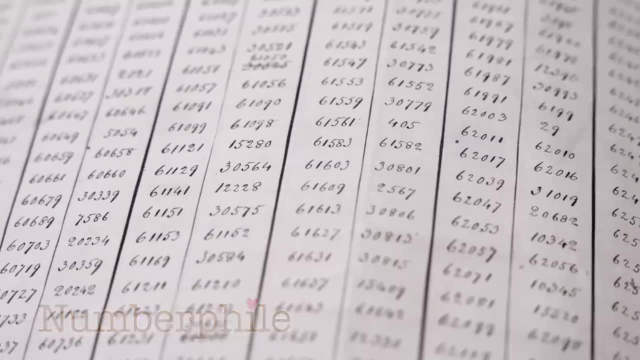 What's today's video about? What have you got here, mate? So this is the handwritten results from a mathematician who lived in the mid to late 1800s, a gentleman called William Shanks, who I think in the modern day we would call a recreational mathematician. 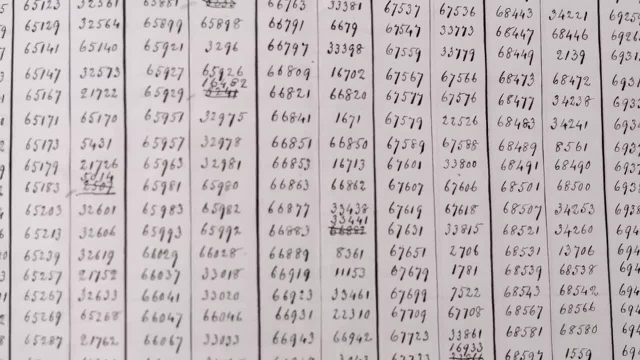 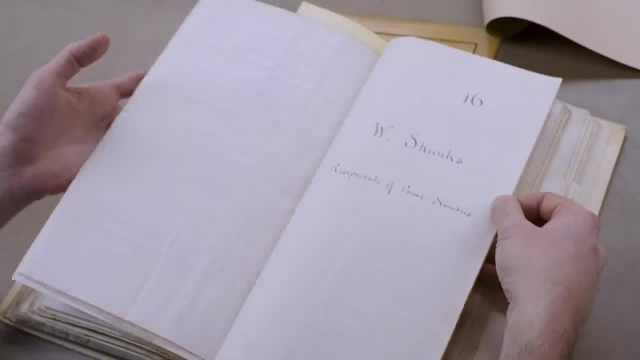 He had a real job, ran a boarding school. In his spare time he just did calculation after calculation. William sent all of his incredible results into the Royal Society. Here we go. So this is W Shanks Reciprocals of Prime Numbers. 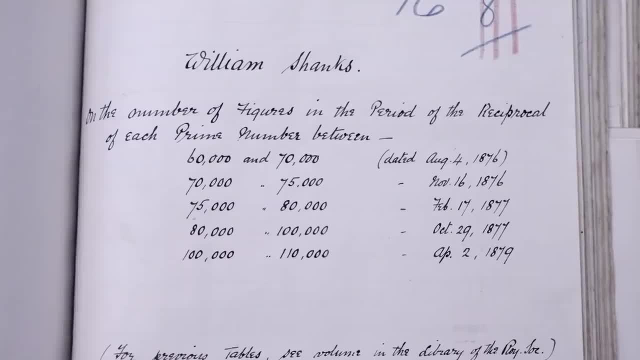 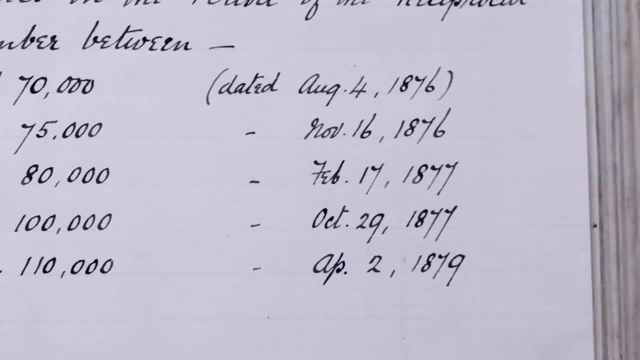 And then what follows is- and these are the sections and when he did them, so you can see- he's got them in batches of 10,000 to 5,000 at a time, and this is across years. This was not a fast process. And then here's what he found: